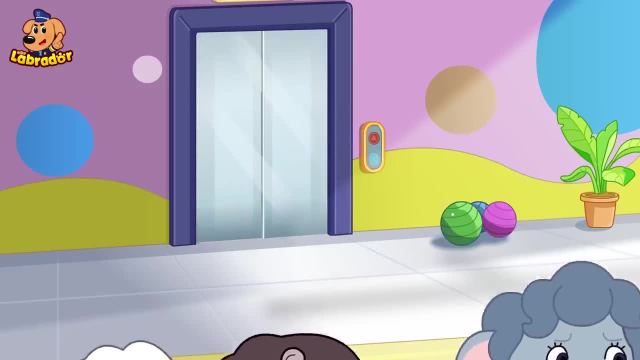 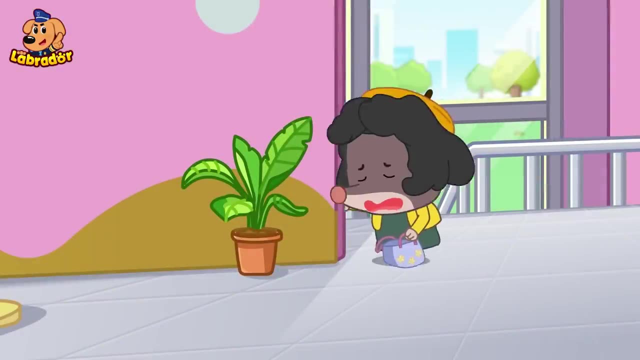 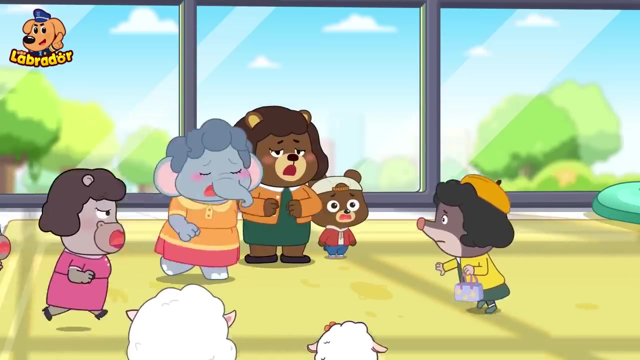 I'm going to the hospital. How did she get hurt? Hope she'll get better soon. Miss Mole, I thought you were at the hospital. I'm not hurt. Where's my son? Someone took him to the hospital to find you. 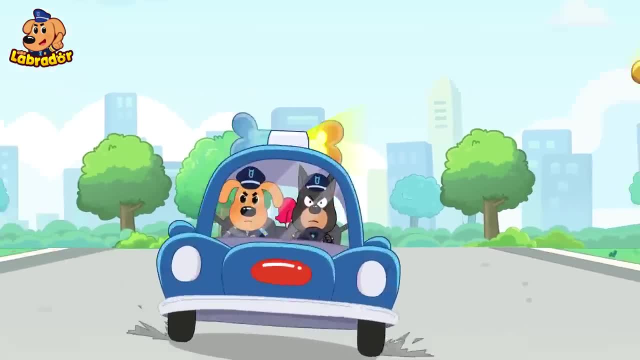 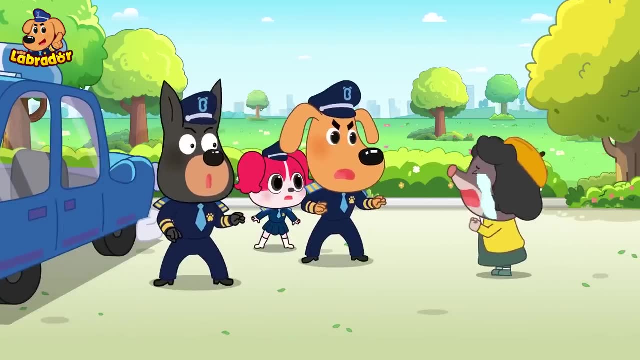 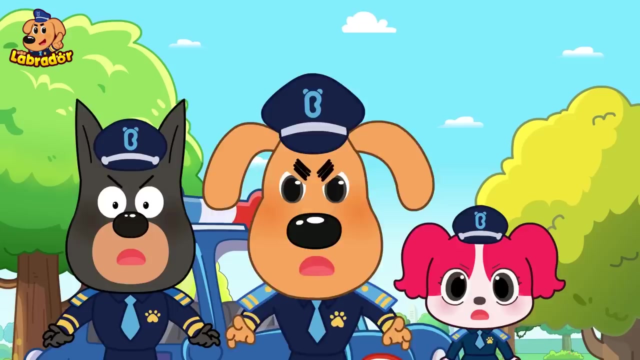 What? Sheriff Labrador, please help me. There's someone claiming to be a friend of Miss Mole. She took Little Mole to the hospital saying that his mom got hurt. That sounds like a scam. Which way did they go That way? 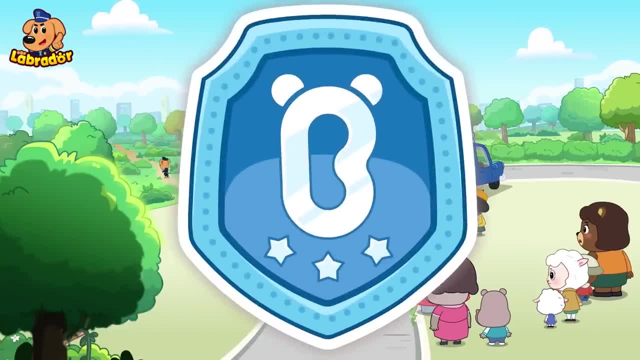 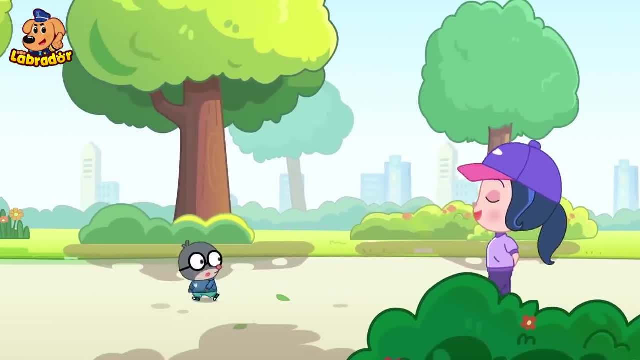 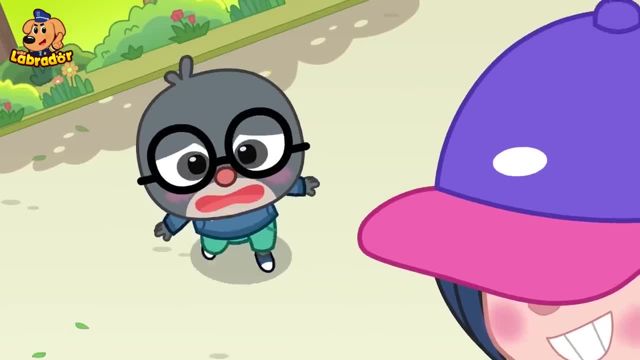 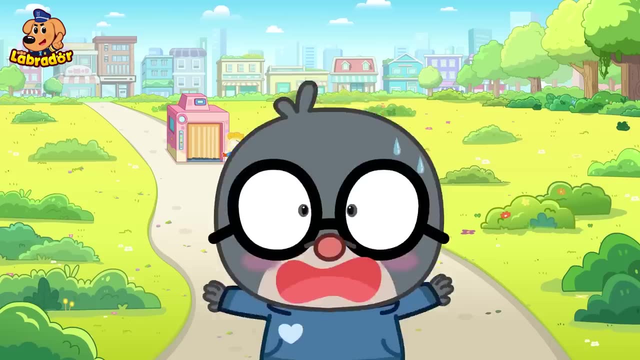 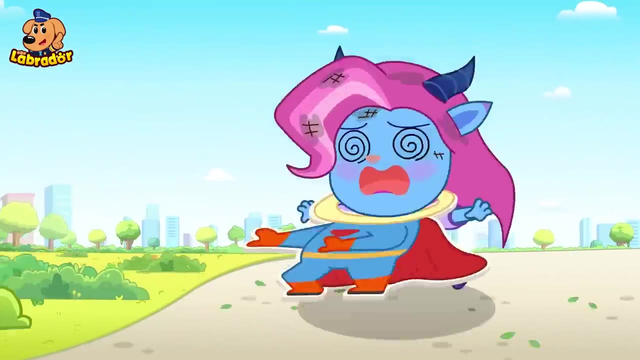 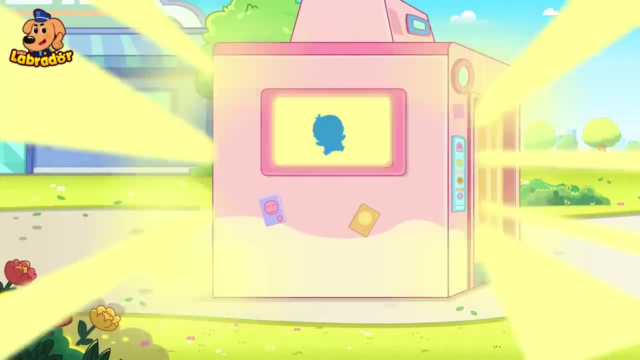 Your mom is not at the hospital, But I saw the ambulance going by. It was a lie. She wasn't hurt at all. You tricked me. Help, You can't run away. Help me, help me, Help, Help. Ha Found them Over there. 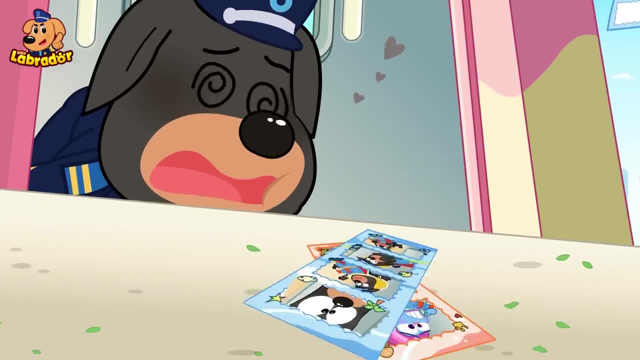 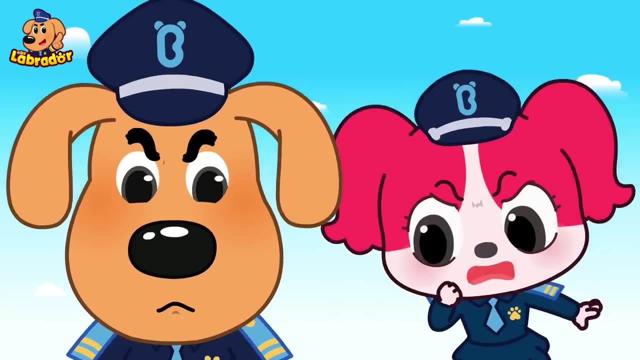 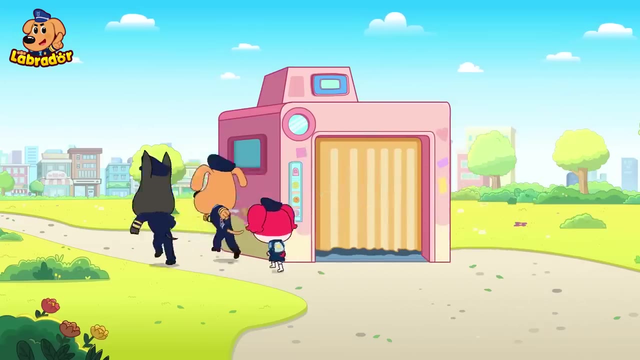 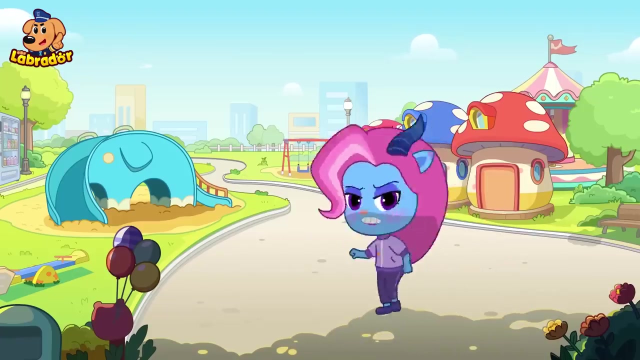 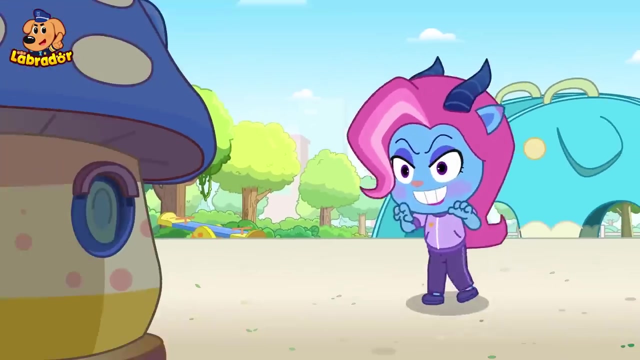 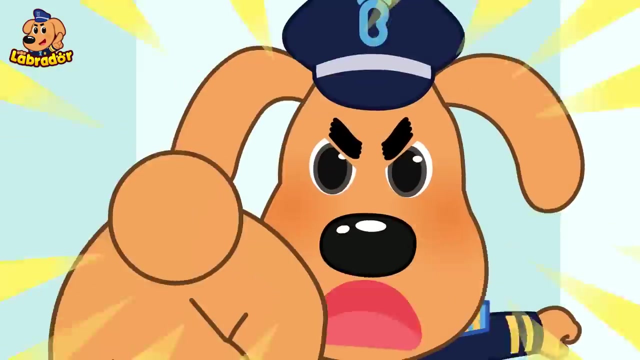 Dobby, It's Antel. She's chasing Little More What. She's causing troubles again. According to the photo, they went that way. Let's go Stop. Where is he hiding? Found you Help? Stop The police. 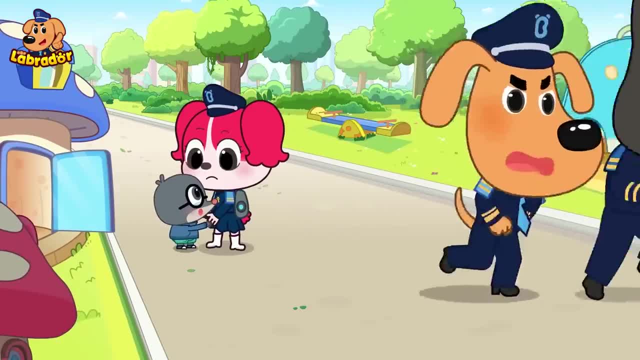 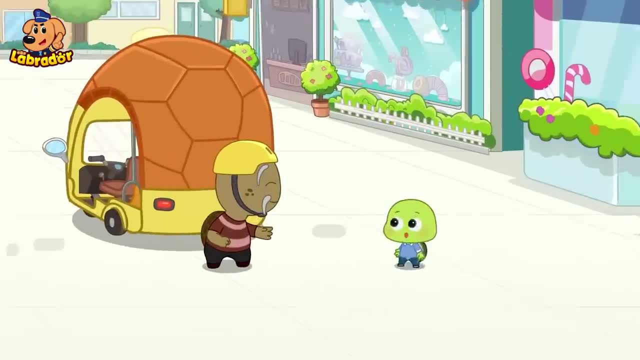 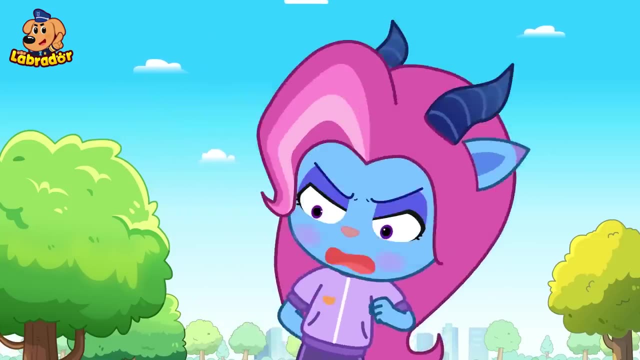 Little More. It's okay now, Don't be afraid, Stop right there. What do I do? What do I do, Grandpa? I'm going to buy some candy. Okay, Be careful. Aha, I have an idea. Let me find a picture of Little Turtle. Yes, That's it. 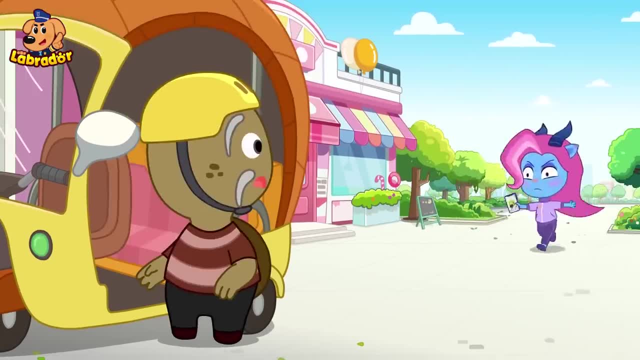 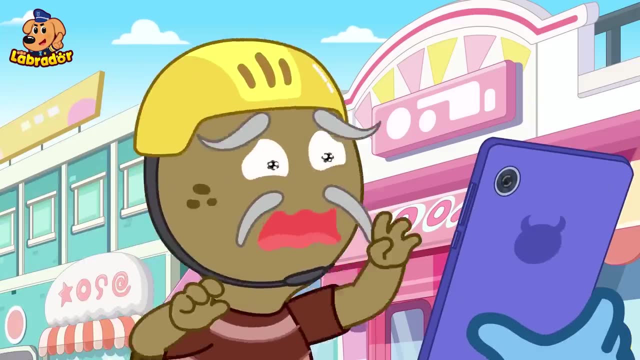 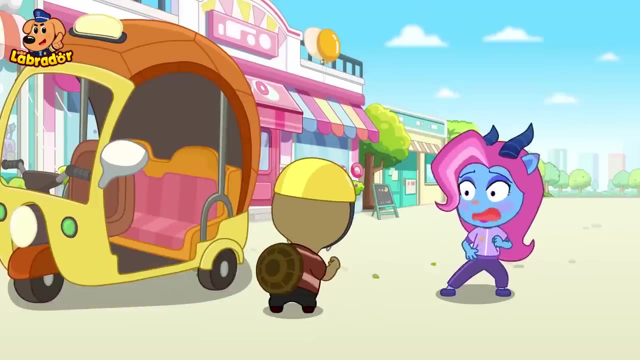 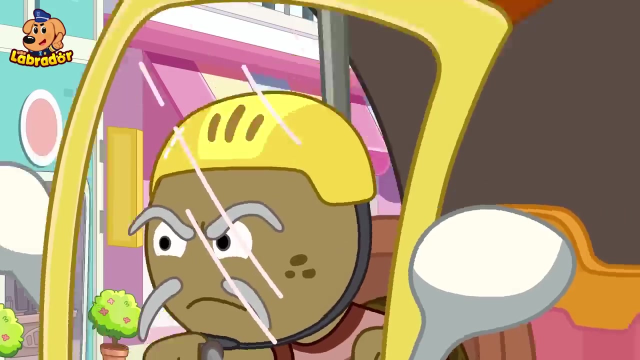 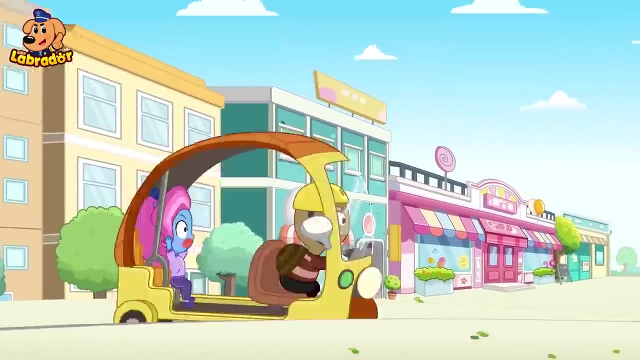 Mr Turtle, Your grandson got hurt and was taken to the hospital. What He was fine just now. Look at this, My grandson Hurry, I'll show you the way. Okay, Checked another one. What are you doing, Mr Turtle? You're going the wrong way. 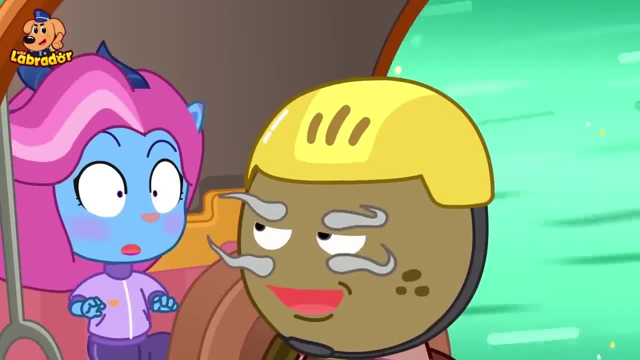 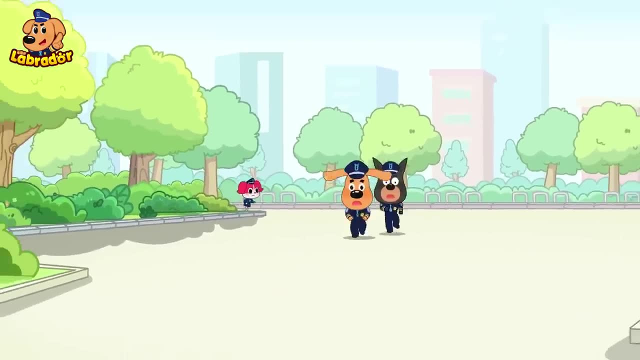 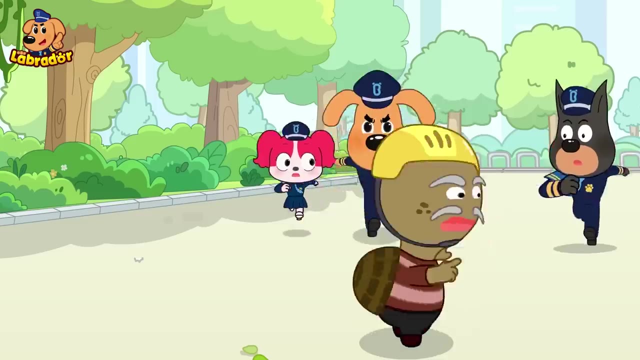 No, I'm not. I'm taking you to the police station. What? Oh, that's great. The police are right there. Sheriff Labrador, There's a scammer here. She's the one we're looking for. Oh, no. 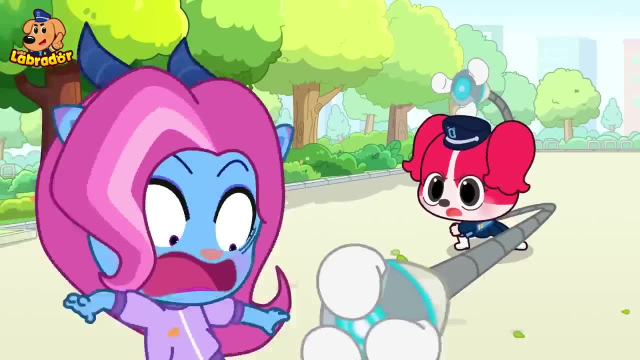 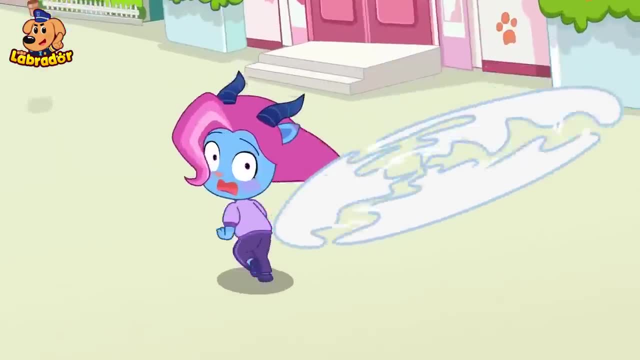 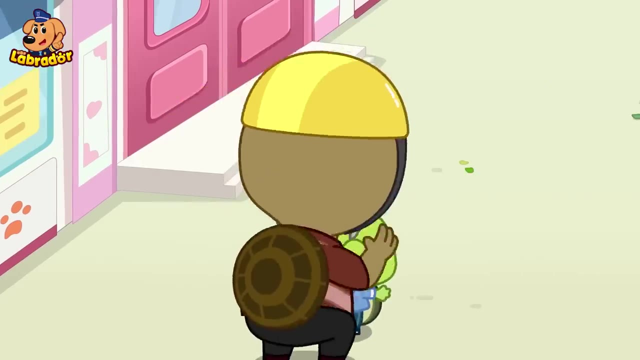 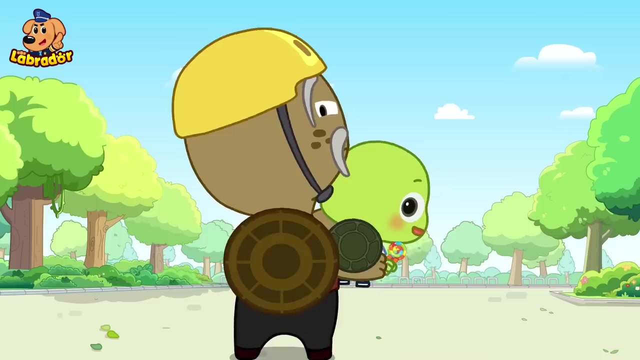 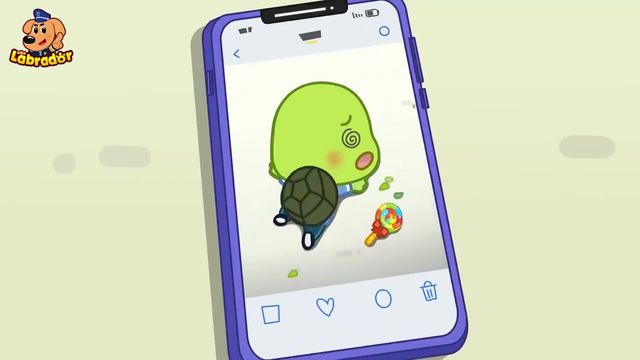 Stop, Stop, Watch my… Nunchucks. Ah, Grandpa, My sweetie, I knew that it was not the picture of my grandson. Look, This is our family's traditional shell pattern. Antel, You're coming with us. 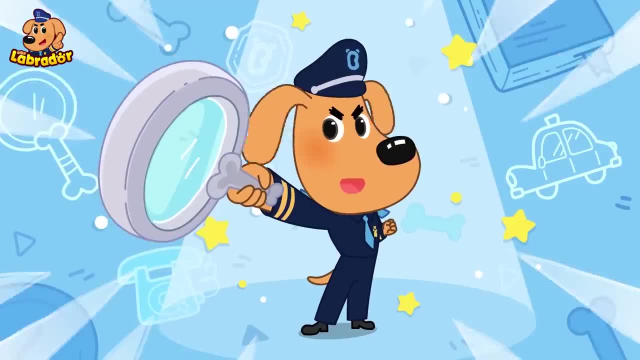 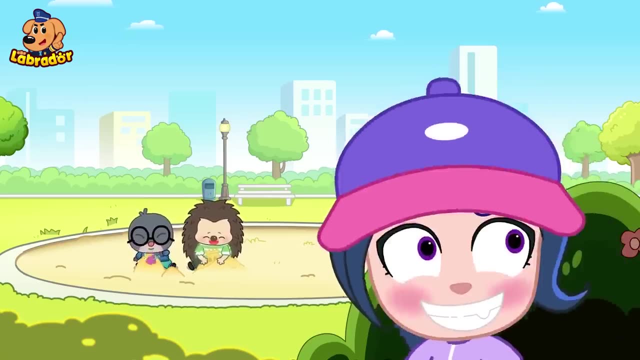 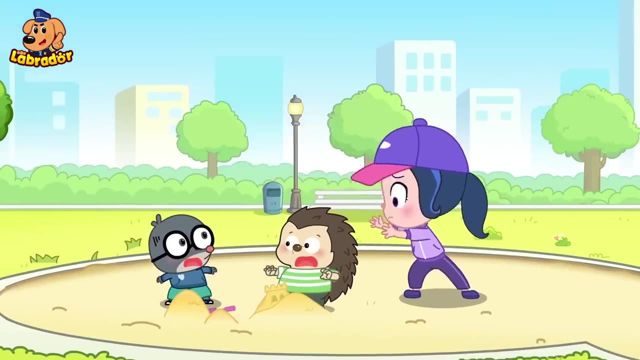 Sheriff Labrador's Safety Talk Kids. some bad people might make up fake stories to trick us. They might say your family is hurt and in the hospital, or that they've been in a car accident. Don't believe what they say and never go with them. 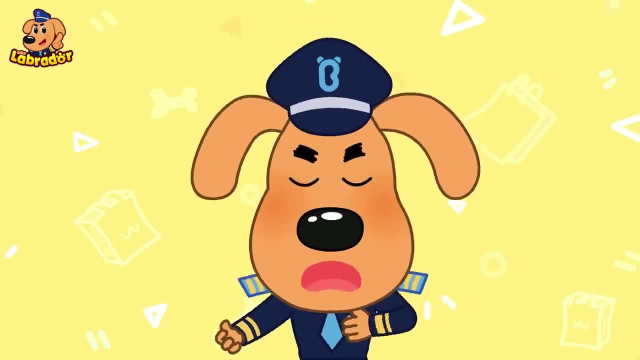 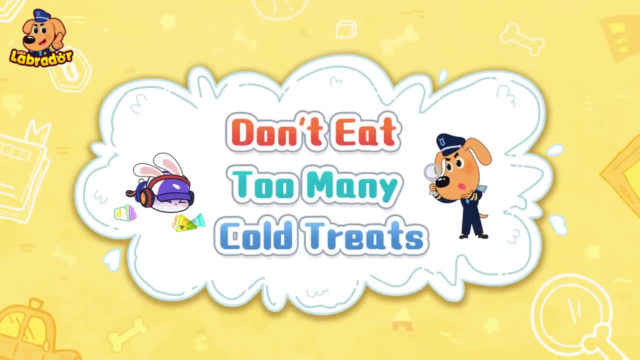 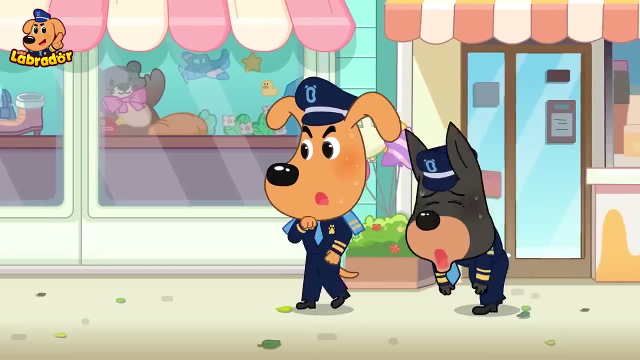 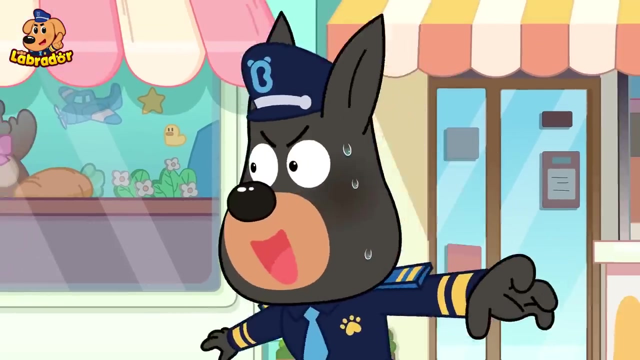 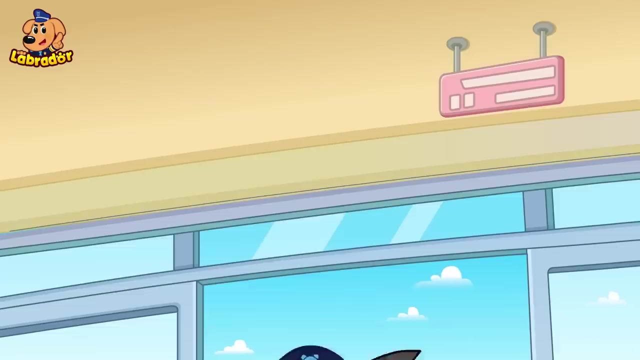 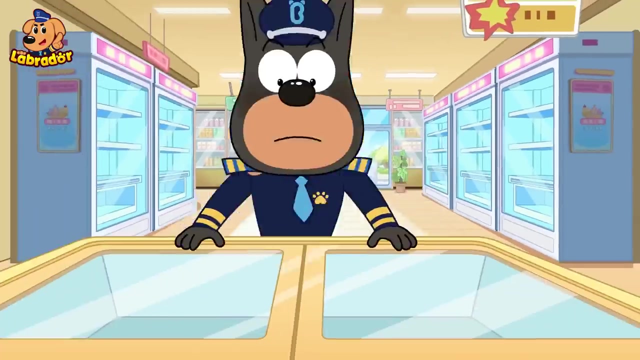 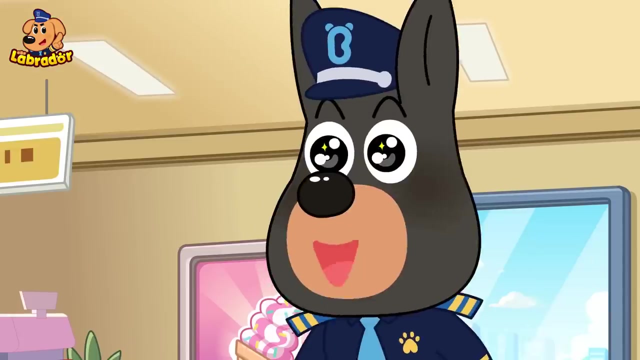 Call your parents or the police right away. Please remember that. What Whoa, Don't eat too many cold treats. It's so hot. Wow, Ice cream. Hey, It's empty. They're all empty. Huh, There's one left. 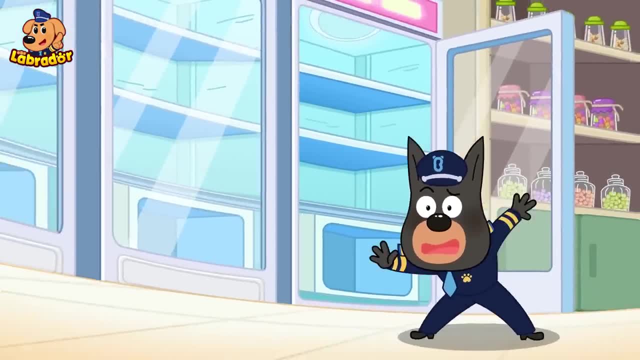 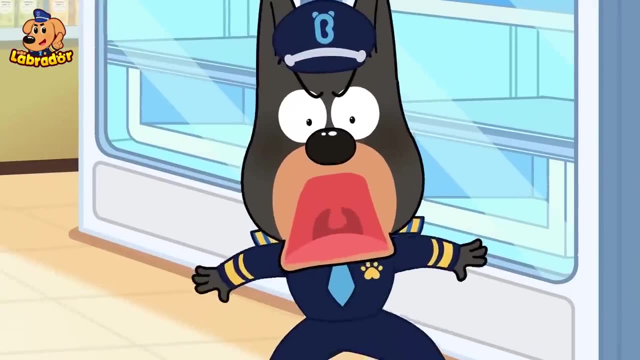 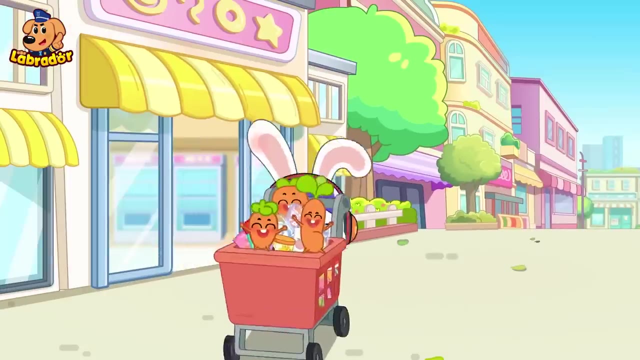 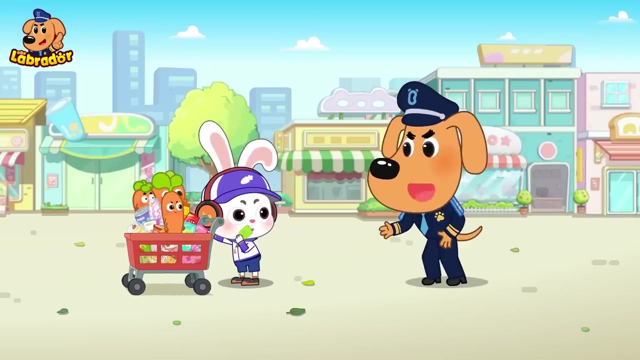 Huh, Buy them all. Buy them all, Sir. All of them, please. What, Oh, I couldn't even buy one. Peepy Rabbit bought all of them. Oh, Fantastic, I'm gonna eat them all. Peepy Rabbit, eating too much ice cream will make your tummy hurt. 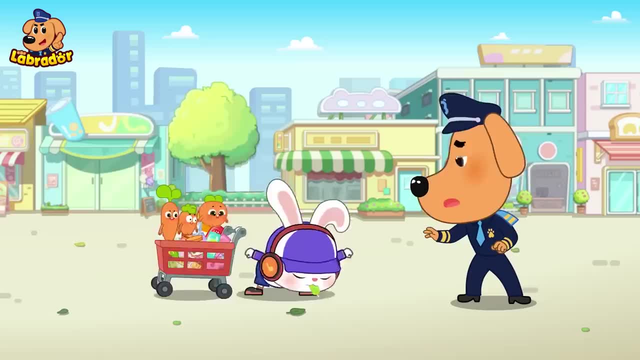 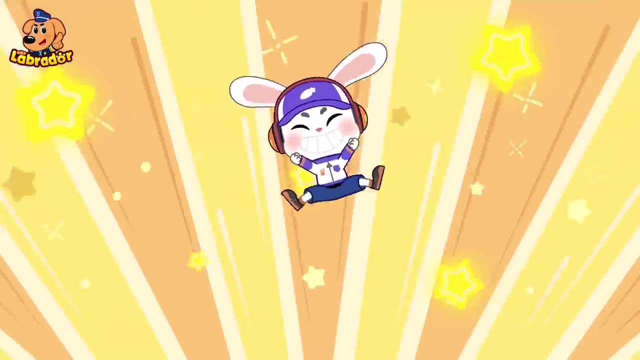 No, it won't. Ah, Bye-bye. Ah, Ah, I'll go and buy more ice-cream, Huh, Why? But you ate too many. It's okay, I'll have another one. Ah, It's perfect. 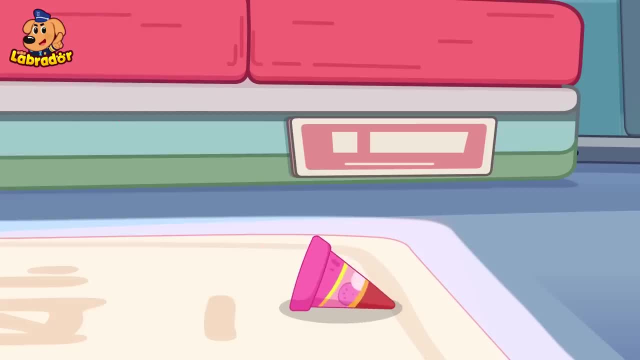 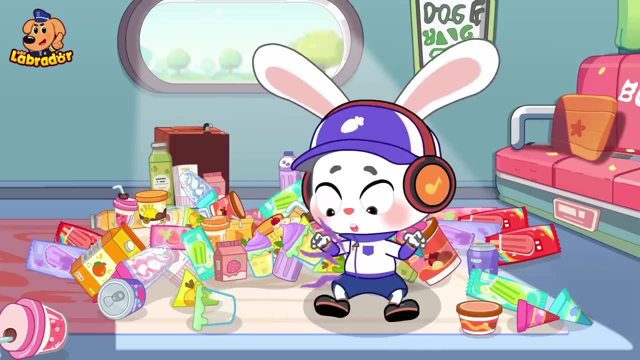 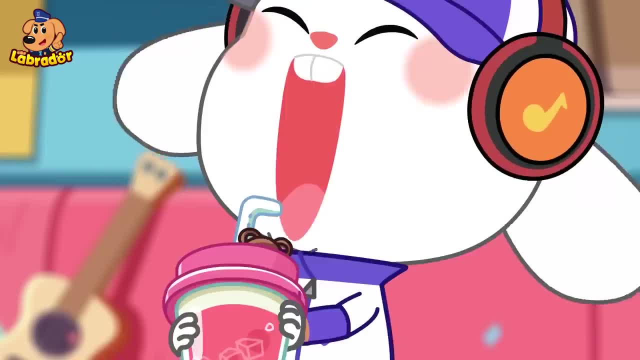 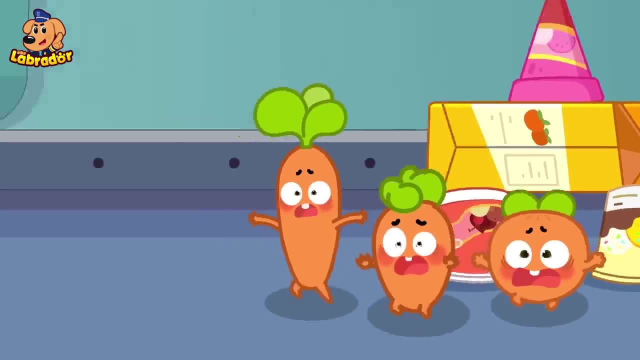 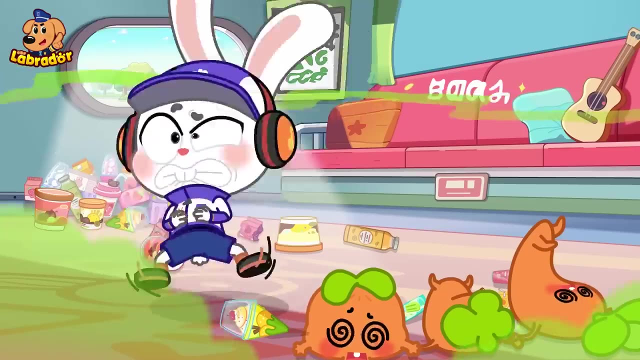 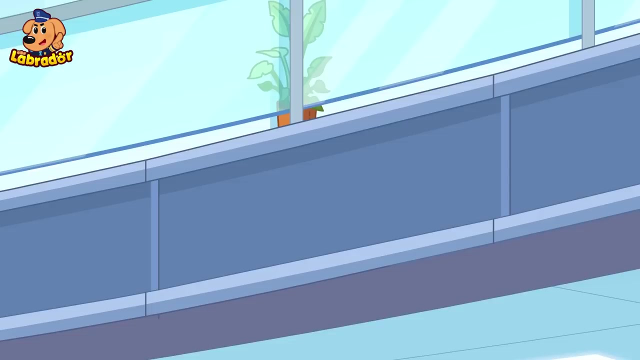 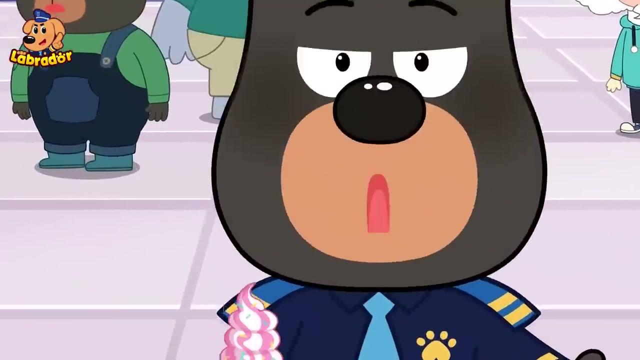 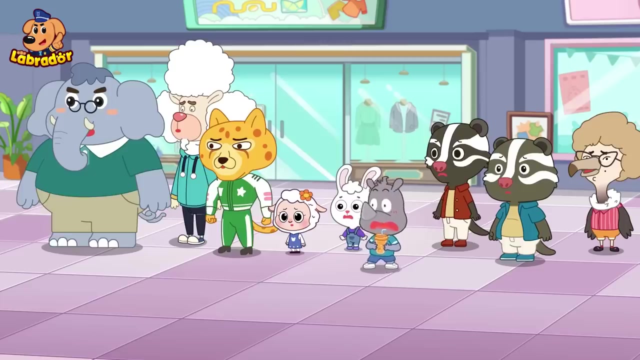 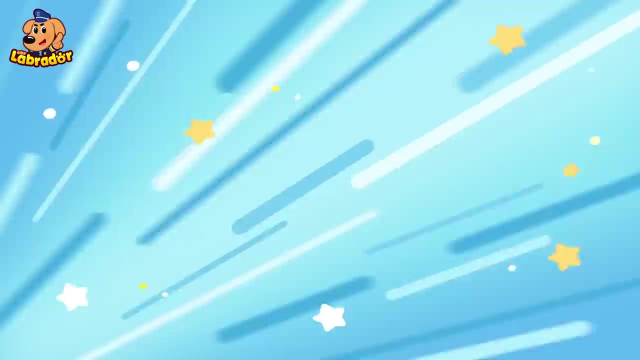 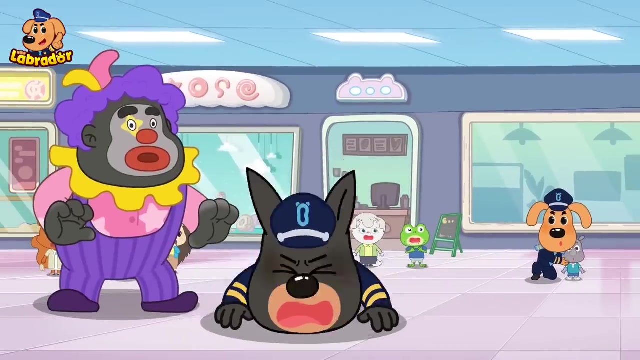 Yay, Yay, Yay Yay. My tummy hurts. I need to go to the bathroom. Wow, Finally got one. Move aside, Move aside, Watch out, Hey Peepy Rabbit, You shouldn't run around like that. 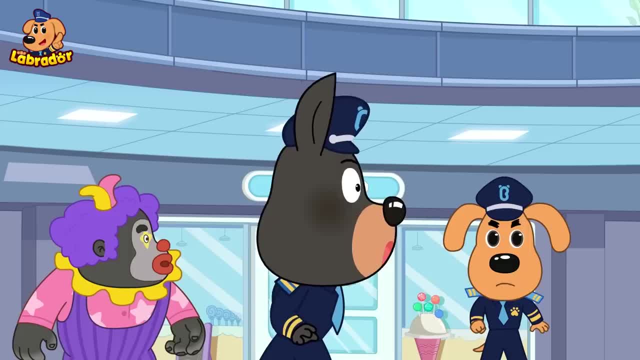 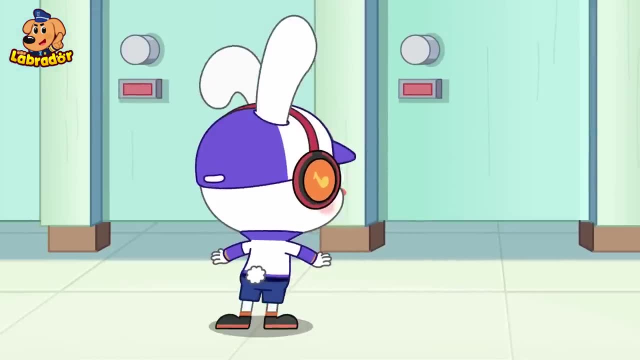 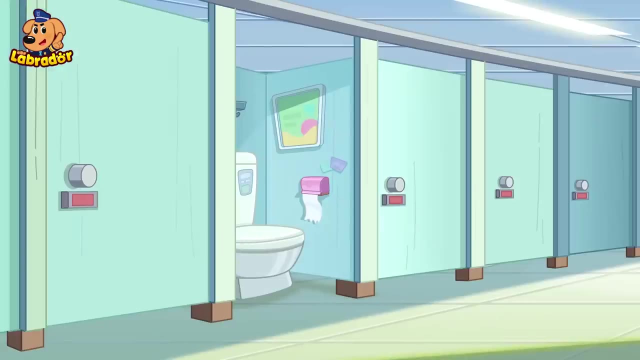 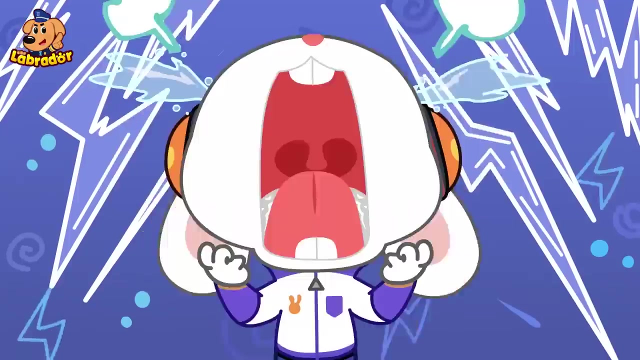 Dobby. I think he's looking for a bathroom because he has a tummy ache Bathroom. Where is the bathroom Occupied? There's another one over there Under repair. There it is. Come on, Seriously, I gotta find another bathroom now. 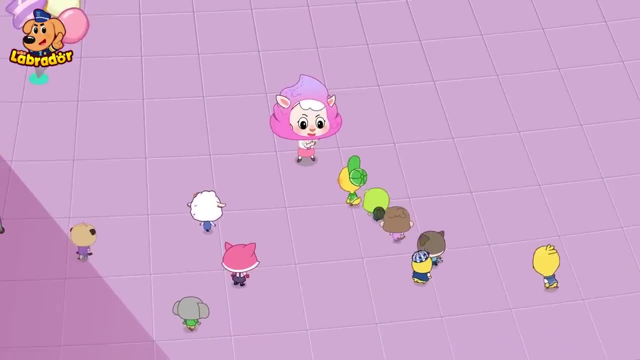 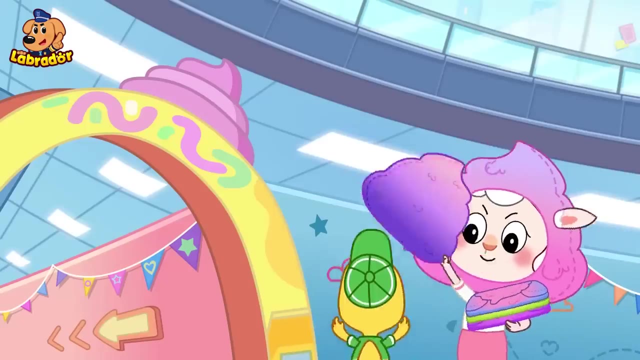 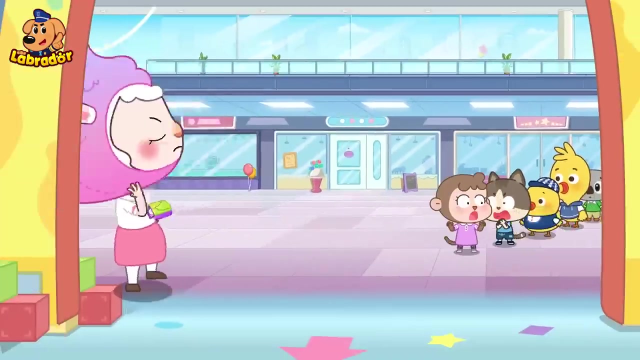 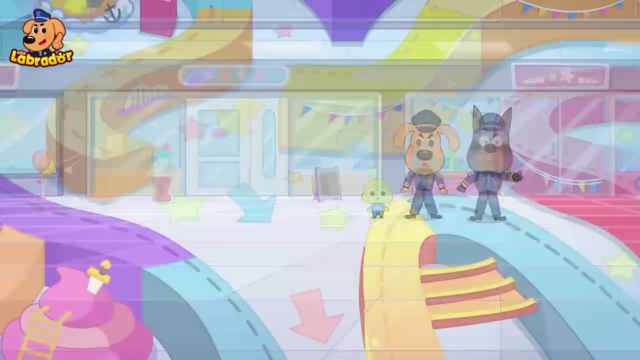 Oh, Welcome to Poochie Poochie Maze adventure. It's a bathroom. I wanna try. Here you go. Next, Here you go, Watch out. Wasn't he looking for a bathroom? Why did he enter the maze? 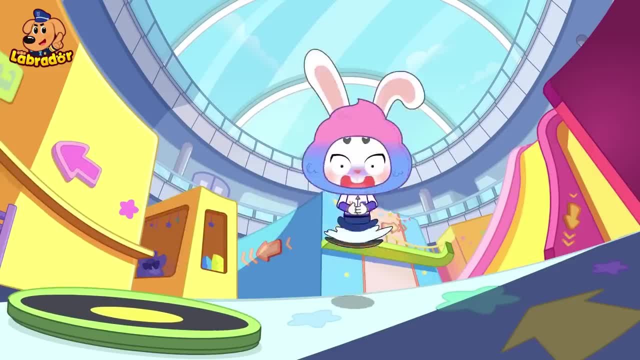 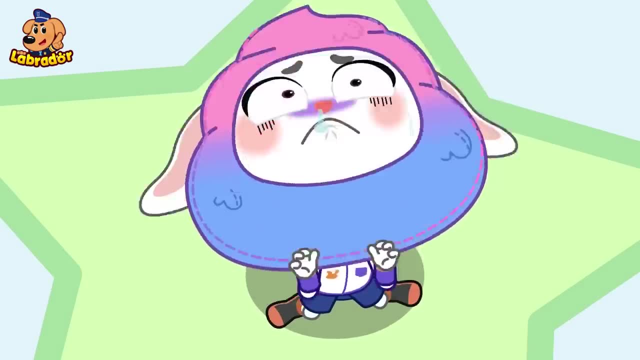 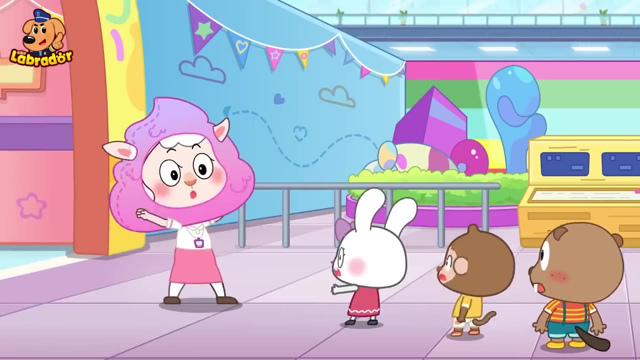 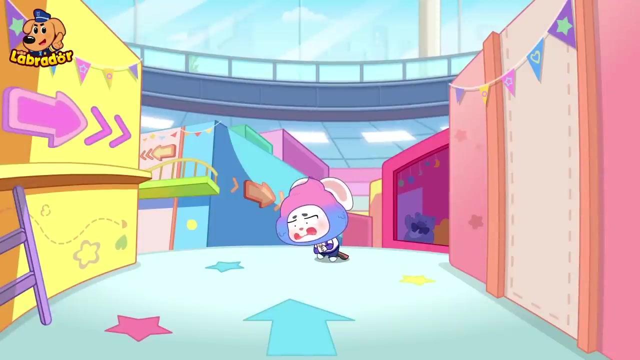 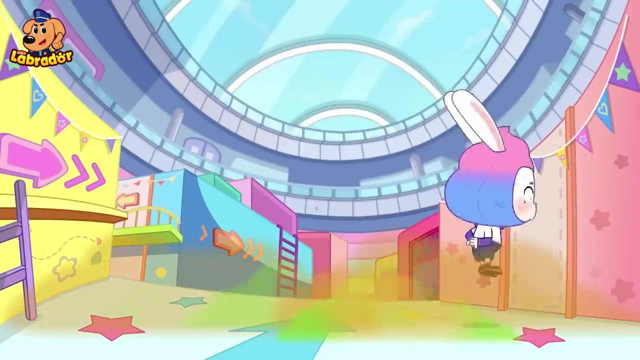 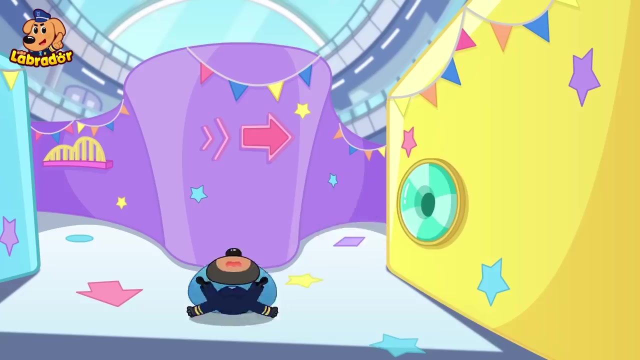 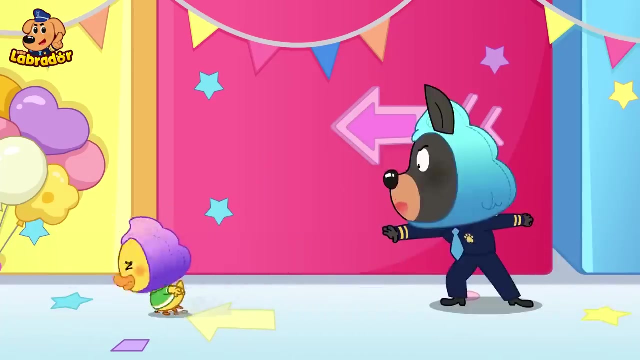 Why am I back here again? Why is going to the bathroom this hard? Help me. Oh no, Peepy Rabbit needs help. Sorry, There's an emergency. My tummy hurts so much. Help, Where's Peepy Rabbit? What's going on? 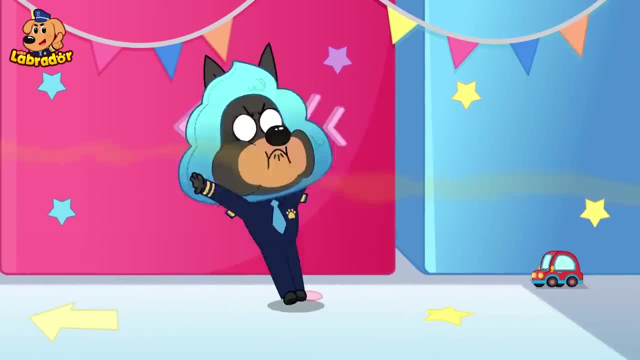 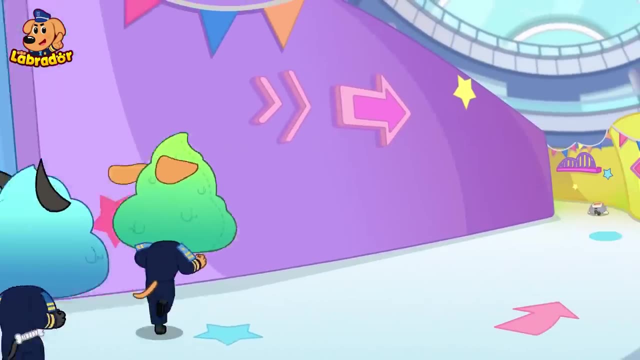 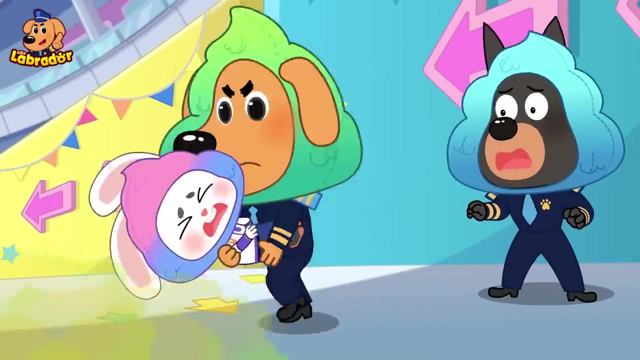 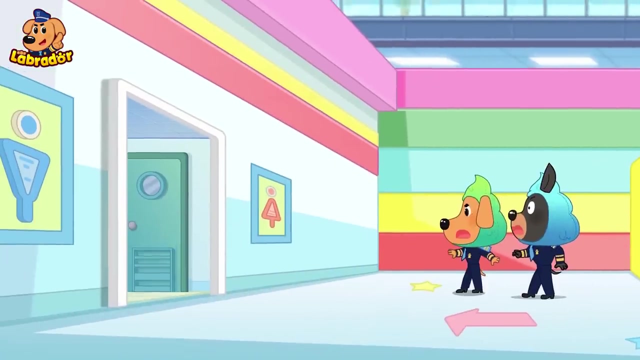 Someone farted. It stinks. It must be Peepy Rabbit Over there. My tummy hurts so much. Peepy Rabbit, Come on, We'll get you out of here. Hurry Phew. I feel much better. 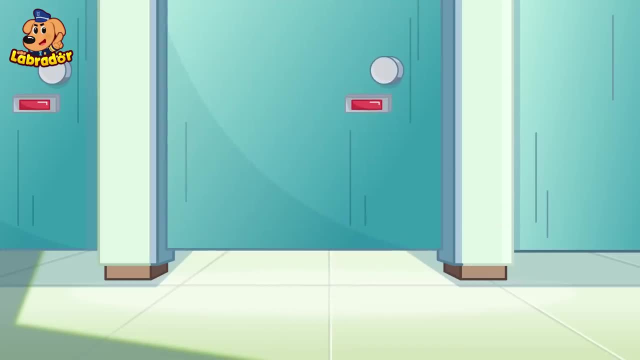 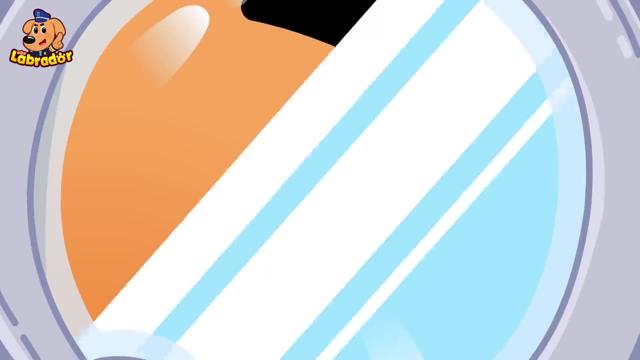 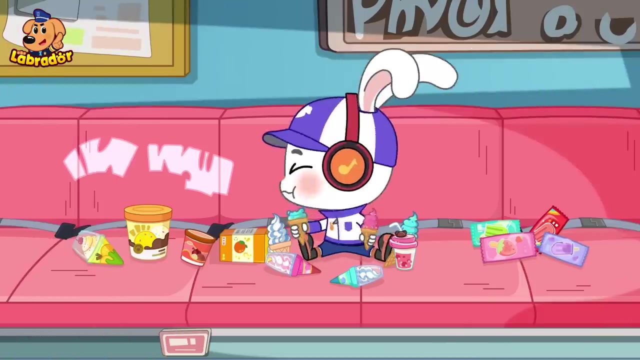 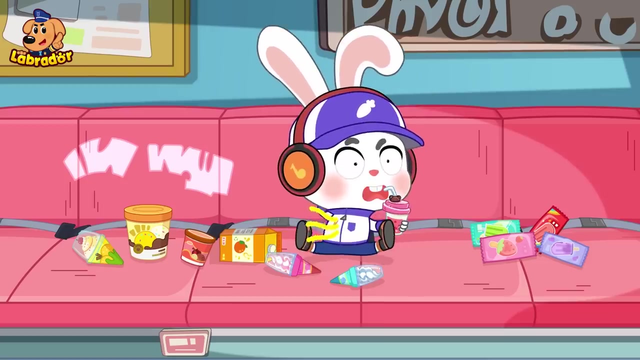 Oh no, I have to go again. I'll never eat so much ice cream again. Sheriff Labrador's Safety Talk: Kids. cold treats are delicious, but you shouldn't eat too much at once. If you eat too much of them, you might get a tummy ache or diarrhea. 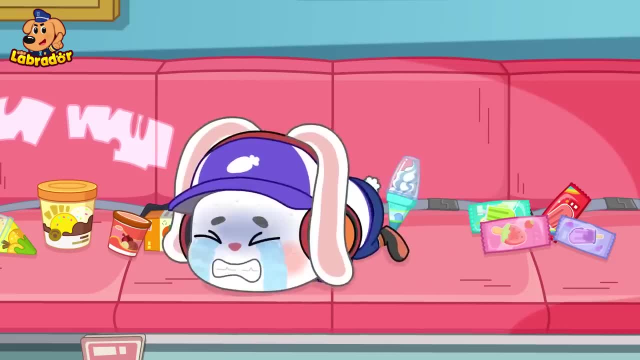 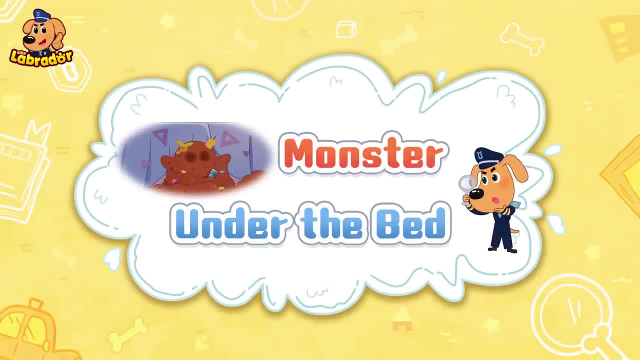 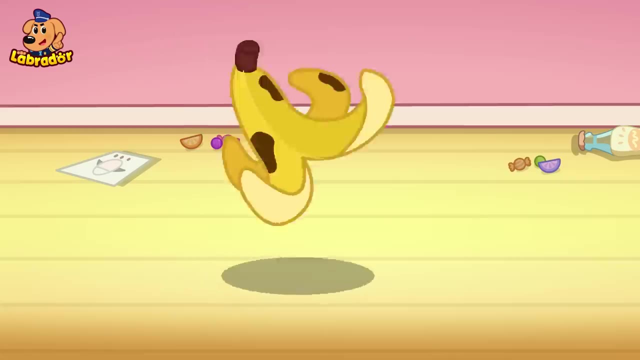 You might even vomit or get a fever, which is not good for your health. Remember, don't eat too many cold treats. Woof Monster Under the Bed, Kick, Kick, Kick, Oh, Oh. Oh, You littered again. 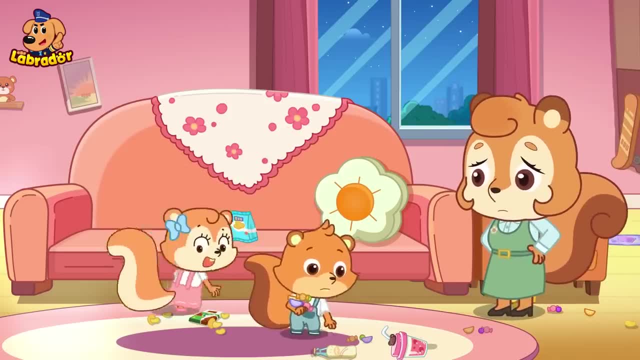 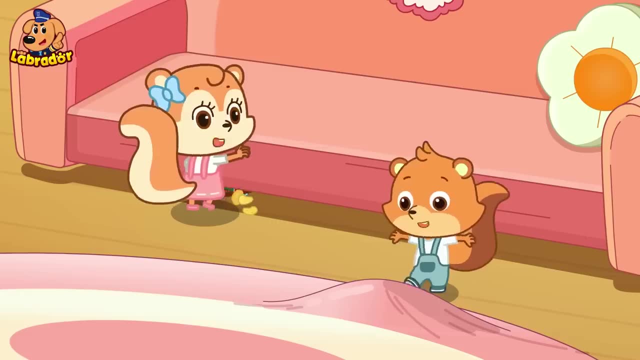 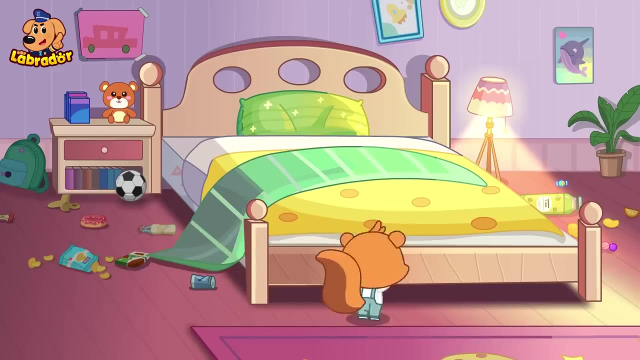 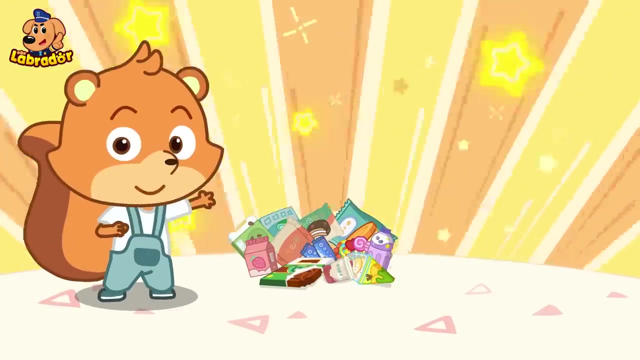 Clean it up, okay, Okay, Okay, Mommy won't find the trash here, right? Let's hide and eat in here so that Mommy can't see us. Whoa, I've hidden so many things to eat, Whoa. 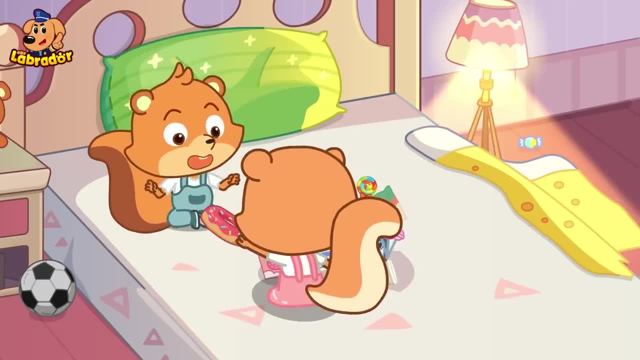 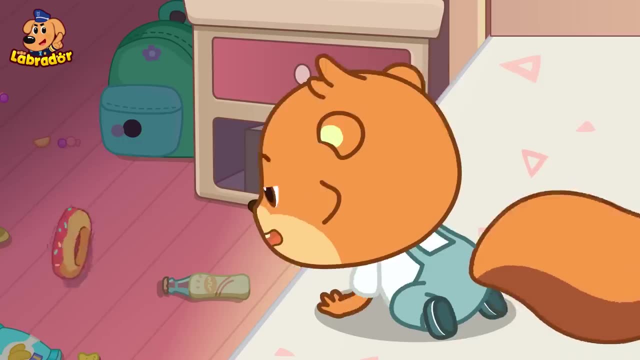 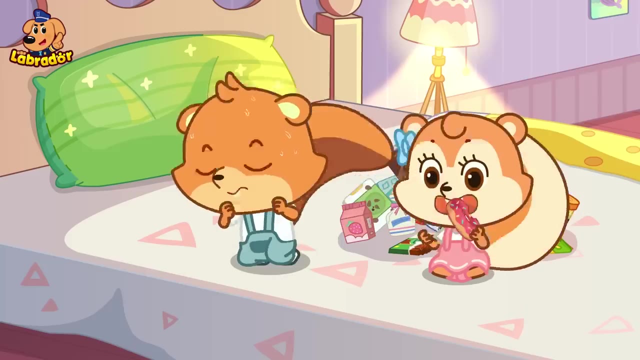 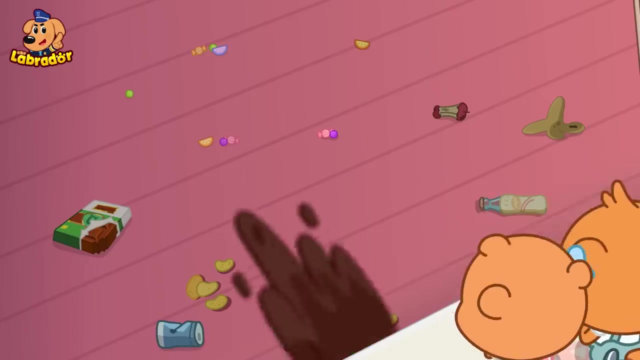 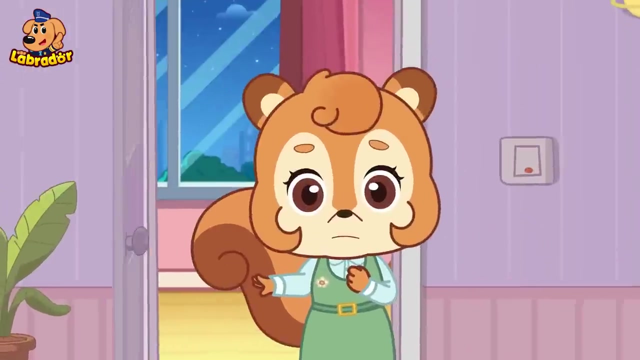 Whoa, I'm going to eat the doughnuts, I'm going to eat the lollipop. Ha ha ha, The doughnut. The doughnut moved by itself. Ah, Ah, Oh. What's going on? Oh, Oh. 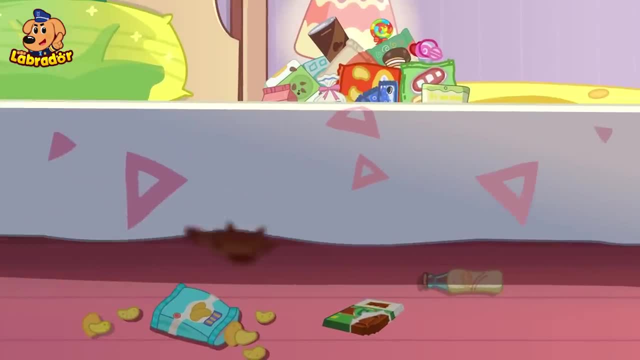 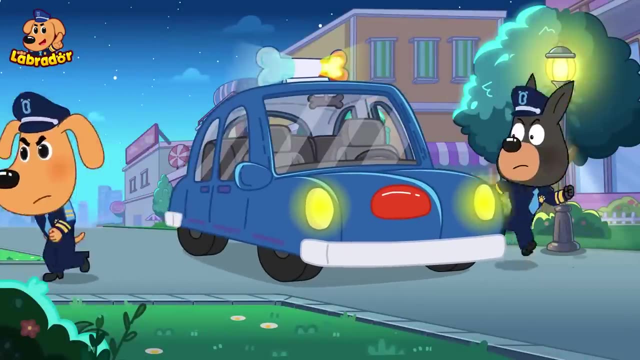 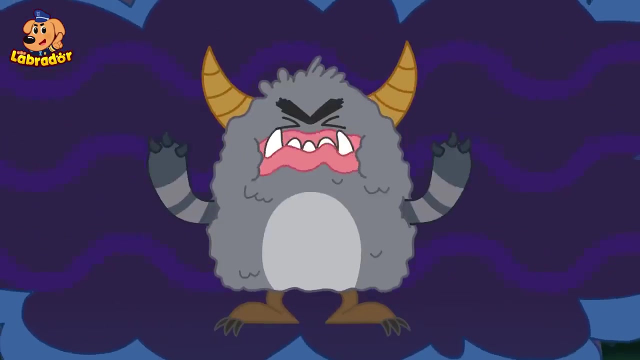 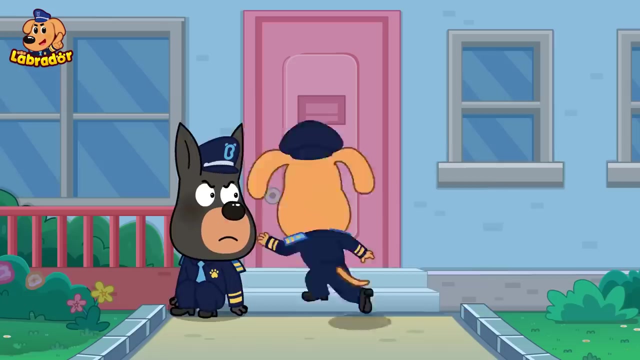 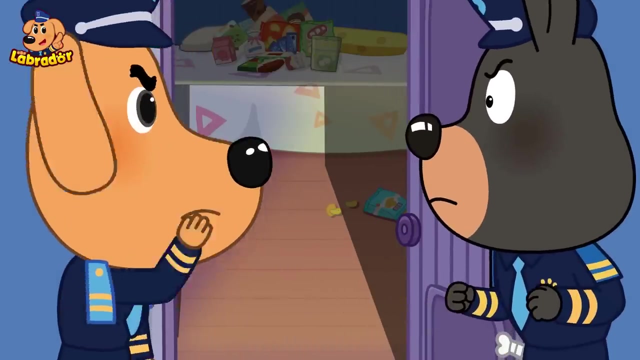 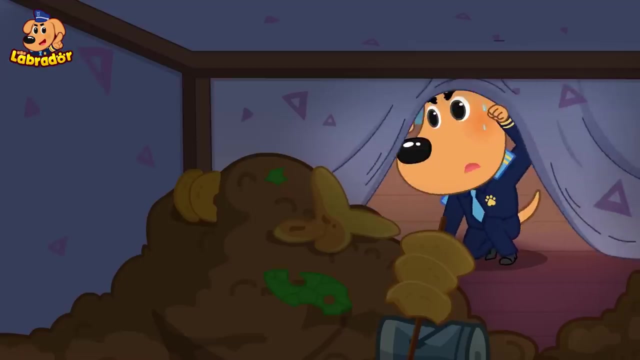 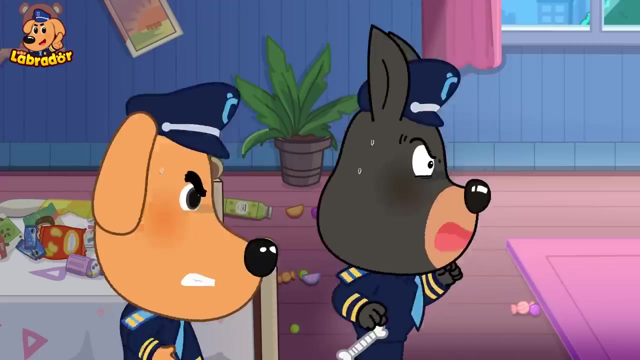 Mommy, There's a monster under the bed. Whoa Monster, Sheriff Labrador, There's a monster under the bed in our house. It ate all our snacks. What? Let's go inside and check There it is. Stop right there. 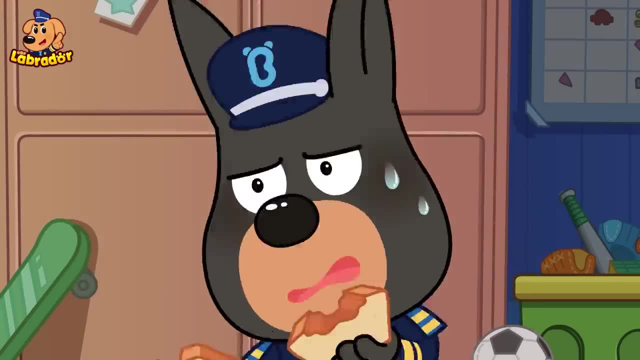 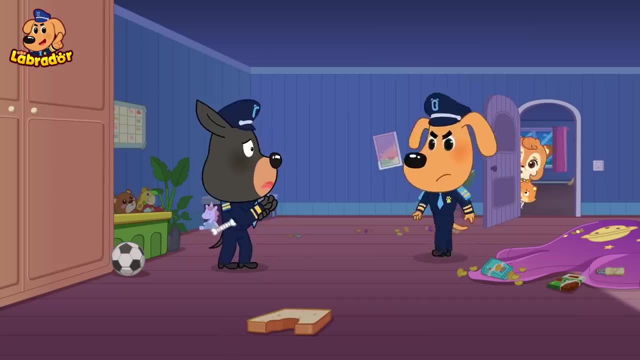 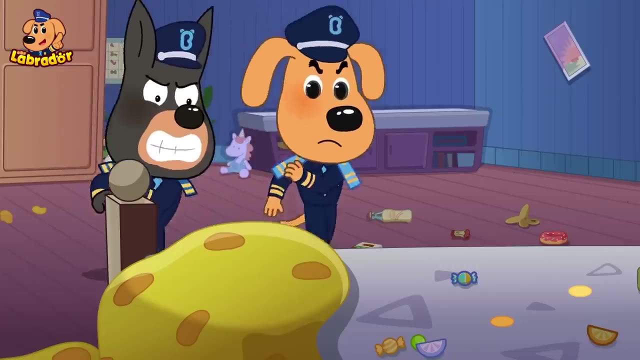 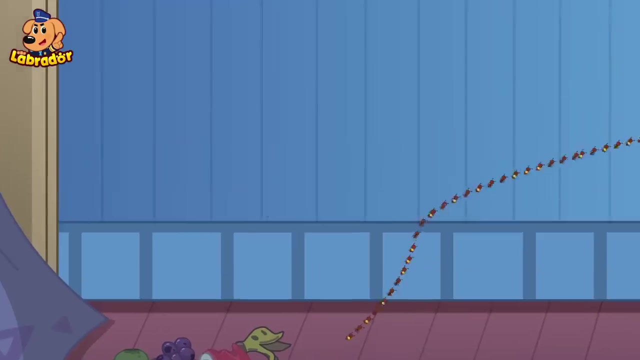 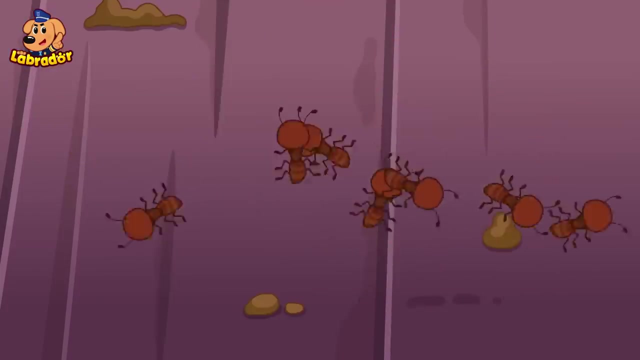 Stop right there. Ouch, It bit me. Ants Move the bed aside. There's so much trash under the bed And so many ants too, So the monster was just a bunch of ants moving stuff, I see. 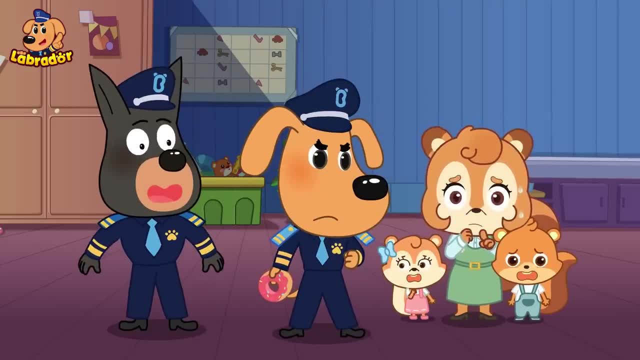 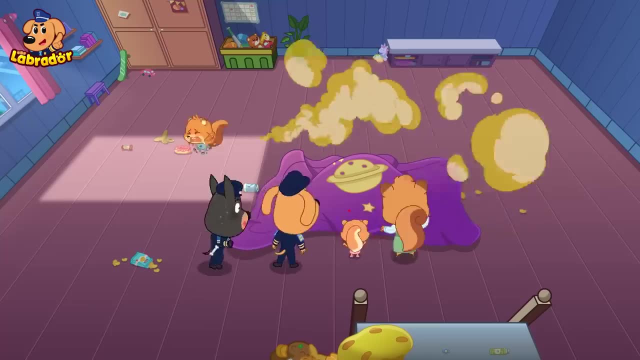 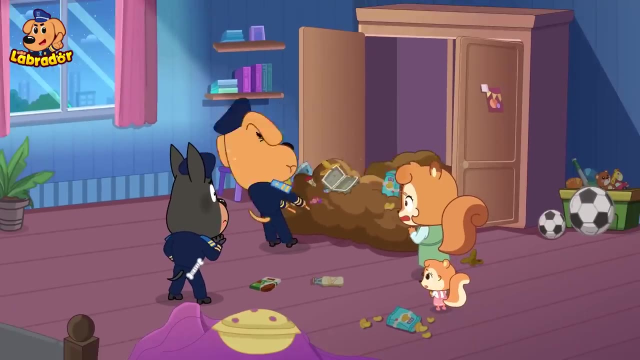 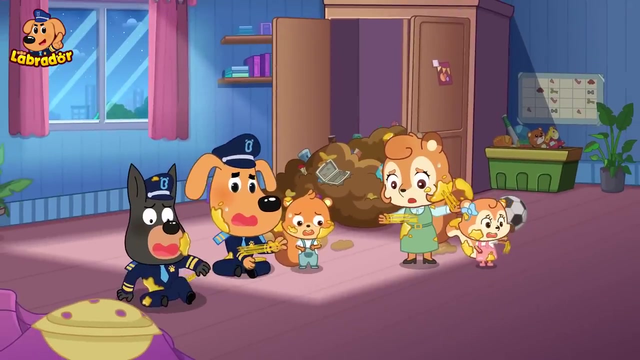 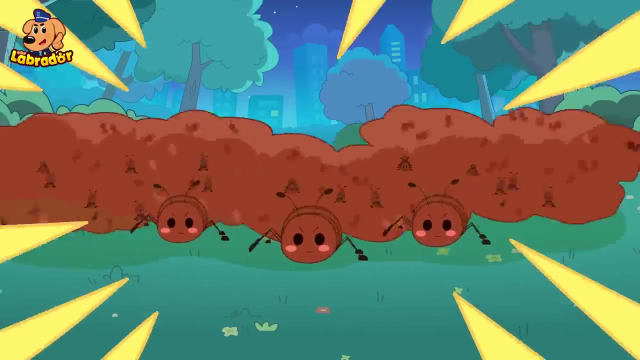 We need to clean up the trash right now. So, itchy Ant, You've hidden food in the closet too. Oh my, It's so sticky. Oh no, The ant army is coming. Let's get out of here. 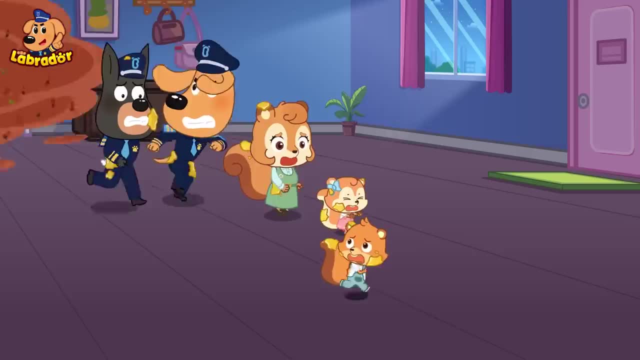 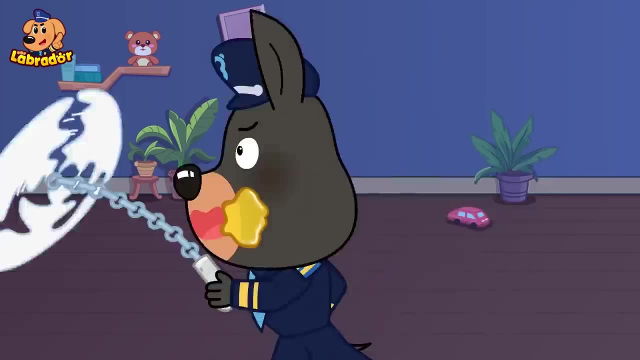 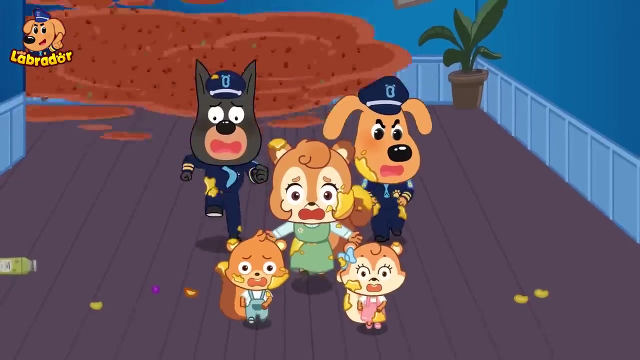 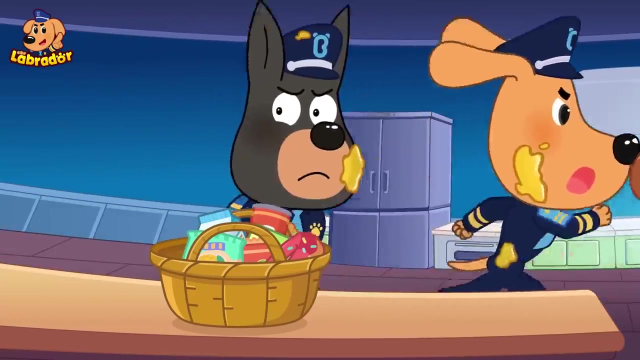 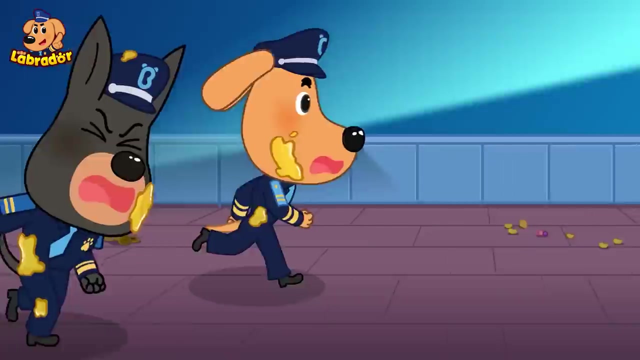 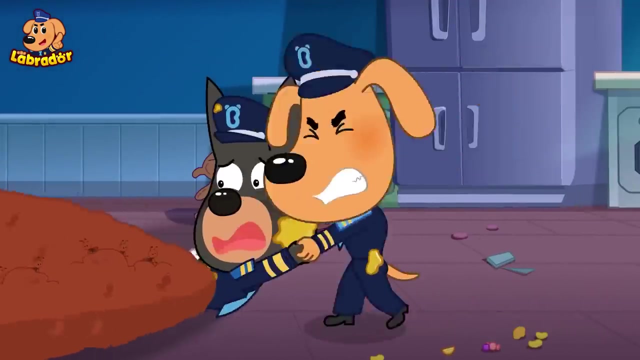 They're breaking the door. Run, Run, Help, Hey, Help. Why are they chasing us? They're attracted to the smell of food on us. I'll stop them. Ah, Wow, Jobe, Ah, Ah, Let's go. 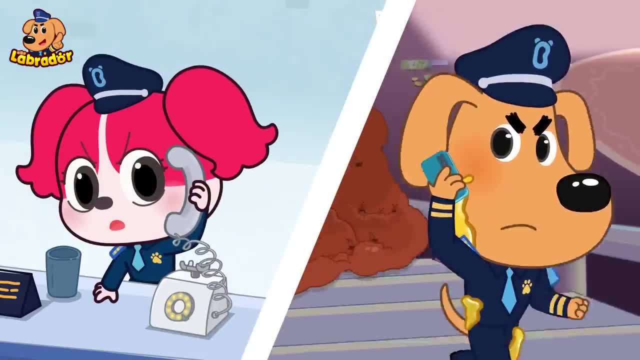 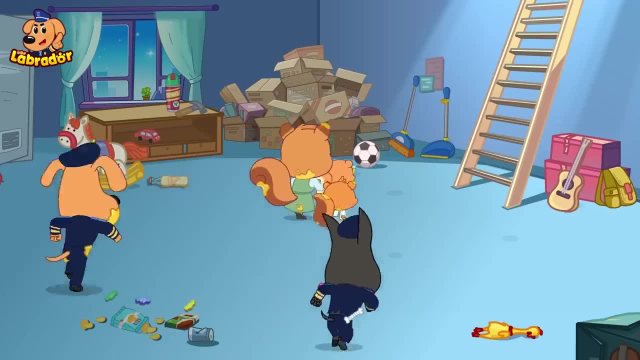 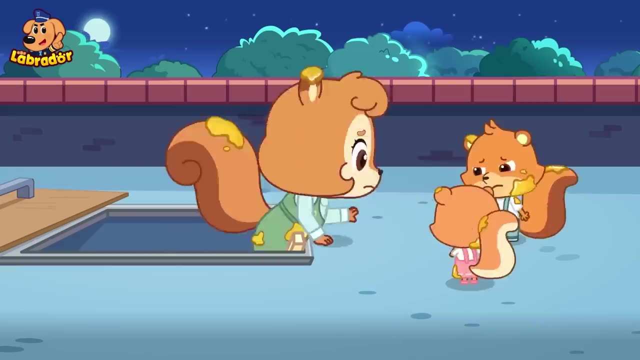 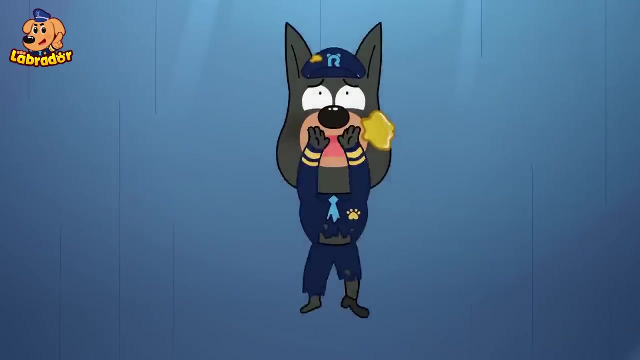 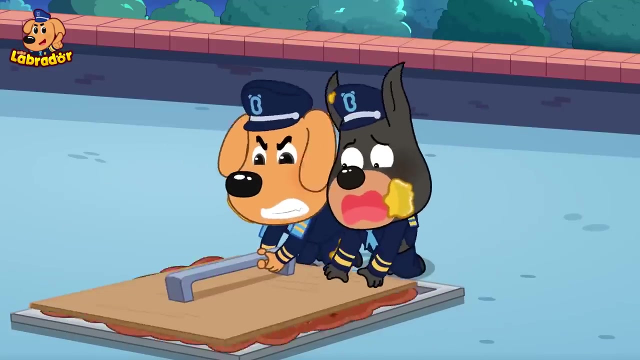 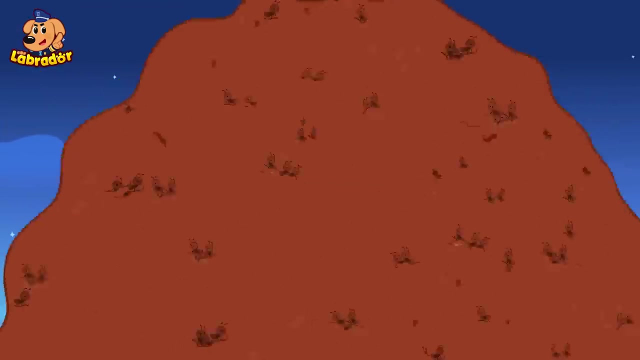 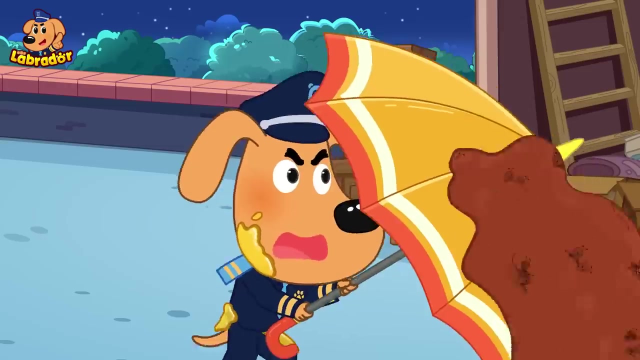 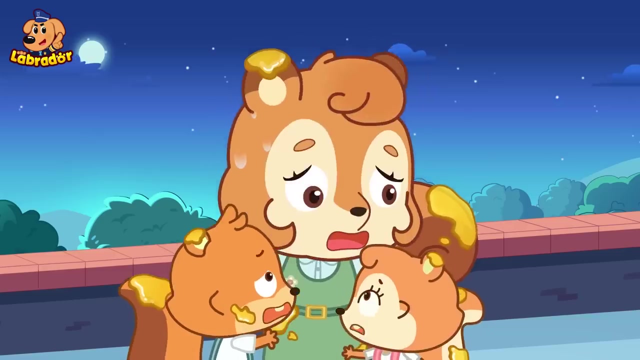 Papillon. ants are attacking the squirrel family's house. We need backup. Got it? Climb up now. Oh no, Close it. What's that? Run that way, Mommy. are those ants going to eat us? Papillon is here. 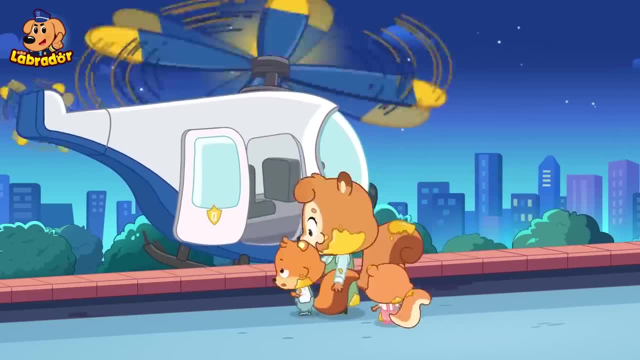 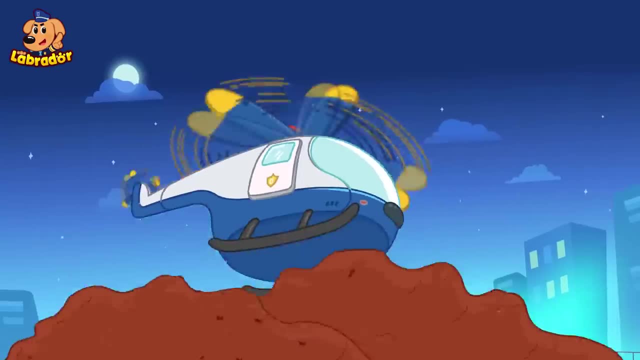 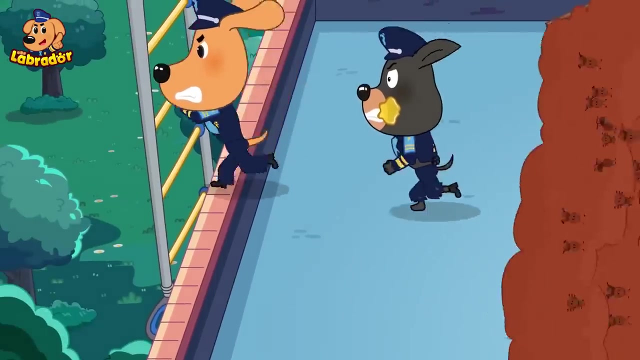 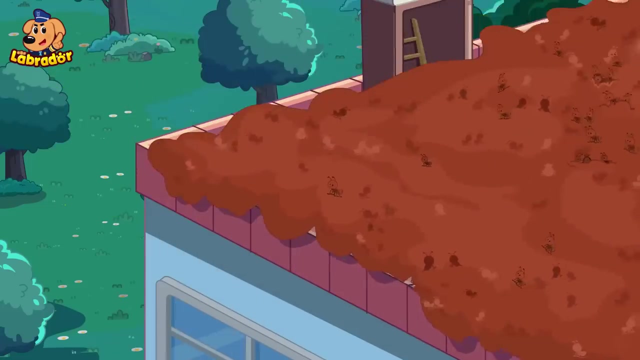 Great, It's Papillon. Come on up everyone. The ants are coming. Hurry up Sheriff Labrador Dobby. Hurry Dobby, let's go Get off me. That was so scary. I'm sorry. We'll never litter again. 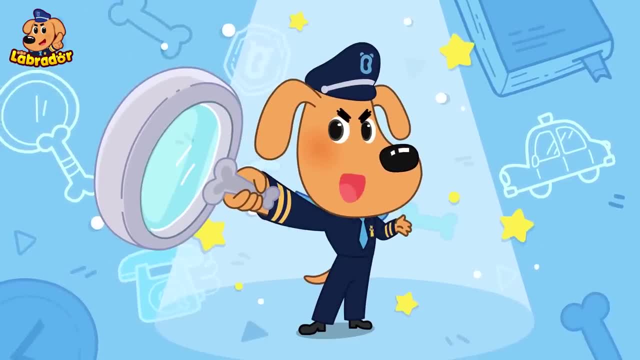 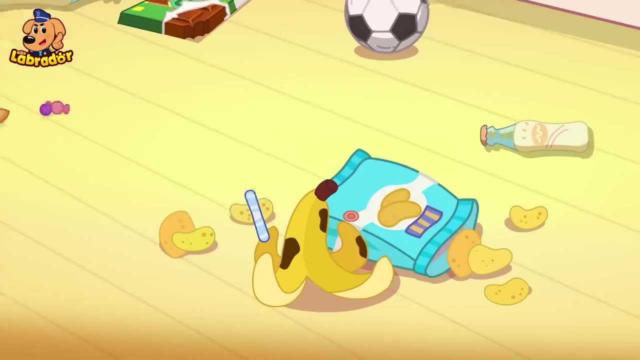 Sheriff Labrador's Safety Talk. Kids never carelessly throw things like food wrappers or fruit peels on the ground. This kind of trash can attract bugs, They can harm the plant, They can harm the places where we live and even affect our health. 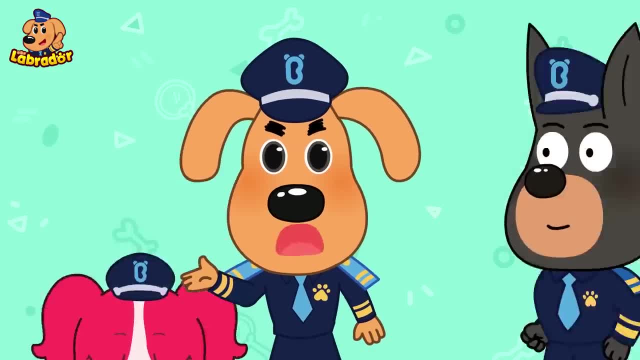 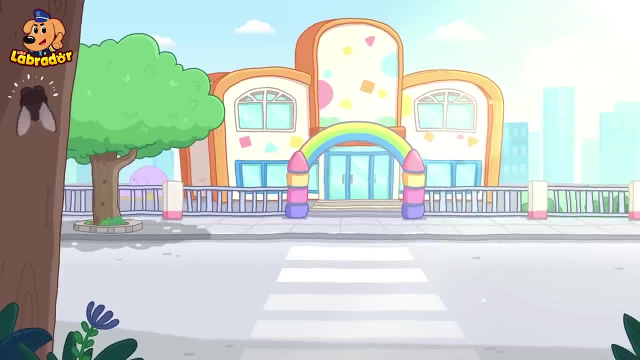 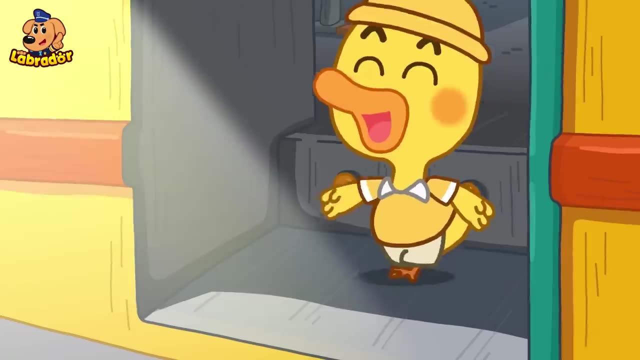 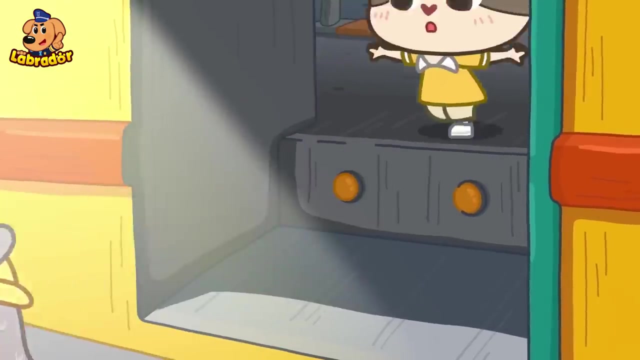 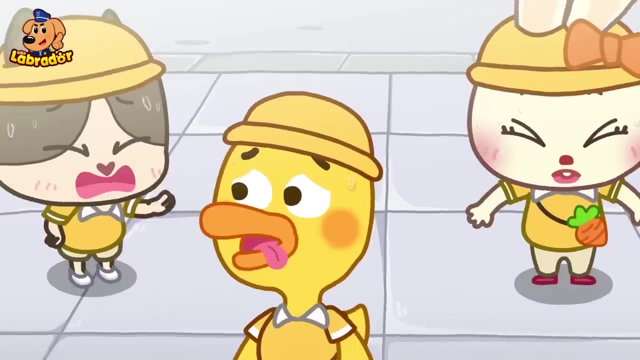 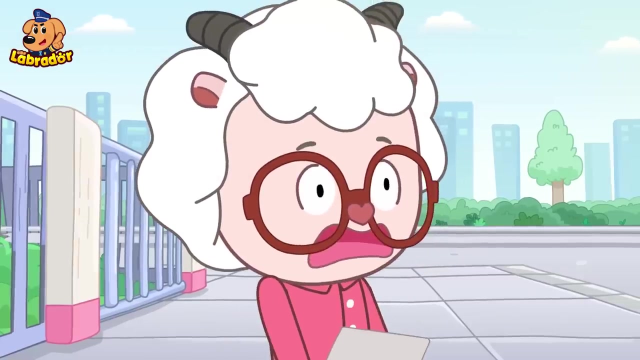 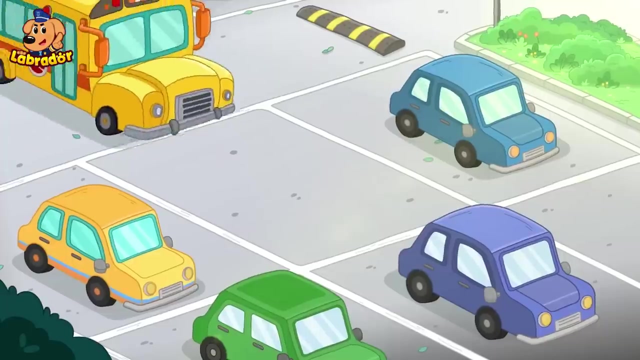 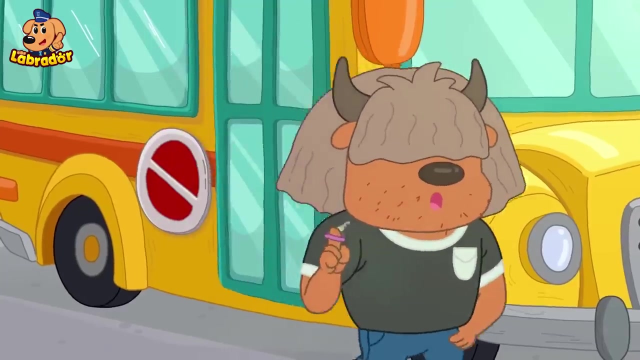 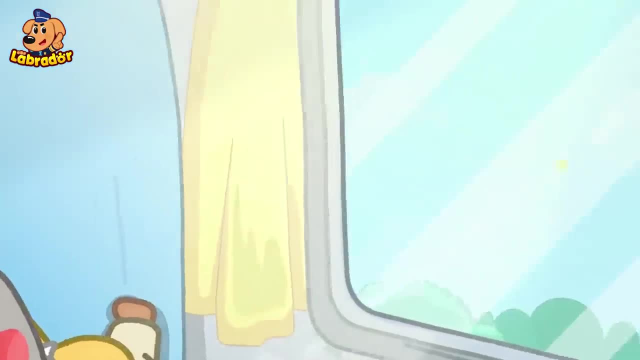 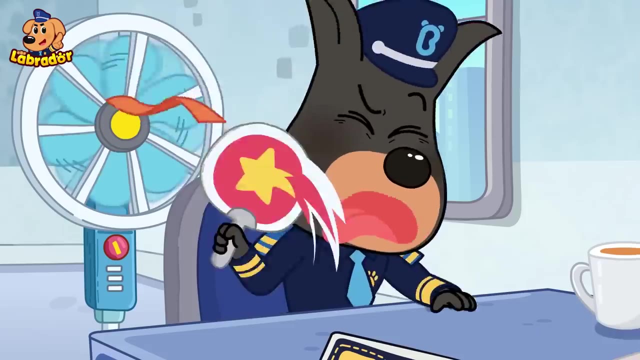 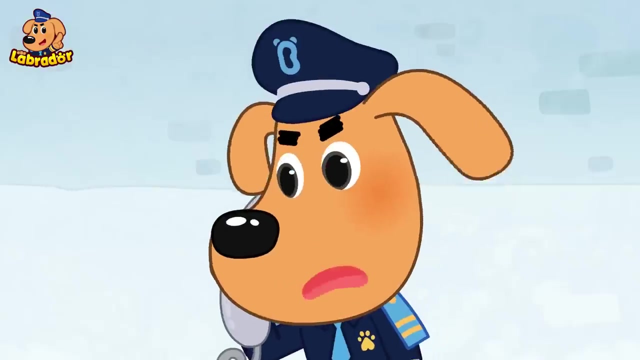 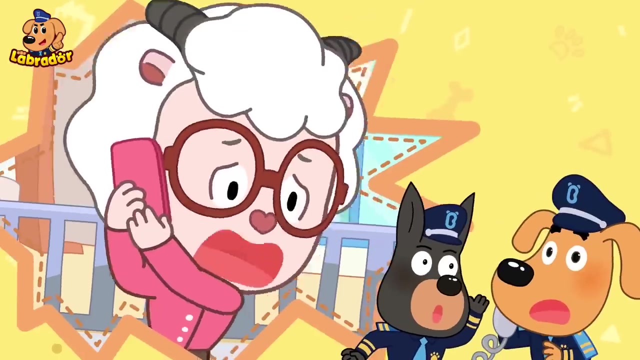 Ugh, it's so hot. Dobie, you'll feel cooler if you just relax. Woof, Hi, I'm Sheriff Labrador. Sheriff Labrador, this is Ms Sheep at the preschool. My student, little koala, is missing. Please help. 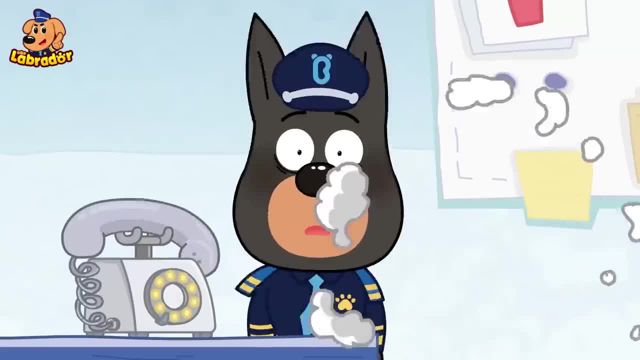 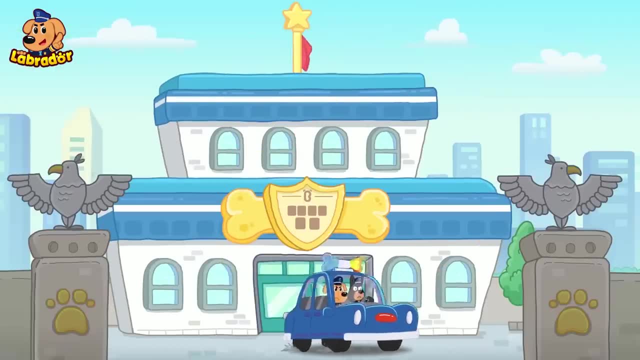 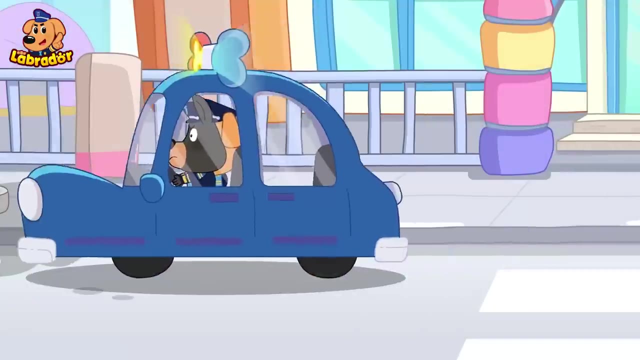 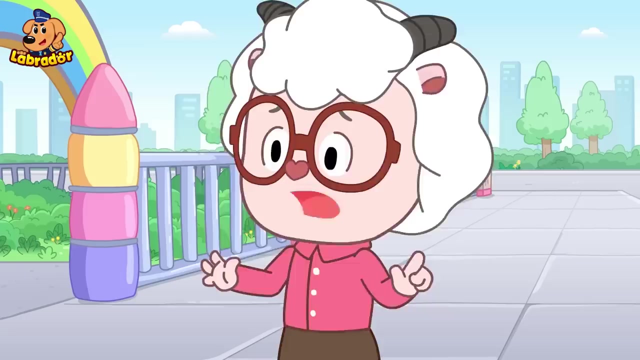 Don't worry, we'll be right there. It's so hot. Ms Sheep, when did you find out that little koala is missing? I found it out when I was counting the children coming off the school bus. What do I do? 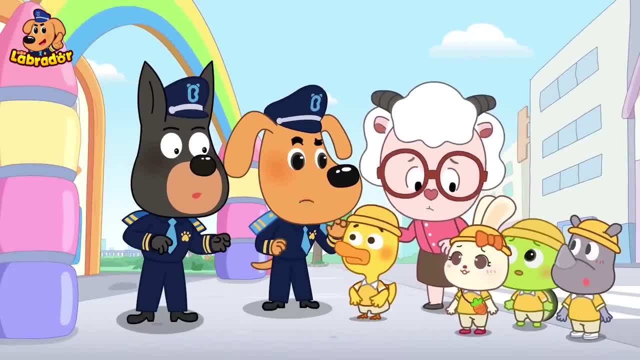 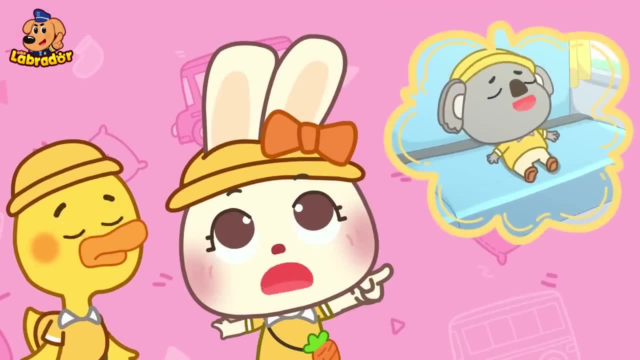 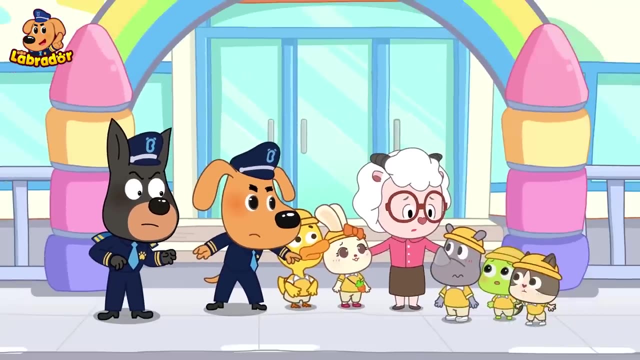 I see Kids. did you see little koala taking the school bus? Yes, I did. Little koala always sleeps on the bus, Then he might still be on the bus. Where's the bus now? It usually goes to the school bus parking lot after dropping off all the children. 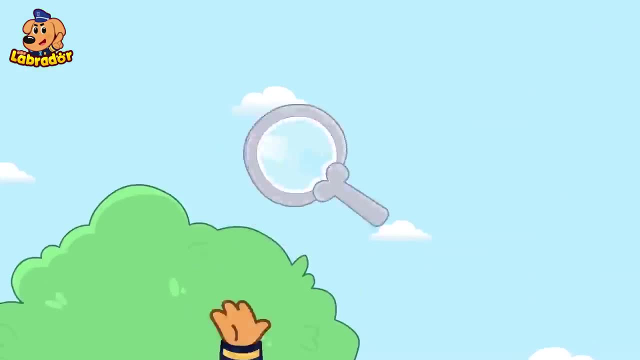 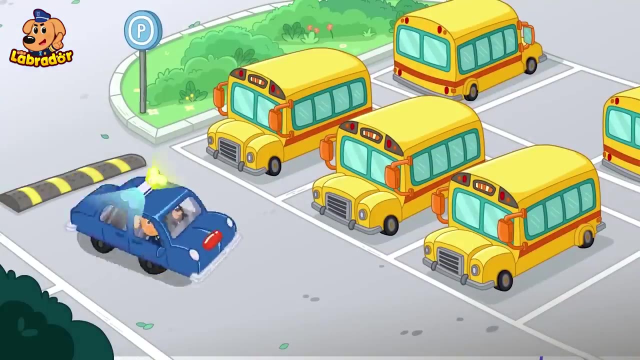 Do you think he's there? We'll go look for him. Don't worry, there's no case that I can't solve. I'm so sorry. It'll be fine, Mr Yacht. Here's the school bus parking lot. 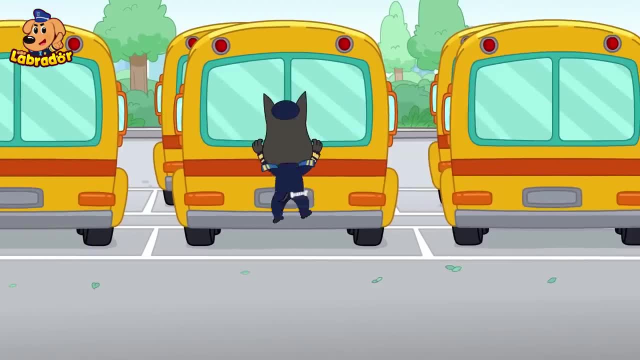 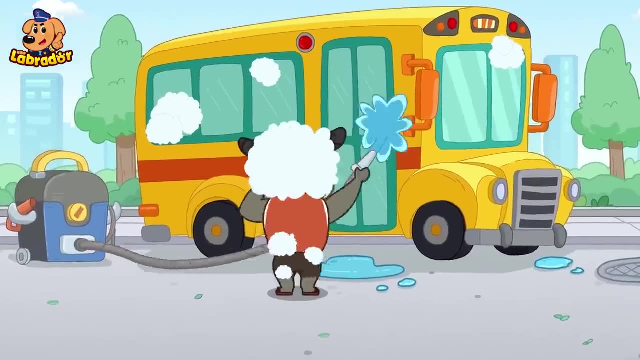 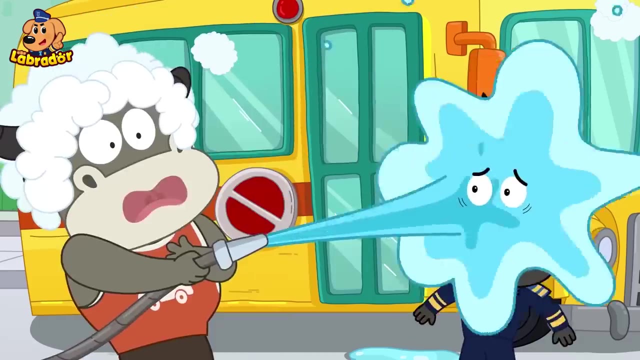 The driver, Mr Yacht, might be around here. Found him, Mr Yacht, Mr Yaaaaaaaaaach, Um, I'm so sorry, I didn't mean it. Thank you, Mr Yacht, You're welcome. 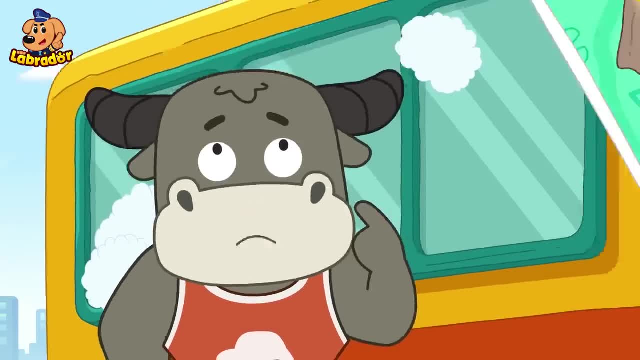 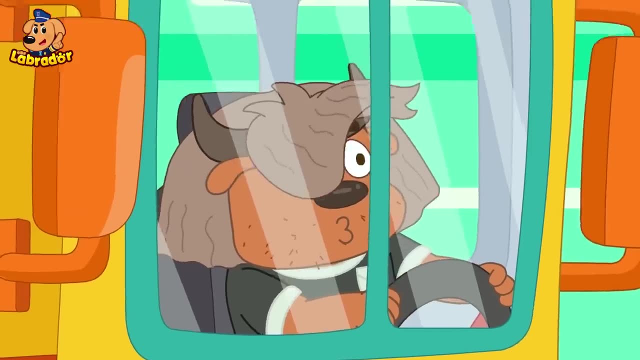 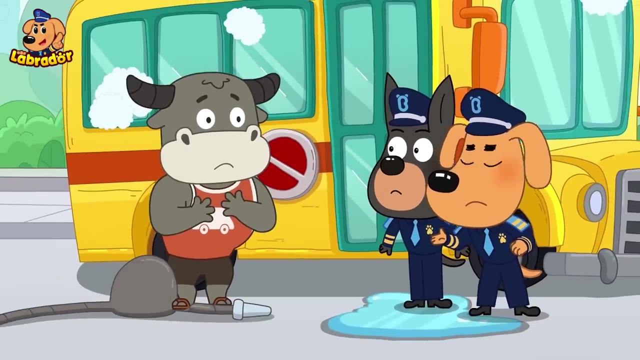 You've got the wrong person here. I'm Buffalo. Mr Yak's hair is much longer than mine. Sometimes I wonder if he can actually see when he's driving. Well, do you know where Mr Yak is right now? No, I don't. 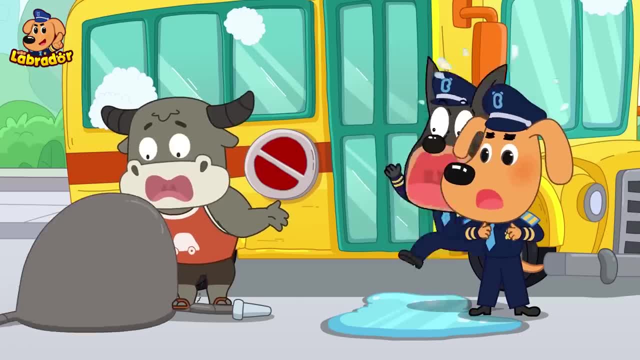 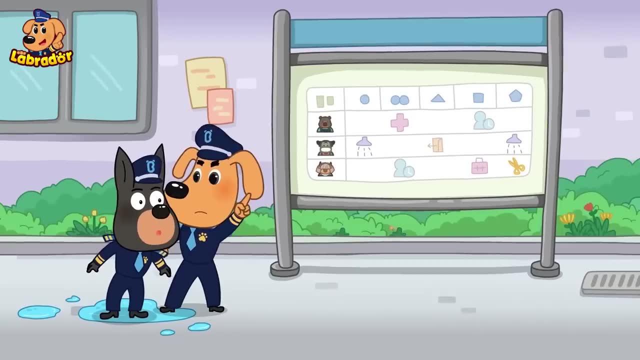 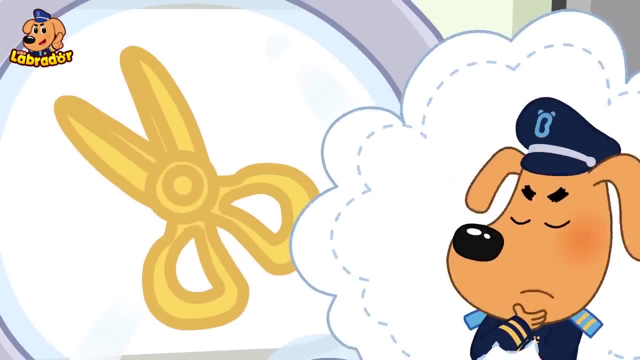 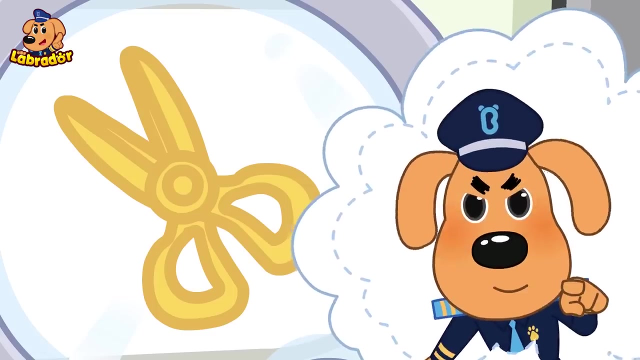 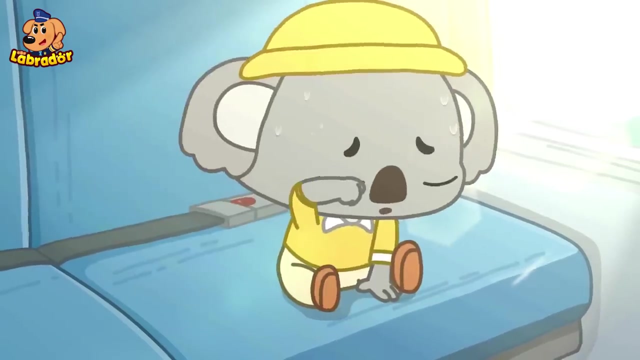 His bus is not here. This is the driver's schedule. This is the logo of the Golden Scissor's hair salon. Mr Yak is probably getting his hair cut there. Let's go. It's so hot. Where am I? Oh, it's so hot. 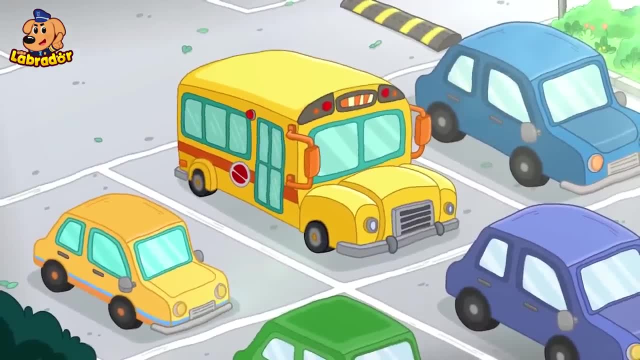 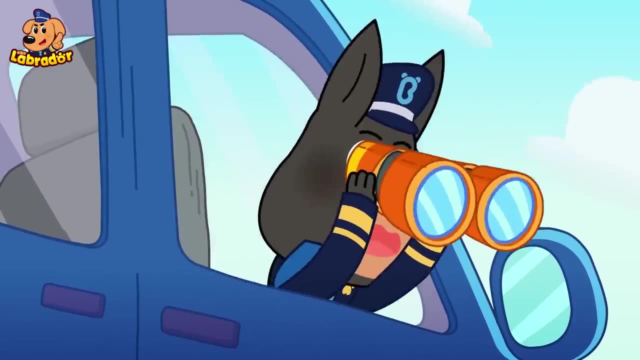 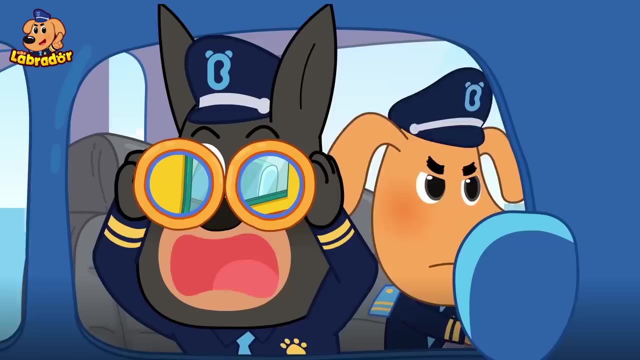 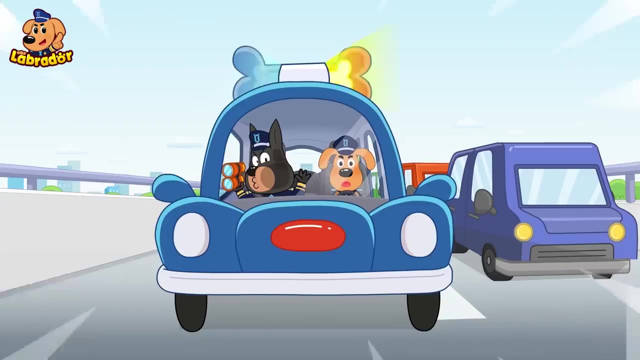 I can't get out. Help, Somebody help me. It's Little Koala. He's stuck inside the bus. Oh no, He has fainted. We need to go save him right now. Oh no, We are stuck. 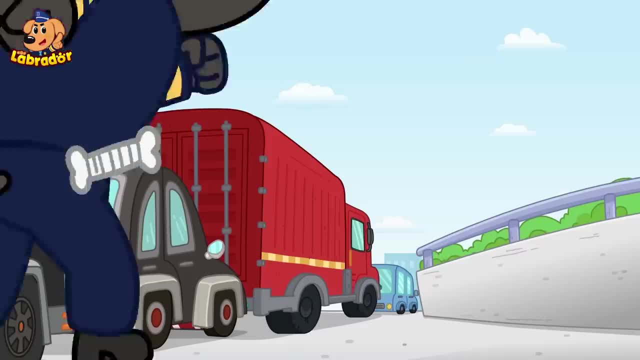 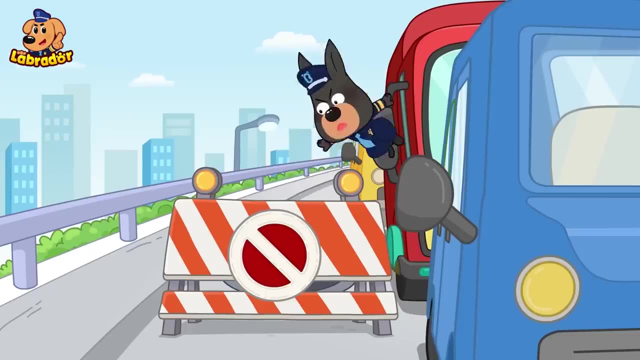 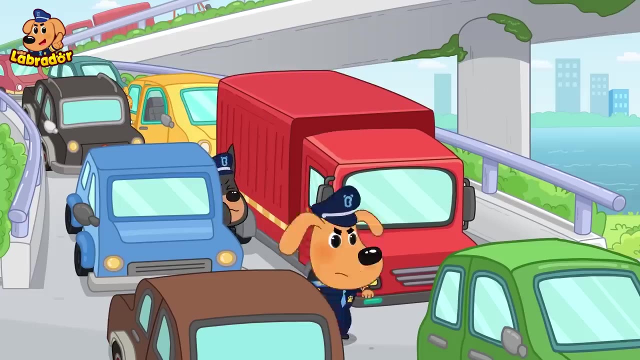 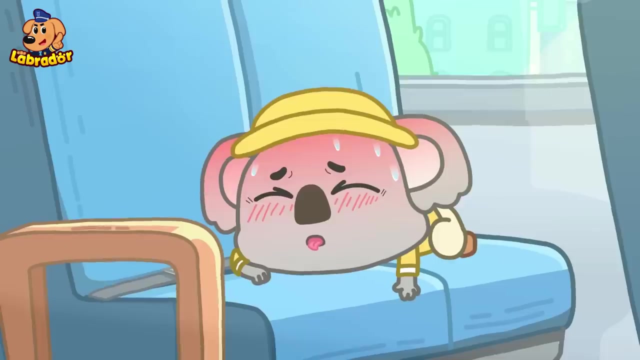 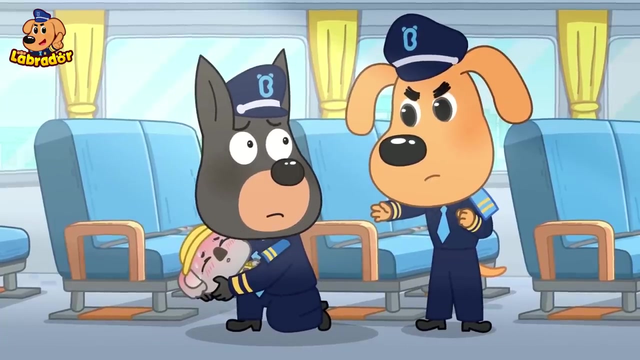 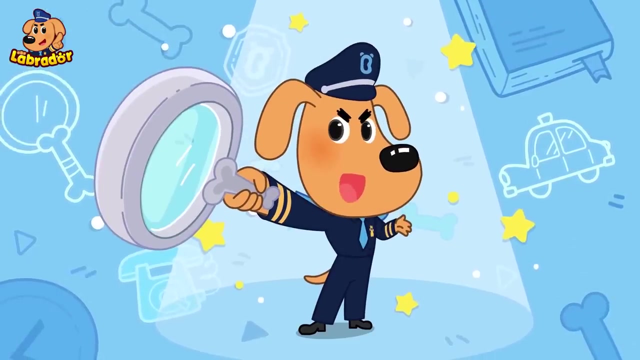 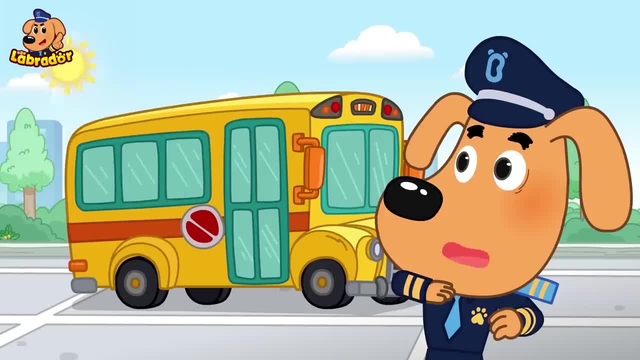 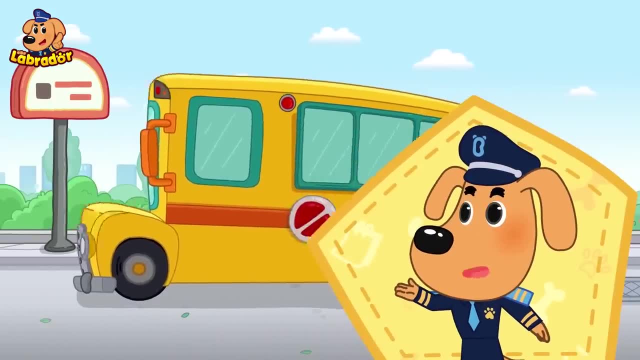 Especially in the summer, the temperature inside the car can get very high, so children's lives might be in danger. Also, children should always remember to get off the bus at the right stop. If you ever get stuck in a car, try to go to the doctor. 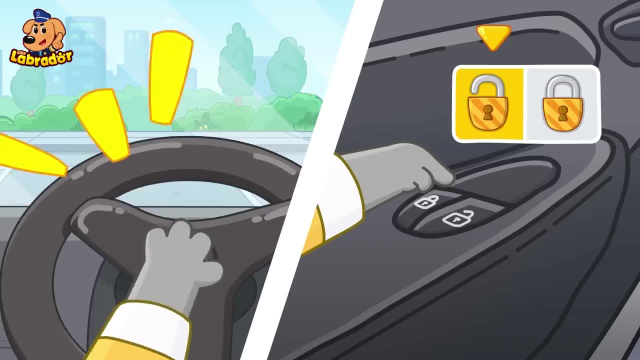 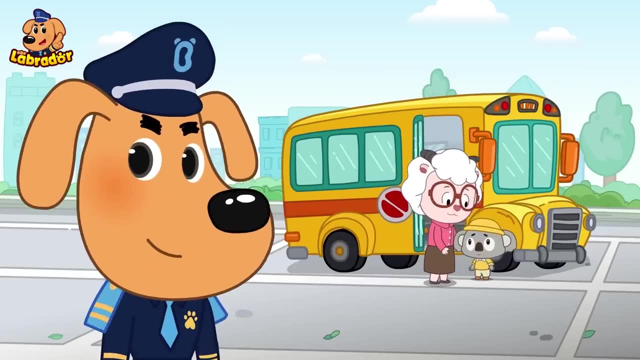 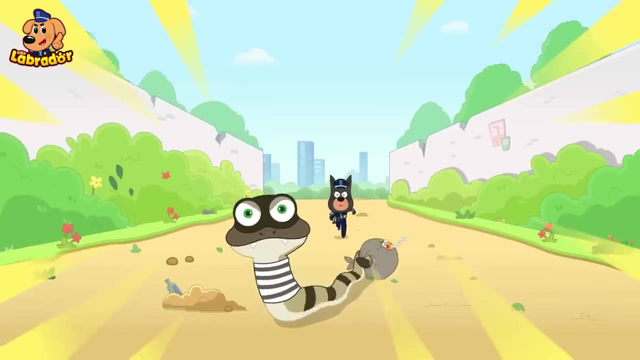 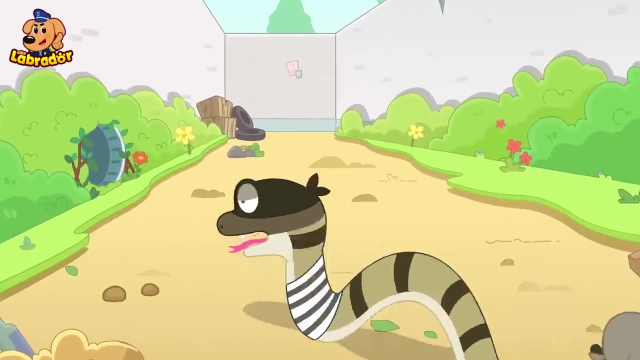 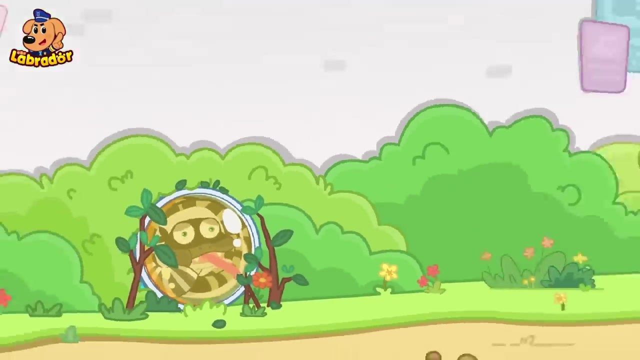 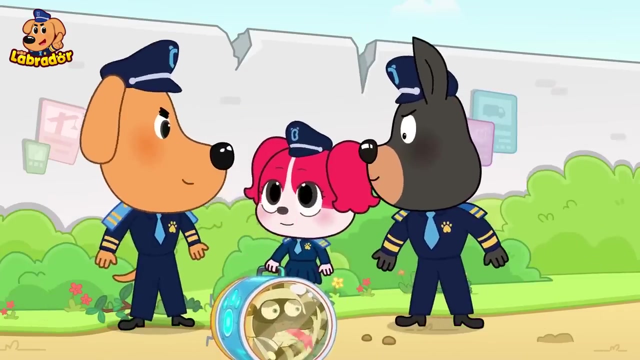 to go to the driver's seat and unlock the doors or honk the horn to get people's attention. please remember these tips, whoop: don't play in construction sites, don't even think about it. you're going to the police station with. you're going to the police station with. 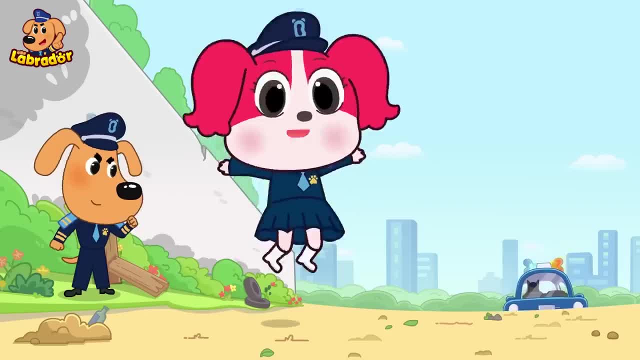 you're going to the police station with me, me, me, good job, papillon. papillon always has a good job. papillon, papillon always has a good job. papillon, papillon always has a way, way, way, wow. there are so many construction. wow, there are so many construction. 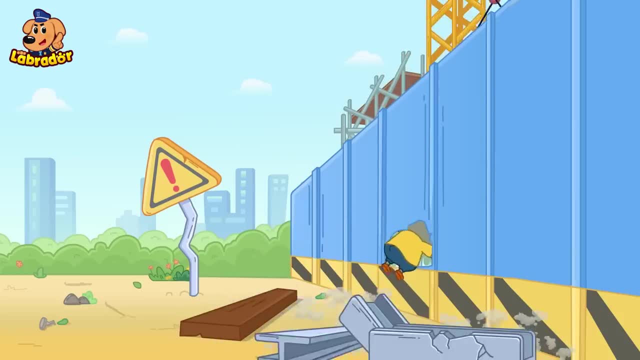 wow, there are so many construction vehicles in here. let's go in vehicles in here. let's go in vehicles in here, let's go in. oh no, little wild geese went into the. oh no, little wild geese went into the. oh no, little wild geese went into the construction site. it's dangerous in. 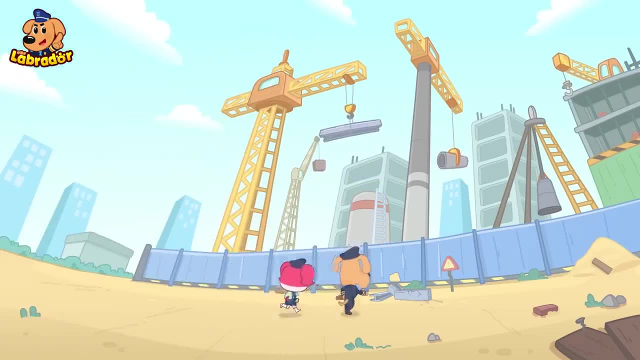 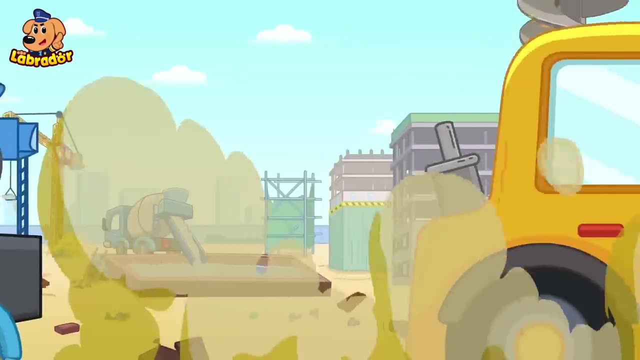 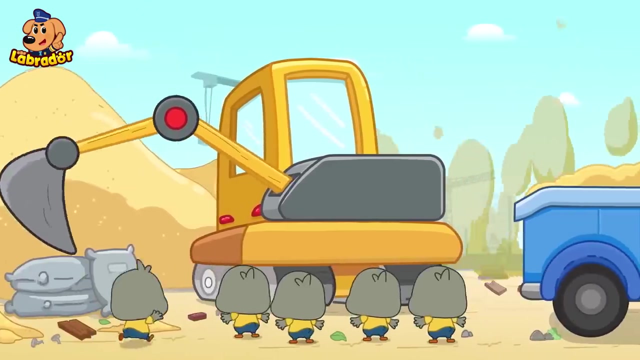 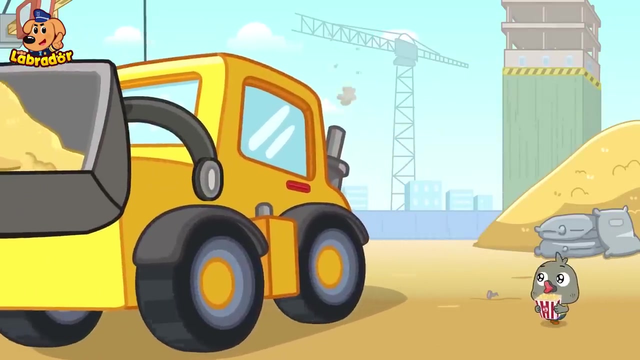 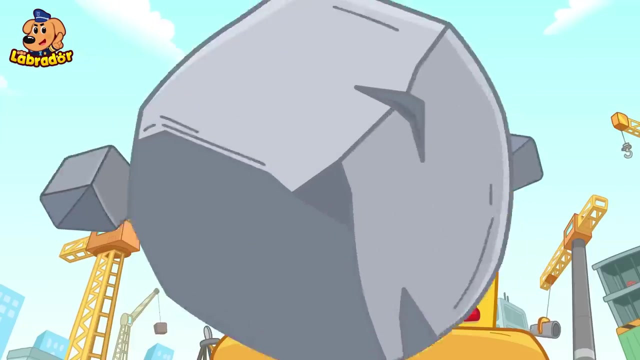 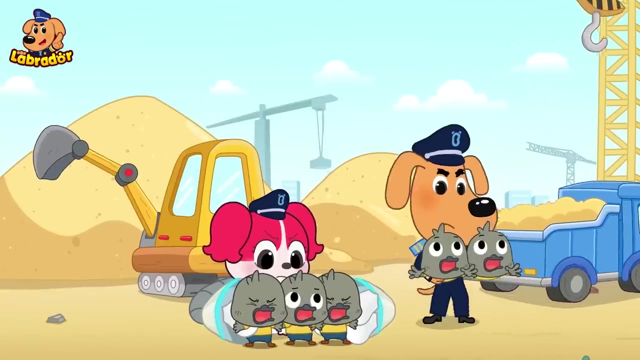 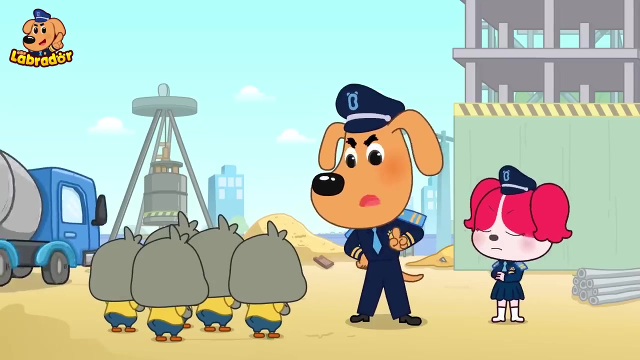 construction site. it's dangerous in construction site. it's dangerous in there. we need to get them out. wow, wow, wow, wow. Look It's an excavator. Wow, It's a loader. It's my favorite. Watch out, Thanks. Construction sites are very dangerous. You should never play here, okay. 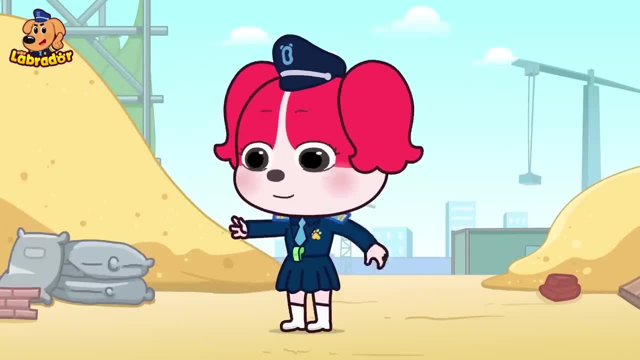 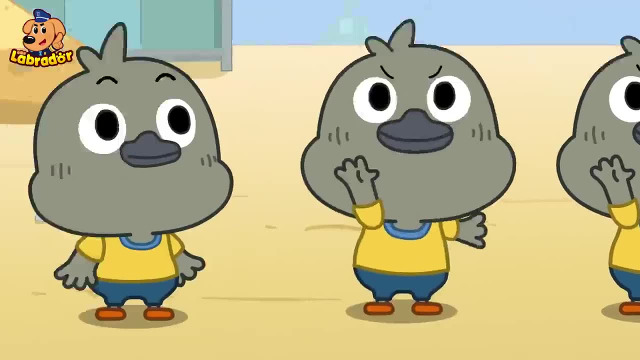 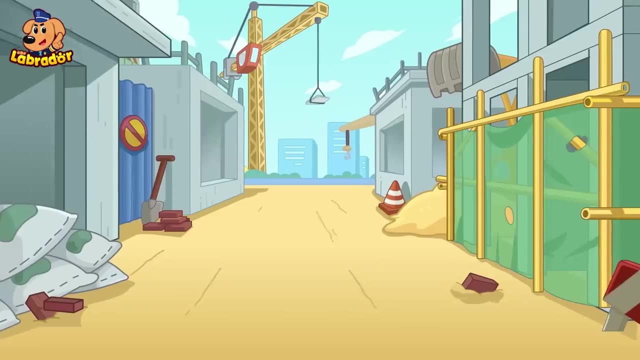 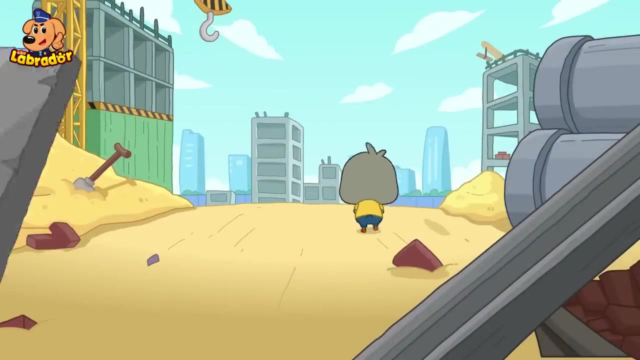 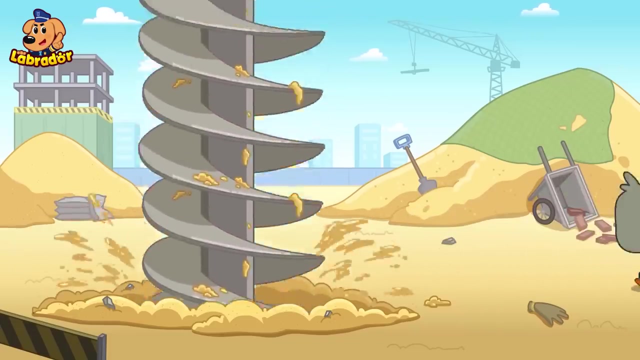 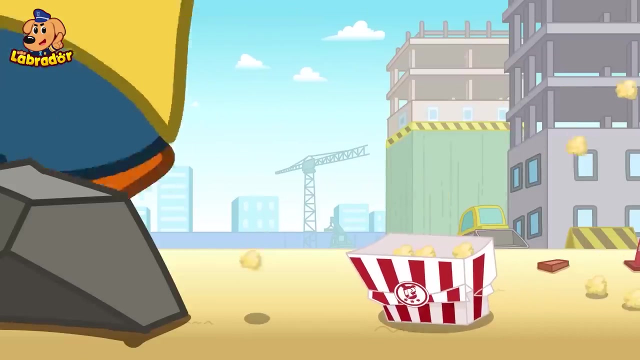 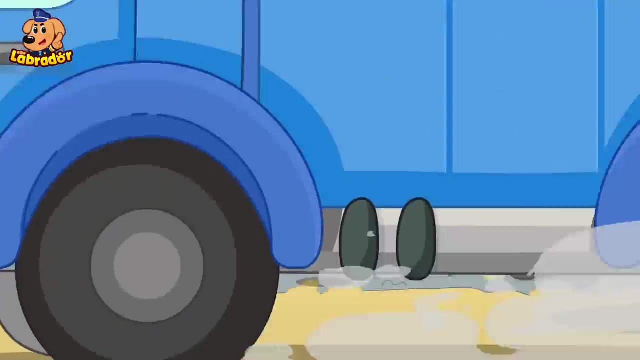 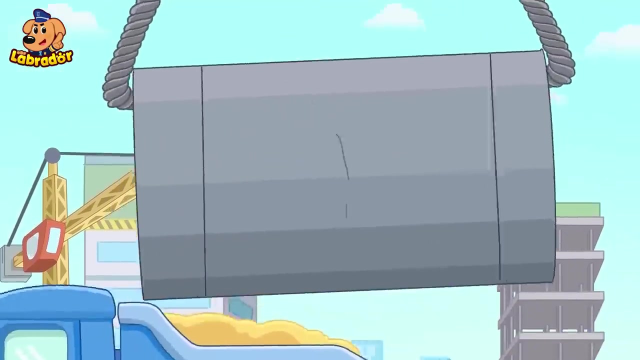 Okay, Everybody line up and count off. One, two, three, four, Six, Five is missing. We need to find him right now. Wow, Wow, It's so dirty. Oh no, It hurts What's going on. 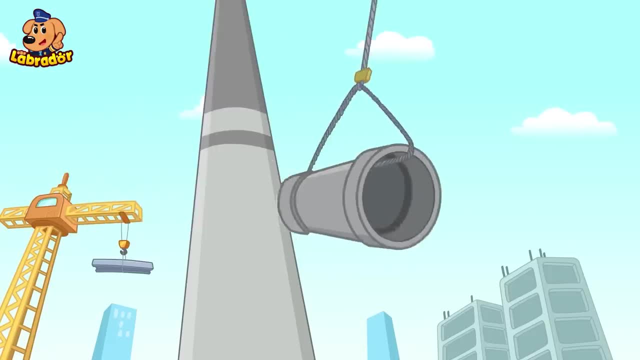 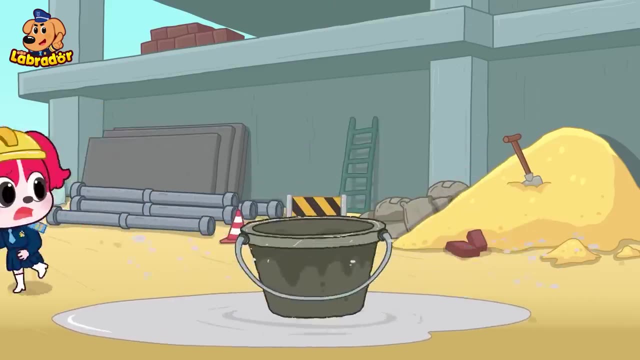 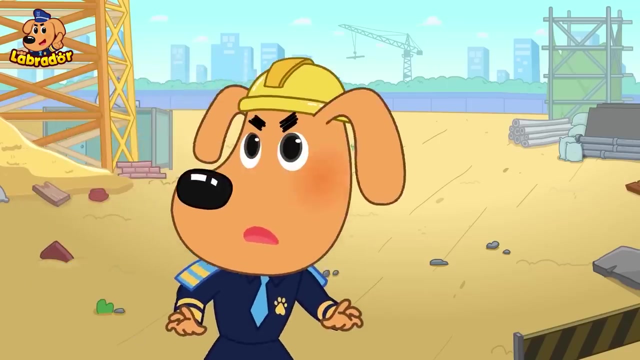 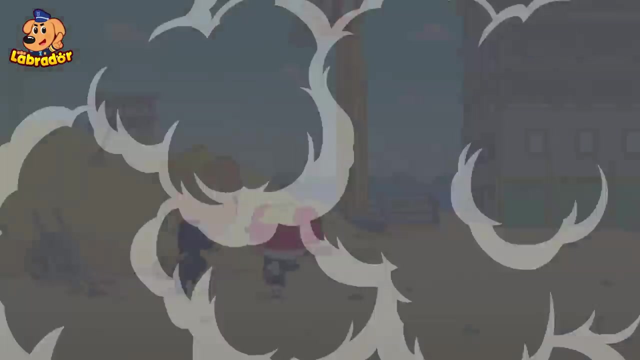 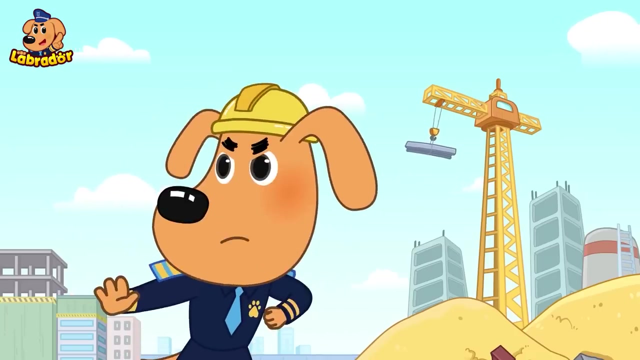 Help, Help Little wild goose. Whoa, Little wild goose, where are you Watch out? It's so dangerous here and it will be hard to find him. We need to use search engines. We need to use search equipment. 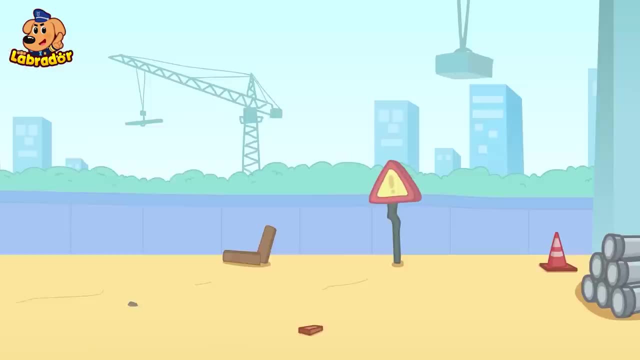 Got it. Ta-da, The awesome searching robot, Little Wonton. He'll help us find what we're looking for. Little Wonton Help us find Little Wild Goose. Ton ton, Ton ton, Little Wild Goose. Little Wild Goose. 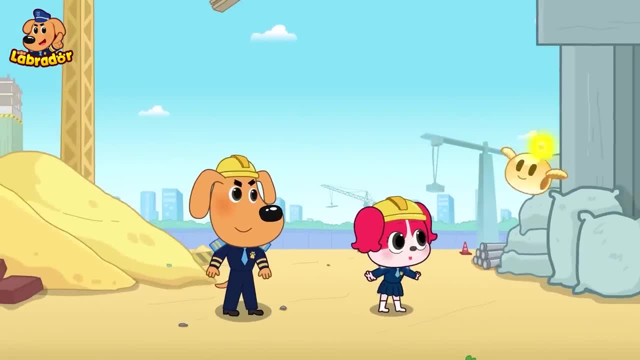 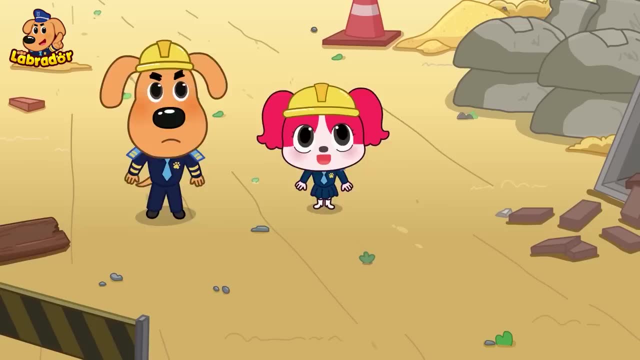 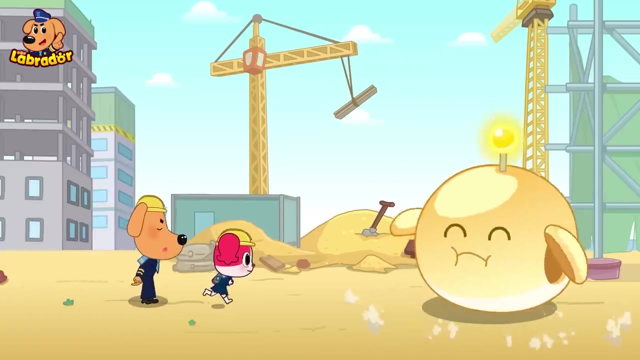 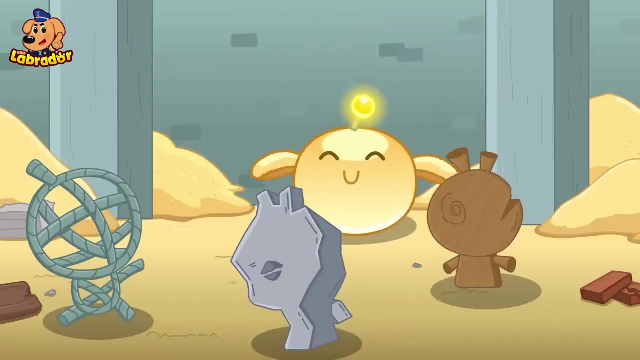 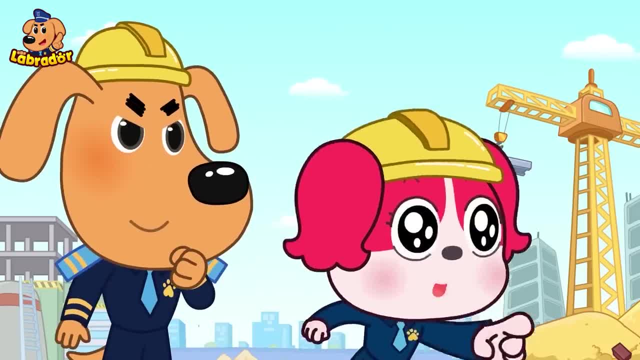 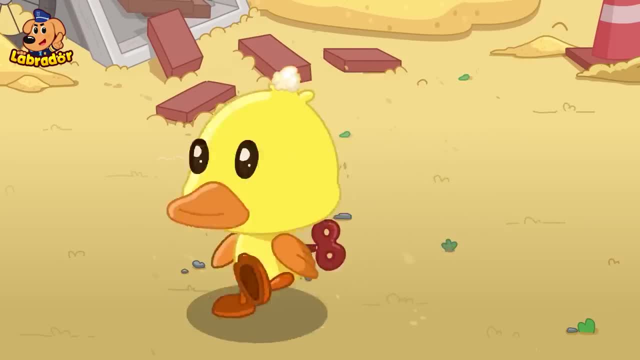 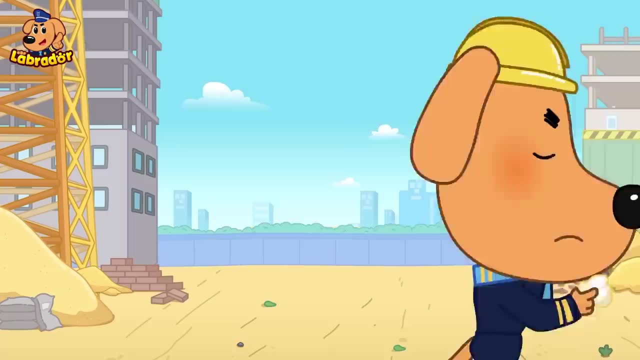 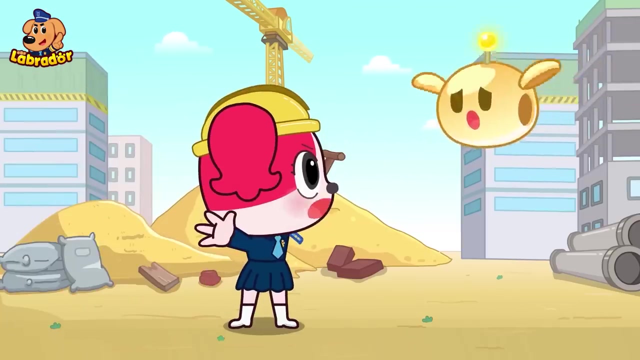 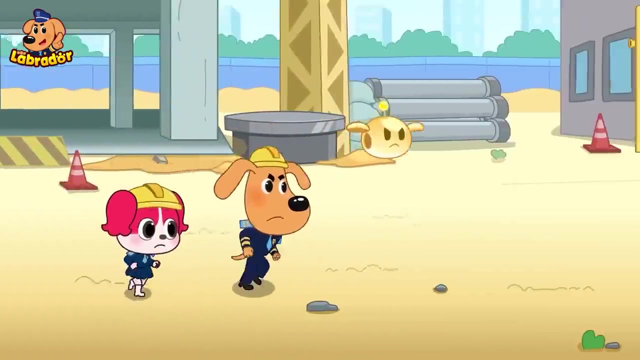 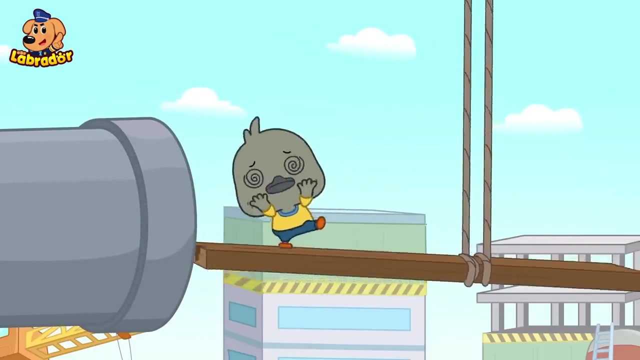 Ton Ton. It must be Little Wild Goose. I am a little duck. Hold on Popcorn. Where did you find this? Huh, Little wanton, lead the way. now I'm so dizzy, It's so high. 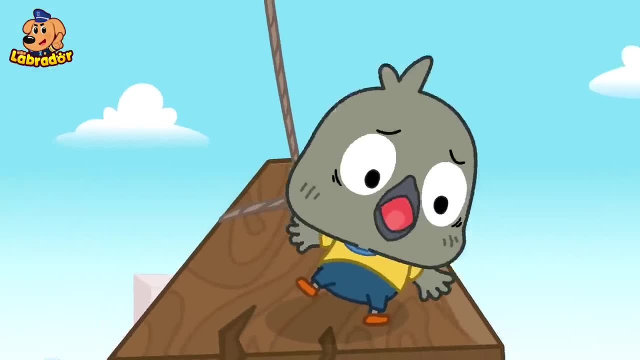 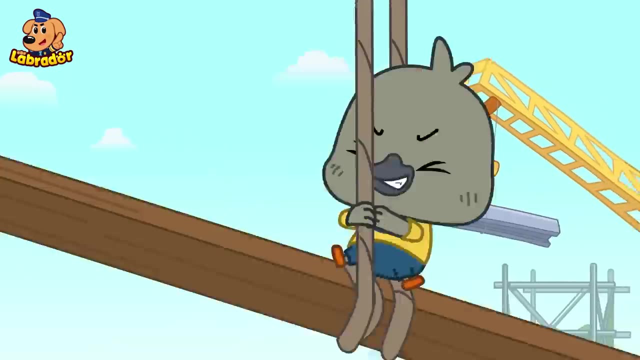 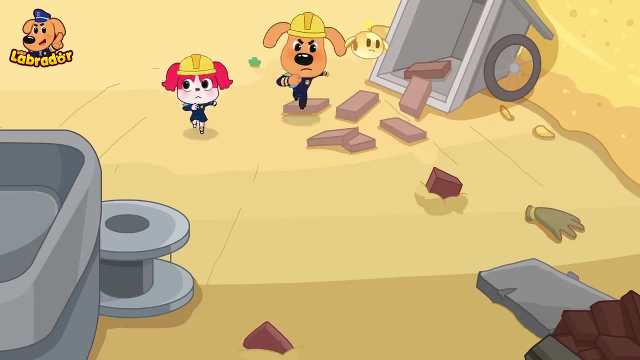 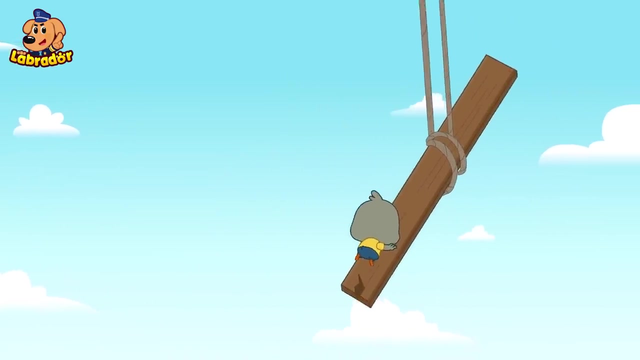 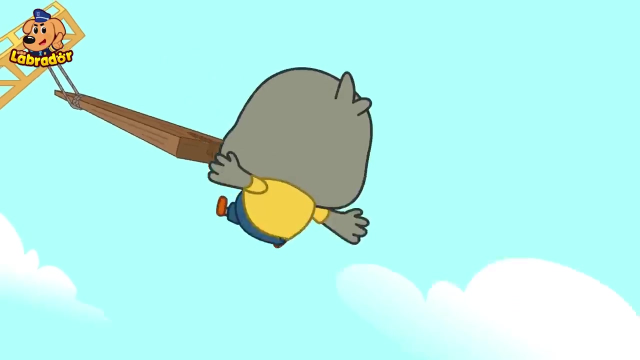 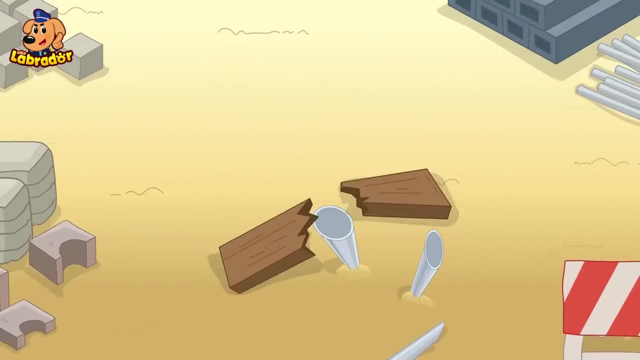 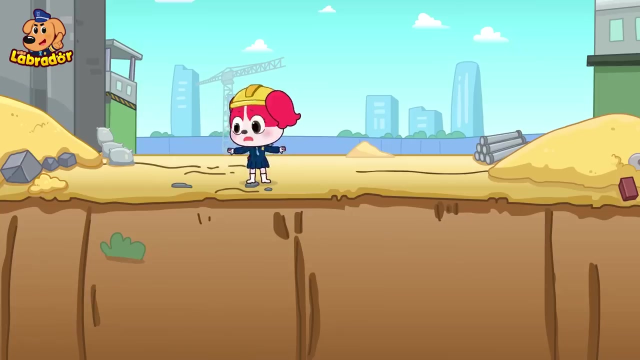 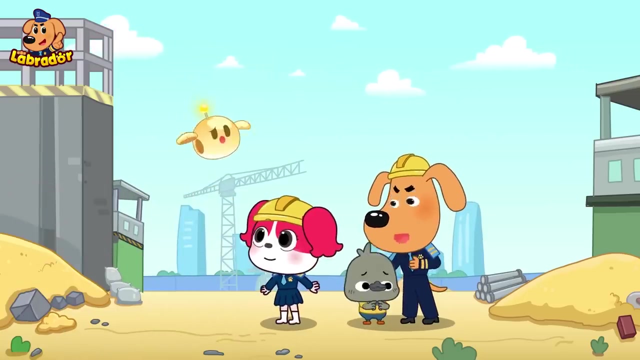 Huh, Help me. Someone's calling for help Over there. Help me, Please. He's in danger. Hurry, let's go. Okay, Yeah, Sheriff Labrador, Ton-ton, Ton-ton, We're all right. Thanks, little wanton. 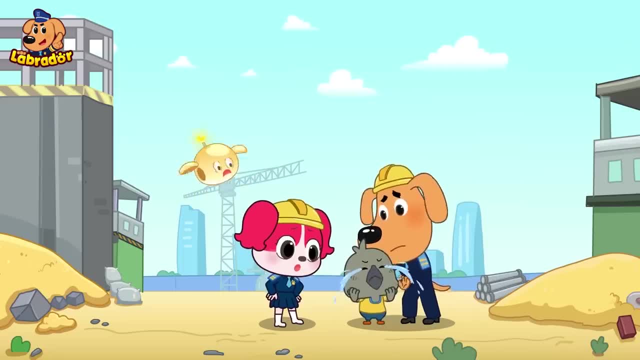 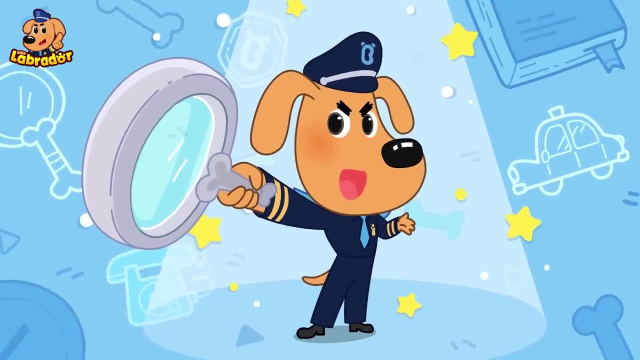 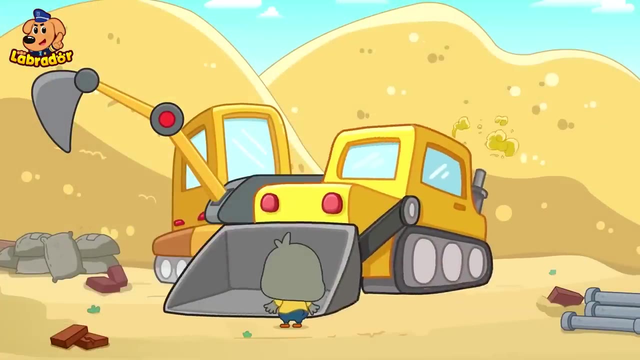 That was so scary. I'll never play in construction sites again. Sheriff Labrador's Safety Talk. Construction sites are very dangerous. They are full of steels and cement. Construction vehicles often move around. You might get hit and even get hurt. Cranes lift materials up in the air. 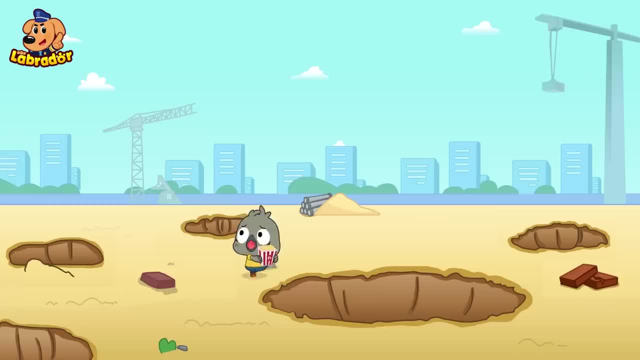 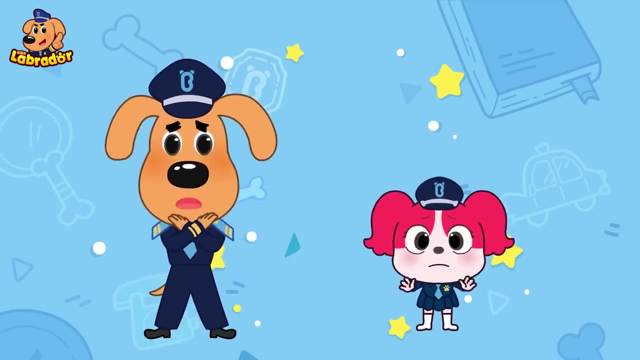 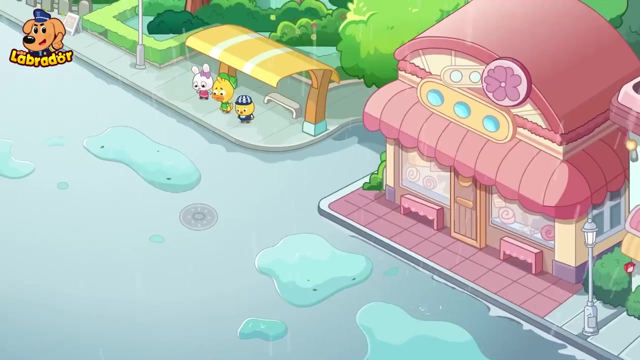 They might fall and hurt people. There are also big and deep holes. If you get close to one, you might fall in. Kids, please remember these and never play in construction sites. Woof, The Scary Puddle. Wow, It stopped raining. 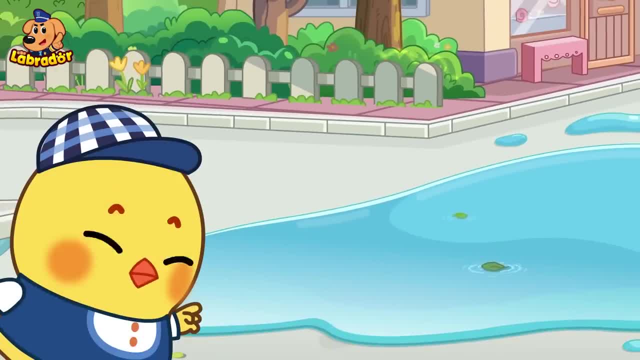 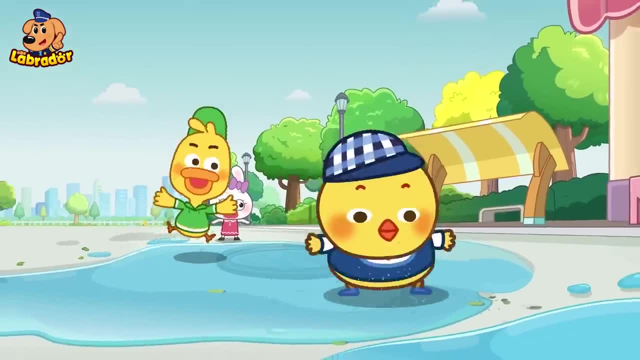 Look, There's a big puddle over there, Let's go play in it. Okay, Here I come. Hey, Jump into the puddle, Jump into the puddle, Let's all jump, Let's all jump, Let's all jump. 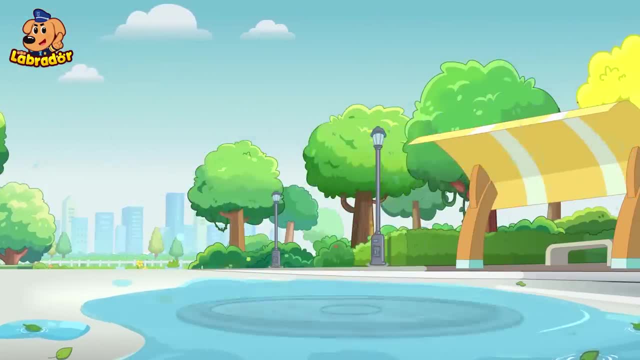 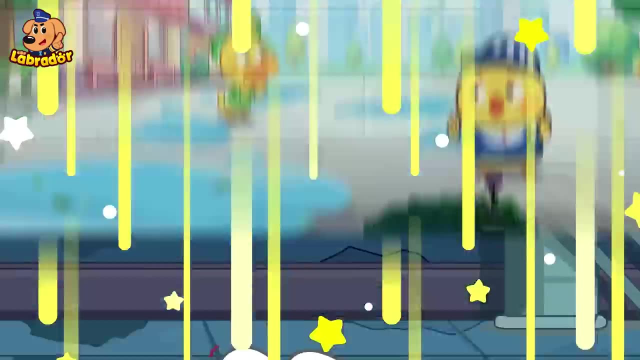 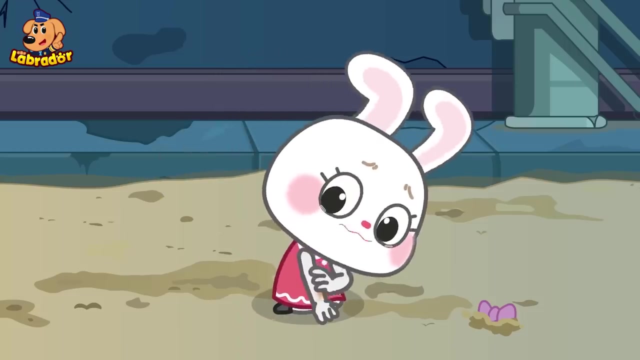 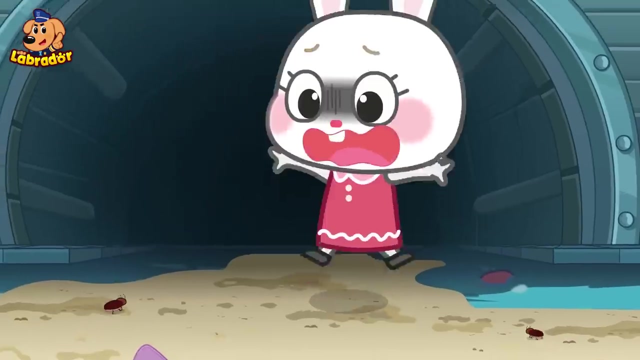 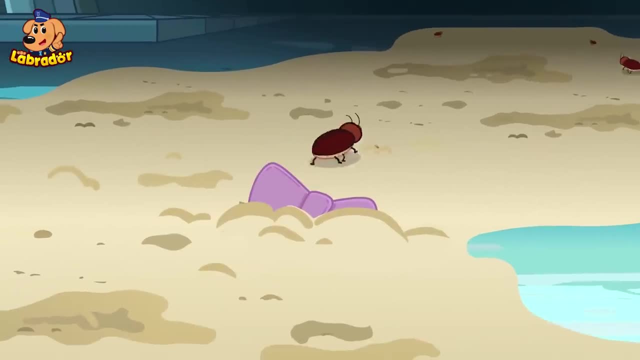 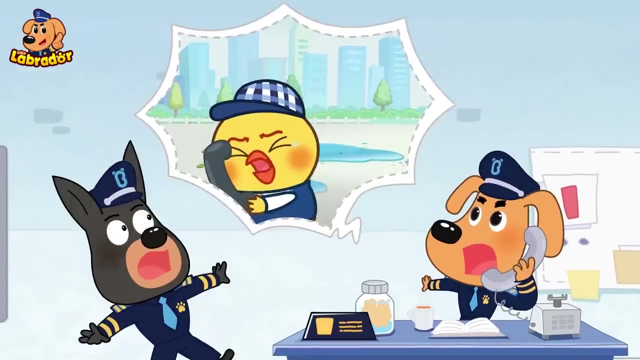 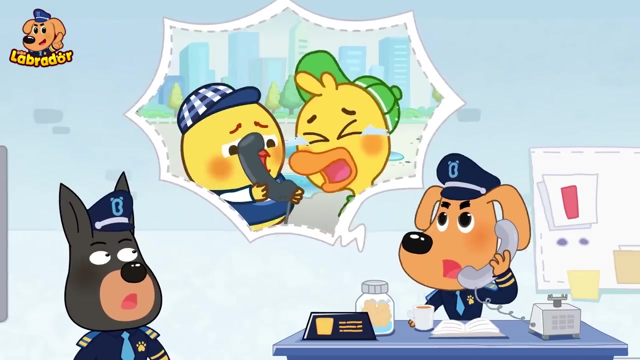 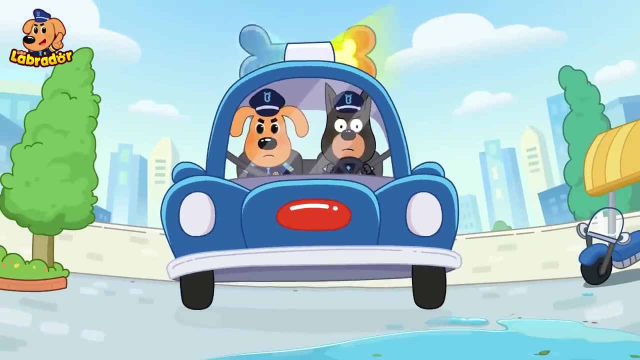 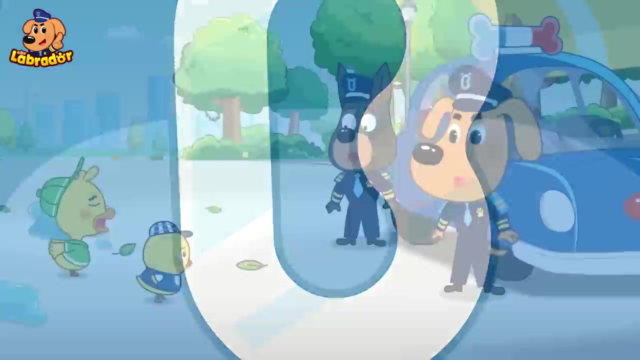 It hurts. Ah Ah Woof. Hi, I'm Sheriff Labrador. No, Labrador, Little Rabbit is missing. We can't find her anywhere. Please come help us. Don't worry kids, We'll be right there, Sheriff Labrador. we were playing with Little Rabbit here and suddenly she disappeared. 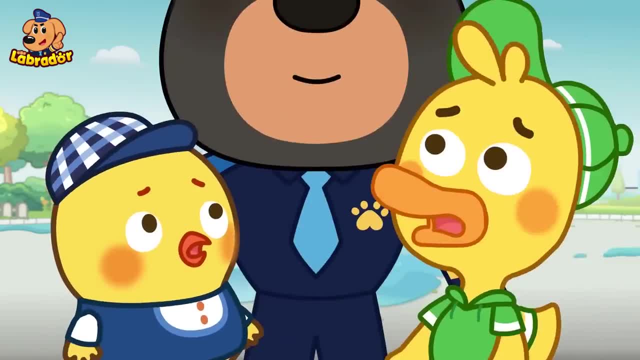 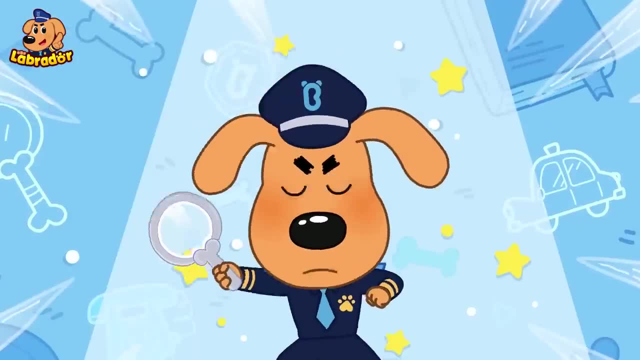 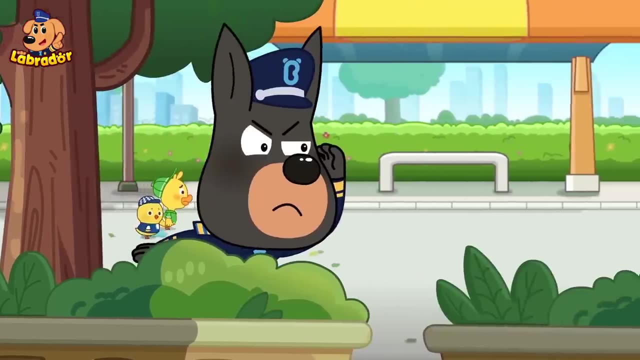 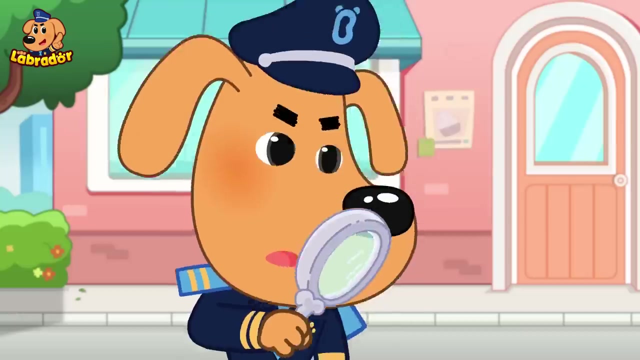 I'm so scared. Don't worry, we'll find Little Rabbit Right. There's no case that I can't solve. The footprints are not in a straight line. Hey kids, what game were you playing just now? Jumping in the puddle game? 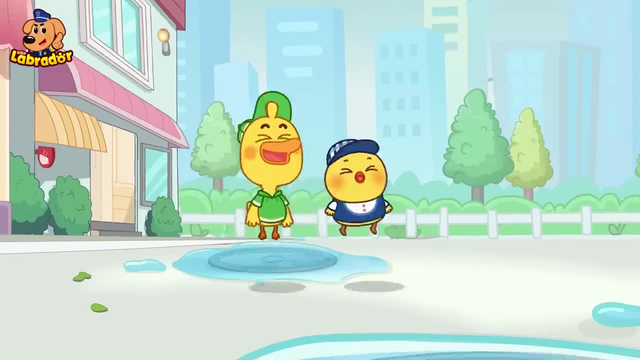 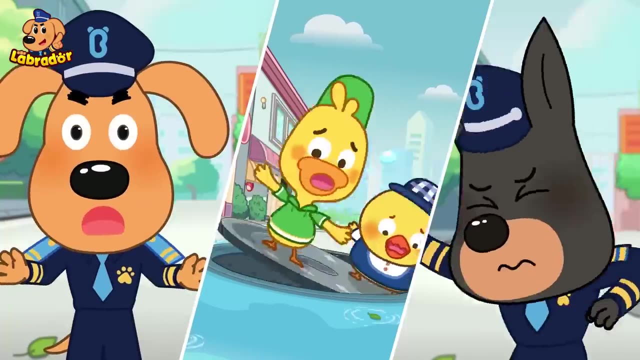 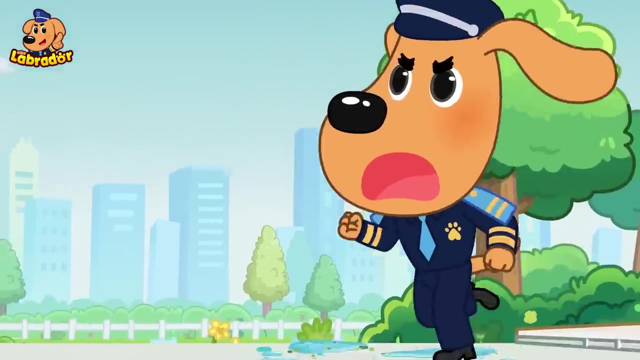 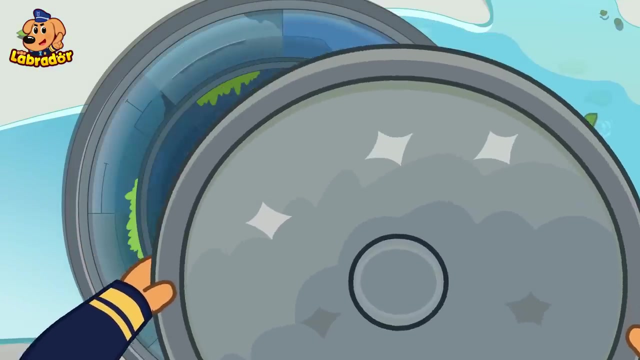 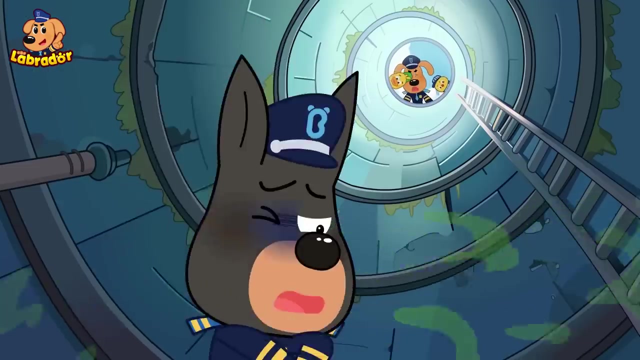 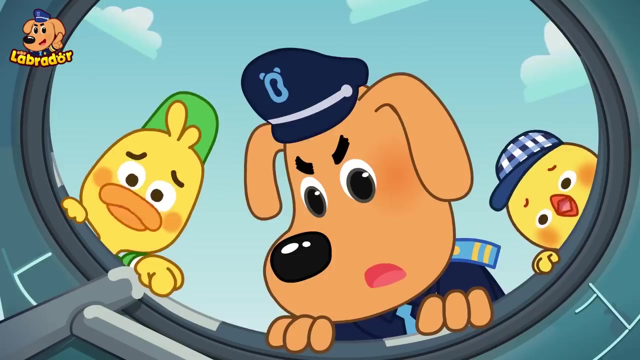 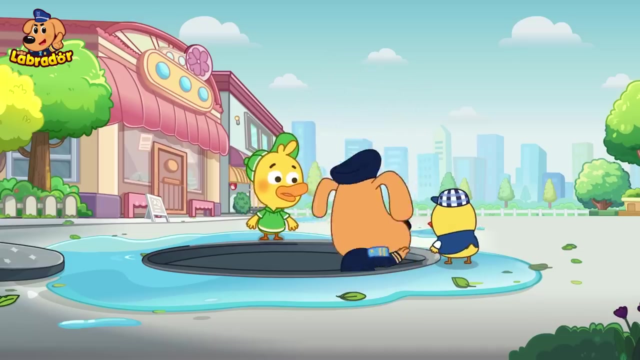 It was so much fun Jumping in the puddle by the road. That's so dangerous. Watch out, Dobie, It's Stig's. It's Stig's. Look at this. It's Little Rabbit's ribbon. Don't get close to the manhole. I'm going down to help Officer Dobie find Little Rabbit. 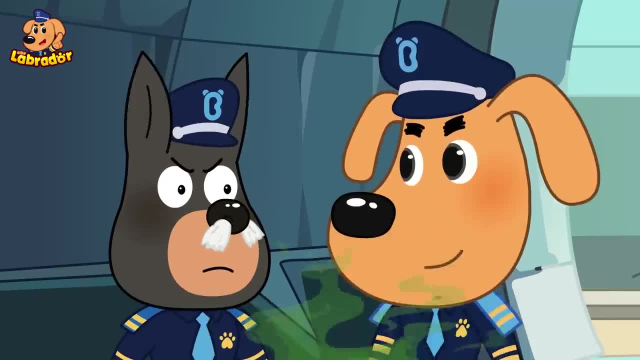 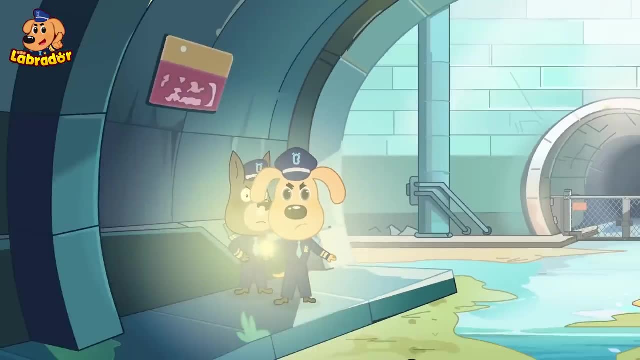 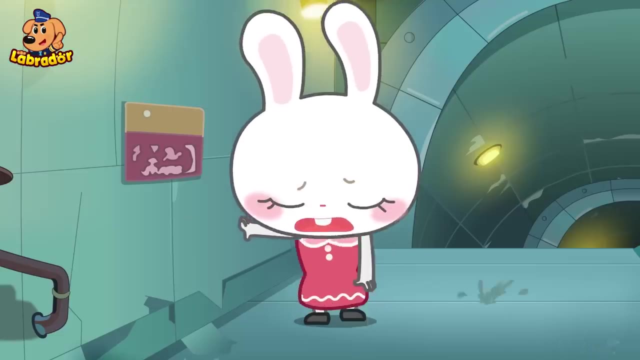 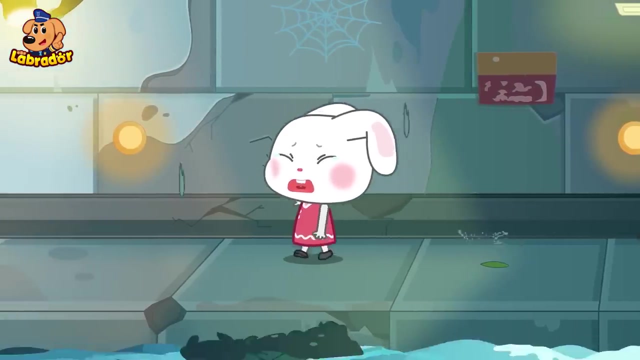 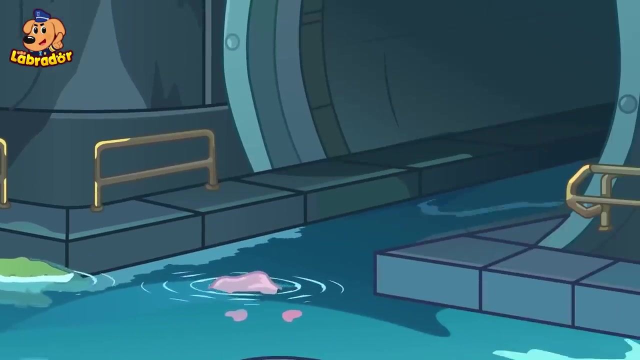 It stinks down here. This way's blocked Little Rabbit would have gone this way. Somebody help me, please Help me, Help me, Help me. The tunnel splits here. Which way should we go? Let me listen, Let me listen. 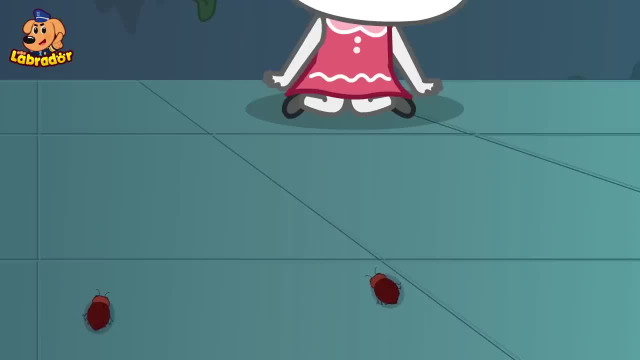 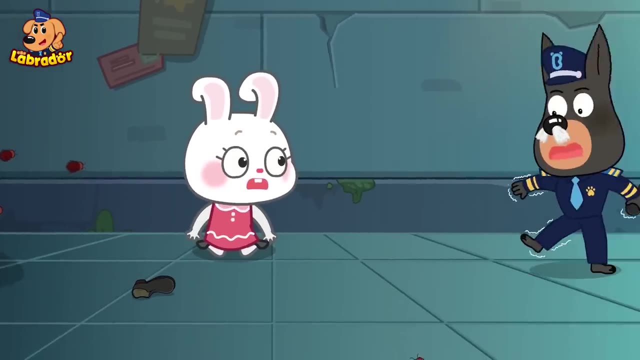 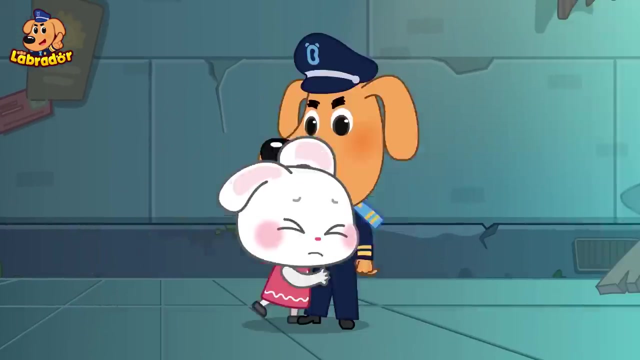 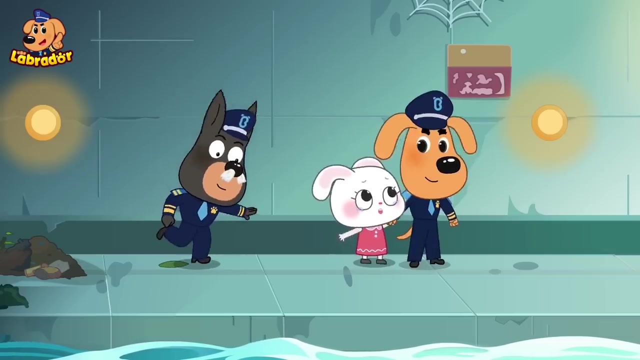 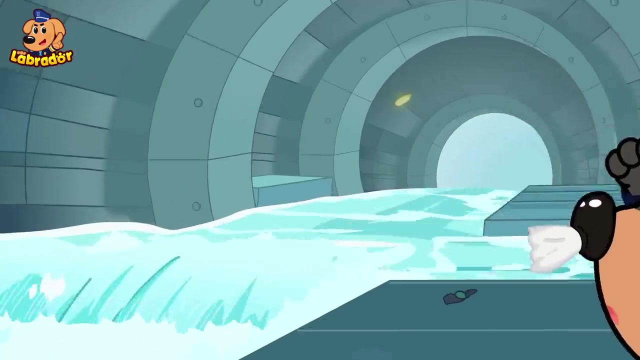 That way, That way. No, Stay away from me, Little Rabbit, Go away. Go away, Sheriff. Rapporteur. Don't worry, Little Rabbit, We'll get you out of here. Oh no, The wastewater is coming this way. 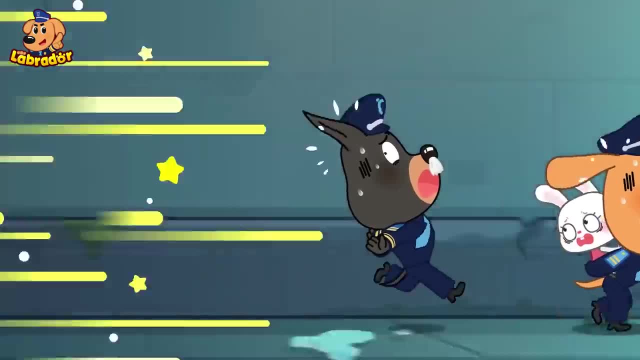 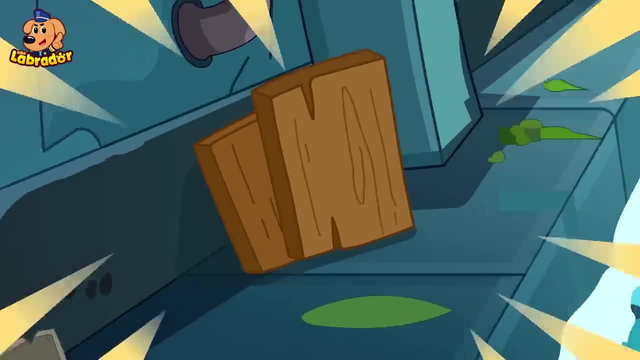 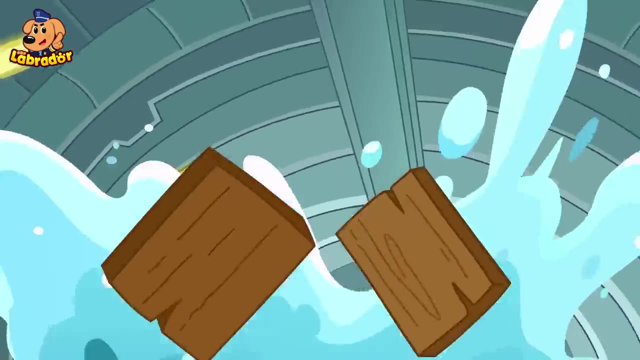 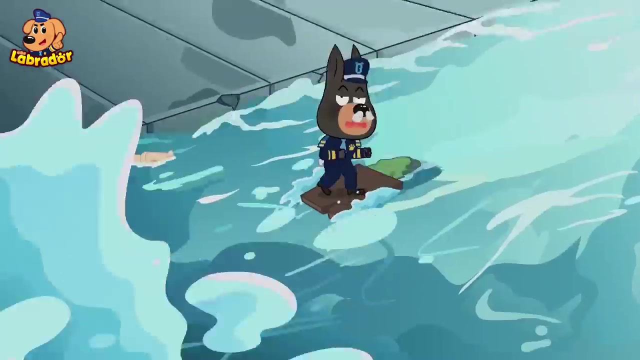 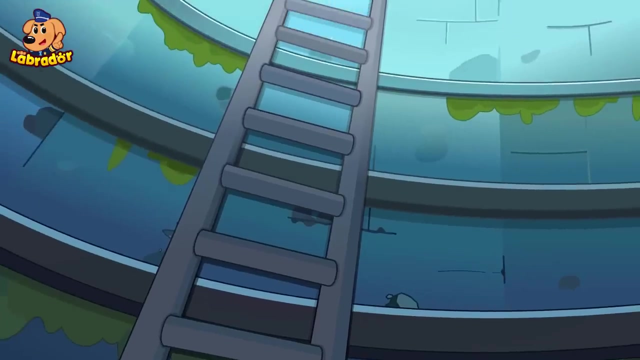 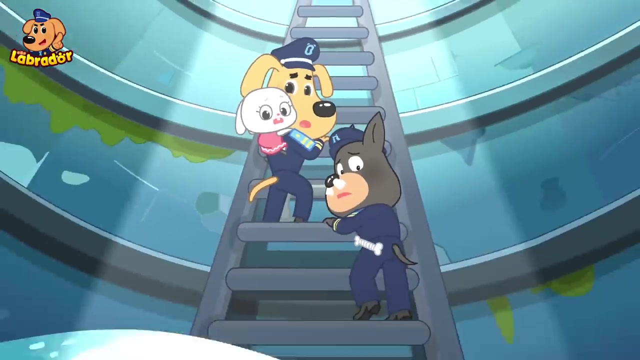 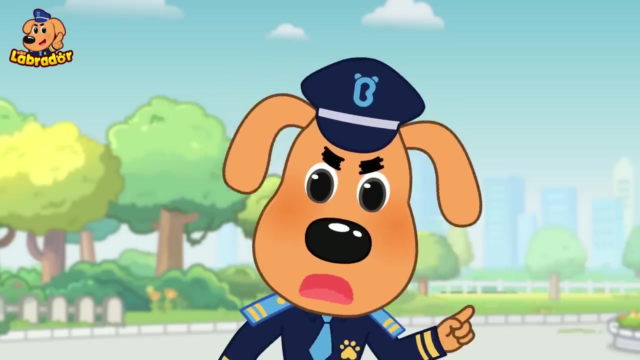 Let's run. It's moving so fast, Dobby, use those boards, Let's go Jump now. Kids, you should never jump in puddles by the road. It was so scary down there. We'll never do that again. 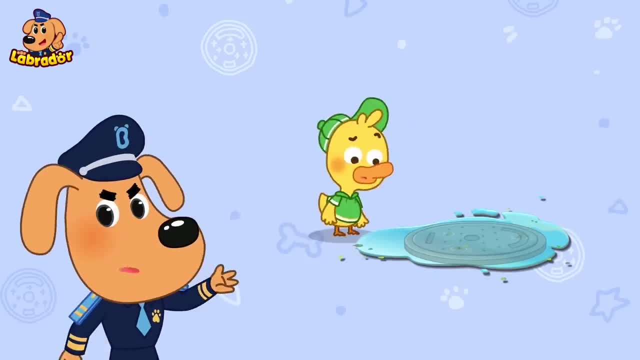 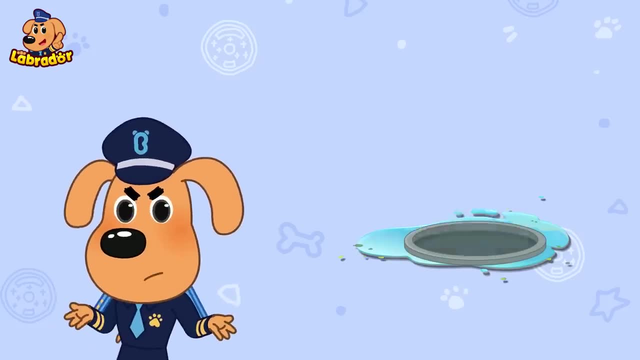 Kids don't jump in the puddles by the road. There might be dangerous things in the puddles that you can't see, And if you step on a broken manhole cover, you could fall down and get hurt. Also, there might be dangerous things in sewers, such as bugs, rats or harmful gas. 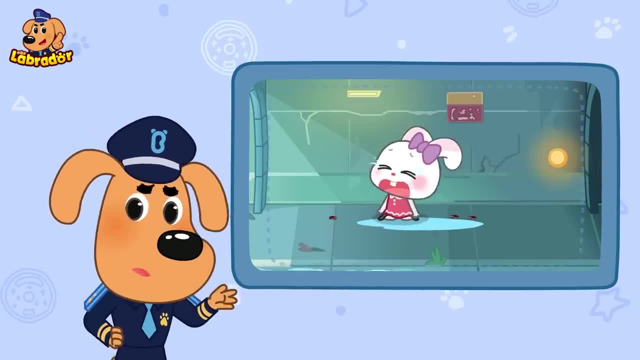 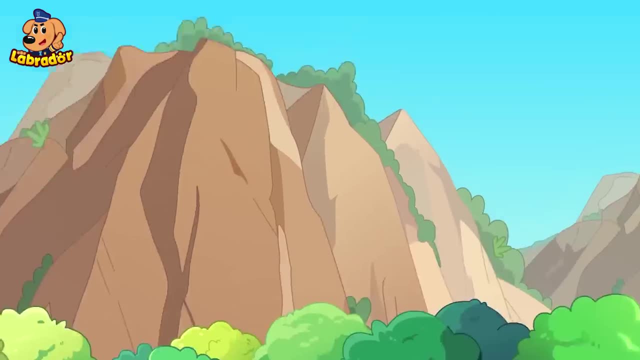 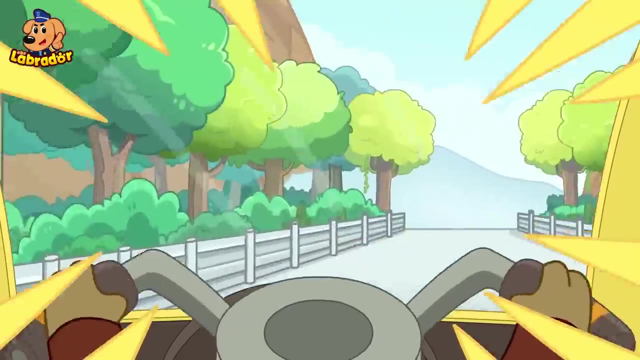 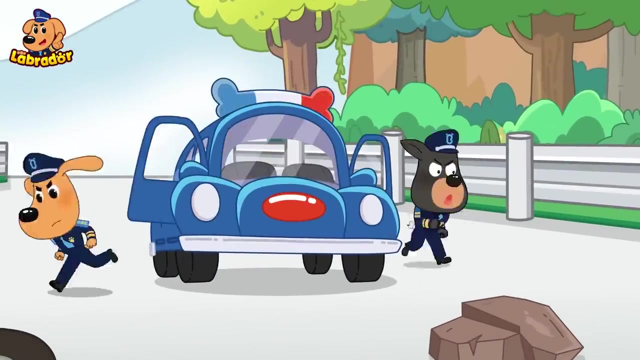 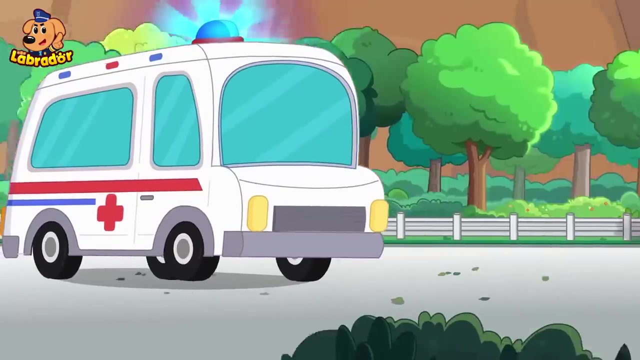 that might endanger your life, So please stay away from them. Woof, Outdoor Earthquake Safety. Ouch, Oh, My leg, Oh It hurts. Mr Turtle, don't move. We'll call an ambulance. He needs to go to the hospital right away. 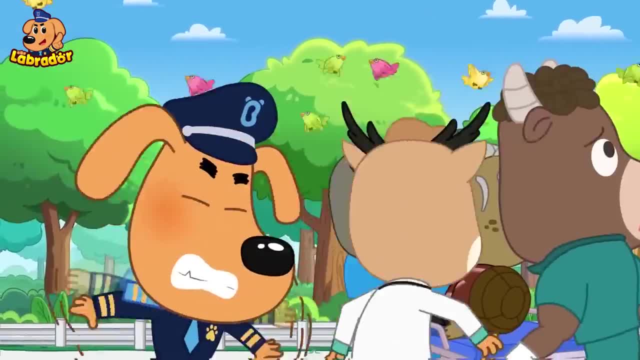 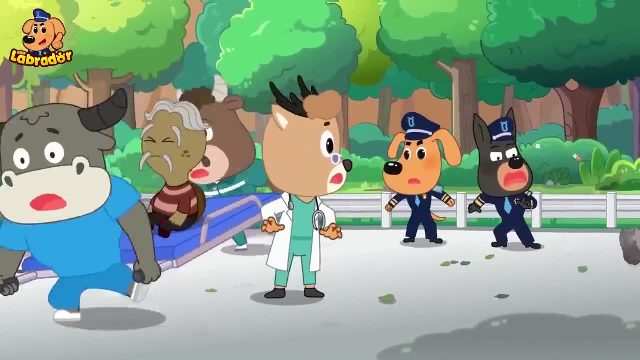 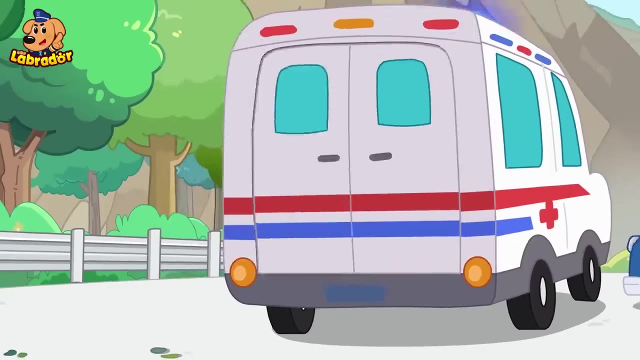 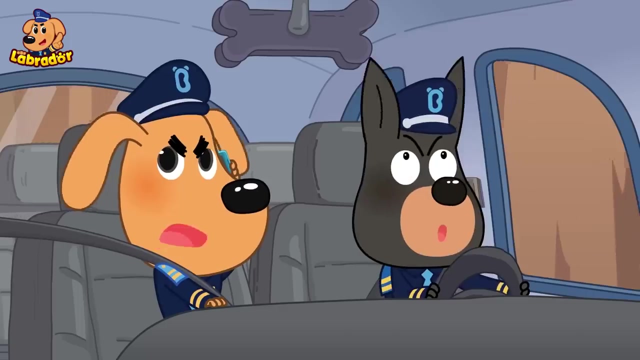 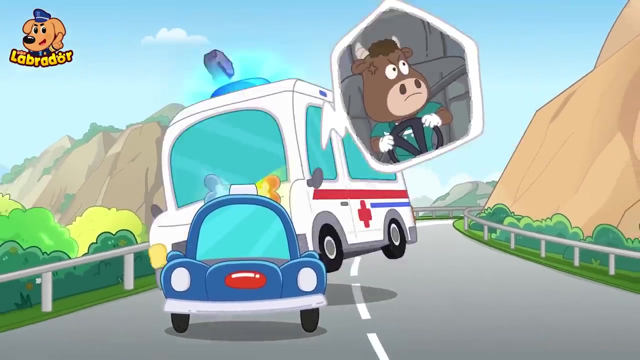 Ah, What's going on? Oh no, It's an earthquake. Let's evacuate. Follow me. Follow me, Mr Bison. there may be falling rocks near the cliff. Please drive carefully, Okay, Oh My goodness, Watch out. 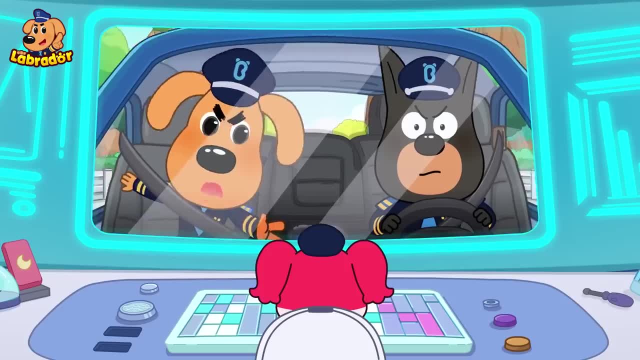 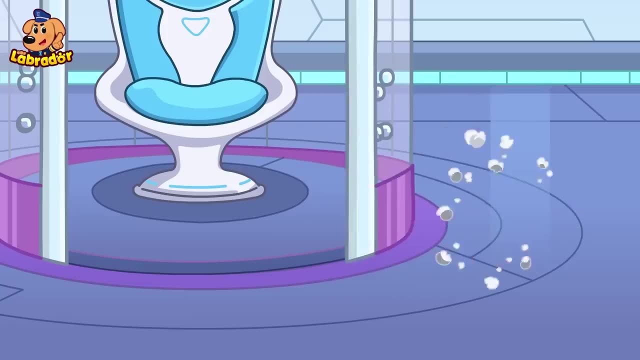 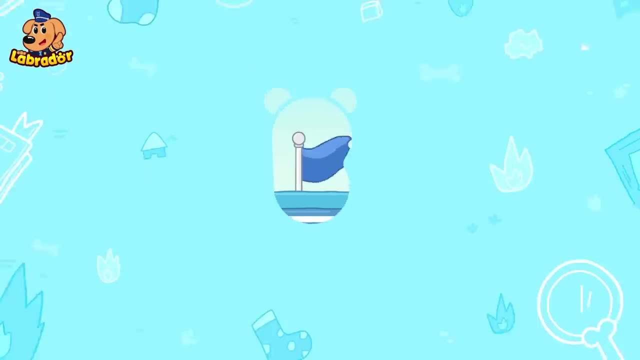 Papillon, there's an earthquake And we're in danger. here. We need your support. Got it. Eek, Eek. Papillon always has a way. Eek Huh, Eek, Woof, Woof, Woof. 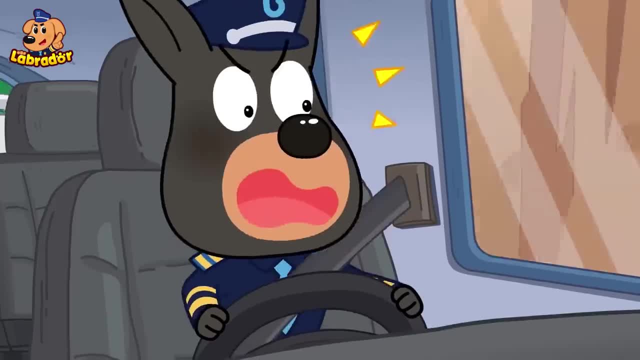 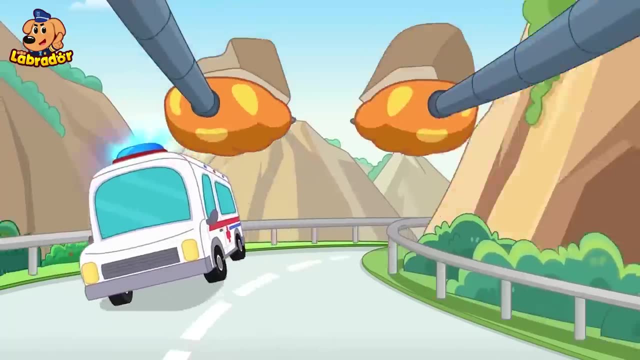 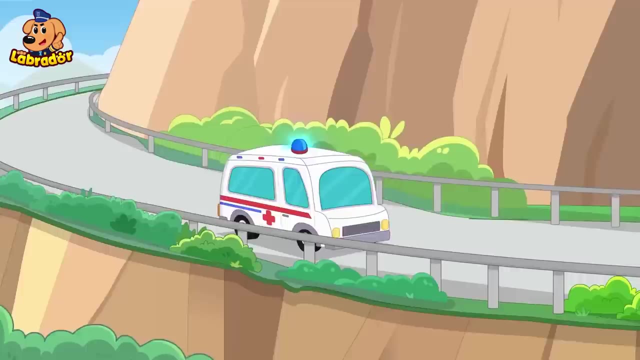 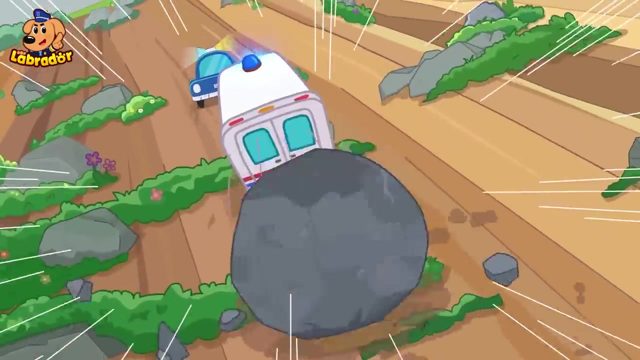 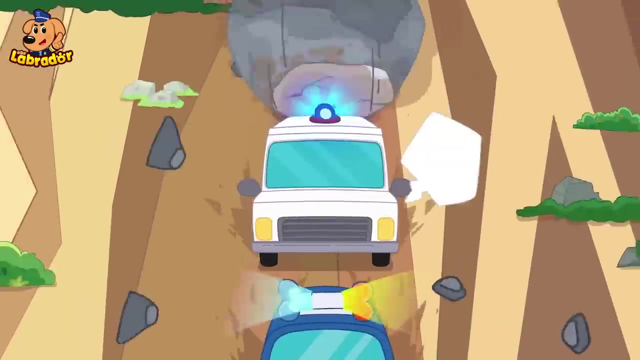 Help? Ah, Fine course, Woof, Ah, Ah, Ah, Ah, Oh no, Oh my, A rock is falling. It's about to hit us. Why is it following us? Don't go in the direction where it's falling. 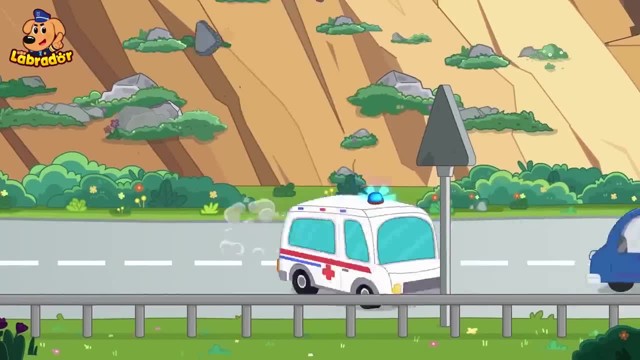 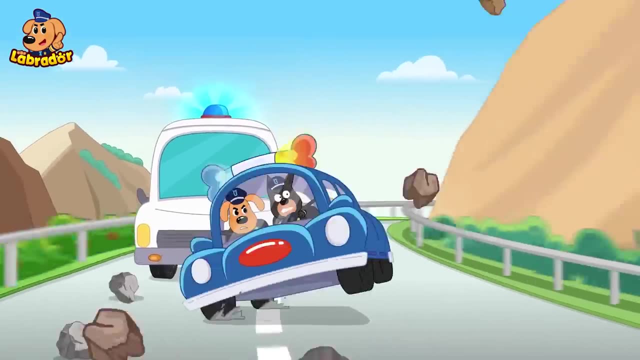 Move to the side and keep up with us. Oh no, That was really close. Huh Huh, Look safe over there. Let's go. We'll wait until it stops shaking. Eek, Eek, Eek, Eek. 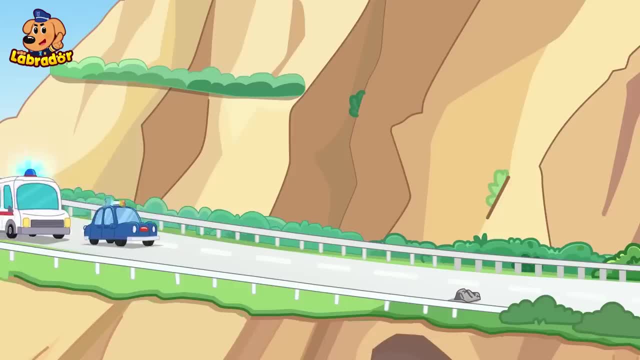 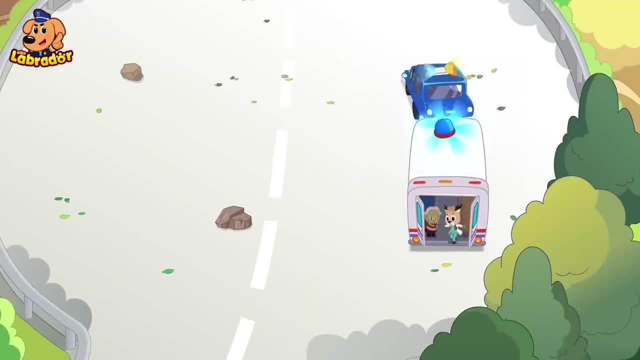 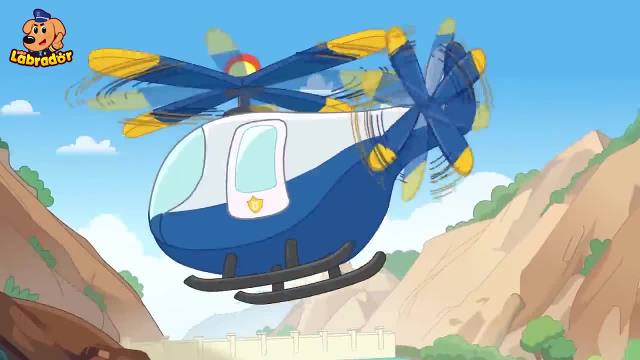 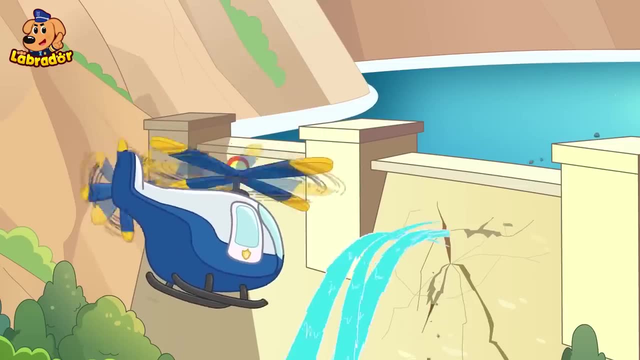 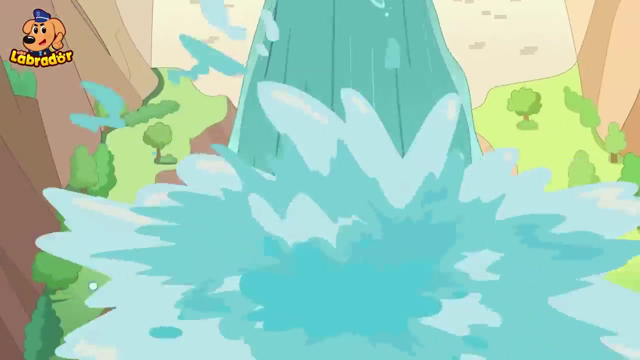 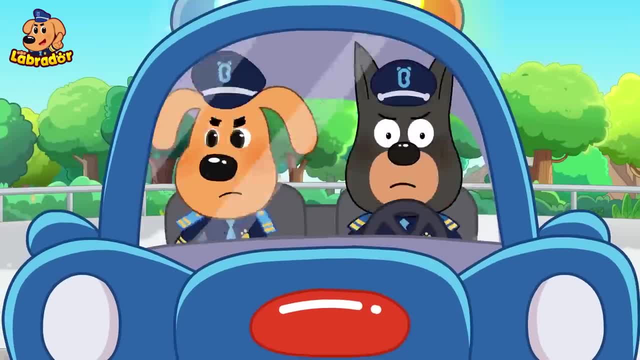 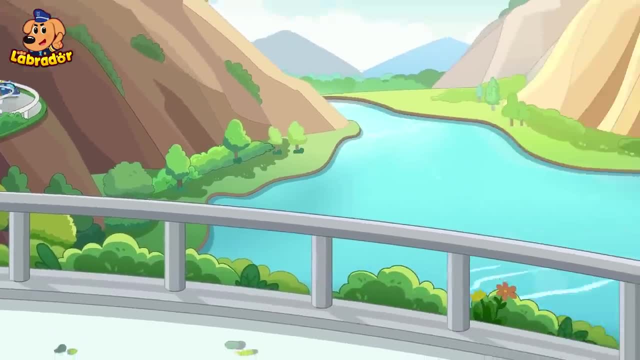 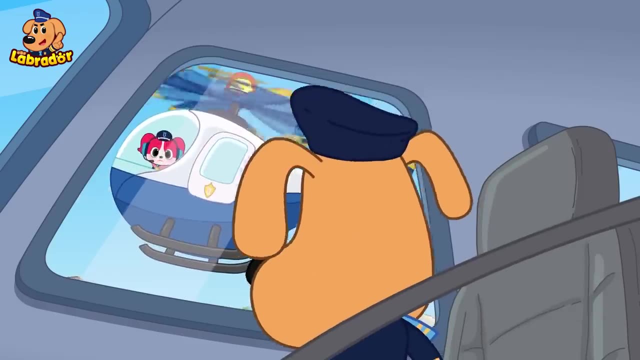 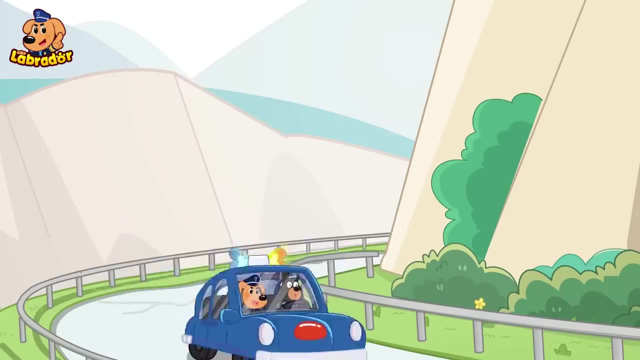 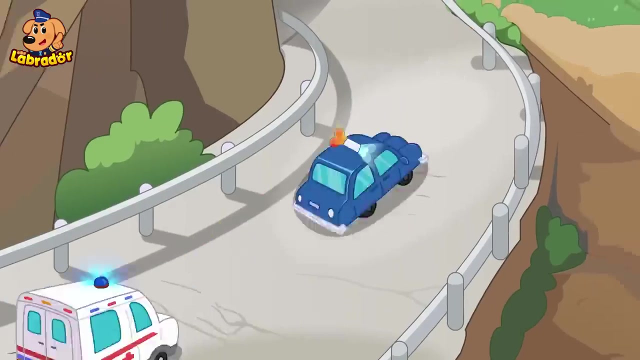 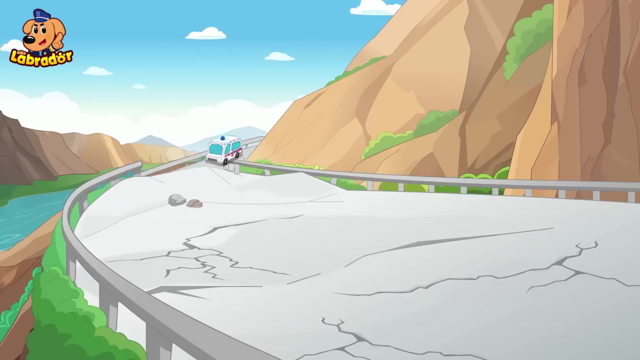 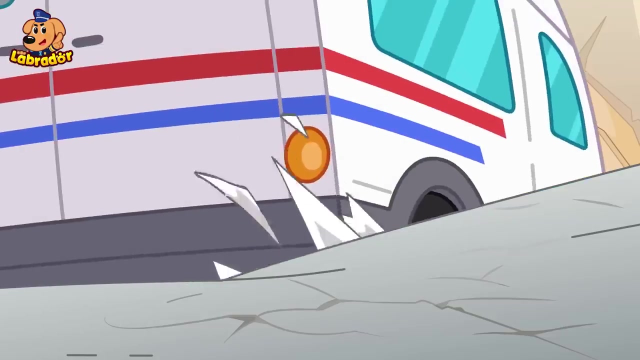 What Everyone get in the car. We're going to higher ground, Sheriff Labrador, the flood is coming. Oh no, We're blocked. Leave it to me Drive up the hill. Oh no, The wheels are stuck. Sheriff Labrador, the flood is coming. 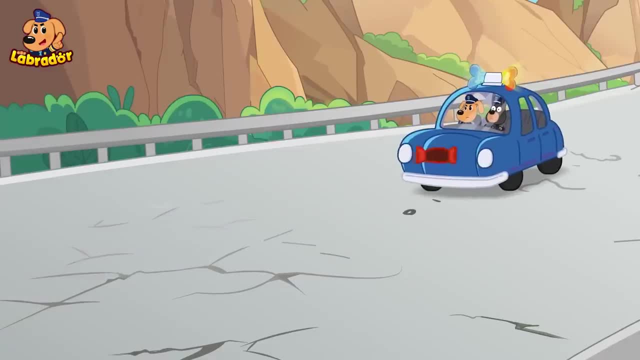 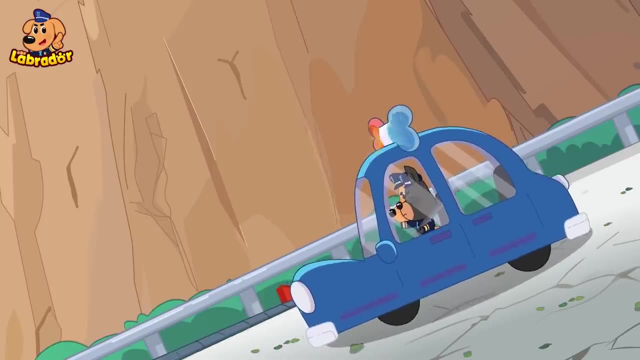 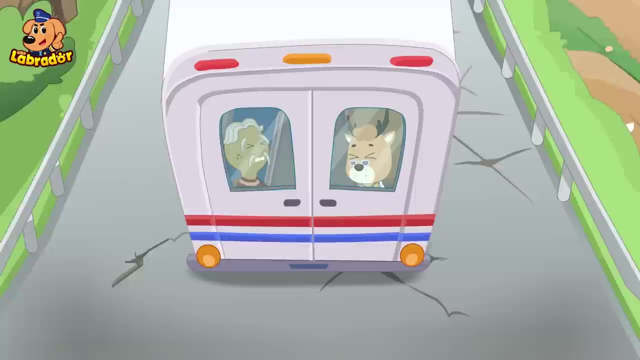 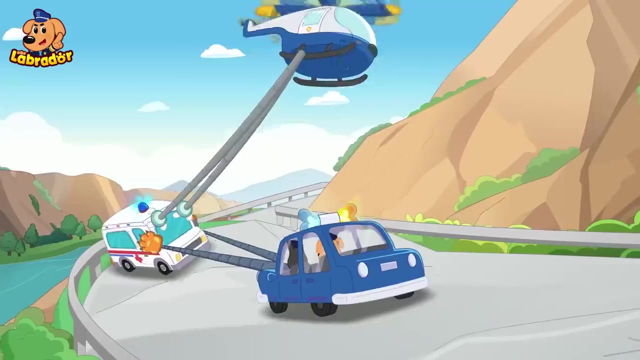 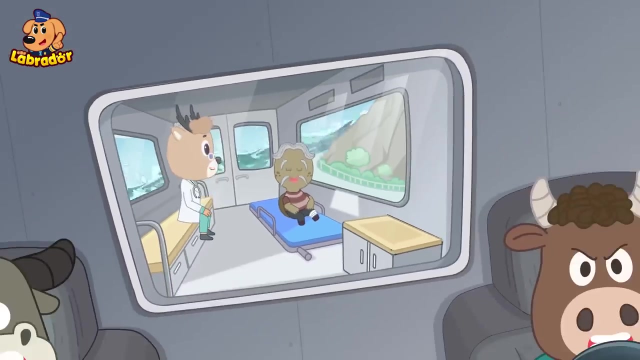 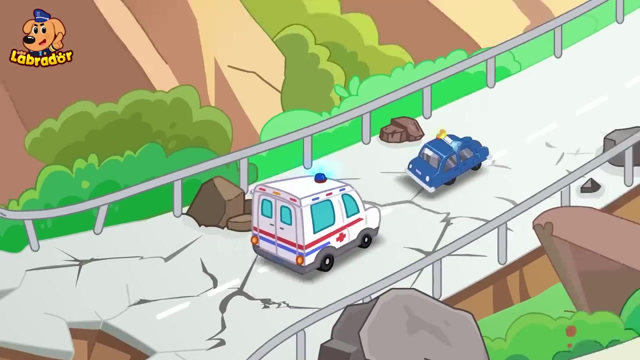 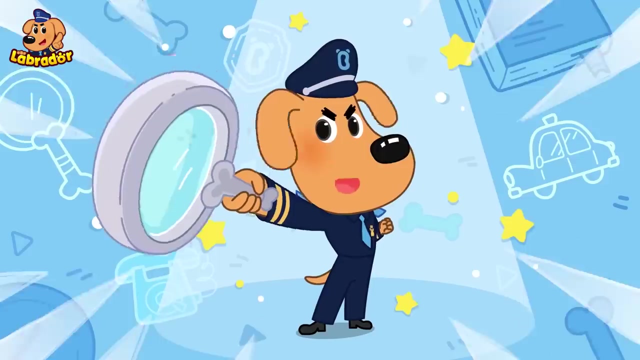 Use flying claws. Got it. Huh, Ah, Ah, Help, Ah, Hurry, Hurry. Phew, That was close, We're safe now. Let's go to the hospital now. Ahem, Sheriff Labrador, Sheriff Labrador. 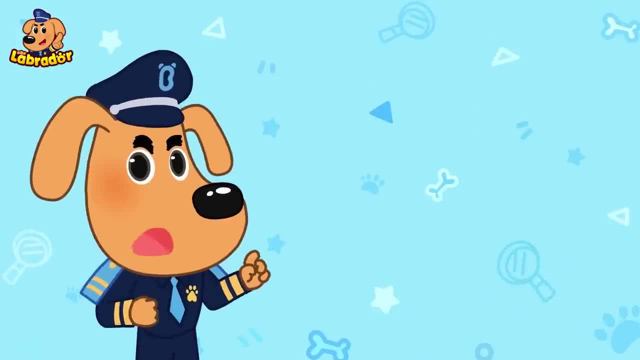 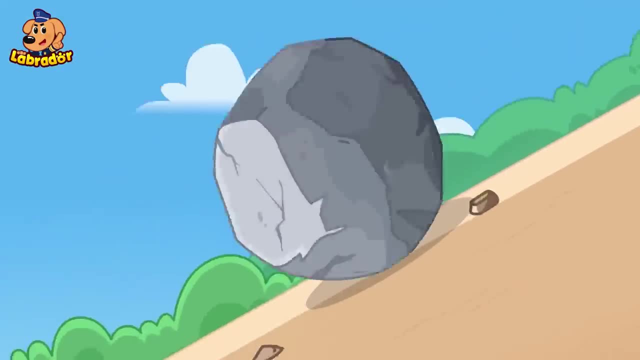 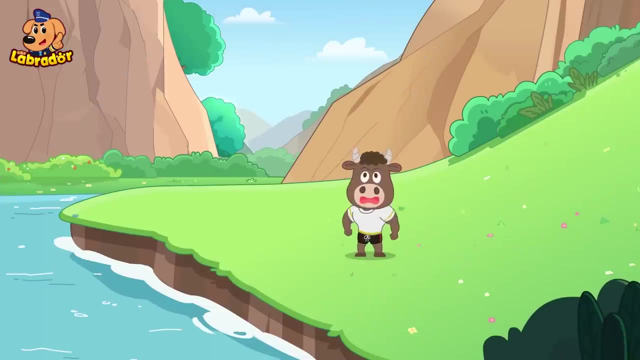 Your safety. talk Kids: if you experience an earthquake. when you're outside, stay away from slopes and cliffs and go to an open area. If you see a falling rock, you should run away from the direction where it's falling. Also, if you're near a river or lake, 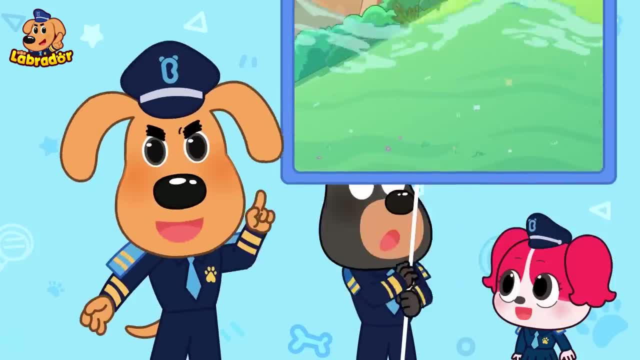 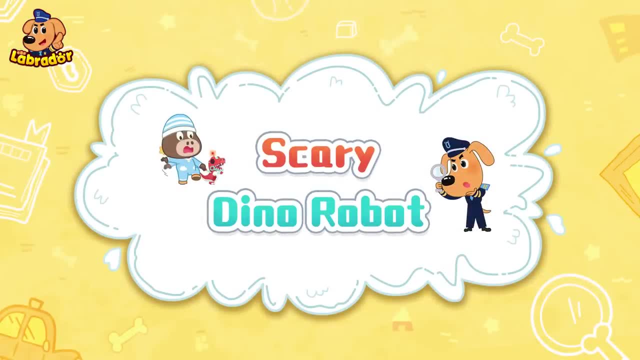 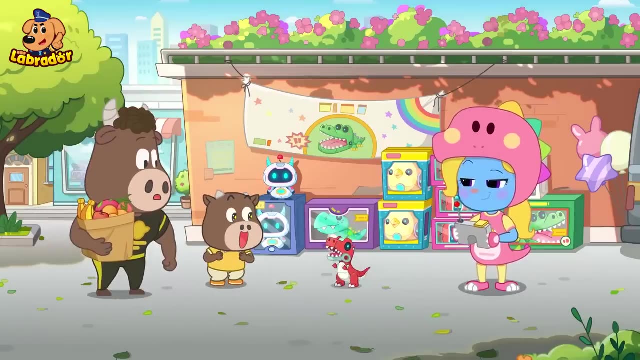 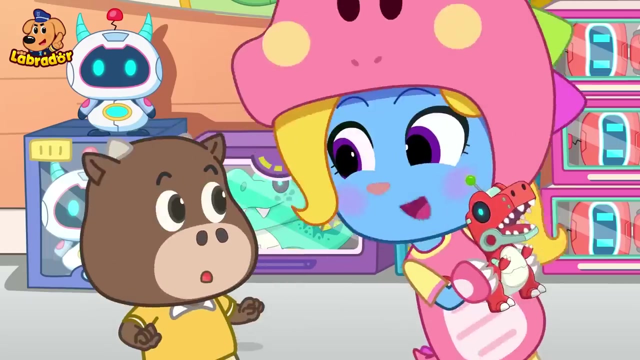 move to higher ground, where you will be safe from suddenly rising water. Please remember that Woof Scary dino robot. Whoa, It's so cool. Do you like it, little kid? Uh-huh, I do. I'll give it to you for free. 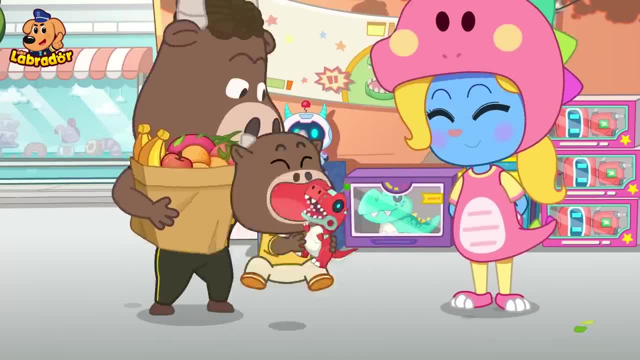 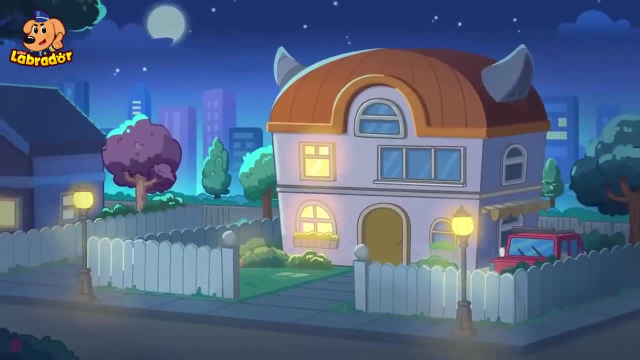 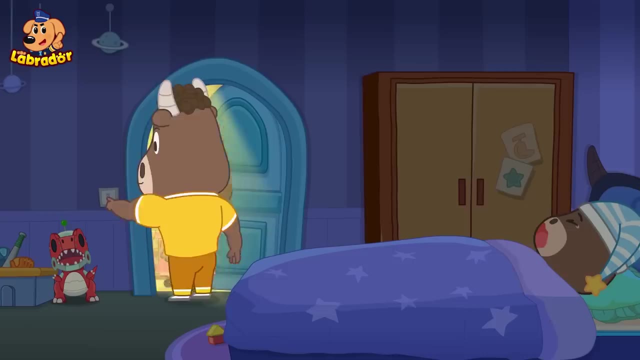 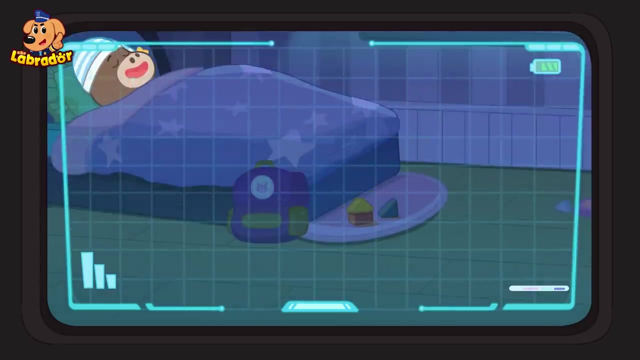 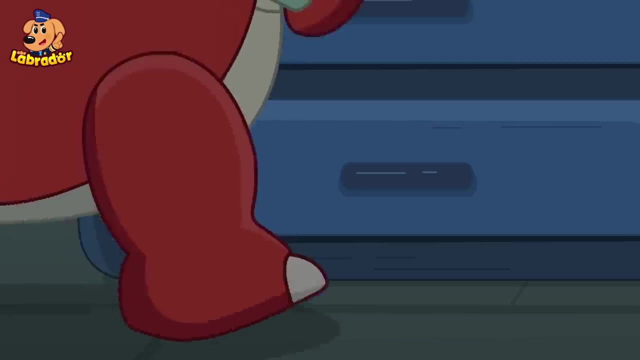 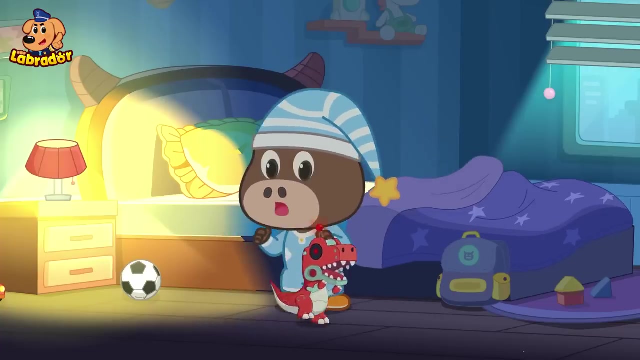 Huh, For free. That's right, For free. Wow, Thank you so much. Goodbye, Bye, Goodnight sweetie, Good night, Good night, Mommy and Daddy. Is it morning? T-Rex, Where are you going? 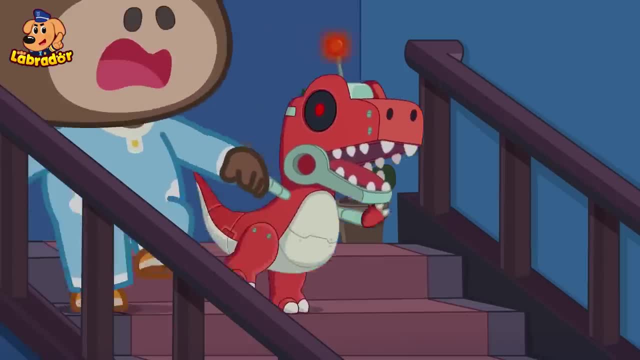 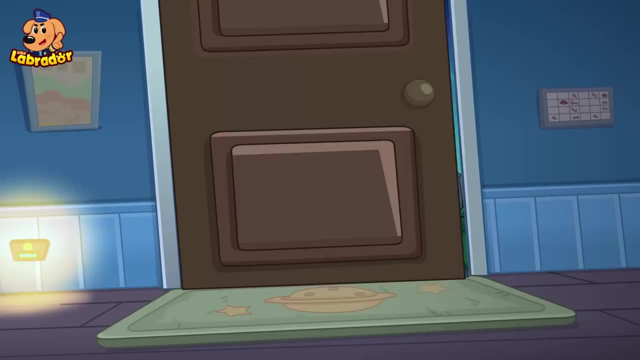 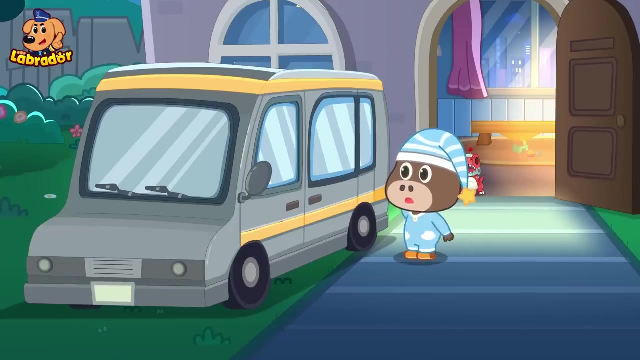 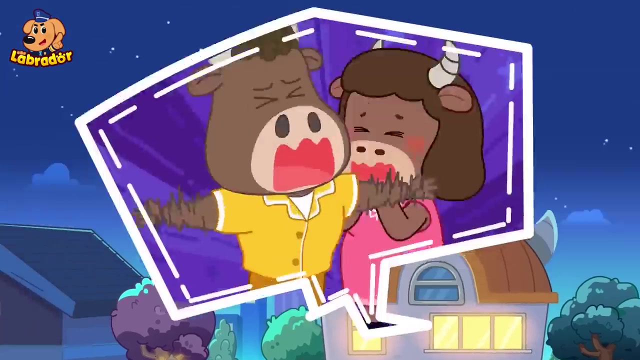 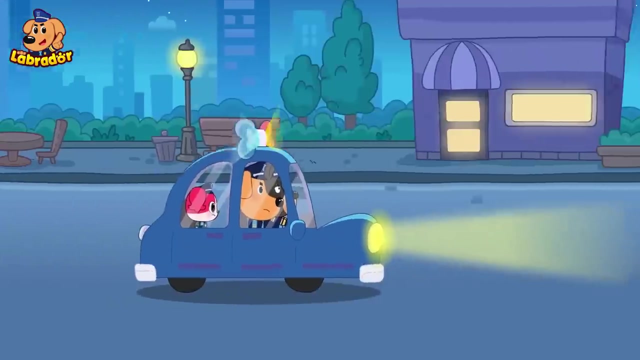 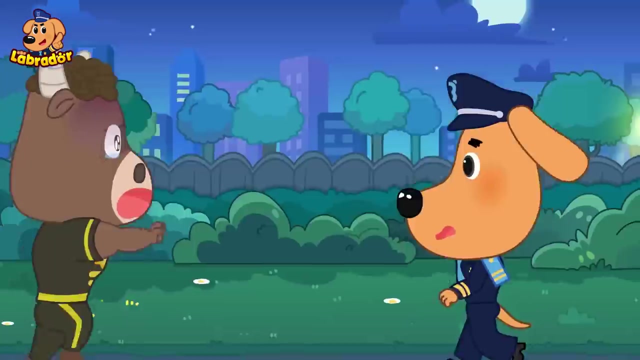 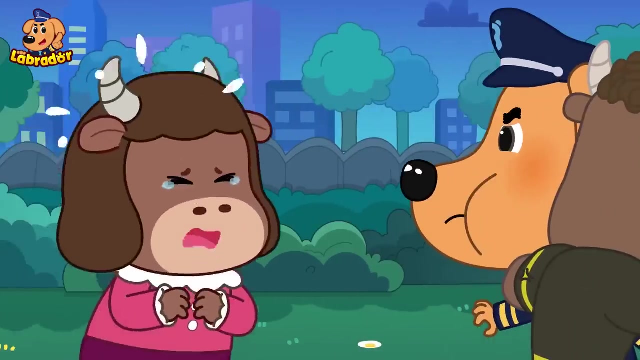 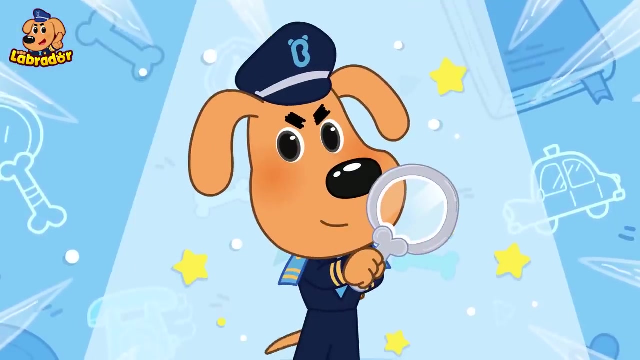 Mommy, Daddy, Where's our son? Where's Labrador? He woke up to the sound of a scream and our son was missing. Please help us. Don't worry, There's no case that I can't solve, Huh. 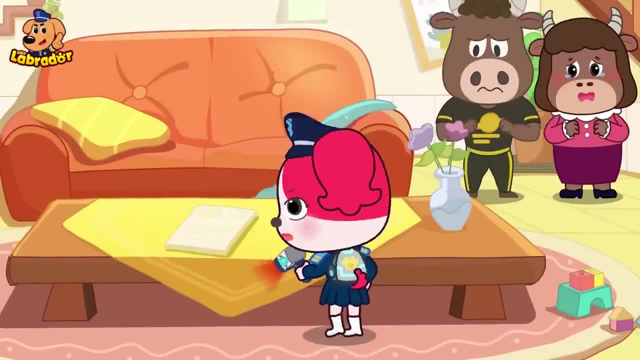 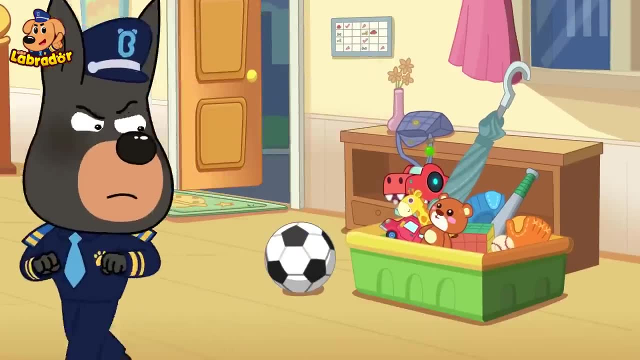 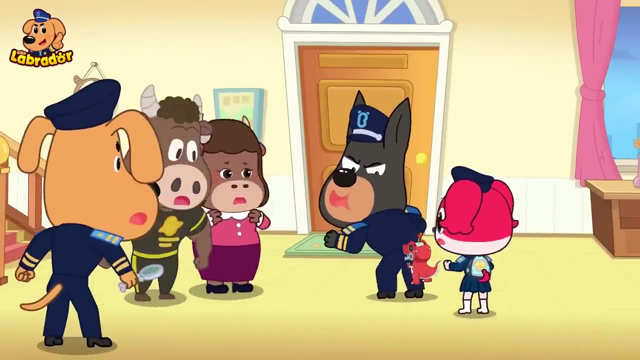 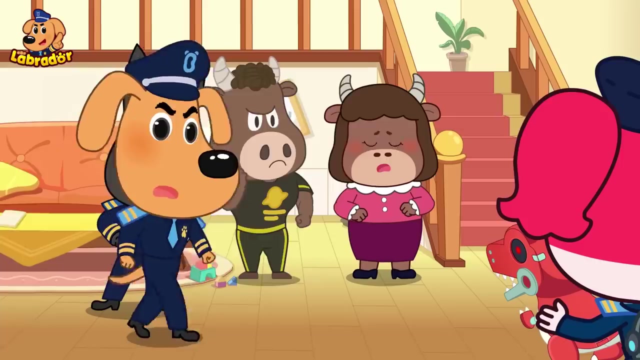 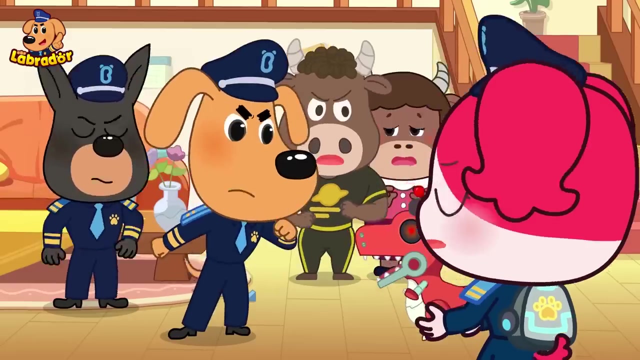 Hmm, Oh Ouch. Who bit my bottom? That hurts. This T-Rex looks so scary. We got it from a strange young lady for free. There must be something wrong with the T-Rex Papillon. check it right now. 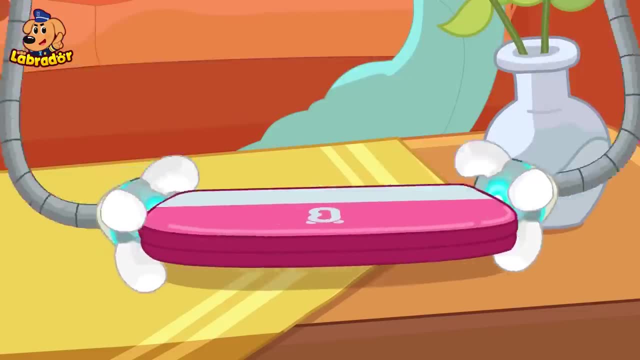 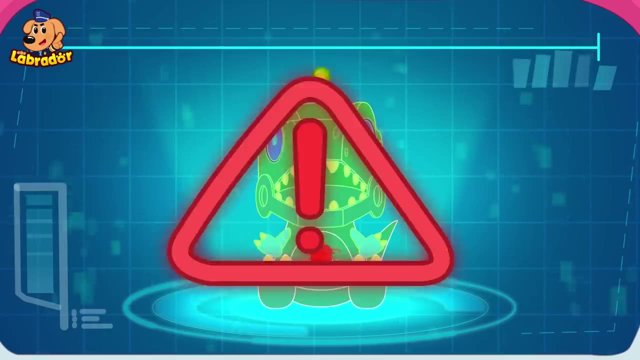 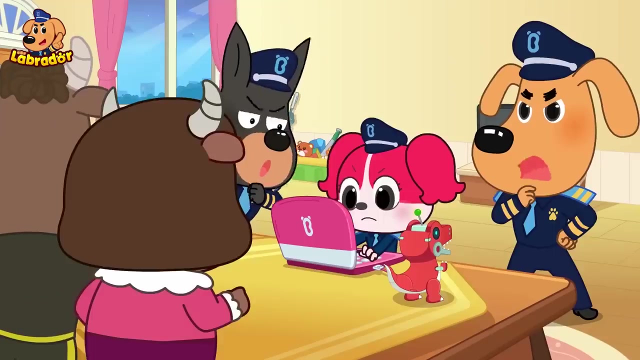 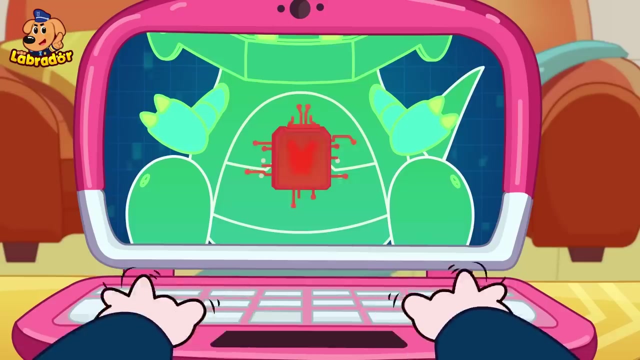 Got it. Here's the result: There's a remote-controlled chip inside the T-Rex. Looks like a bad person lured away Little Bison by a remote-controlled T-Rex. Huh, But what should we do? Huh, But what should we do? 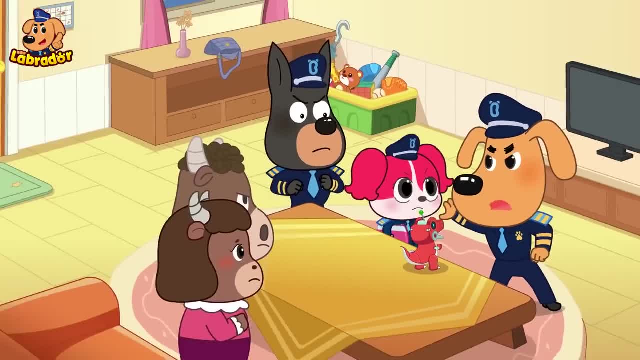 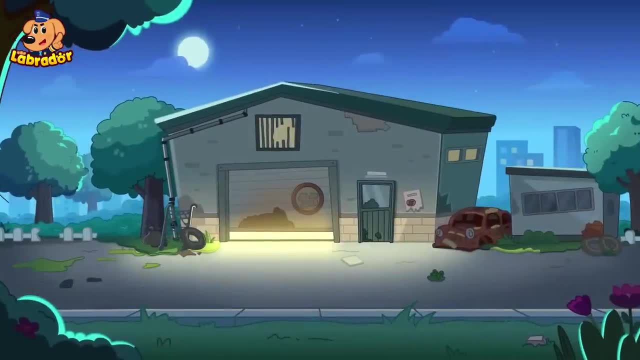 I've already located their position. I've already located their position. I've already located their position. Huh, Let's go save Little Bison. Ha, Let's go save Little Bison. I want to go home. I can't stand it anymore. 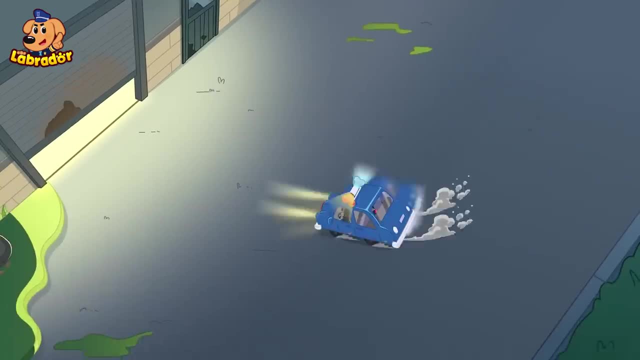 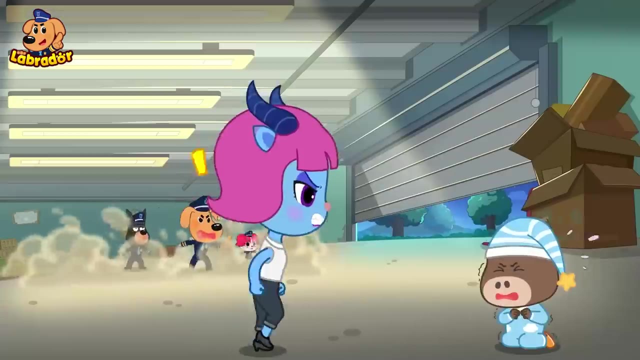 I can't stand it anymore. It's Little Bison's voice. It's Little Bison's voice, Hurry, Hey, Stop, Hey, Stop, Hey, Stop. How did they find me here? Hey, Hey, Hey need help. 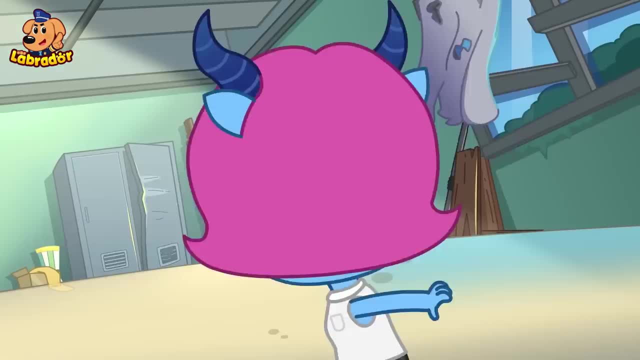 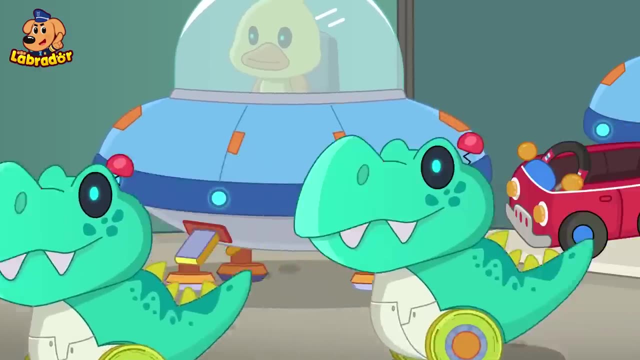 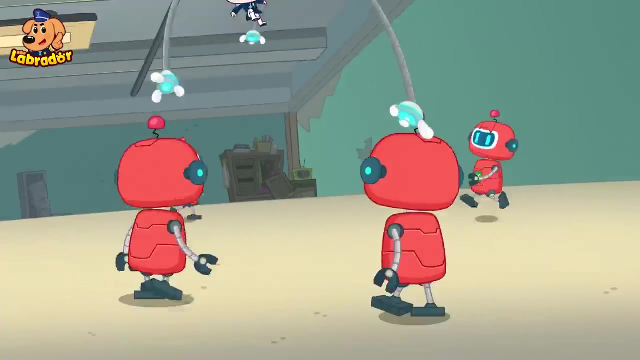 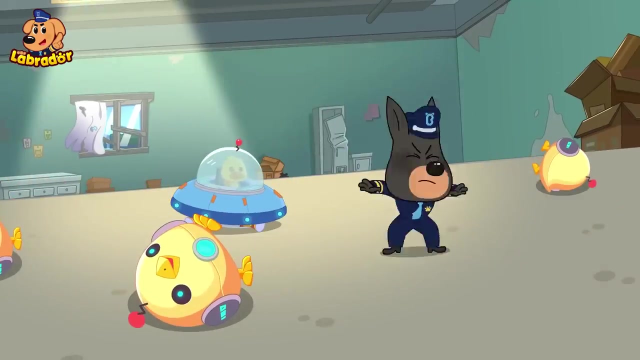 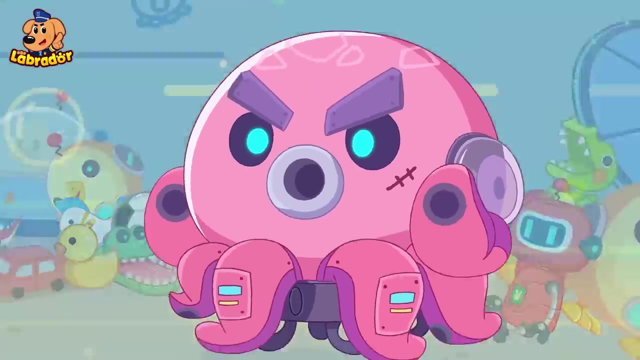 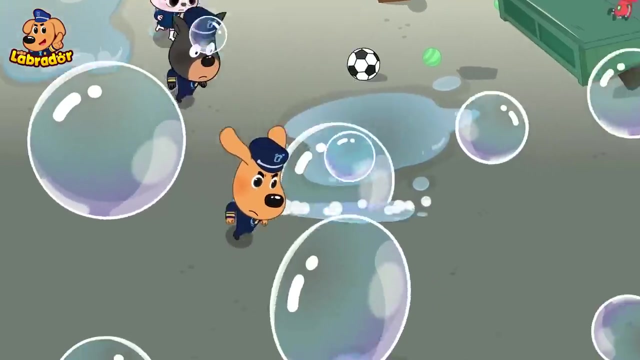 How did they find me here? How did they find me here, Huh, What do I do? Huh, I have a plan. Watch me. Oh, take a look at this. Huh, It's so slippery, Huh. 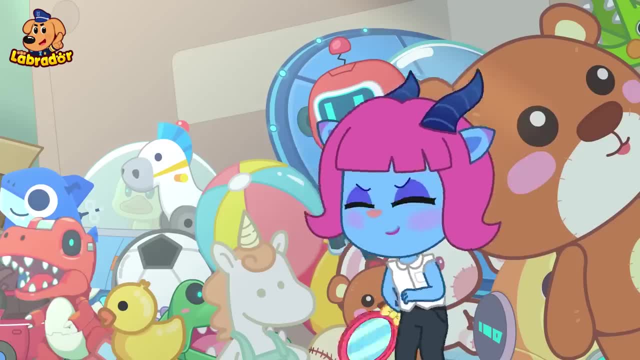 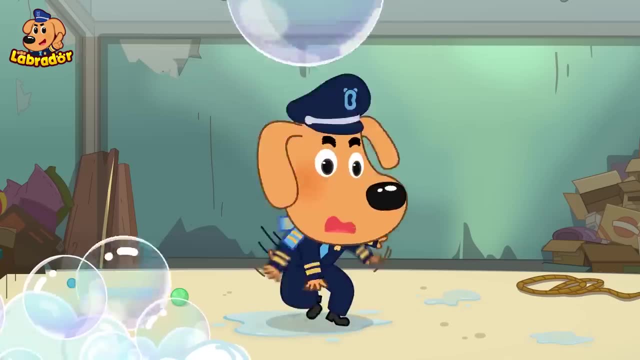 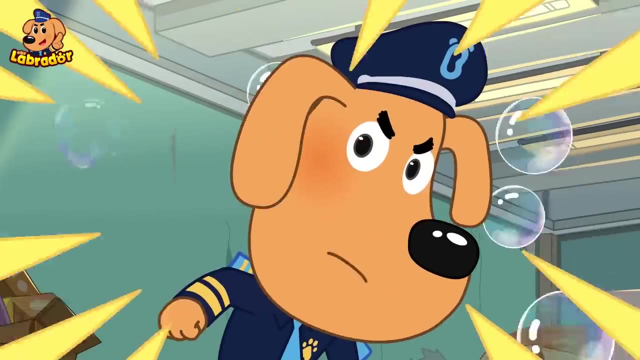 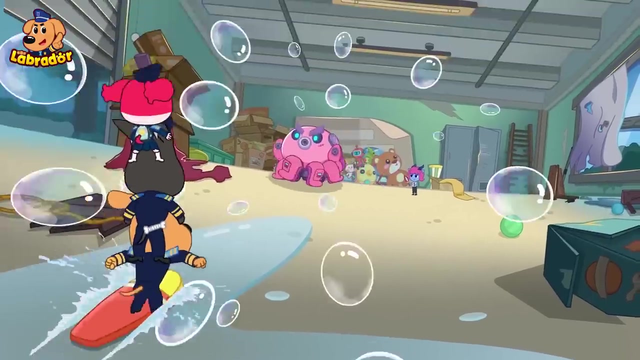 Oh, Ah-ha-ha-ha, Aren't my toys amazing, Oh easy, Ah, Huh, Huh. Hey, Joby, Papillon, Huh Coming. Hey, Yeah, Huh, Hmm, Whoa, Oh no. 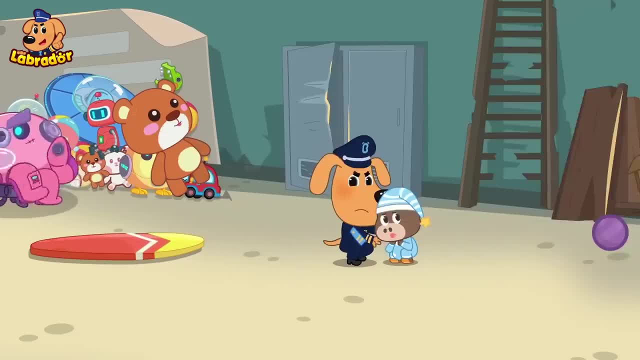 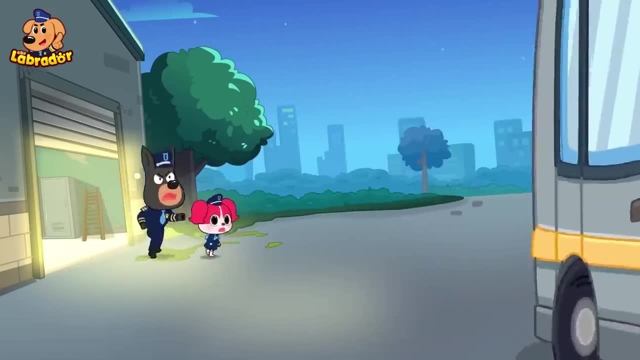 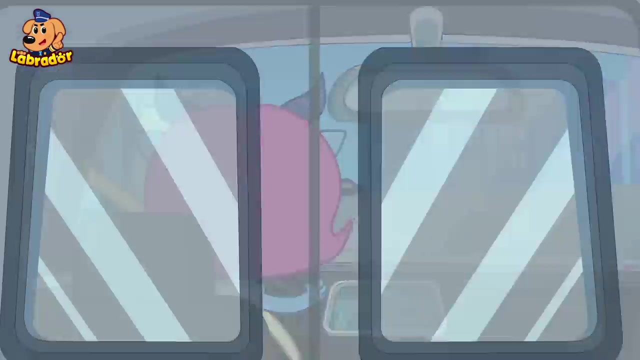 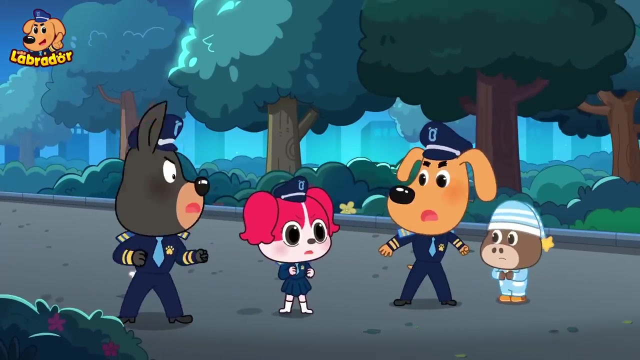 Ha-ha, Sheriff Labrador, Stop right there, Heading to the end of the Earth, Good-bye. Oh no, She escaped again. Don't worry, I've already hacked into her car control system. Huh, Let me give her a surprise. 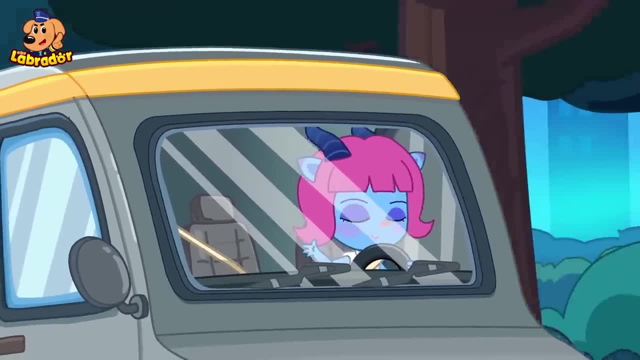 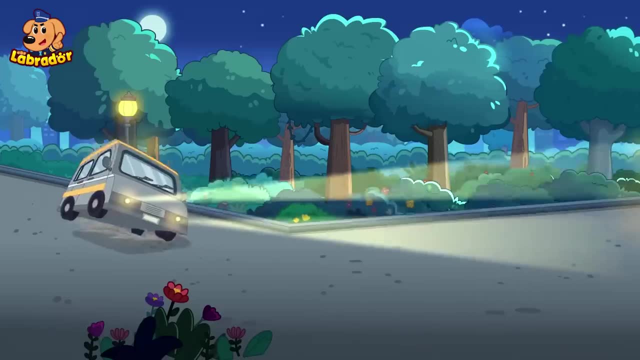 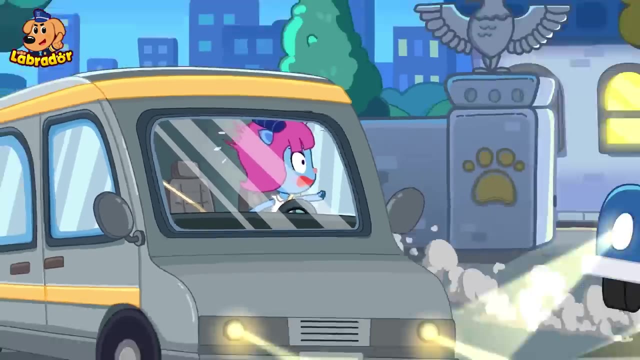 Hey, You'll never catch Dr Antel Boss Now heading to the police station. Uh-oh, What's going on? Oh, I failed again. Uh-oh, Oh, I failed again. Hmm, Antel, you're under arrest. 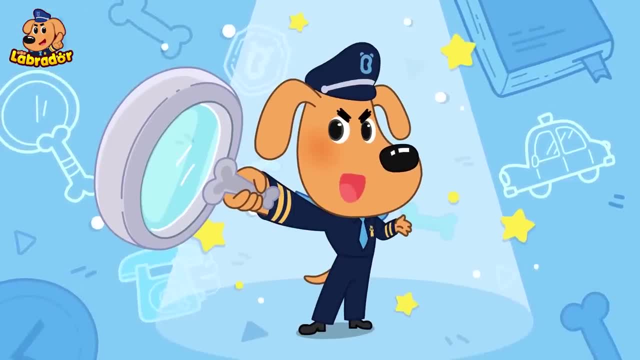 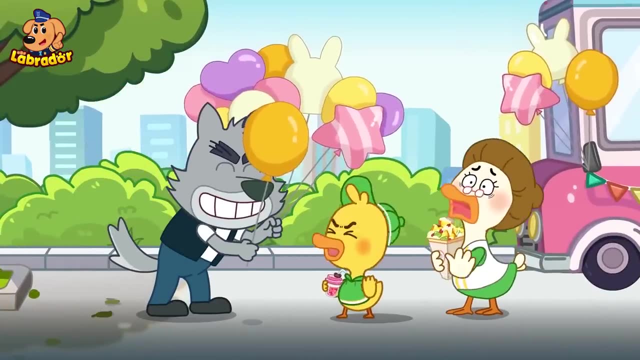 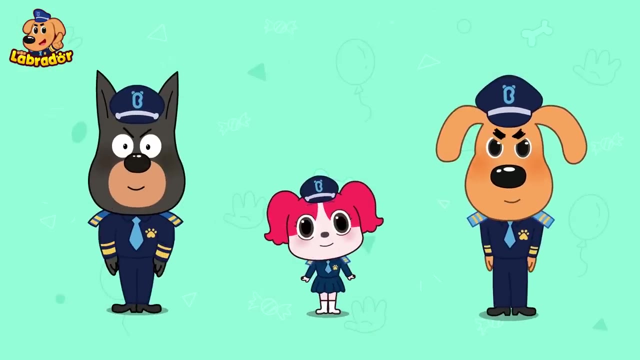 Sheriff Labrador's Safety Talk. Kids, you shouldn't take anything from strangers. There might be something dangerous in those things, so you should be careful. Can you remember that? Woof, Woof, Woof, Woof- Dangerous Calls. 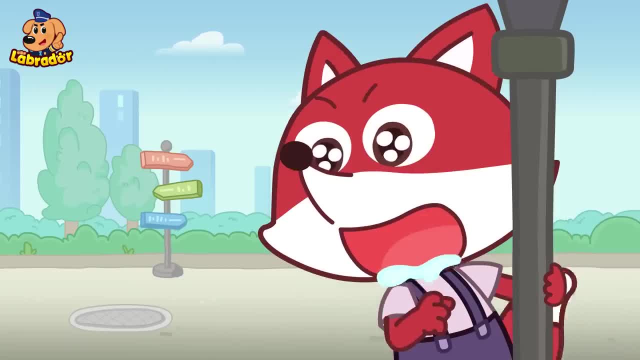 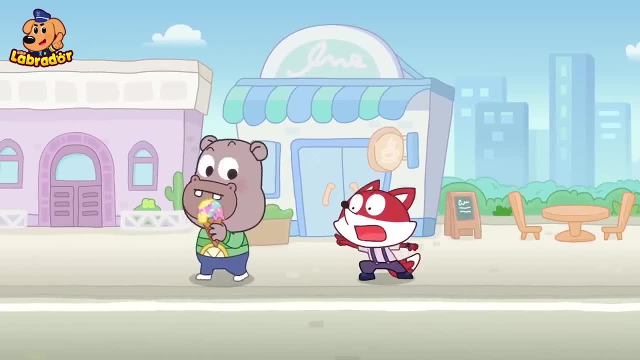 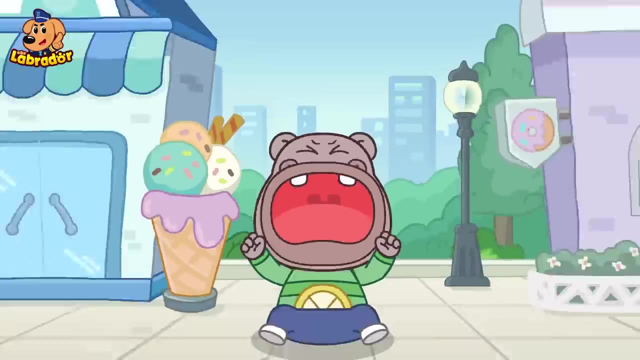 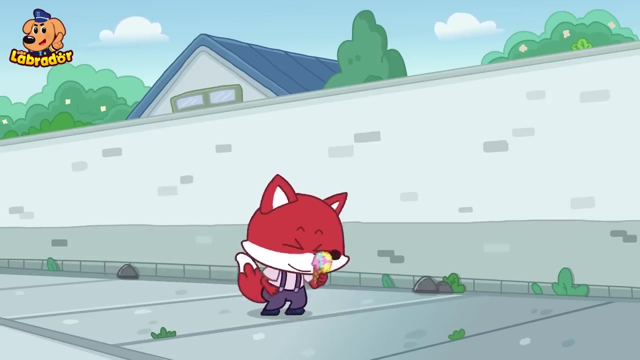 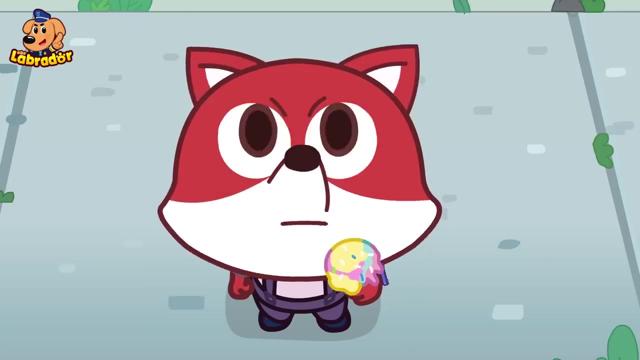 Huh, Huh, Wow. Oh look, It's a YOLO. Huh Oh, My ice cream Whoa. Huh Oh. Hmm, Fugitive Brown Bear. Call the police immediately if you see him. 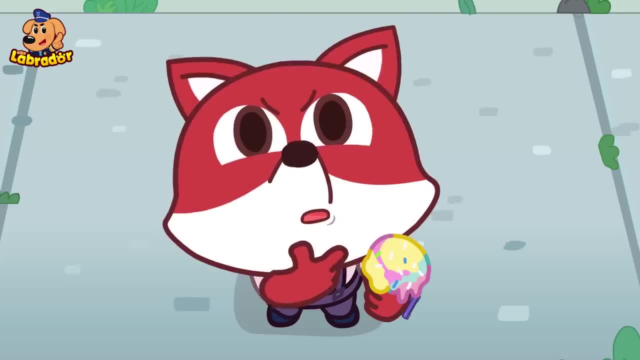 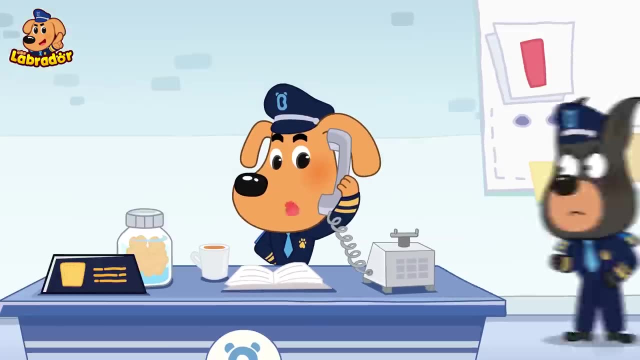 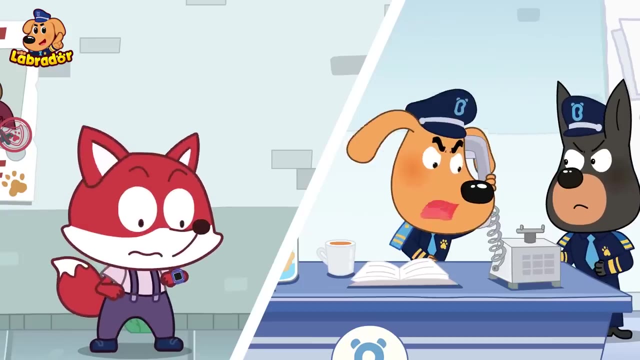 Hmm, Hey, Woof, Hi, I'm Sheriff Labrador. Sheriff Labrador, I saw Brown Bear, the fugitive. What? Where is he now? He's hiding at 10 Rose Road. Protect yourself. I'm going to call the police. 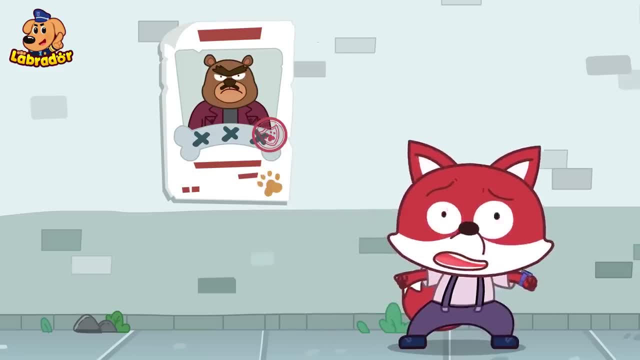 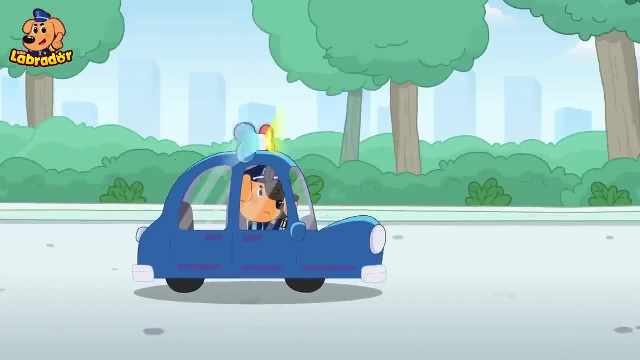 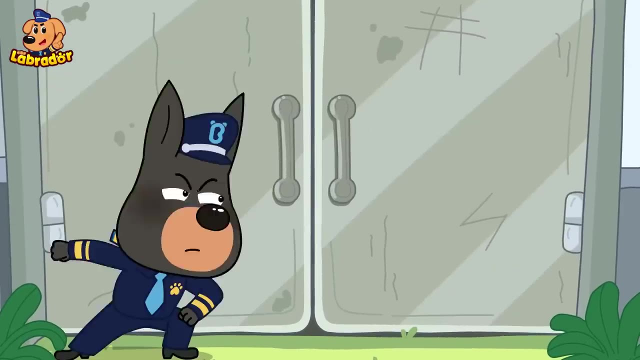 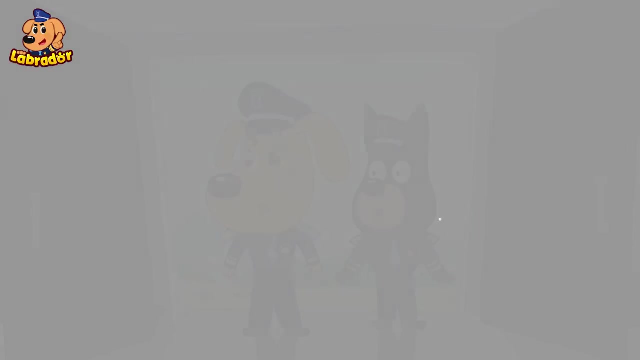 I'm going to call the police. Woof, Protect yourself and stay safe. We'll be right there. Uh-huh, Shh, Huh, Huh, Oh, Ah-choo. Yeah, It's full of dust here. 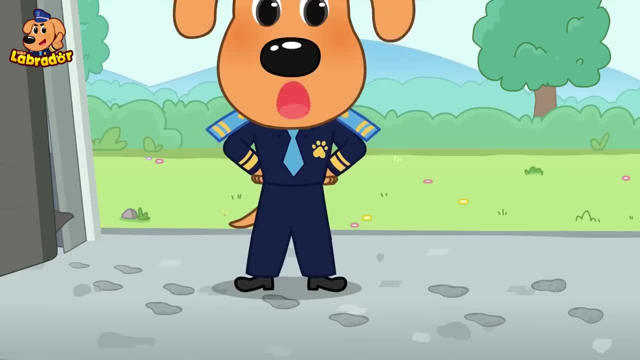 And there aren't any footprints. This place has been unoccupied for a very long time. Would it be that…? Sheriff Labrador Brown Bear is coming after me. I'm hiding right by the bee hives. Ah, Ah, Ah. 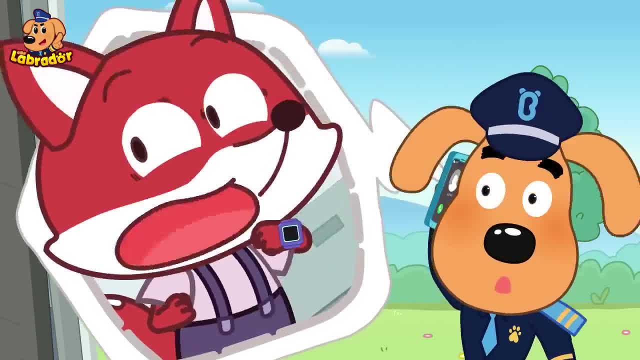 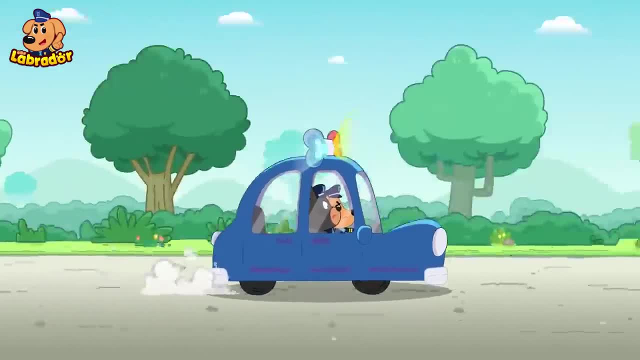 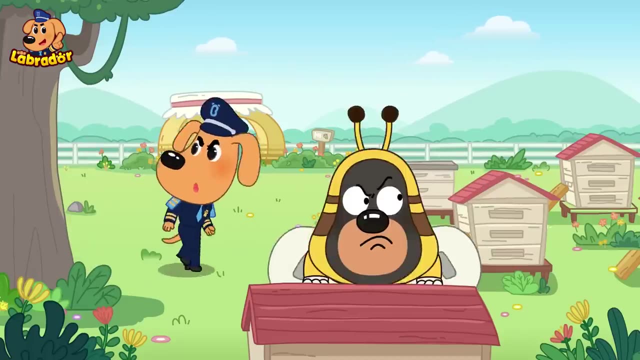 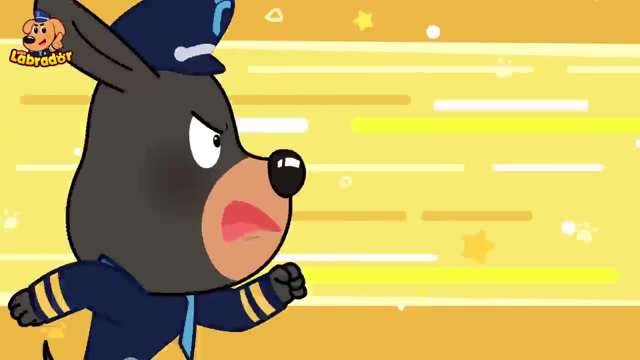 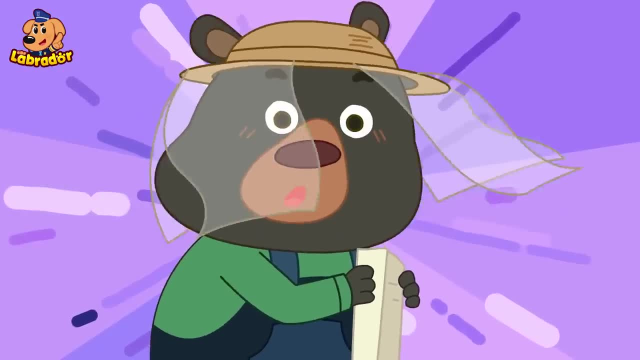 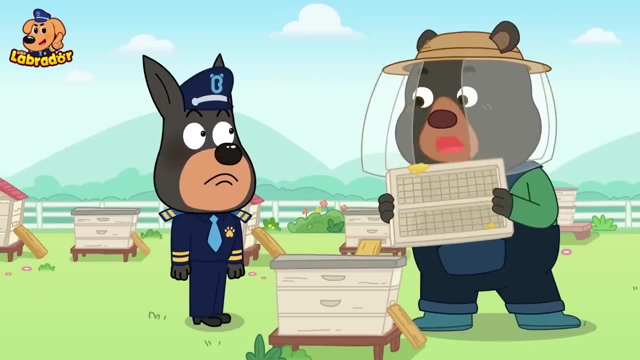 Ah-heh, Huh, Ah-huh, Ah. It's not Brown Bear, It's Mr Black Bear. Is there something wrong, Officer? Uh, ha-ha, I am just here to buy some honey, Ha-ha-ha. 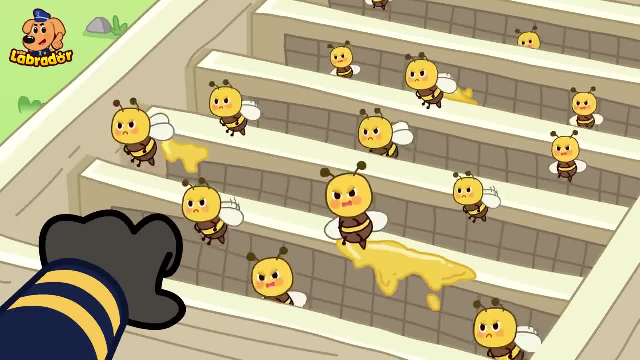 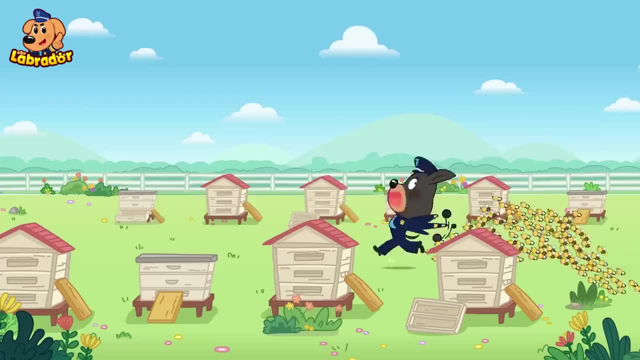 Ooh Huh, Ah-ah Ah Ow ow ow Ah, Ah, Ah Ah Ow ow Oh, Ow ow ow Ow Oh Ha, ha, ha, Ha, ha ha. 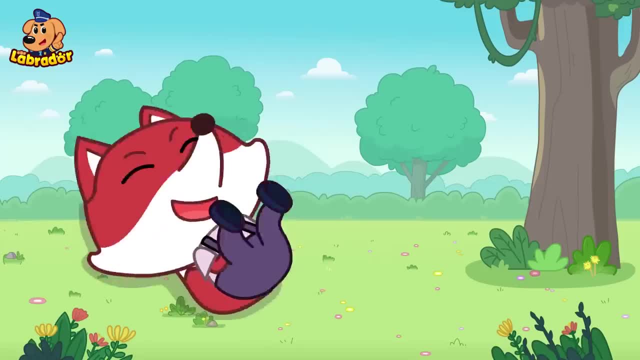 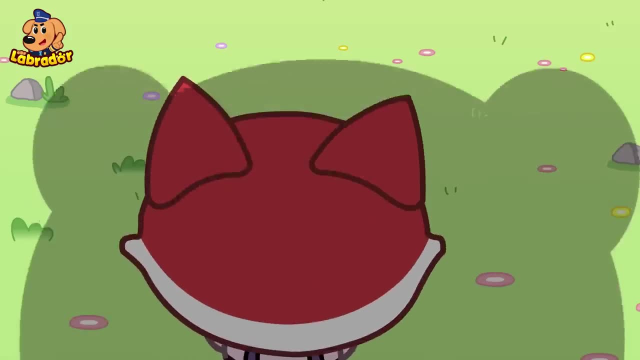 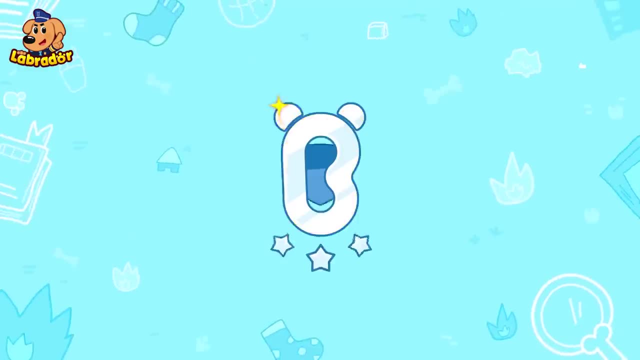 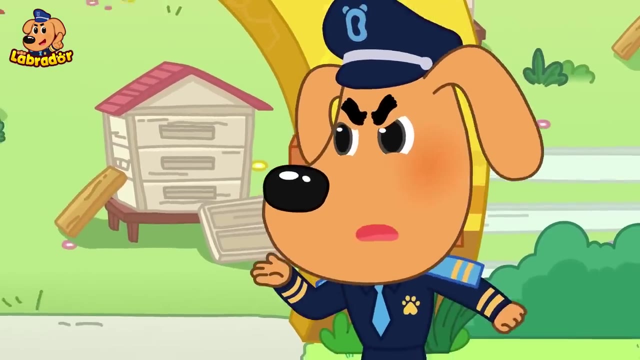 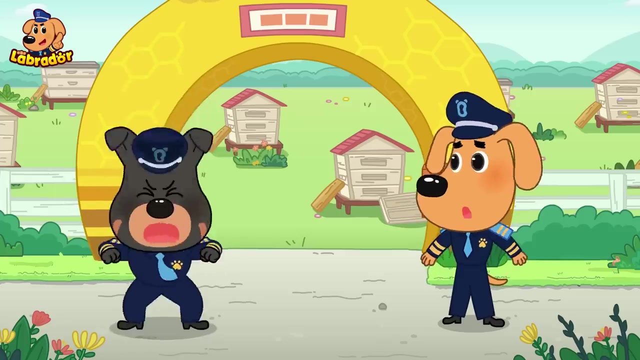 B-B-Brown Bear. Hmm, looking at the two prank calls, I'm sure Little Fox did them just for fun. Uh, What Little Fox Prank calls? Ha Ow, Huh, Help me, Sheriff Labrador Brown Bear has kidnapped me. 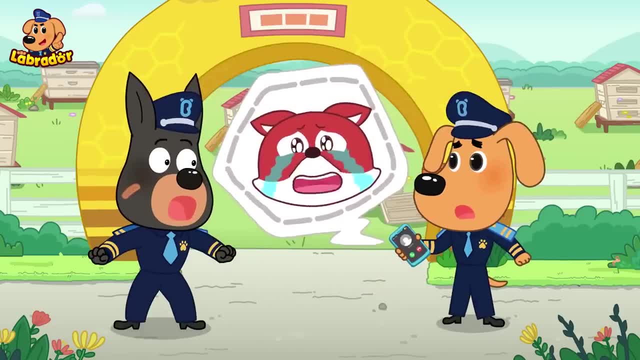 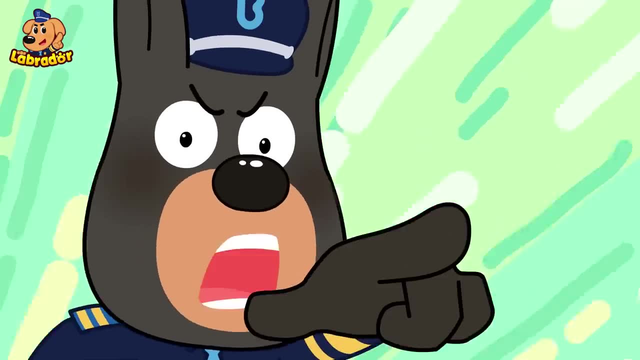 Liar. You're lying again. Please help me. This is not a lie. Don't you know that they can fall on their own? Huh, Huh, Huh, Huh, Huh, Huh, Oh no. 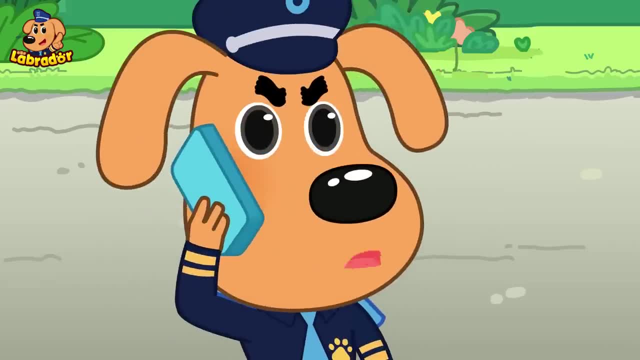 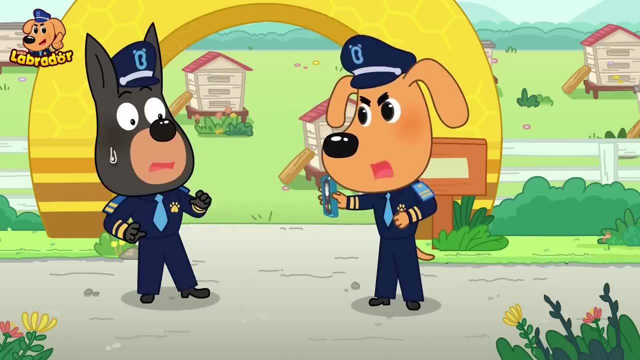 Most police calls. He's against the law. No, I think Little Fox isn't lying. Uh, Listen to the echoes and the sound of the engine. He might be trapped in a car right now. Uh, Brown Bear, Ha ha ha. 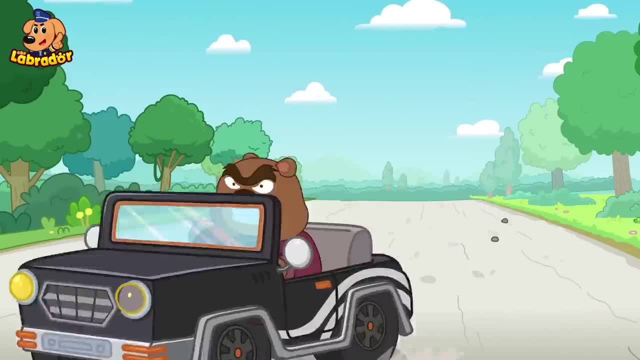 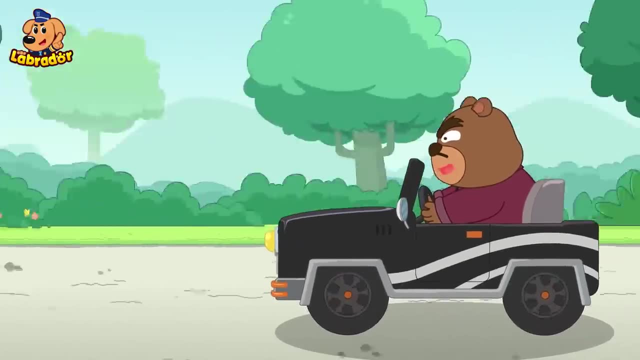 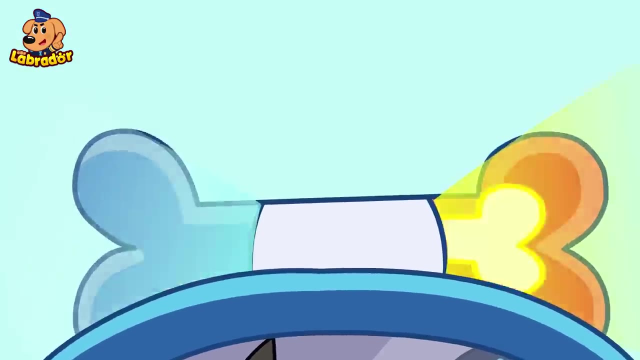 Brown Bear. Ba-ba-da, I'm Brown Bear, Everybody's scared of me. Yeah, Uh, Follow him. Uh, Uh, Oh, Uh, What the Uh, What the hell? Ah, What the? Oh Brown Bear, Stop the car. Stop the car now. 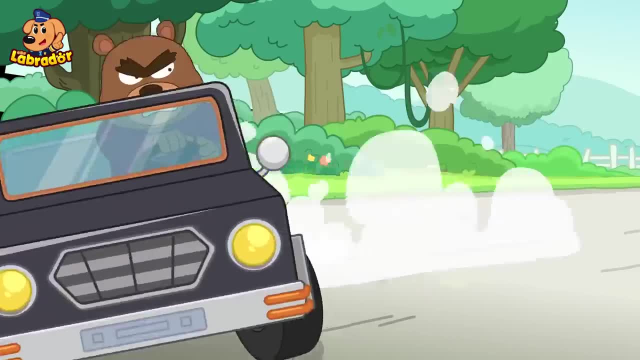 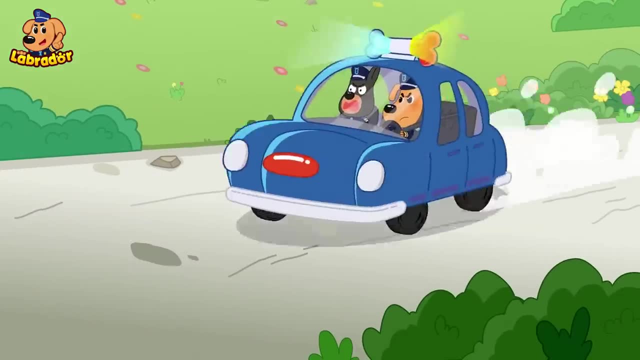 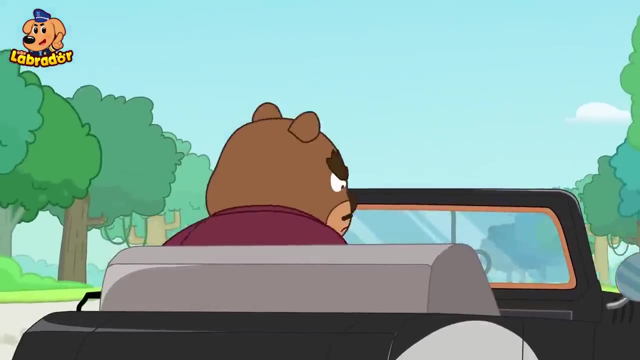 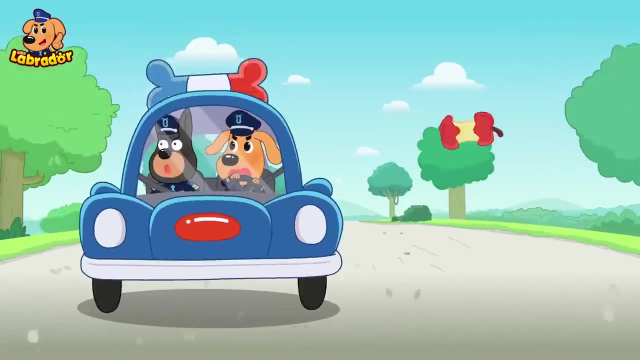 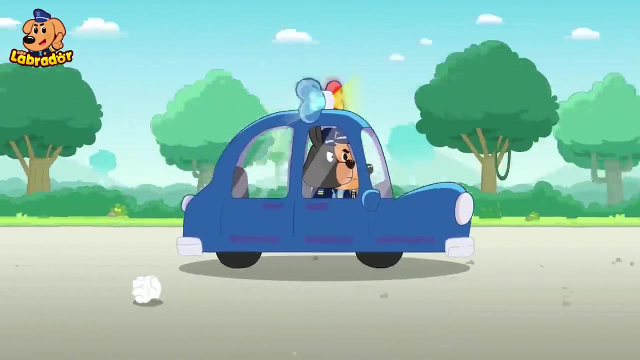 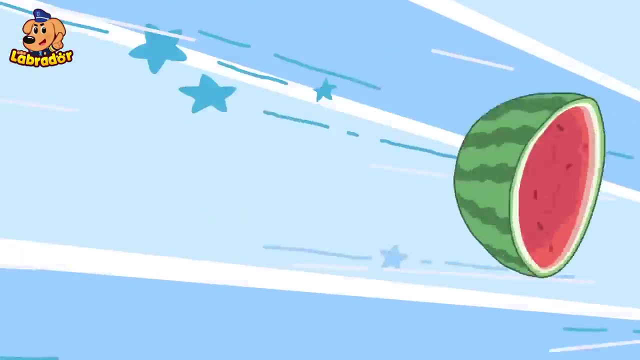 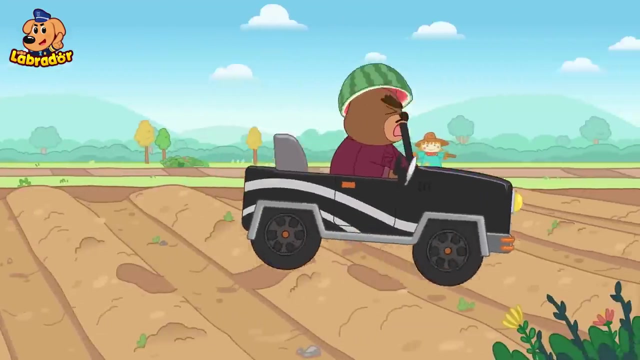 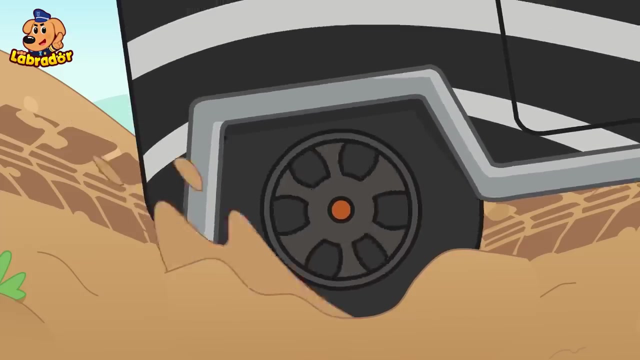 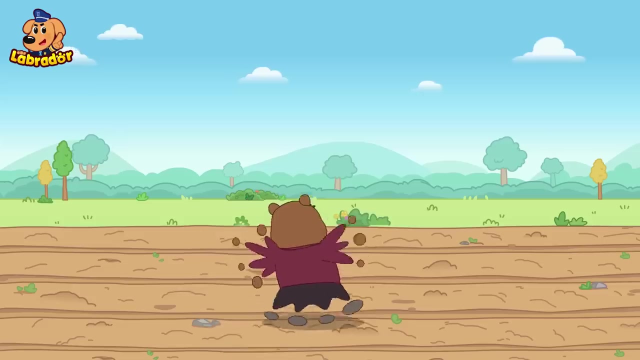 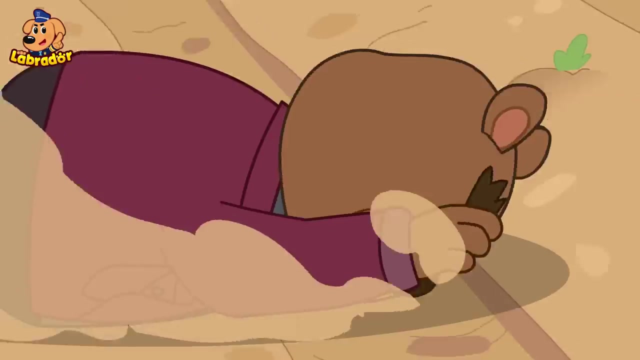 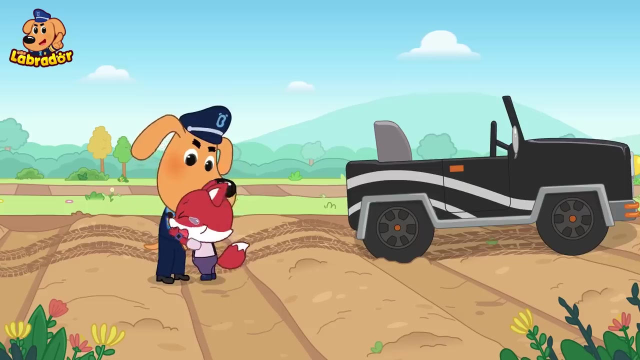 Huh, Police, They're so annoying. Let me show you what I can do. Oh no, They're right behind me. I need to run. Stop right there. Huh, You can't run away from us. I was so scared. 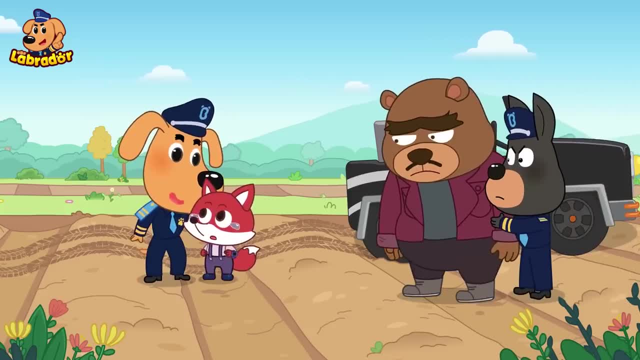 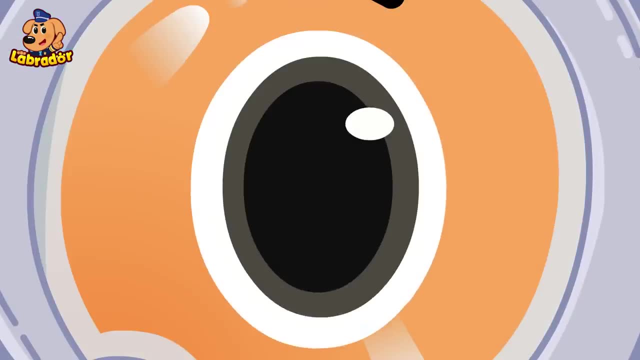 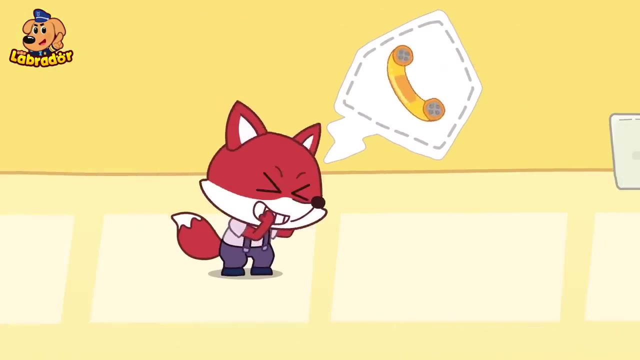 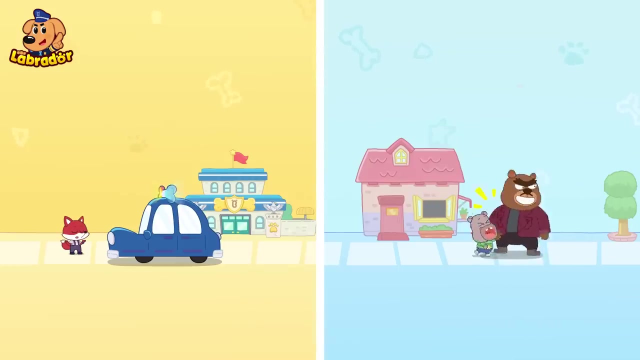 It's okay, You're safe now. But remember you shouldn't make false police calls for fun. But I'm I'm so sorry Sheriff Labrador's Safety Talk. Making false police calls are against the law. It leads police to wrong places so people in need can't get help. 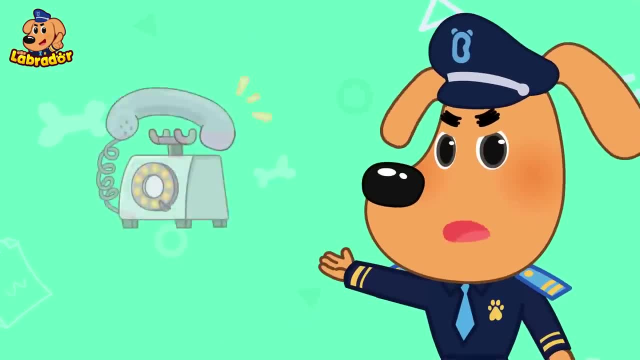 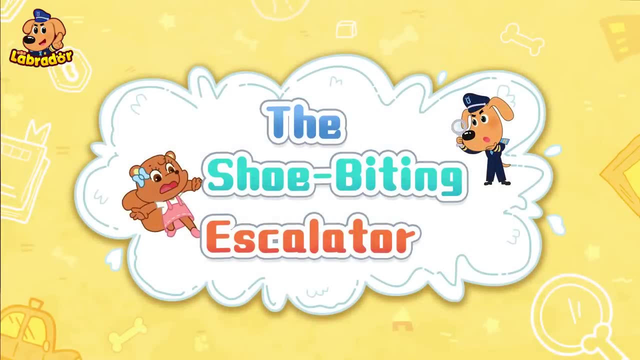 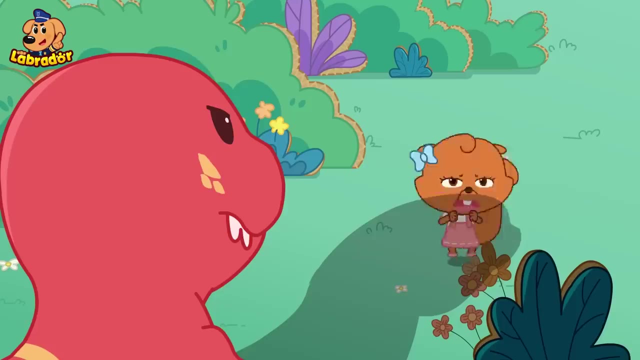 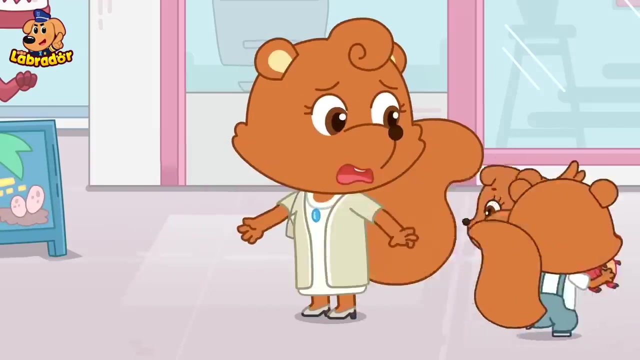 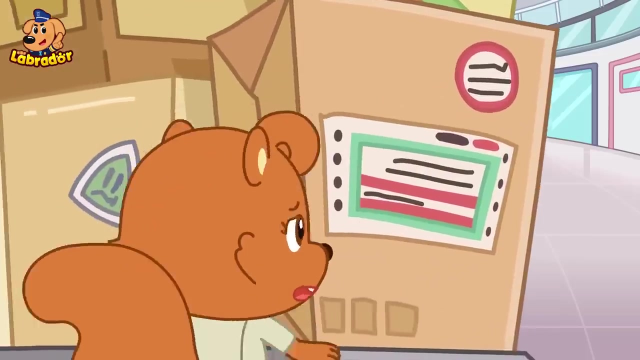 Kids, please call the police only when you're actually in danger. Never make false police calls just for fun. Woof, Woof, The shoe biting Escalator, The shoe biting Kids. be careful, Look, Look, Look. 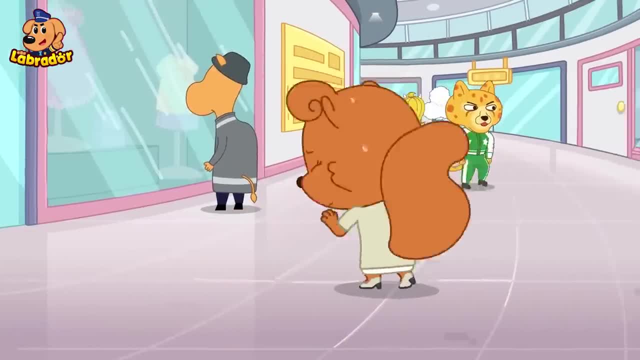 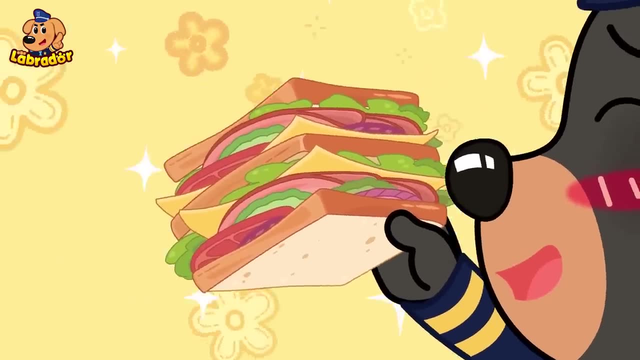 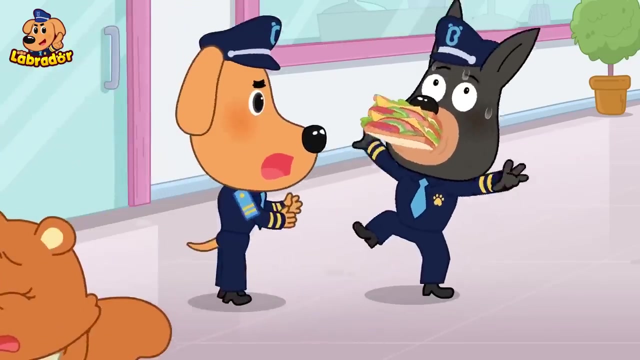 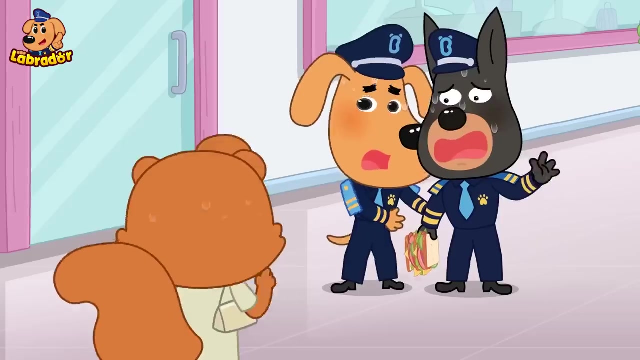 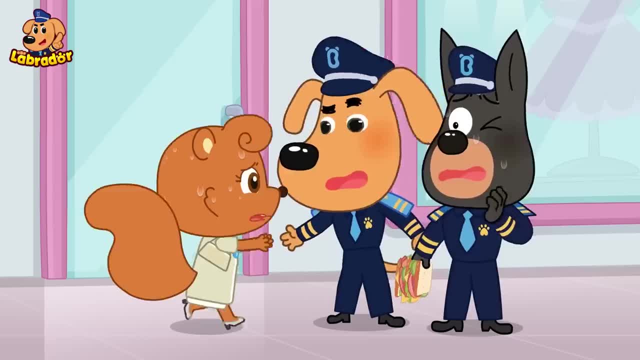 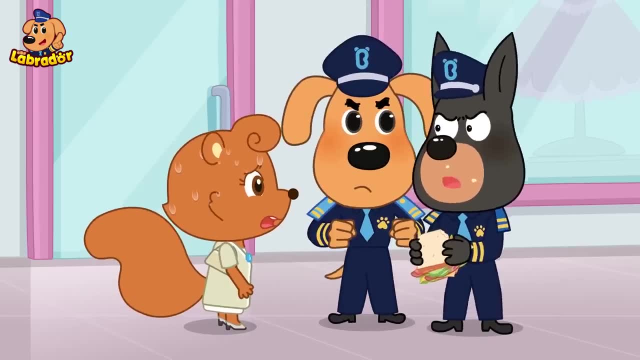 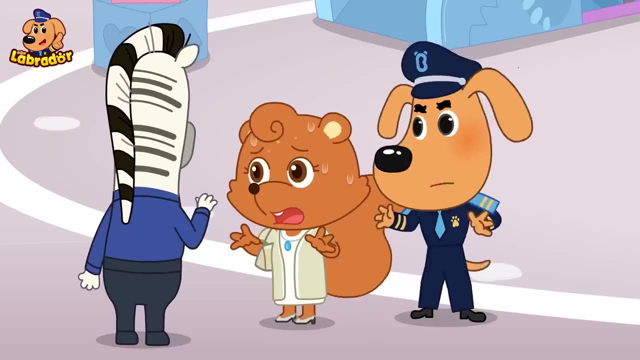 Are you alright, Ms Squirrel? Are you in a rush? Sheriff Labrador, my children are missing. Please help me find them. We're on it. Excuse me, have you seen two little squirrels around About this tall? 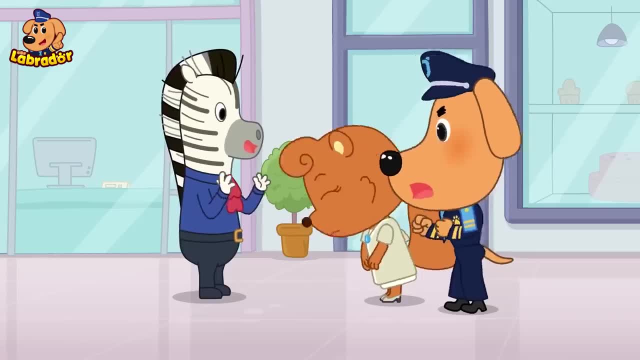 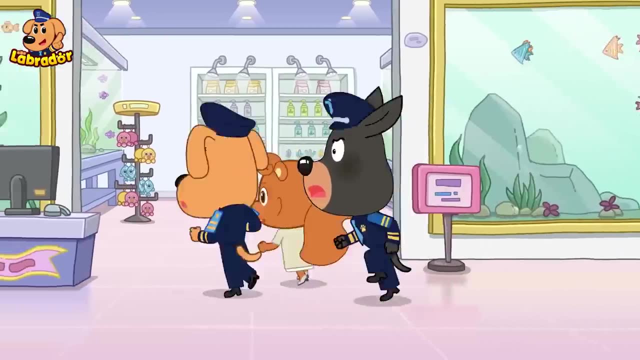 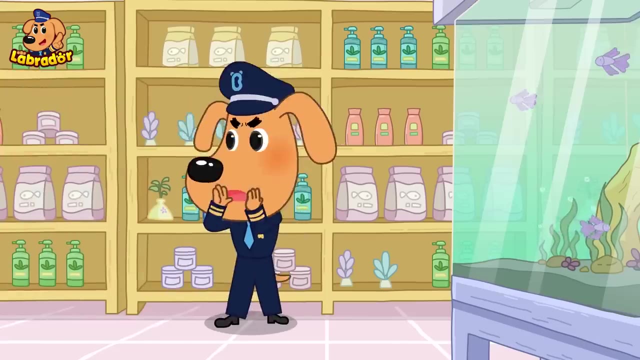 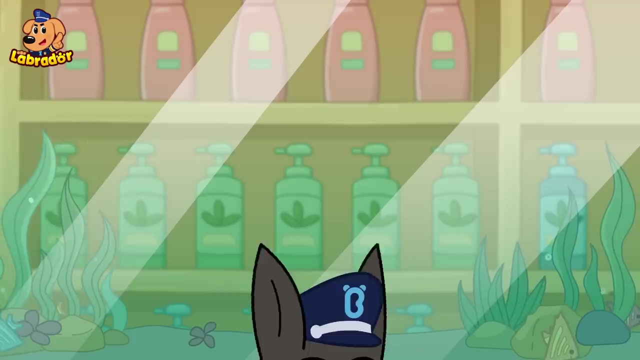 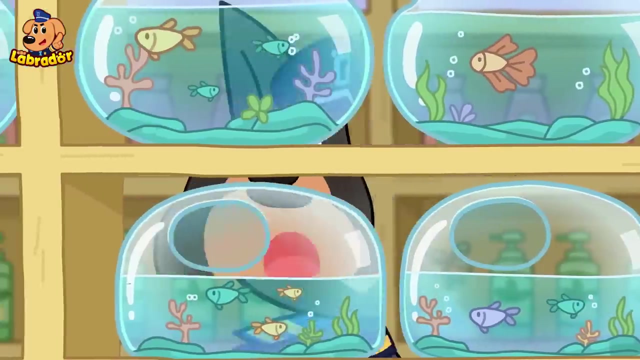 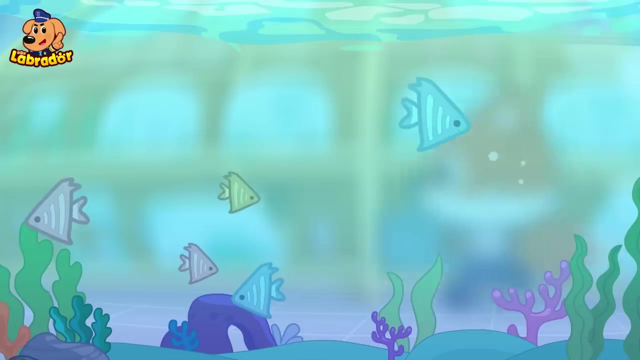 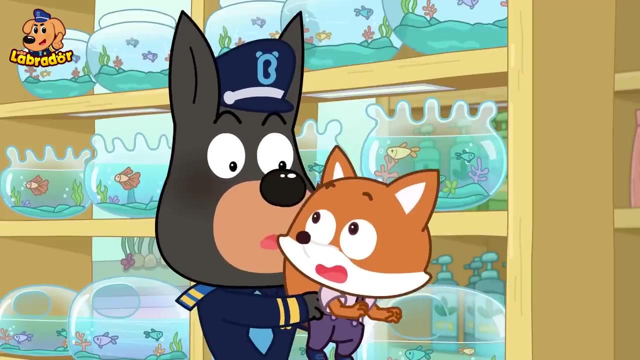 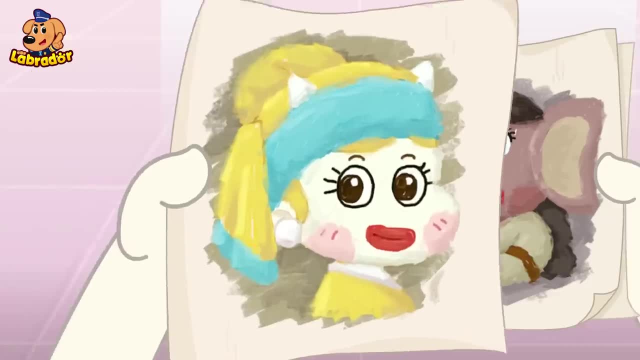 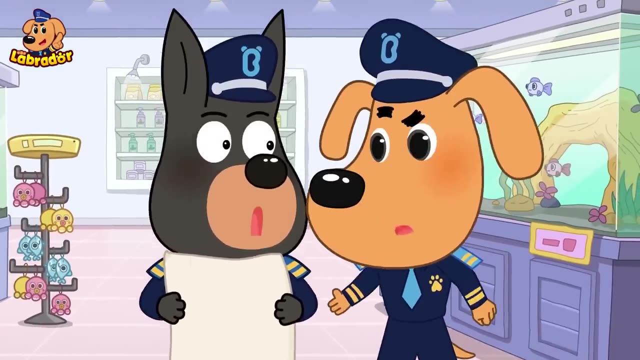 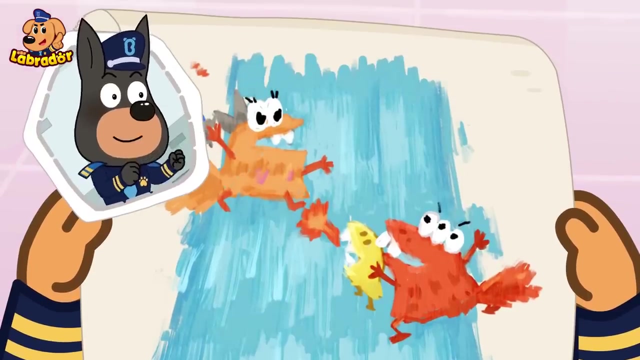 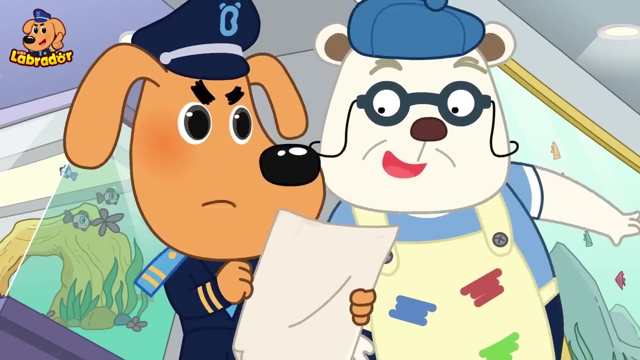 Oh no, My paintings. Thank goodness they're all safe. This painting, What do you think? Nice huh, Wow, Are these two monsters fighting under a waterfall? No, These are two little squirrels on an escalator. That's right, You have good eyes. 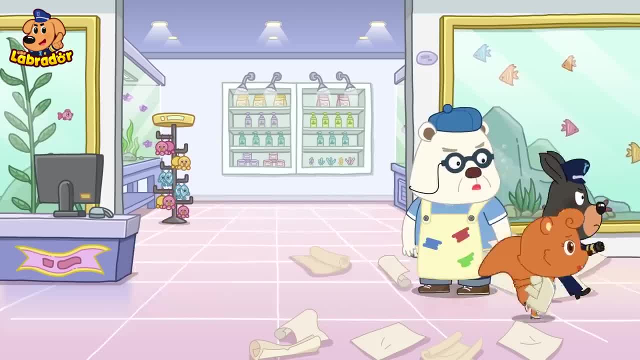 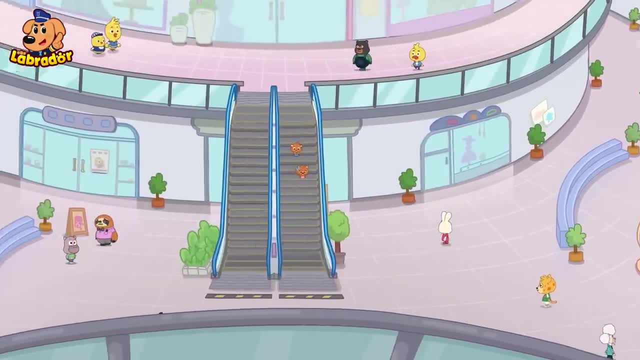 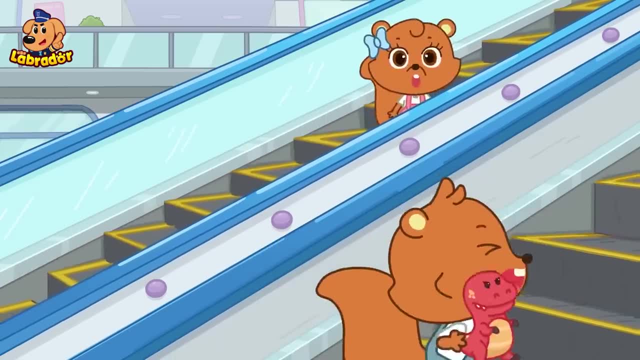 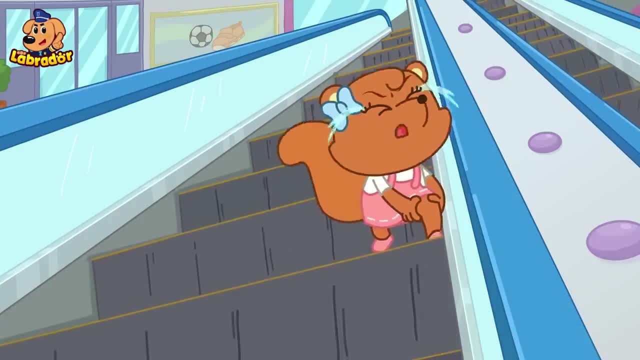 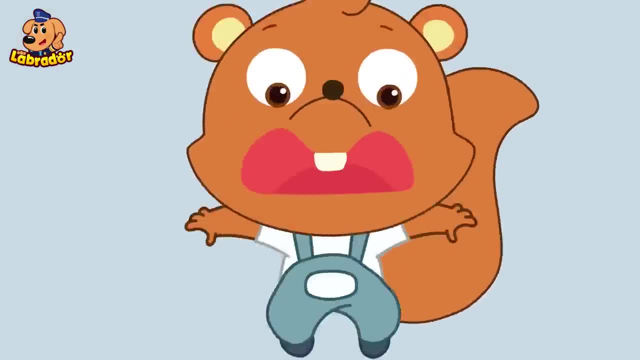 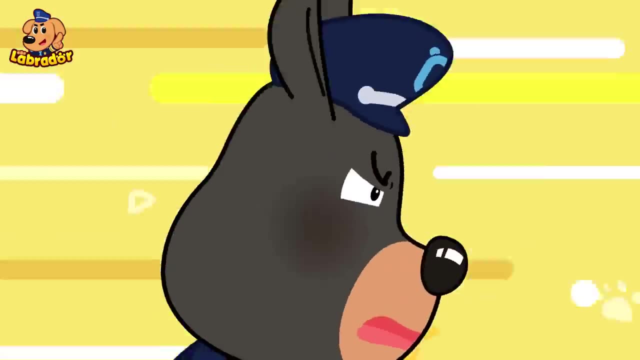 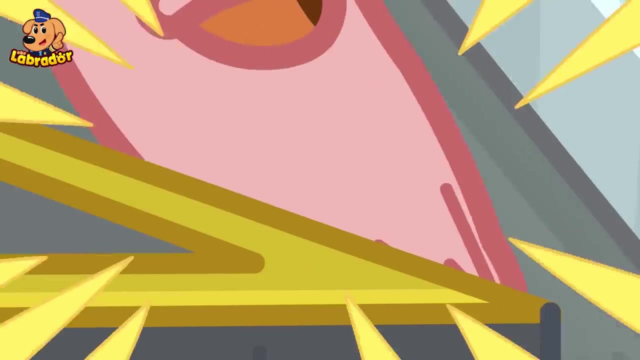 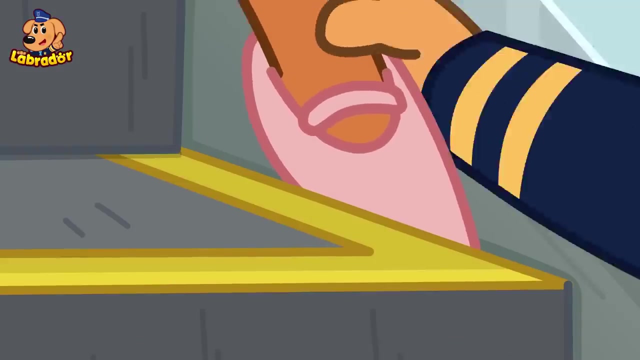 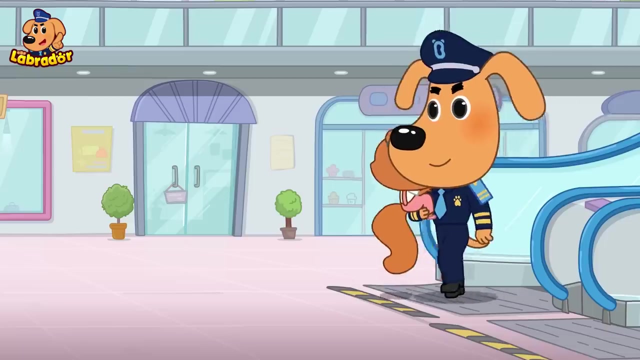 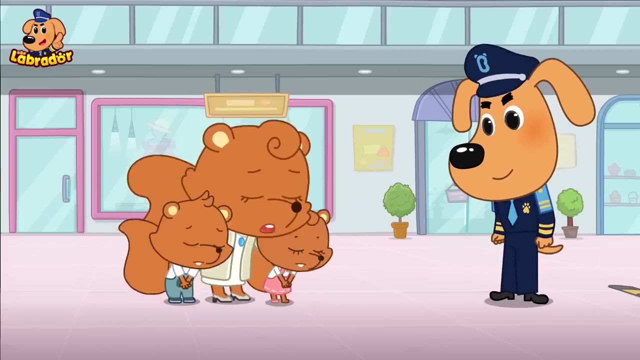 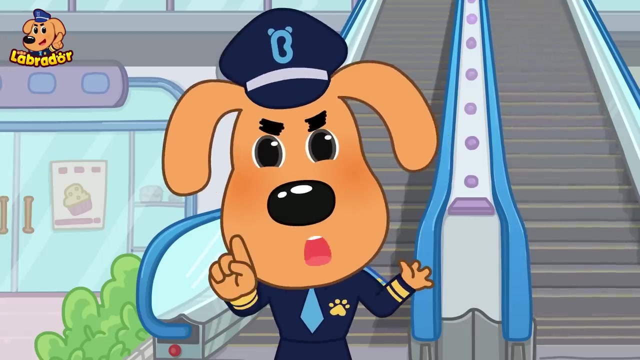 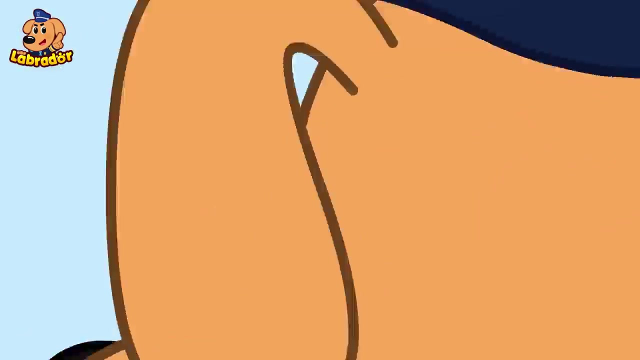 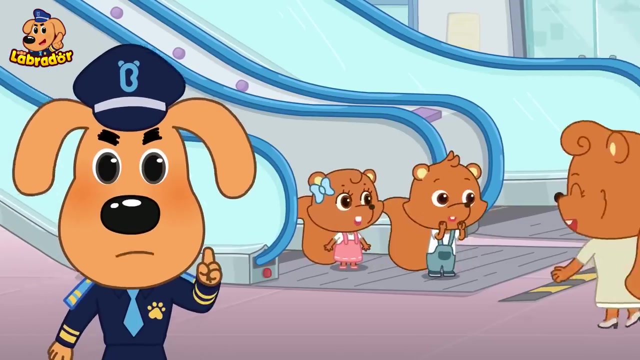 Hmph Watch out. Thank you, Sheriff Labrador. Kids playing on the escalator is very dangerous and you could get hurt. I'm sorry, We'll never do that again. Sheriff Labrador's Safety, Talk Kids. you should only take an escalator. 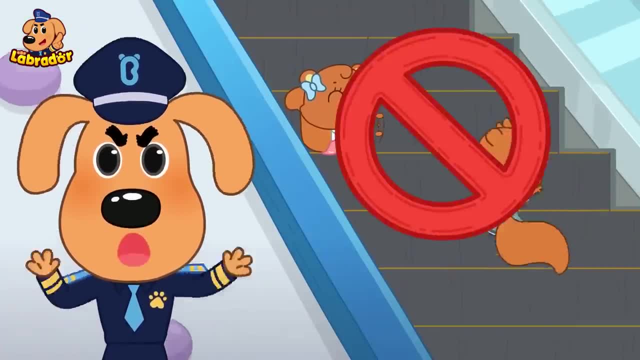 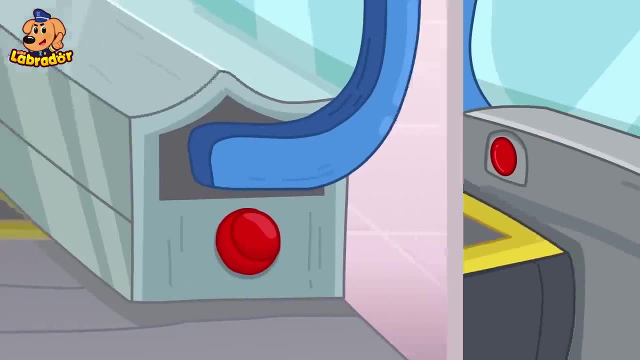 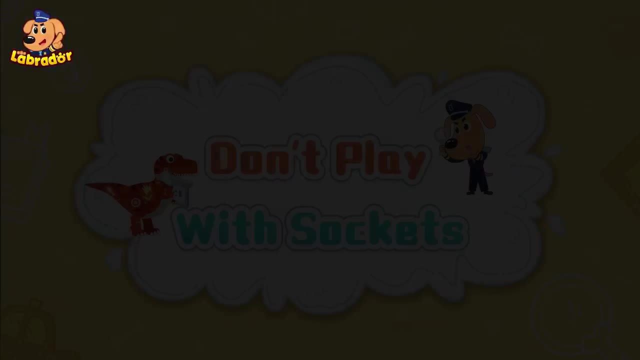 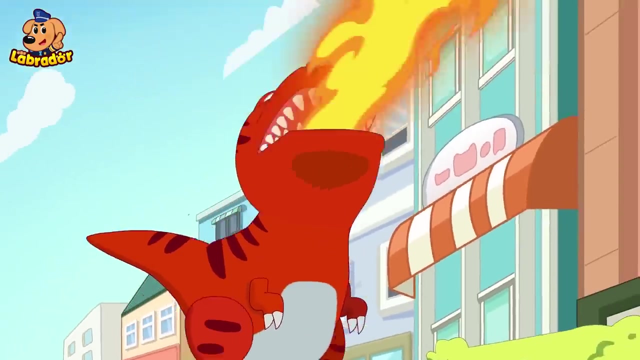 Take an escalator with your parents and never play around while standing on it. In case of an emergency, press the emergency stop button and the escalator will stop right away. Please remember that Don't play with sockets. Go Dino. 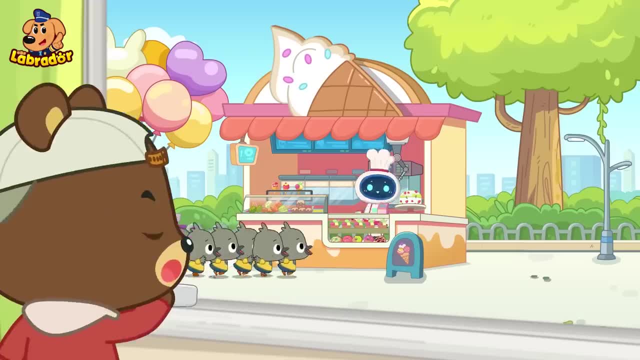 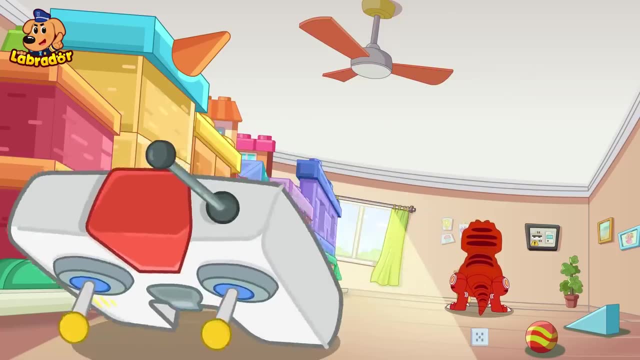 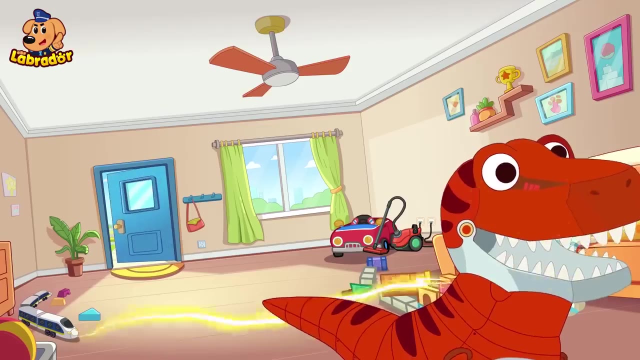 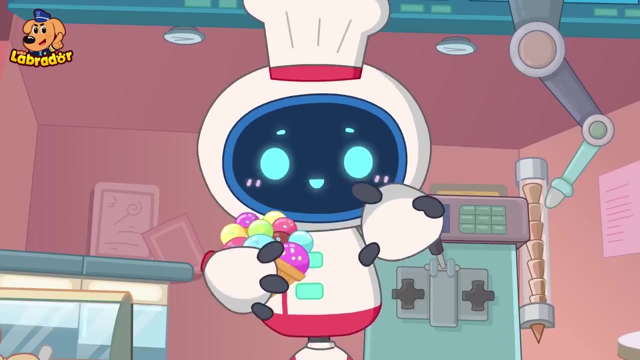 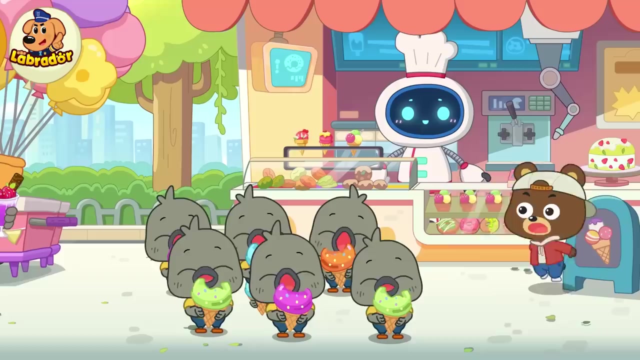 Welcome to Robot Snack House. How can I help you? Ice cream, Ice cream. I want to get some too. Here's your ice cream. Yay, It's so yummy. Wow, One chocolate cake please. Okay, Please. 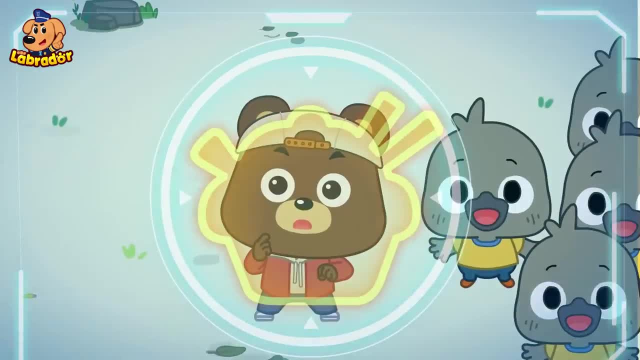 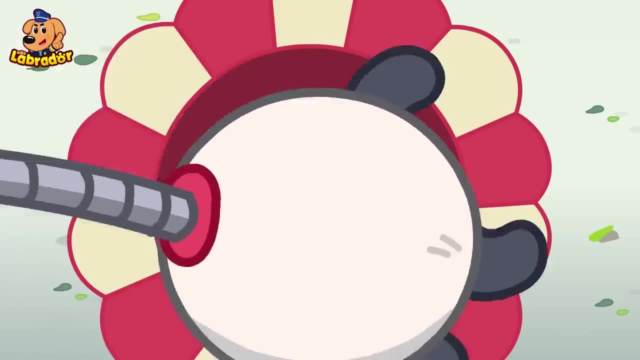 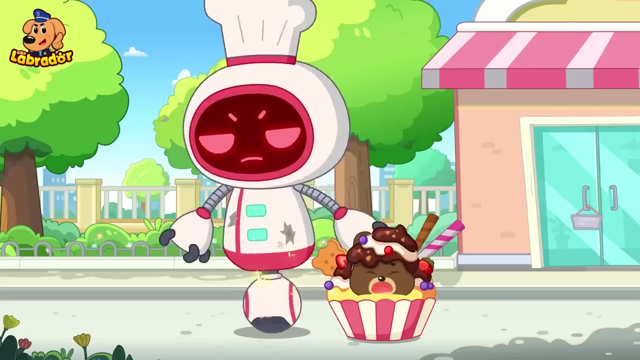 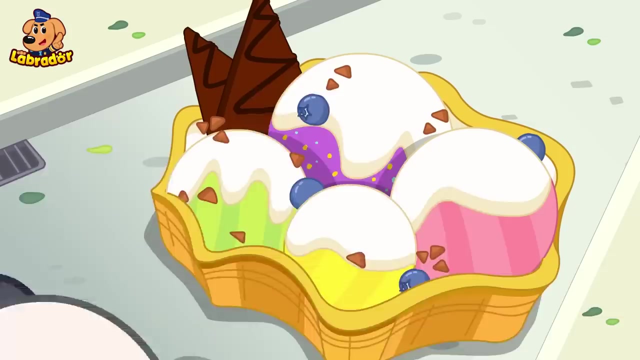 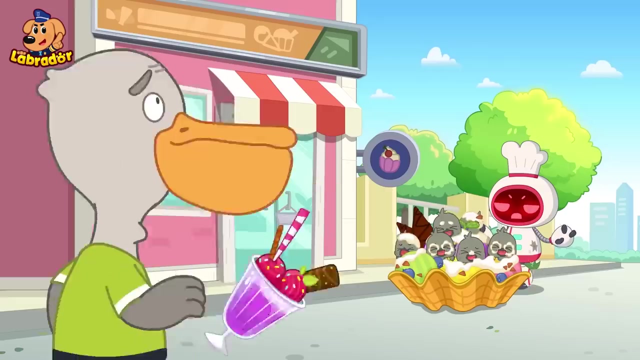 What's going on? Chocolate chocolate, Chocolate cake is ready. Oh no, The robot turned me into a cake. Blueberry Blueberries- We're not blueberries. Help, Let me down. Blueberry ice cream is ready. Oh, that's so terrible. 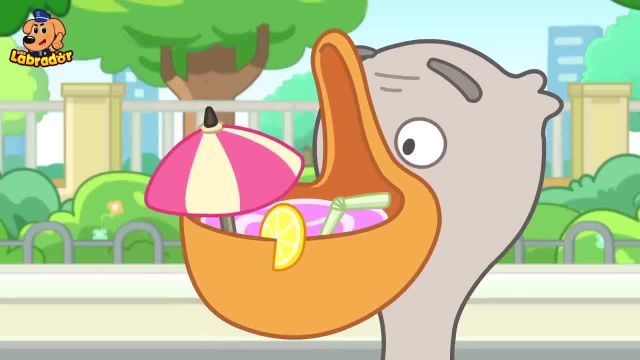 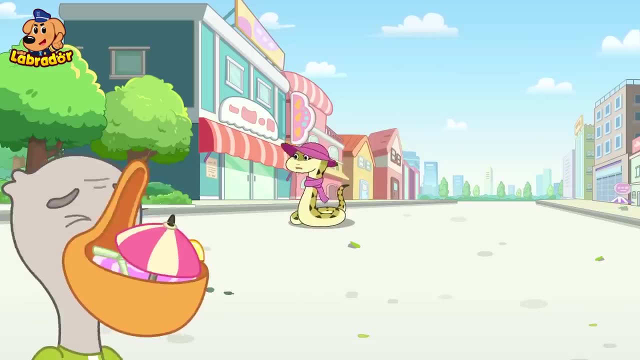 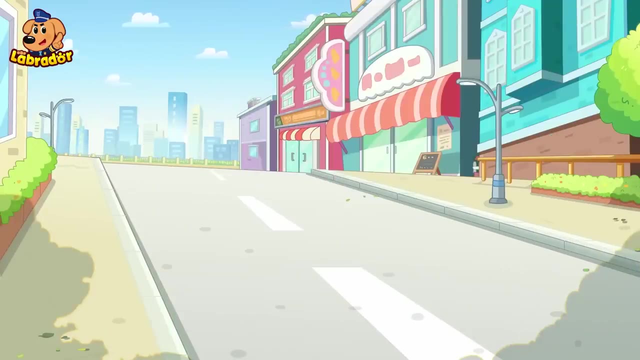 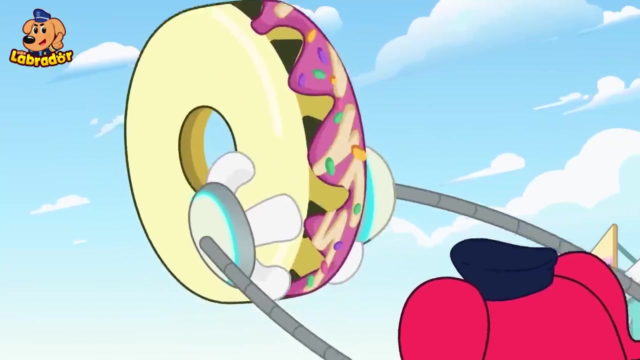 Ouch, The juice cup needs to be filled with juice. Yummy juice is ready. Oh, please help. Huh, What's going on? Oh Oh, Oh. a super donut. Oh, Oh, Oh Help. 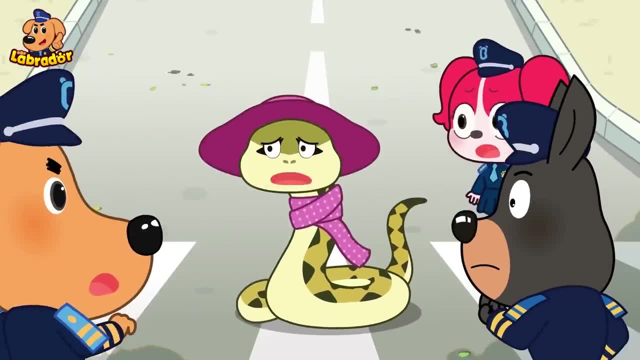 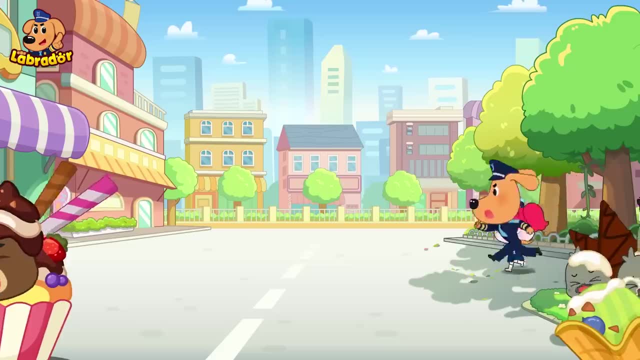 Ms King Ratsnake, what made you become a donut? Sheriff Labrador, something's wrong with the robot at the snack house. Huh, Let's have a look. Help us please. Oh Oh no, They all became food. 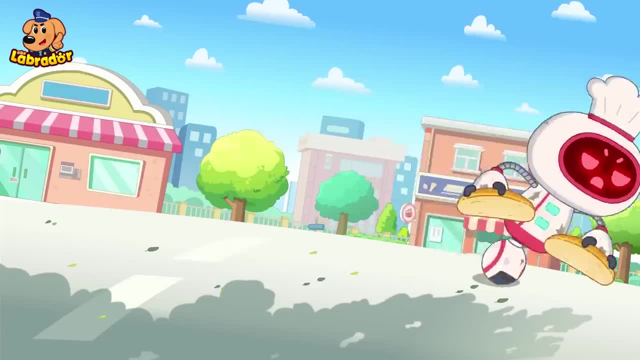 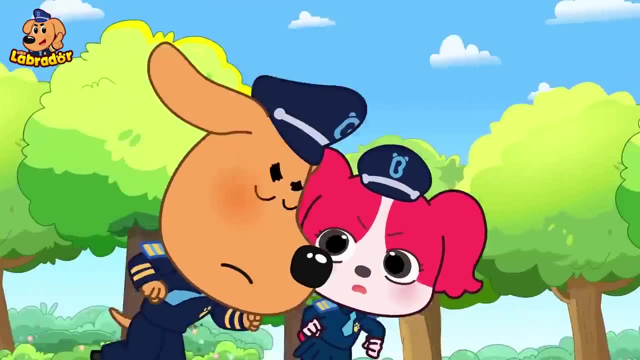 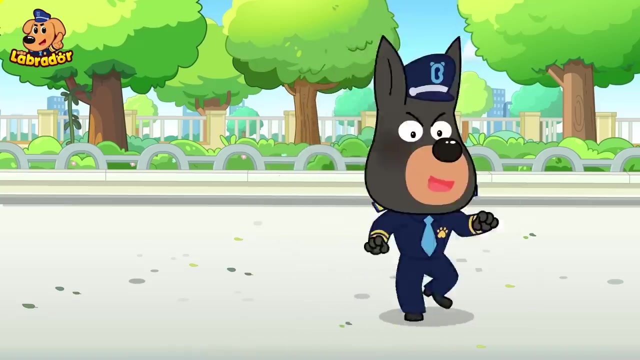 Hot dog, Hot dog. Ugh, Ah, Stop chasing me, Dobby. draw the robot's attention, Help you, Let's save others. Hey Robot, look here, Come on, turn me into a hot dog. Hot dog, Hot dog. 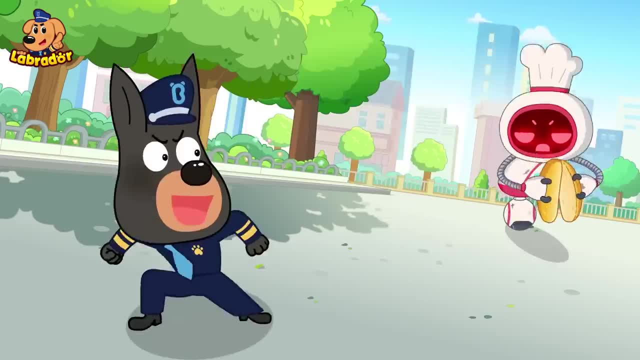 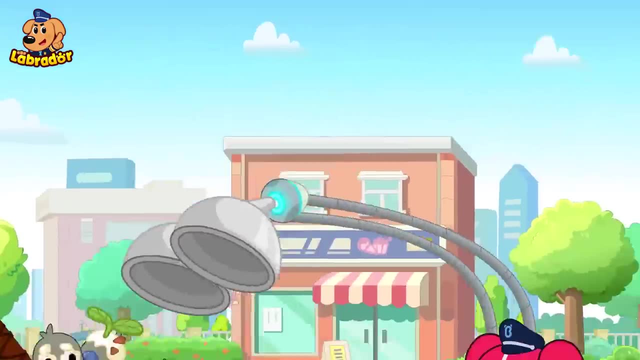 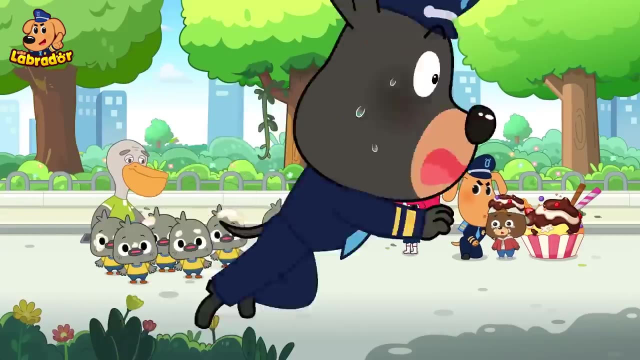 Huh, Huh, It's coming. Come on, Oh, run, Help. Huh, Phew, We're safe now. Huh, Oh no, It's so fast, Sheriff Labrador. Ah, I can't go on. 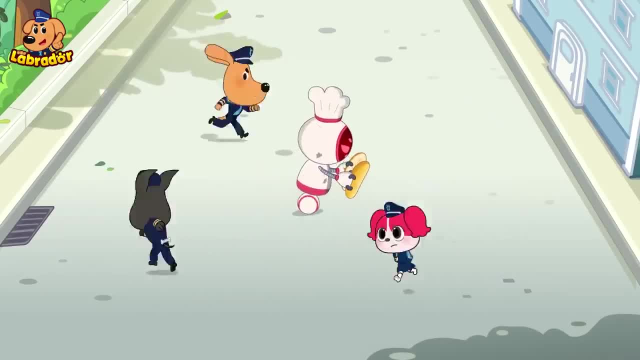 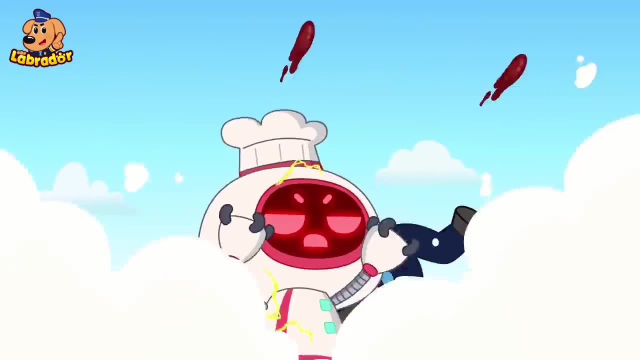 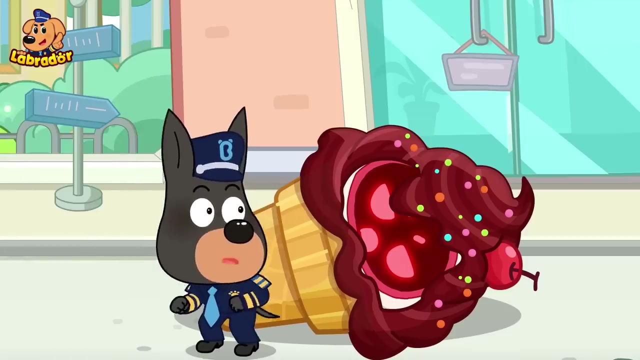 I have an idea. Let's run circles around the robot. Hey, Hey, Hey, Hey. Strawberry, Mango, Avocado, Fruitcake, Fruitcake, Ugh, Huh, Finally it stopped. Uh, what's wrong with the food robot? 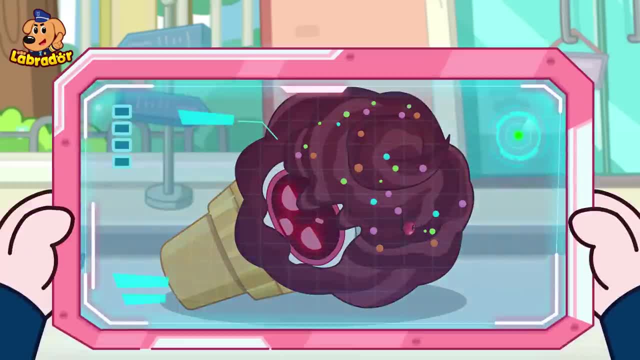 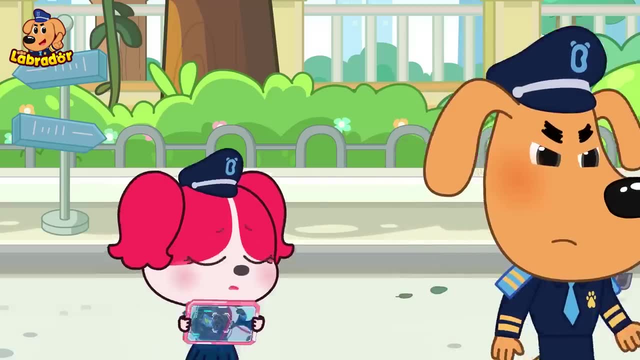 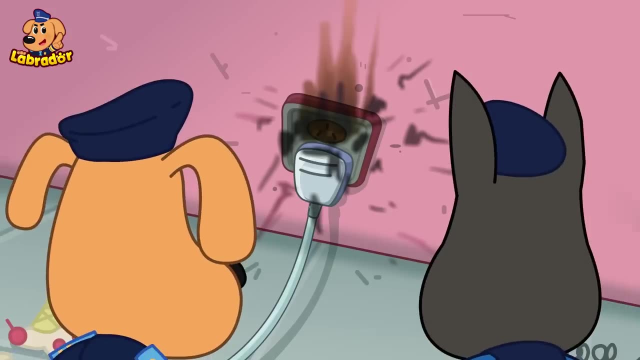 Papillon. give it a check. Hm Eh, Hmm, Its circuits are broken. No wonder it went out of control. Huh, Let's go check the shop. Huh, Huh, Huh, Huh, The robot's charging socket is burnt. 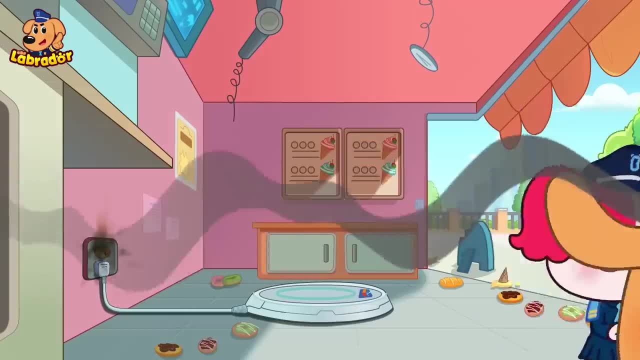 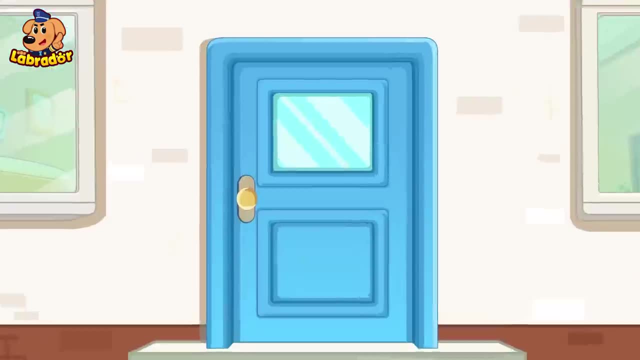 Huh. Oh no, Something's wrong over there. Huh, Huh, Huh Huh. The smoke's coming out of my house. Stay here, We'll go have a look. Huh, Huh, Huh. 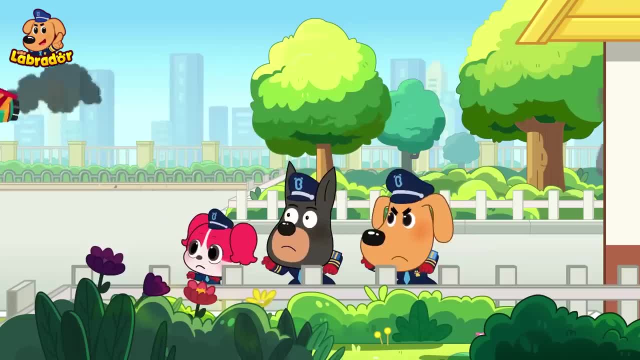 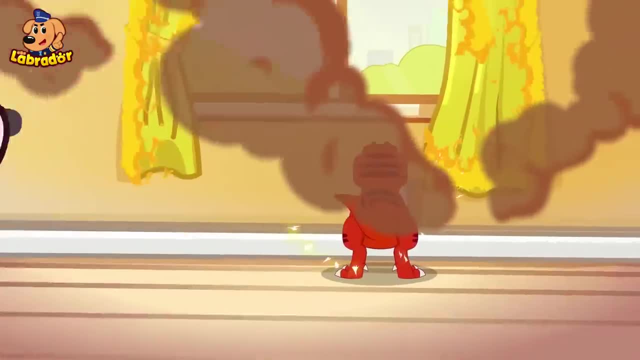 Huh, Get down. Huh, Huh, Huh, Huh Huh. Oh my, What's going on? Huh Huh, The dino robot's hand got stuck in the socket. That's what made the food robot and other sockets broken. 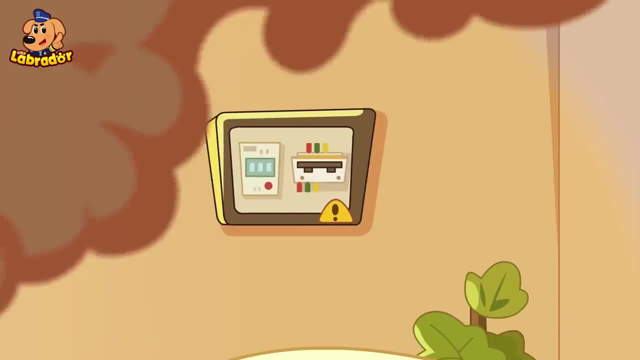 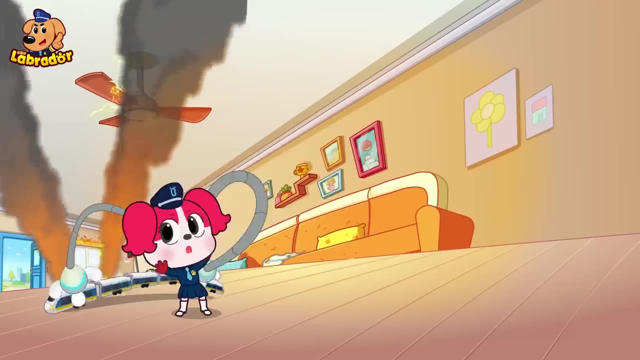 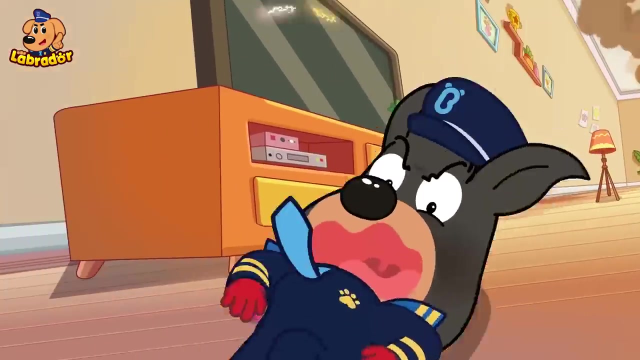 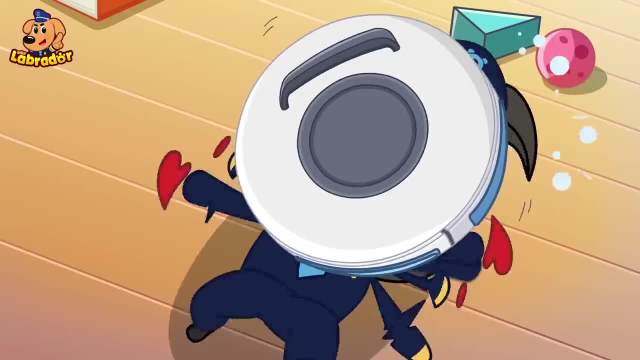 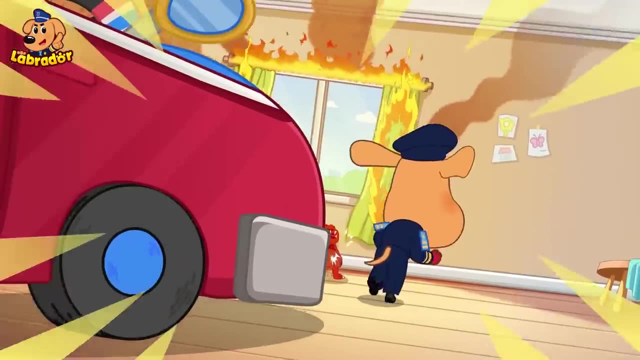 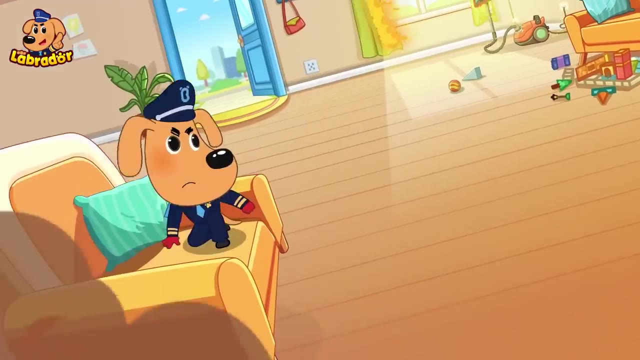 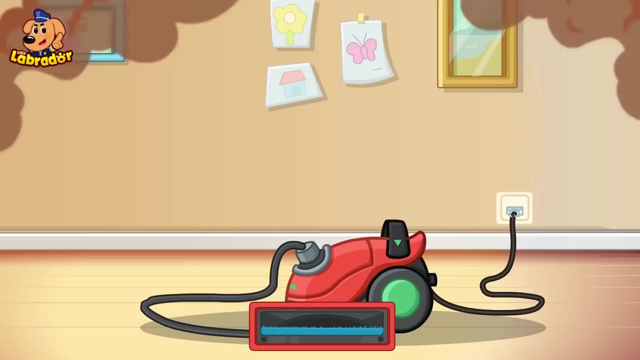 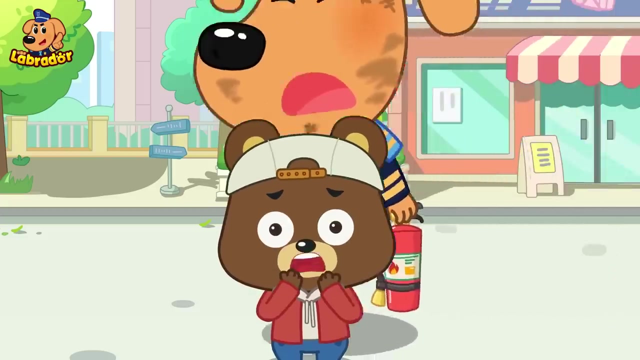 Huh Huh, Trash detected, Trash detected. Go away, I'm not trash Trash. Uh Huh Huh, Watch your back. Eh Ugh, hey, Hey, Power off. Oh, That was so scary. 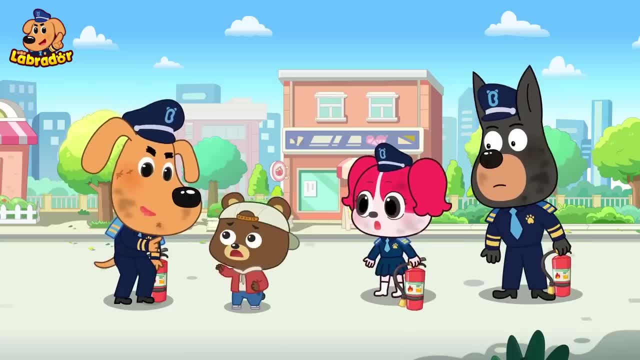 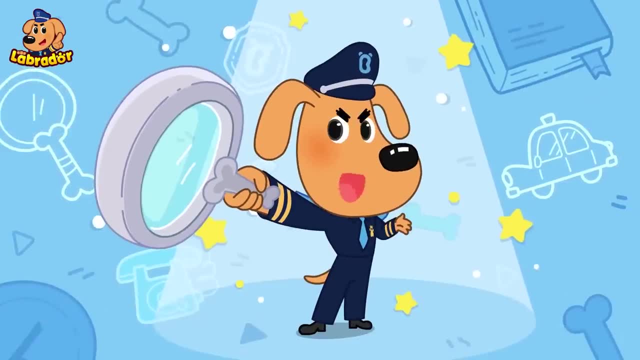 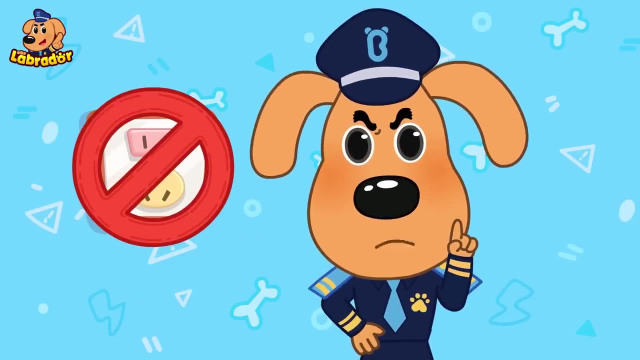 Little Bear, you should stay away from sockets. OK, Oh, I got it. Sheriff Labrador's Safety Talk: Kids. sockets are very dangerous and you should never touch them. If you do, you could get seriously hurt by electric shock. 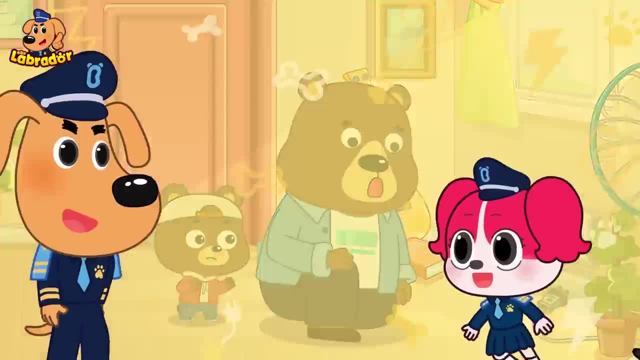 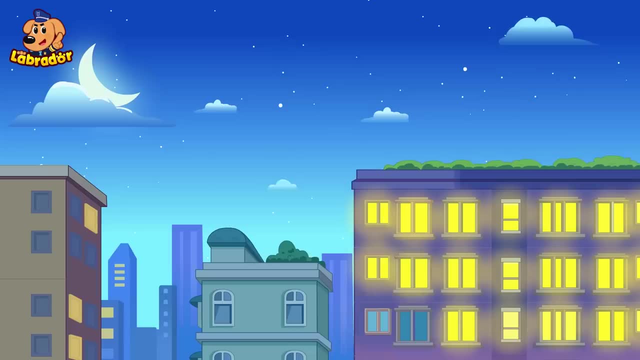 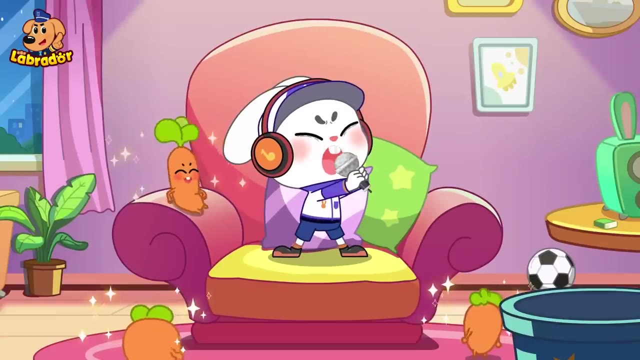 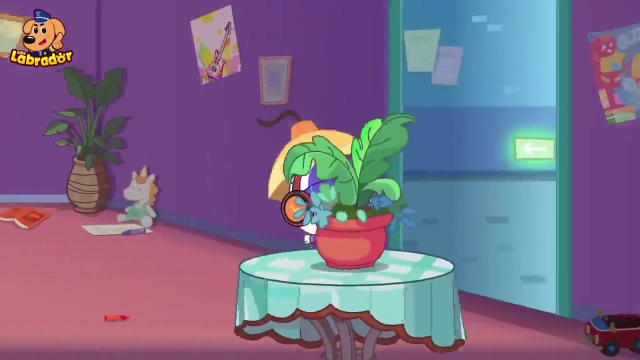 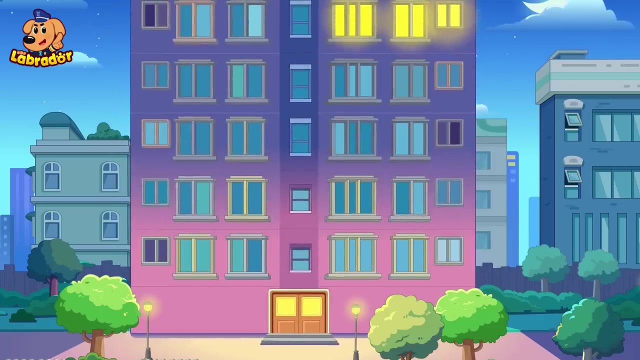 So if you need to use electricity, ask an adult for help. Please remember that The Scary Noise Peep-pee Rabbit. Peep-pee Rabbit Loves to sing. loves to sing. Who is it? Stop banging? I can't bear it. 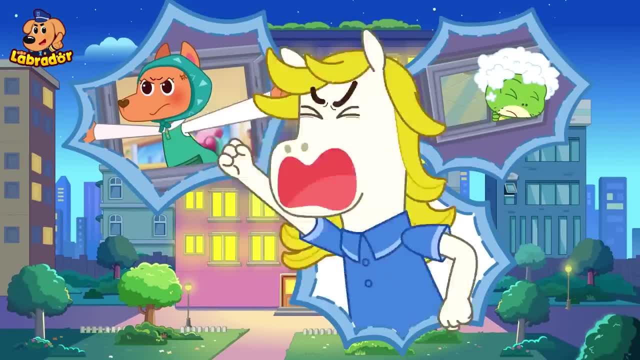 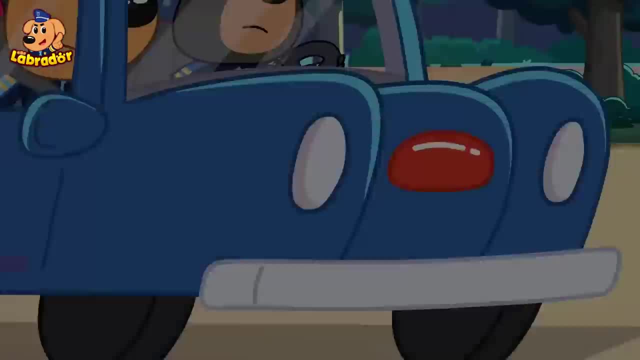 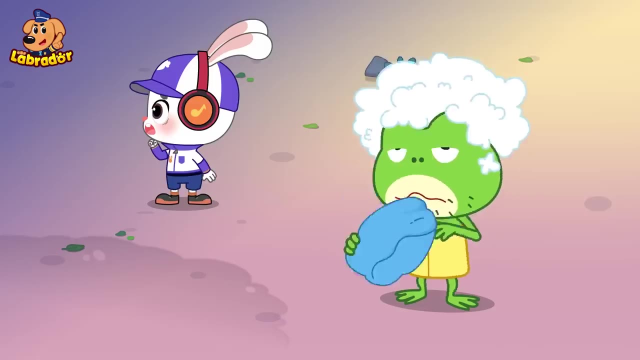 Ribbit, stop it. Who is it, Please stop? Who is it? Stop banging. Who is it? Stop banging? Sheriff Labrador, someone's playing a prank. They can't sleep at all. Ribbit, That's right. Please find out who it is. 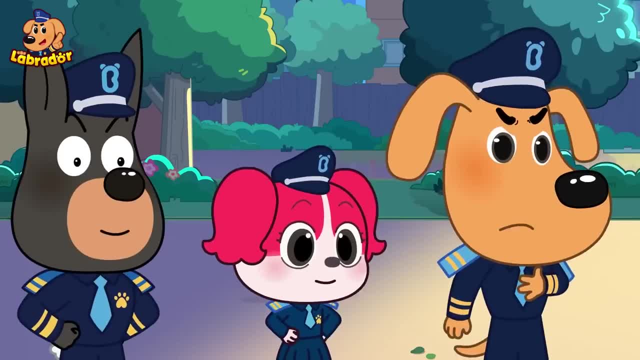 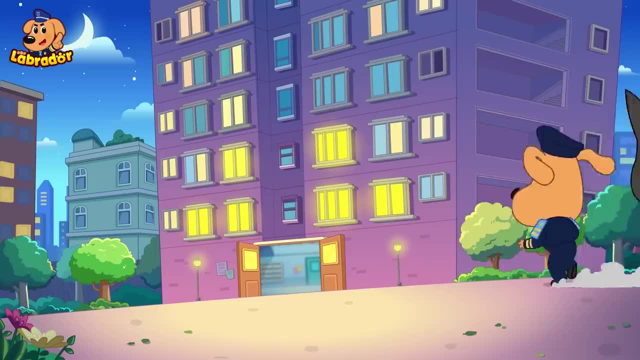 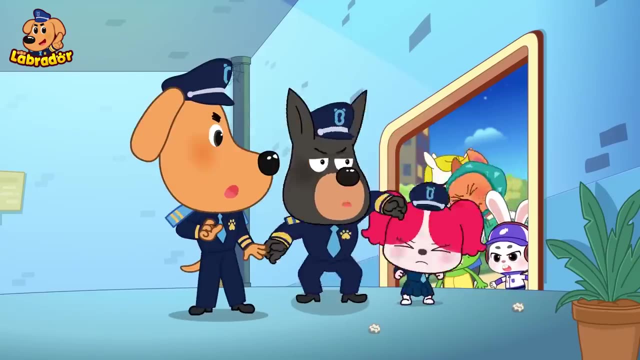 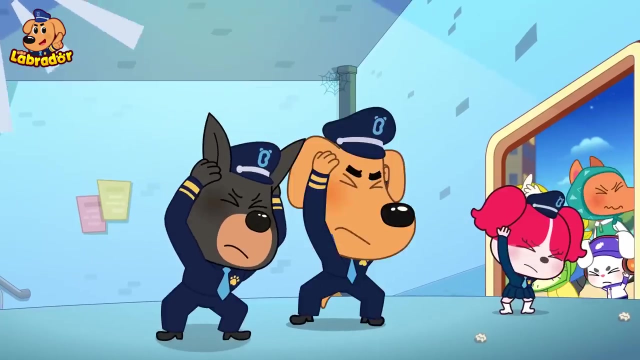 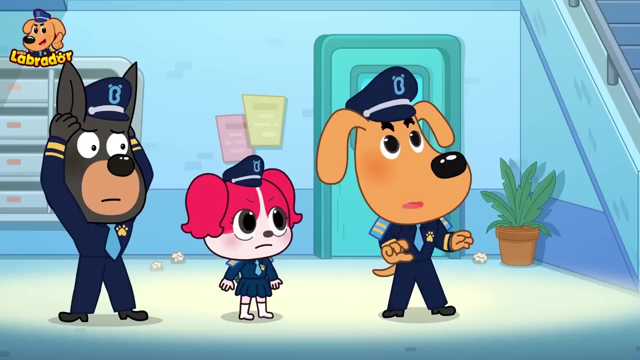 Everyone, don't worry, Leave it to us. Who could it be? I'll go have a look. Let's go. Grrrr, Let me use my sensitive ears to listen. No, Gimme a break. Excuse me, I couldn't find my ears. 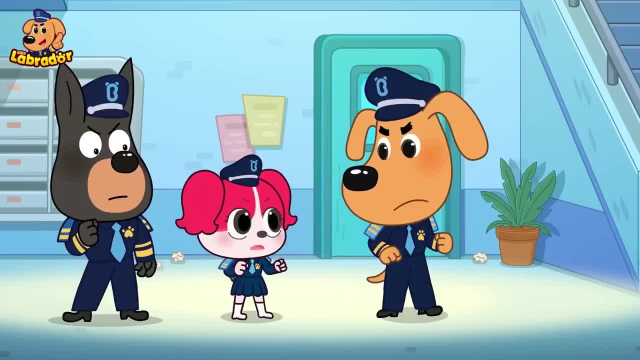 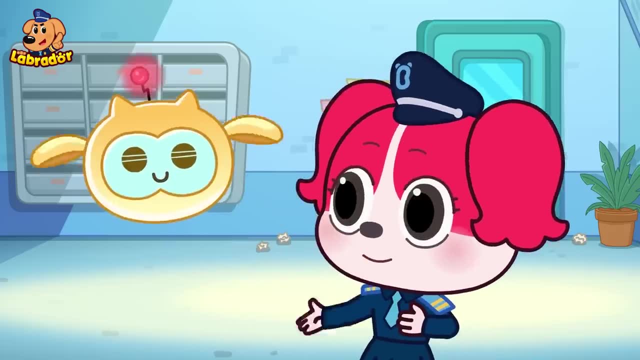 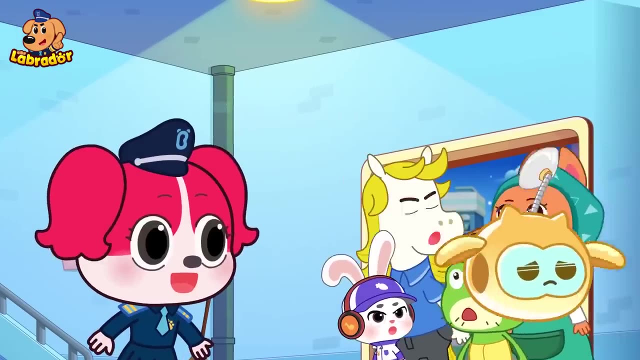 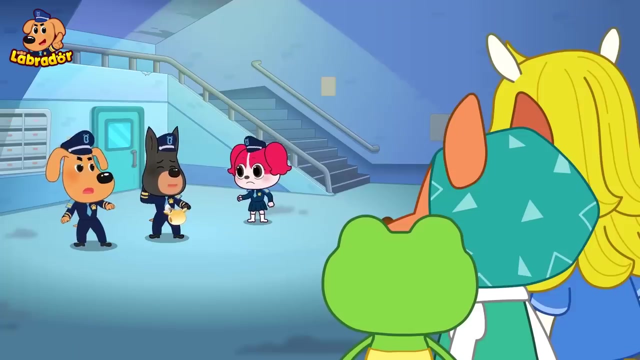 Papillon, I may not hear you belts. well, We'll figure it out. I'll put it around your ears, Holi, that It'll find the source of the sound by detecting the vibration. Wow Found it. It's my stomach growling. 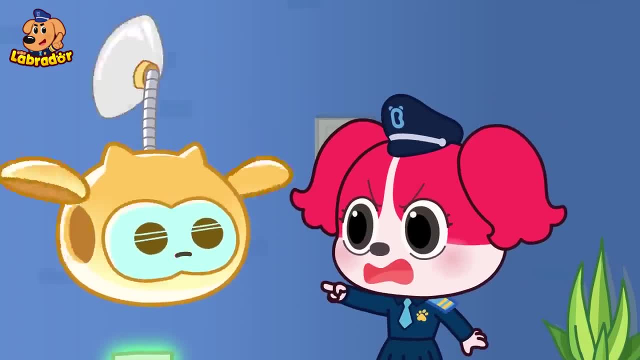 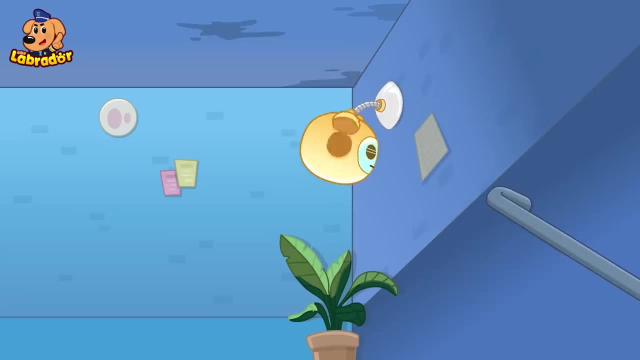 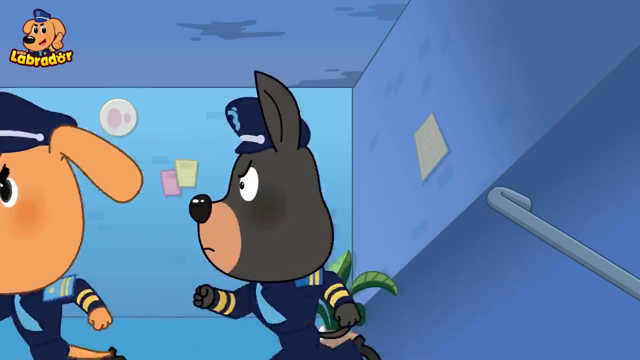 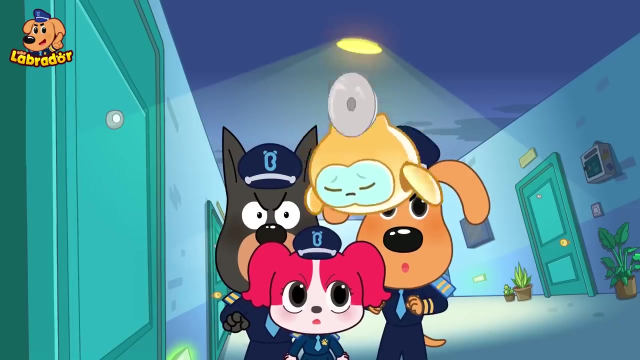 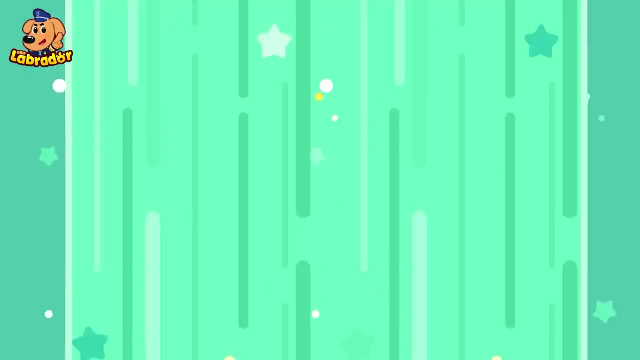 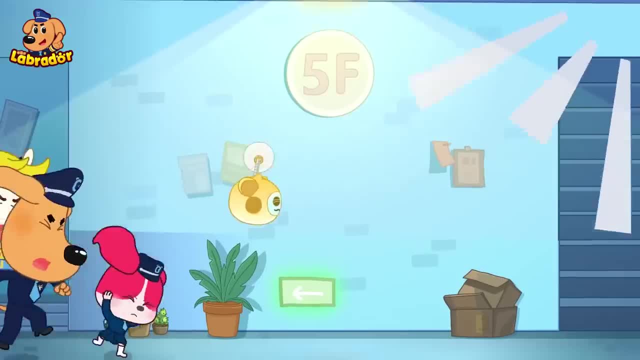 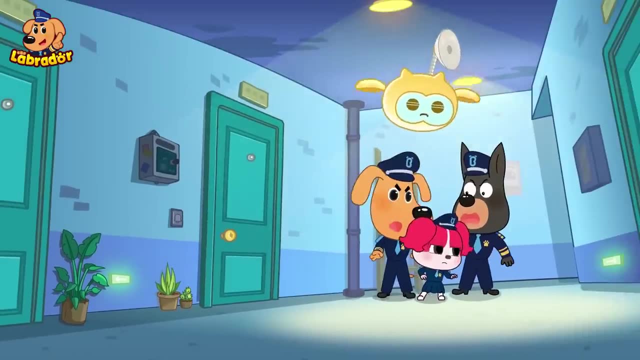 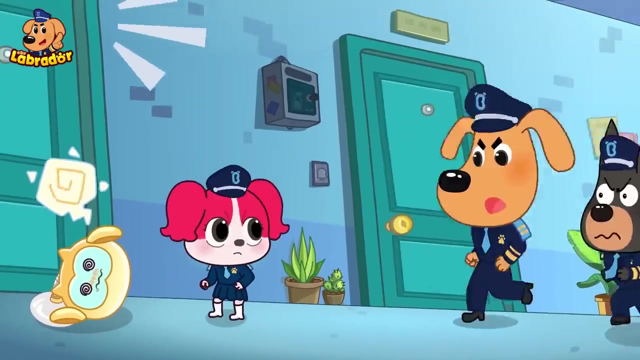 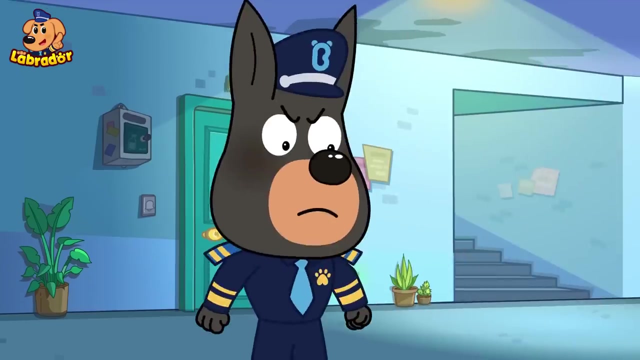 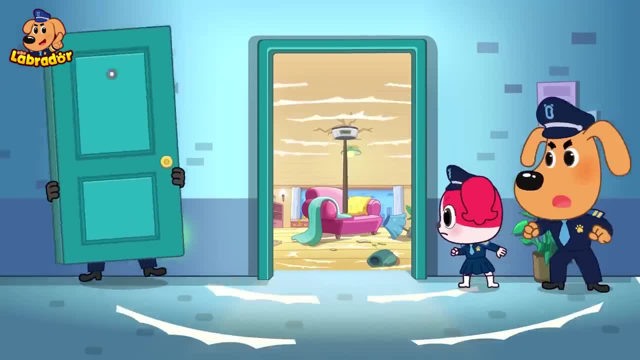 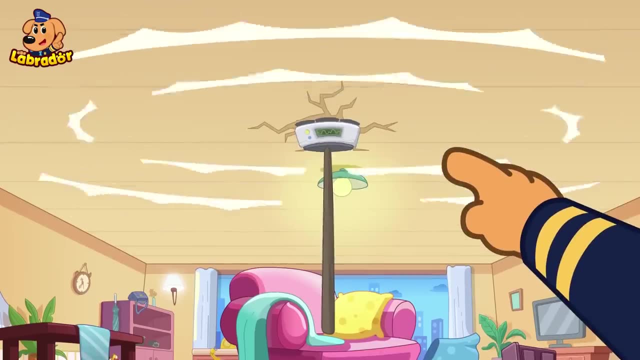 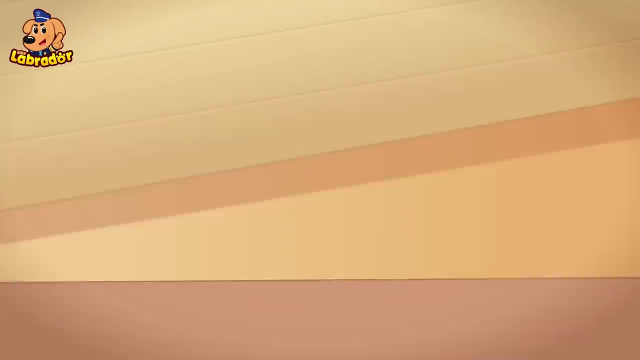 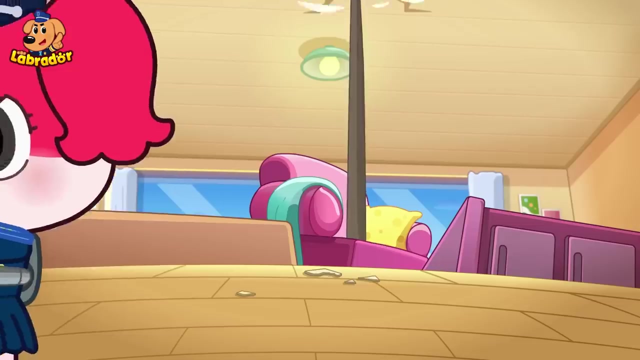 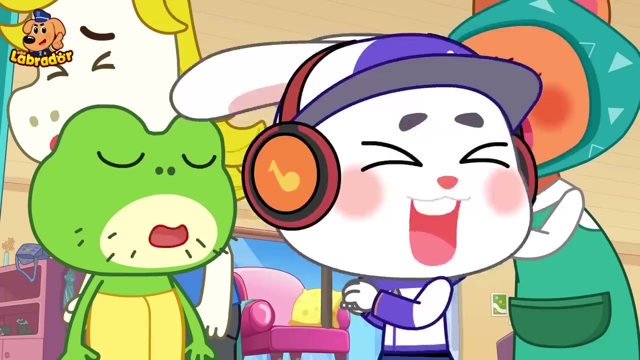 Turn around, Turn off that thing. It makes my head hurt so much So that machine has been banging on the ceiling and making noise. Papillon, take me over there. Come on, Papillon. it finally stopped. Mr Bison, that was too much. 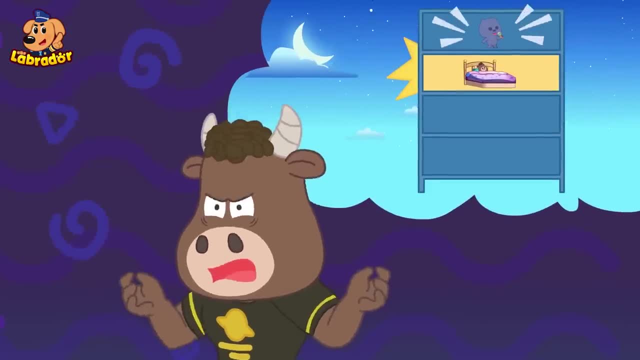 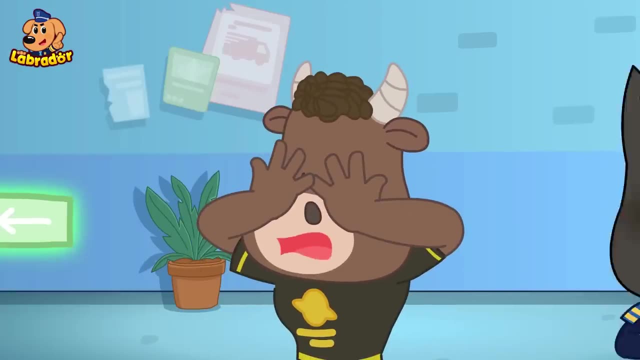 I didn't want to, but the person upstairs was singing so loudly every night that I couldn't sleep. I just wanted to get my revenge. I didn't expect that I couldn't stand it either. I didn't hear anything Again. That's what I was talking about. 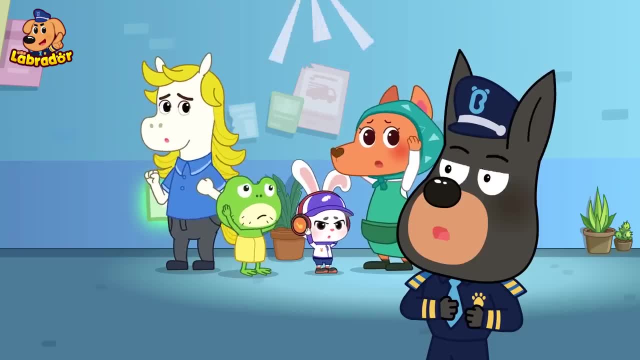 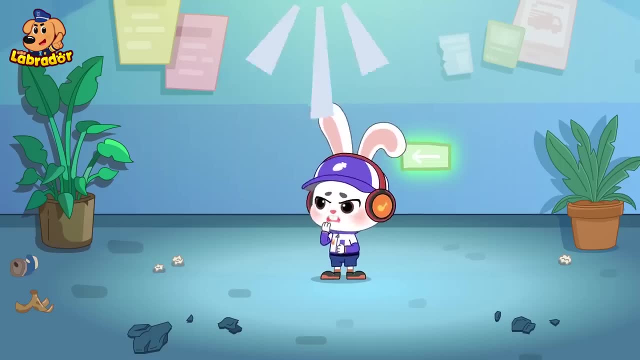 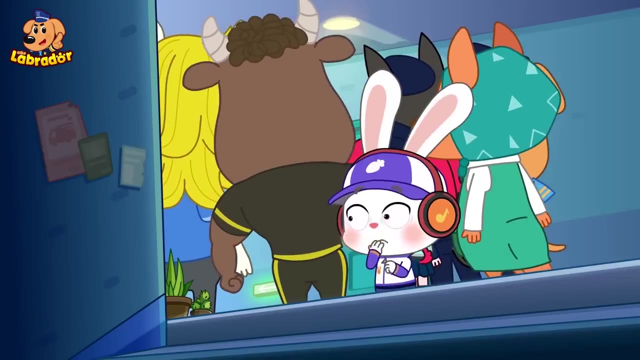 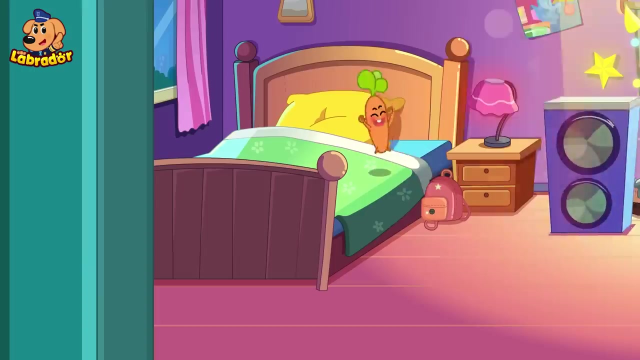 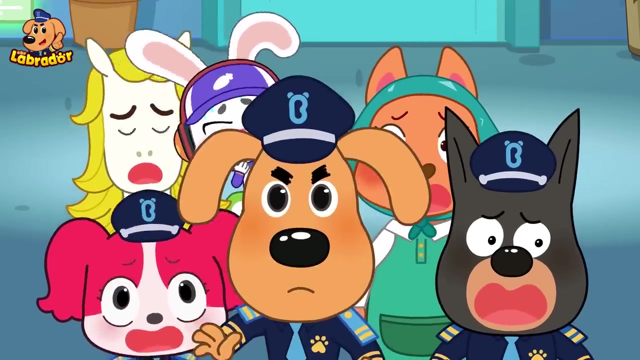 Who's singing now? It sounds awful. It's getting louder. Let's go take a look Upstairs. Could it be This house? Oh no, It's my house. They're playing instruments. Oh fine, Pee-pee. 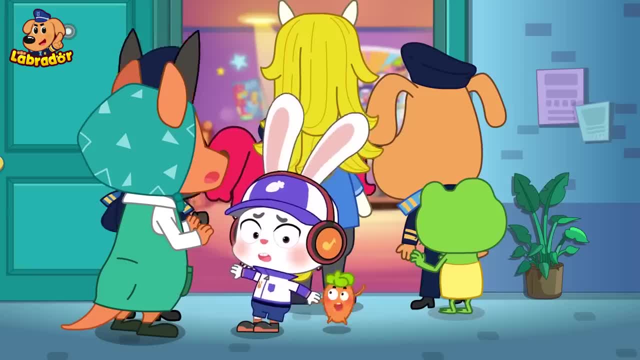 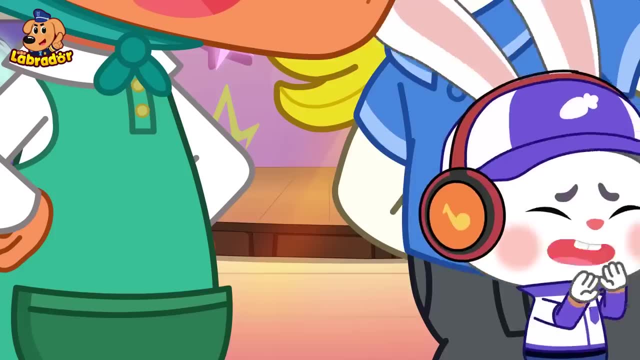 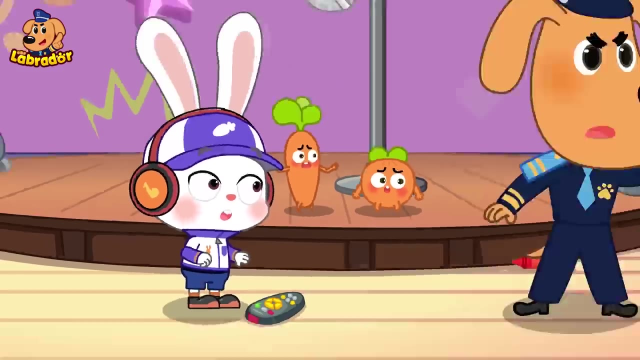 Pee-pee, It's your house, So the one who kept me from sleeping is you Sorry. I'm sorry, Pee-pee Rabbit. Mr Bison, since you've made so much noise and disturbed everyone, you'll be doing community service. 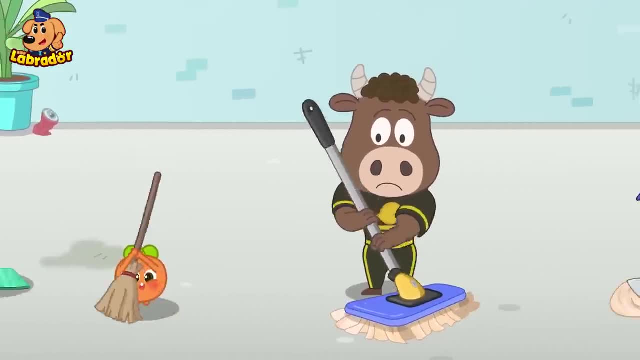 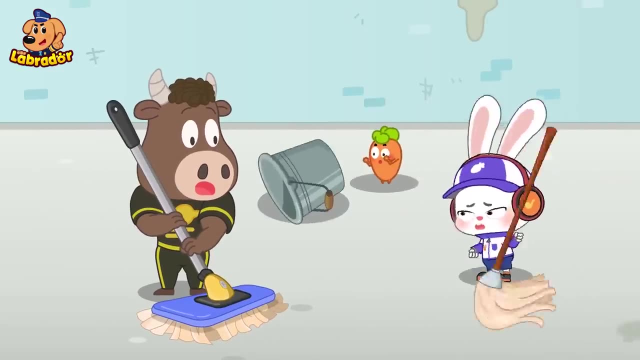 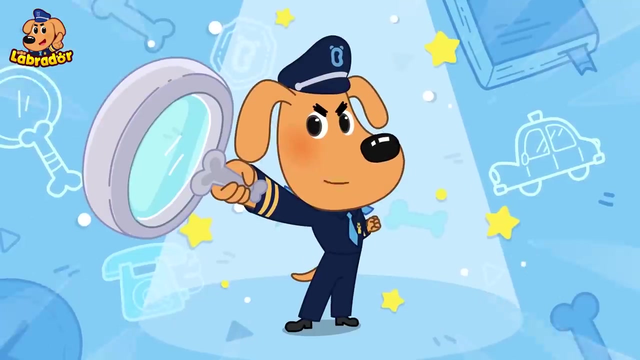 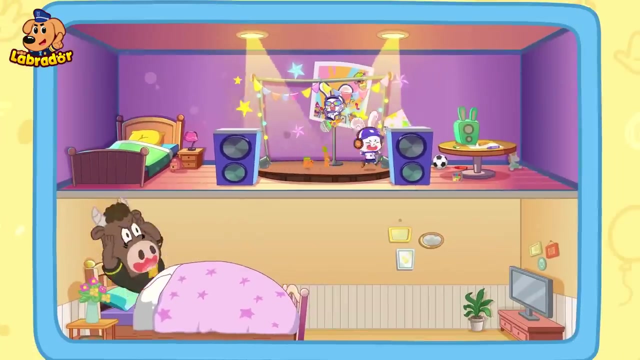 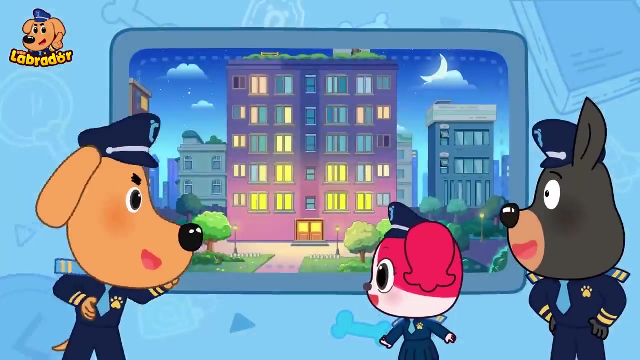 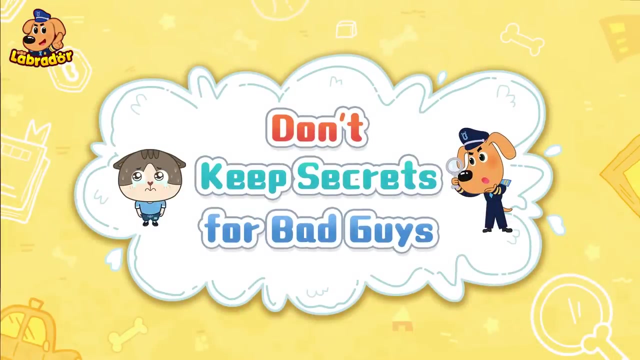 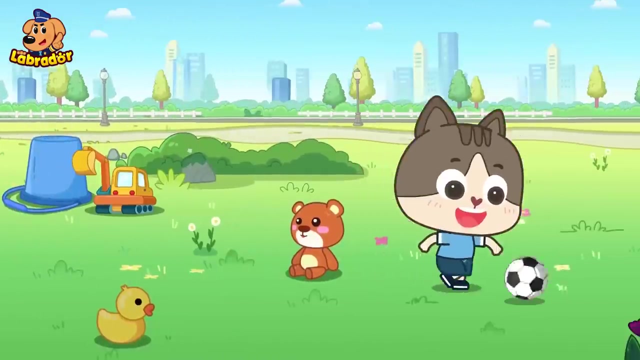 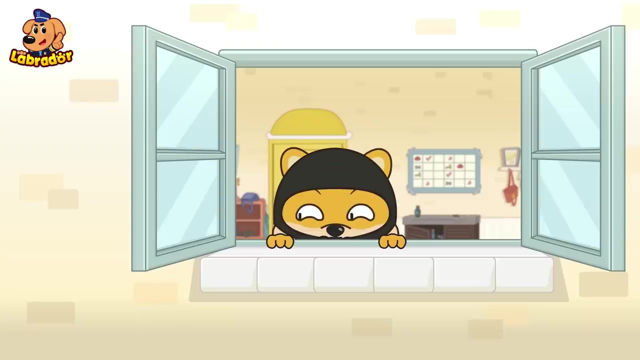 Okay, Oh, I'll never make loud noise again. Ah, Shh, Shh. Don't keep secrets for bad guys. The game is starting. Look at my power kick. Ah My ball. It's my lucky day, Ah. 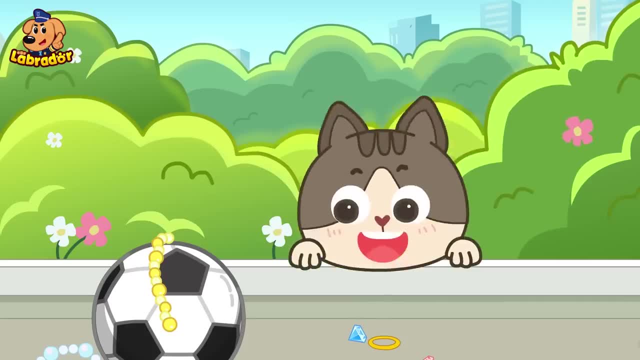 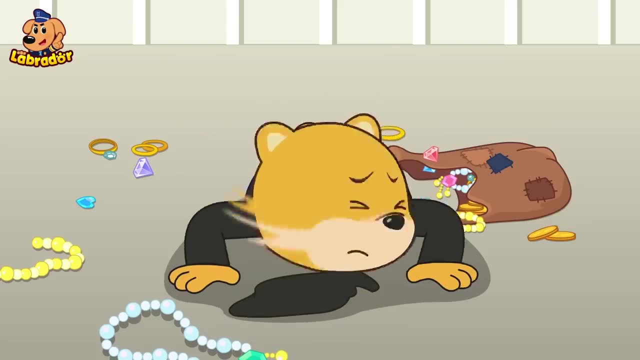 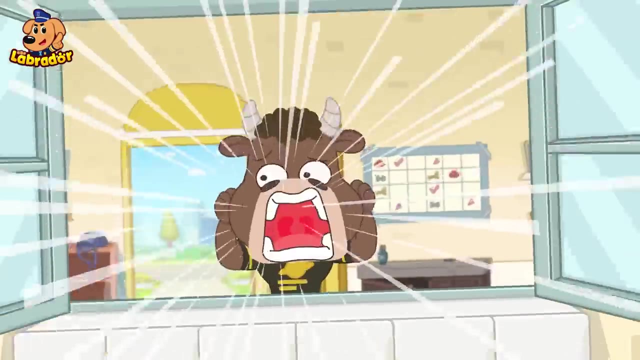 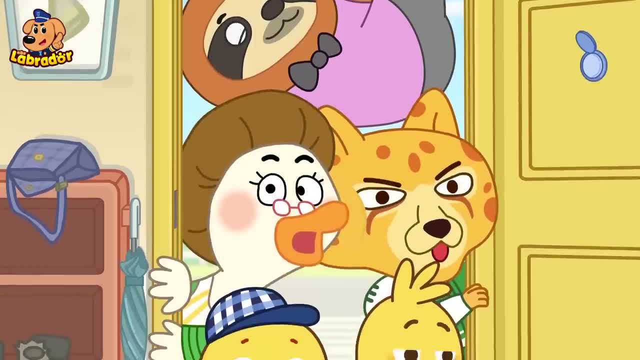 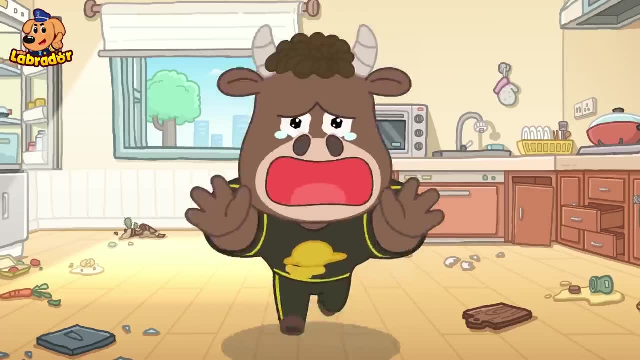 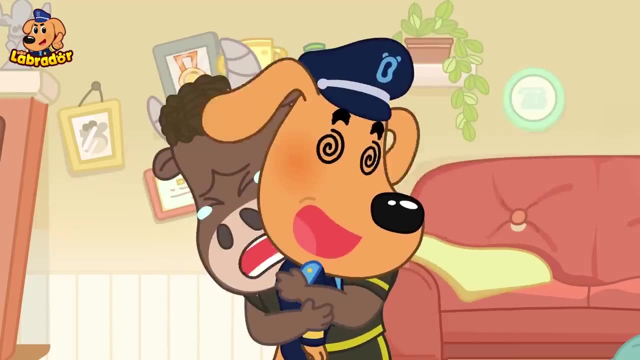 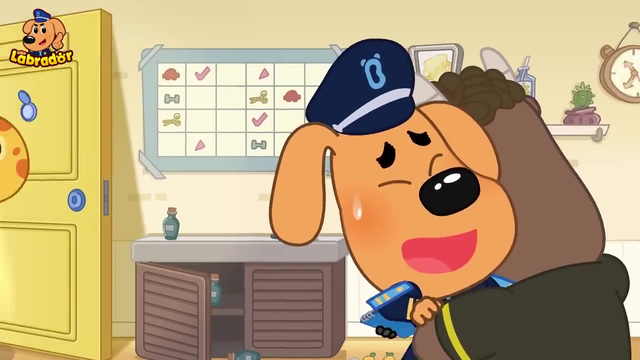 I will. It's such a mess. Ah, Sheriff Labrador, All of my valuables are gone. Please find out who did this. Don't worry, There's no case that I can't solve Everyone. have you seen anyone suspicious today? 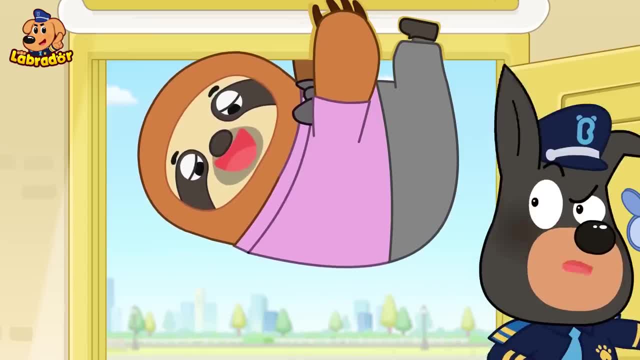 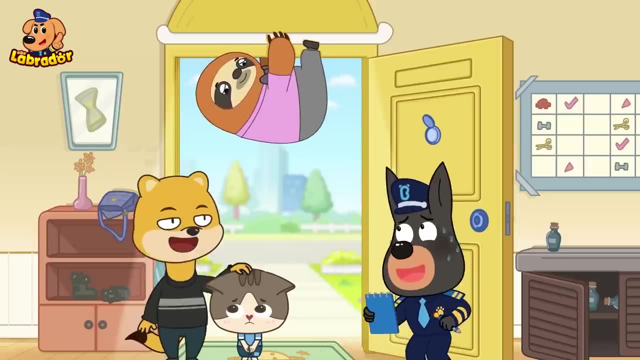 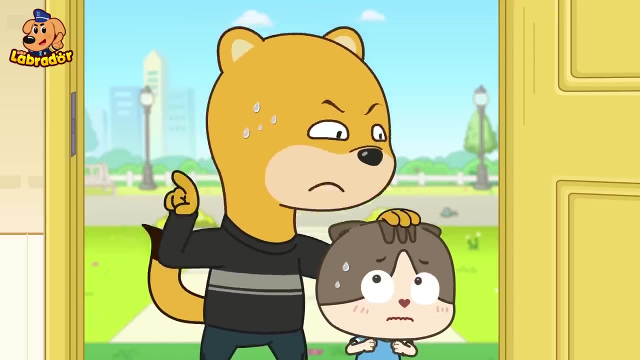 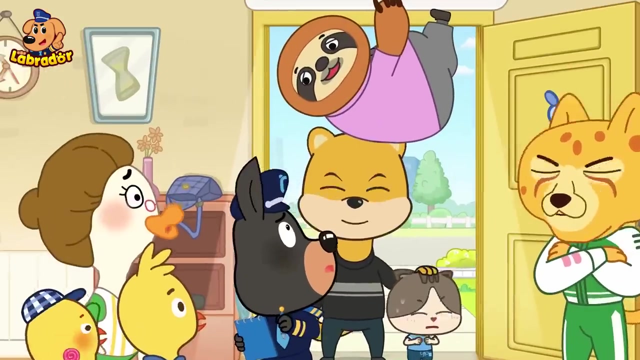 Slowly, One by one, please. I saw no one. If I see the thief, I won't let him get away. How about you guys? Uh well, it's such a bad thief. We didn't see anyone. I have been sleeping all day. 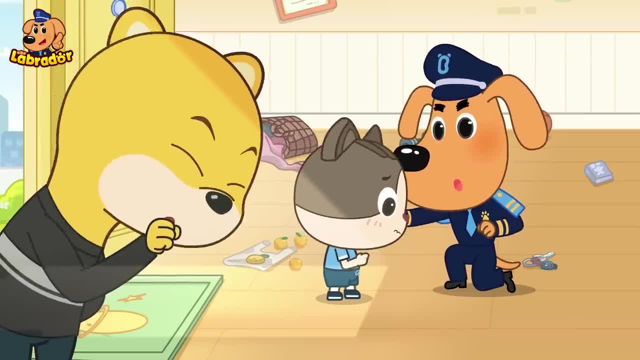 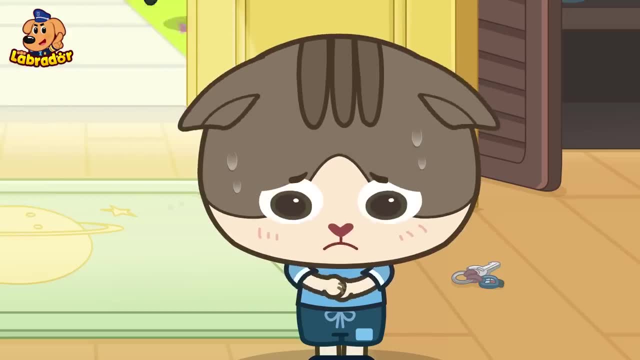 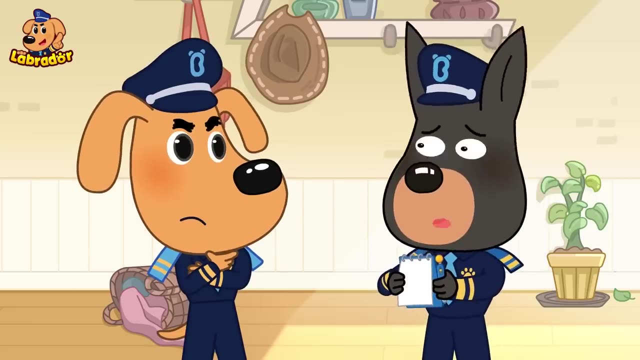 Little Cat, do you have anything to tell me? I, I See you later, sir. I I didn't see anything. Ouch, Looks like we've found no clues. No, I think Little Cat's hiding something. Let's go find him. 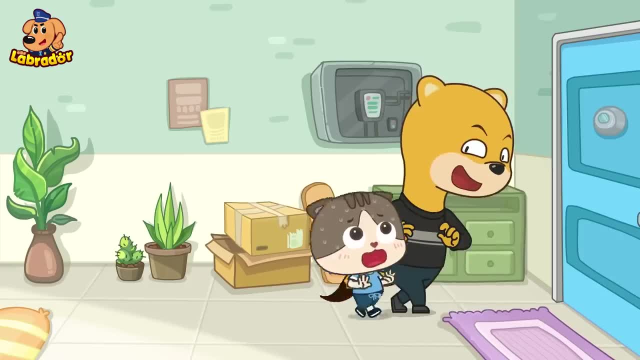 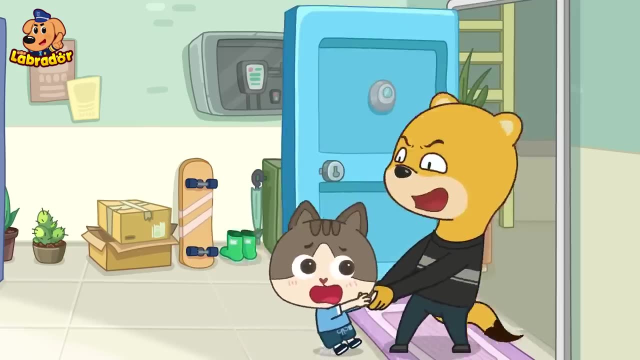 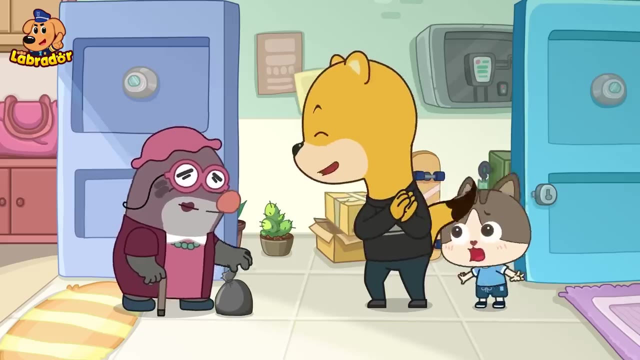 I, I didn't tell anyone, Didn't think you would. All right, let's go into your house. But Hello, Little Cat, Ms Moore, Hi, Good afternoon. Good afternoon, Ms Moore. Little Cat and I were playing. 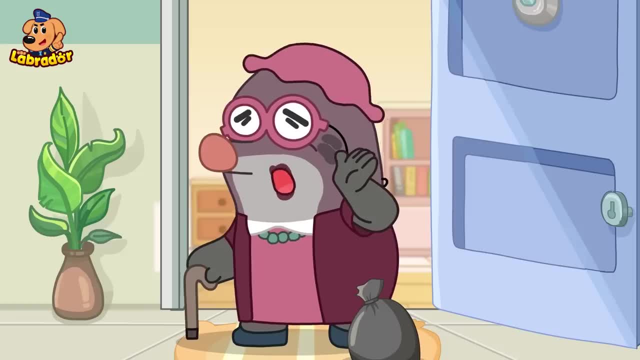 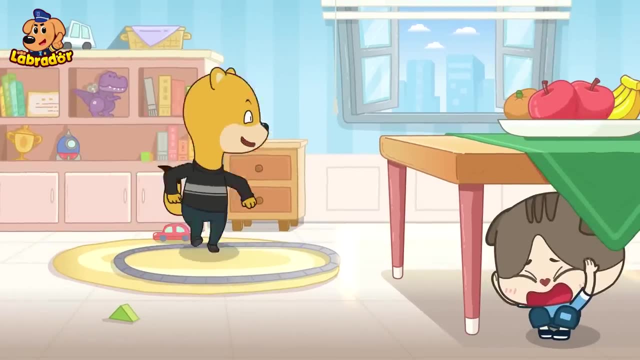 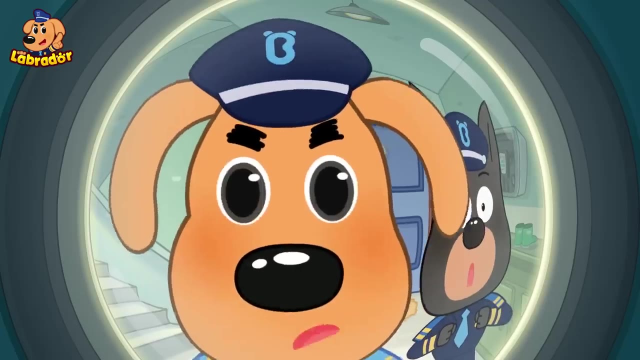 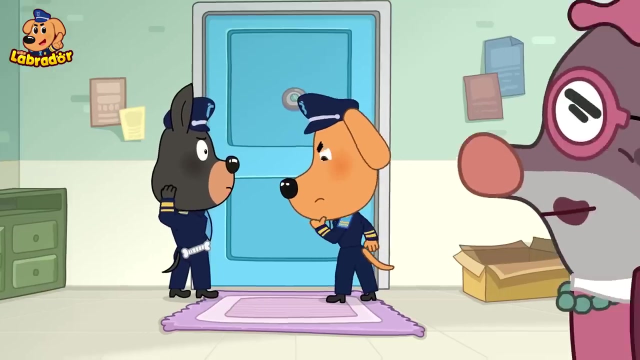 Well, goodbye. What did you say? Hey, Oh, Ouch, There are lots of valuables in your house. Are you home, Little Cat? Maybe he's still on his way. Huh, Oh, Sheriff Labrador, is that you? 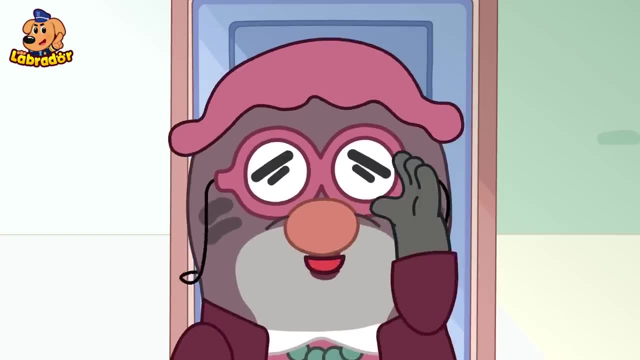 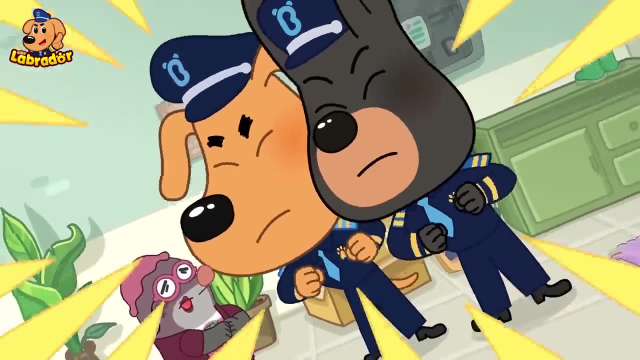 Ms Moore, have you seen Little Cat around? Huh, What was that? She can't hear us well, Hm, Is Little Cat home now? Ah Oh, I saw Little Cat entering his house with Weasel And he didn't look like a nice guy. 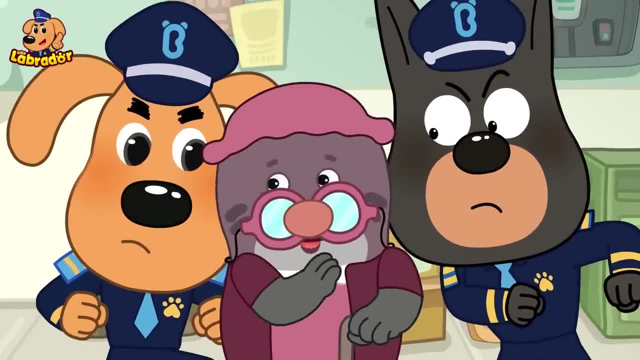 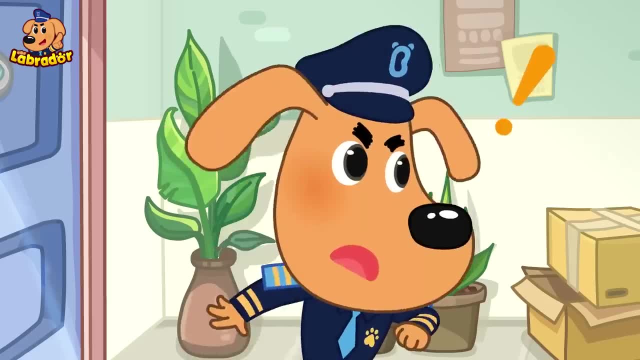 Hm. Oh no, Dobie, Little Cat's in danger. What, Ms Moore, Go back to your house. Oh no, Dobie, Dobie, Dobie, Dobie, Dobie, Dobie, It's our home. 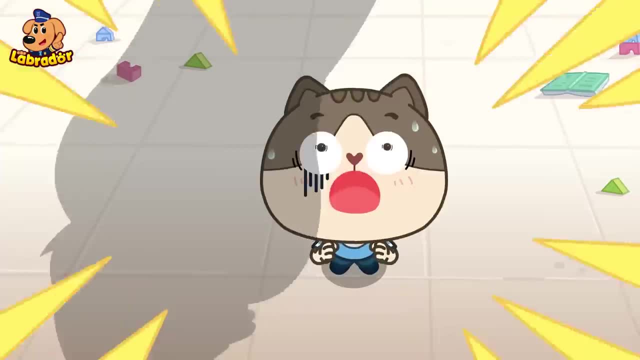 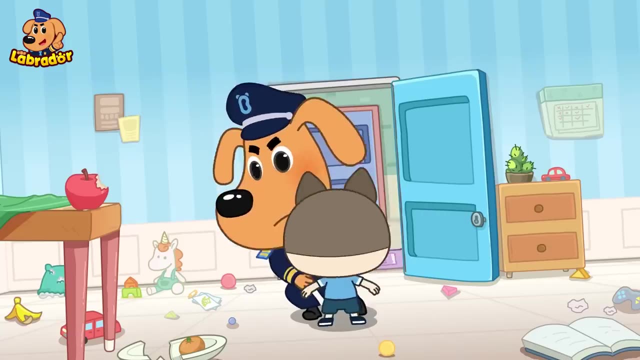 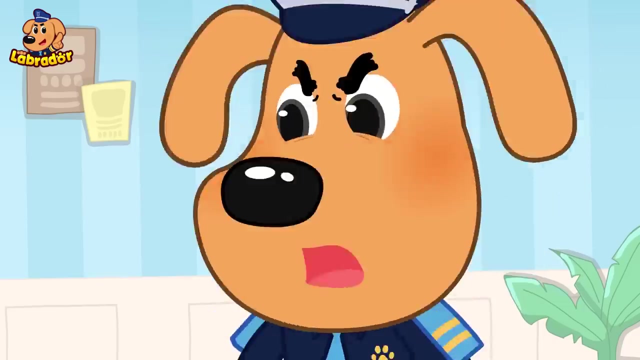 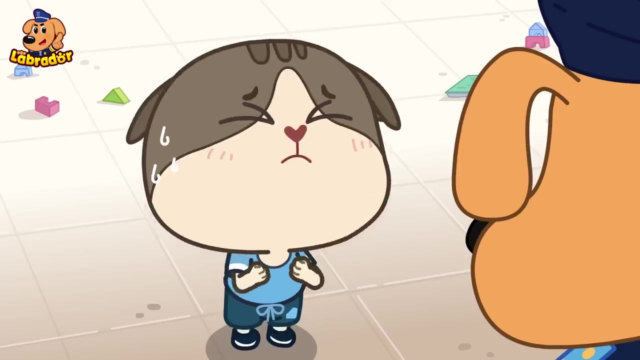 Go back to your house Watch me. Hee-hah. Ah, Ouch, Are you all right? Little Cat, Nyeh, Little Cat, was anyone else here with you? No, But Ms Mole said you came home with someone. 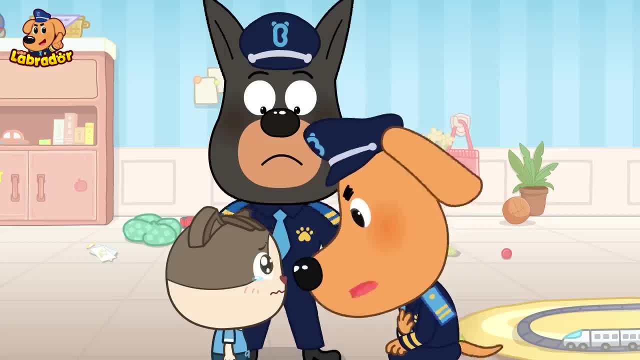 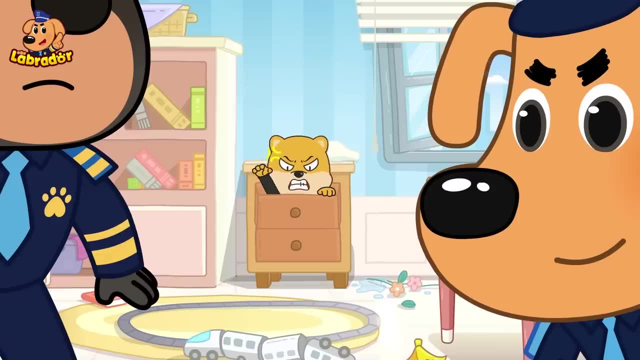 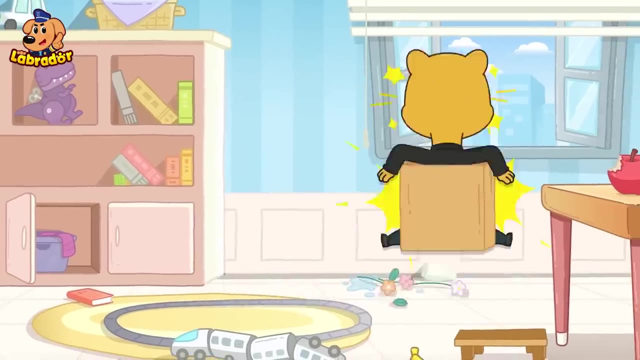 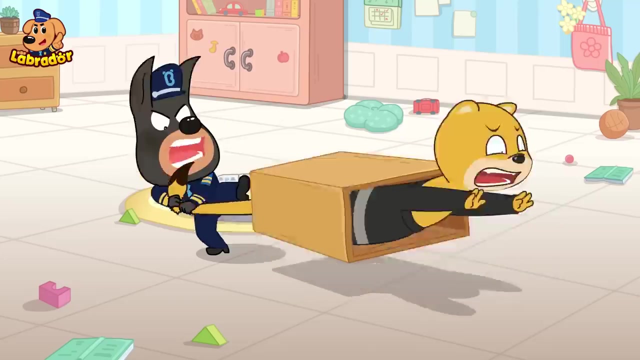 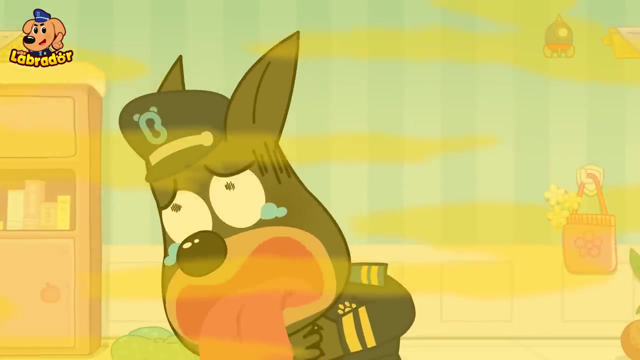 Don't be afraid, little cat. If you're being threatened, you can tell us I, He's right there. How dare you say that, little cat? Oh, I got you. Hey, You think you can catch me? It stinks. 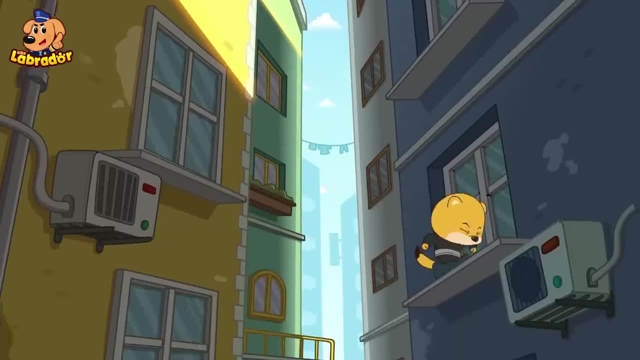 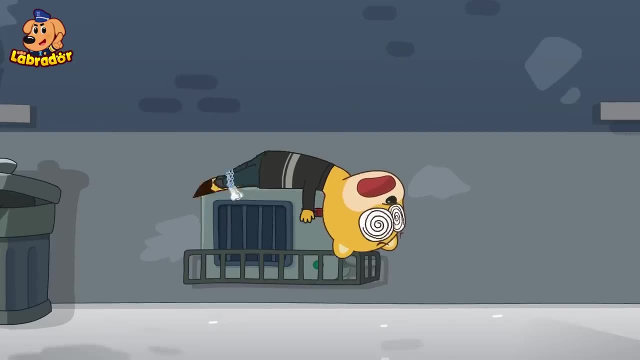 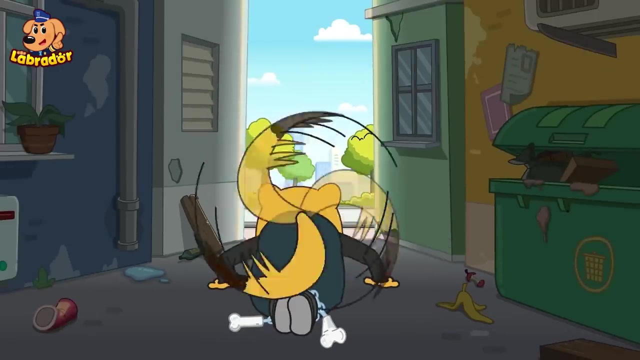 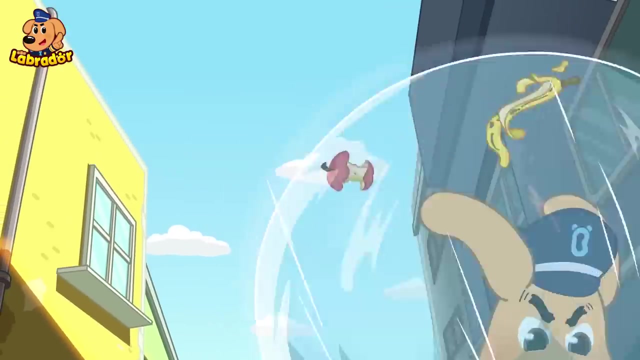 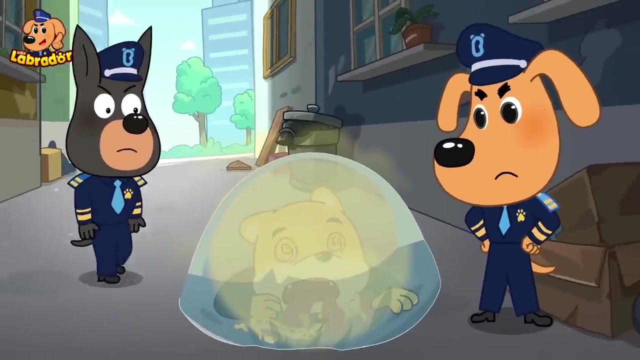 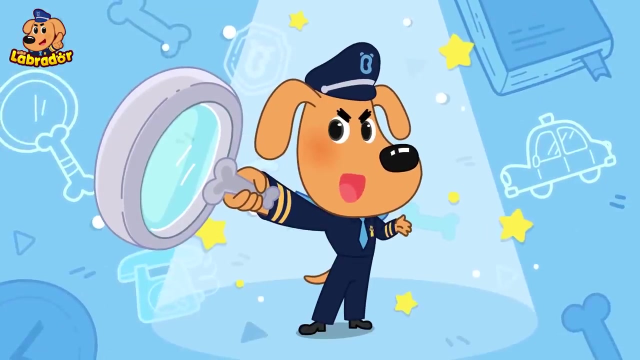 Stop Bye-bye. Hey, Stop right there. Have a taste of my stinky fart. Move aside, Toby. Hey, Ha, It stinks. Help me. Help me, Sheriff Labrador's Safety. Talk, Kids, if you happen to find out bad guys' secret. 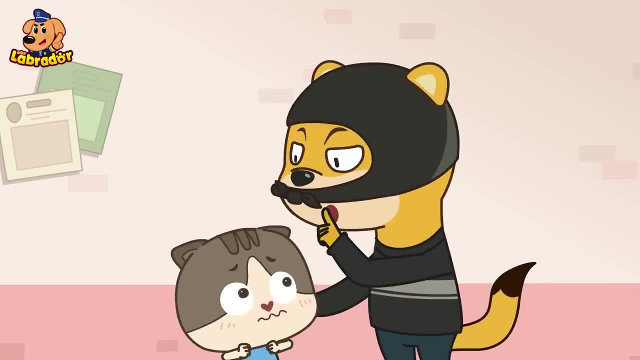 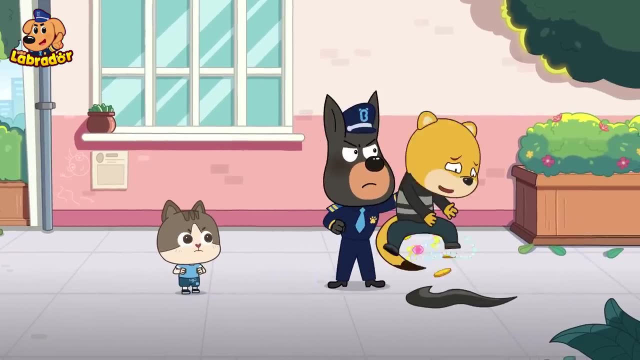 get away from them right away If they threaten you to keep the secret, don't be afraid and don't listen to what they say. Find your parents or the police right away and ask for help from them. Please remember that, Woof. 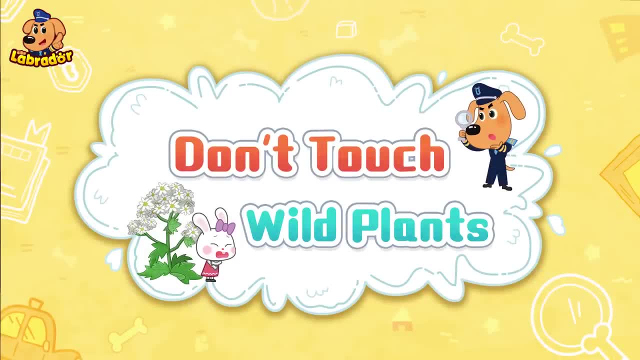 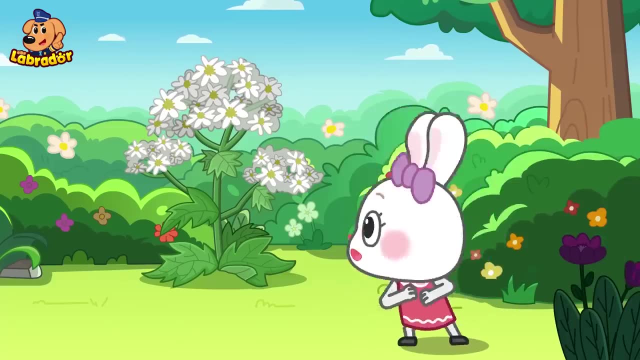 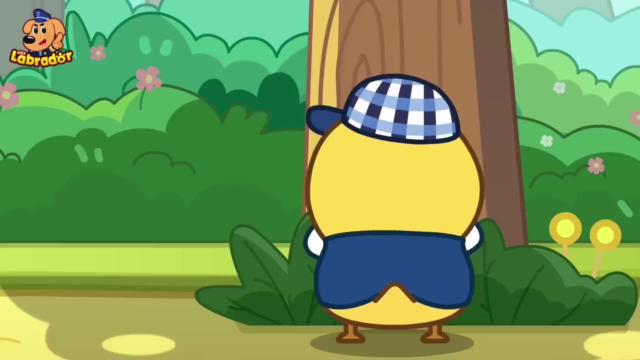 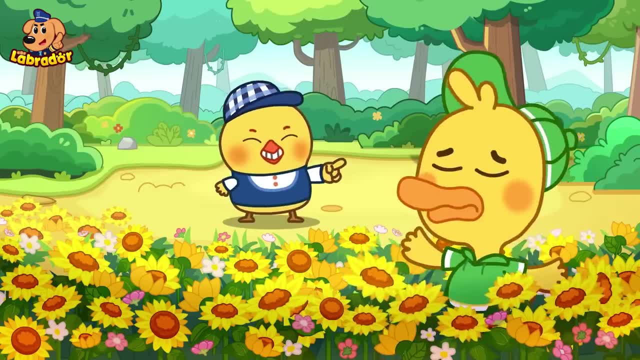 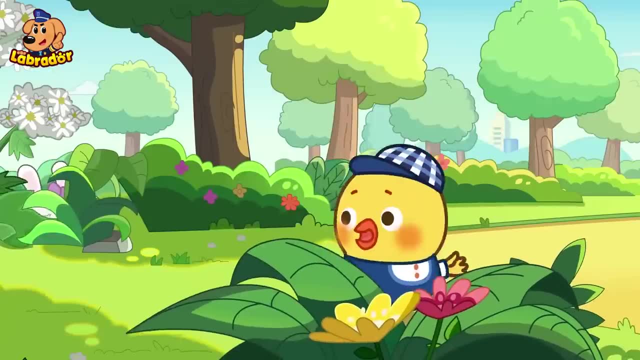 I'm ready, Ah, I'm coming. Look out, Go Watch out. I found you, Ah. Ah, I found you too, Coming for you, little rabbit. Ah, Found you, Huh, Ah, Little rabbit. what's wrong? 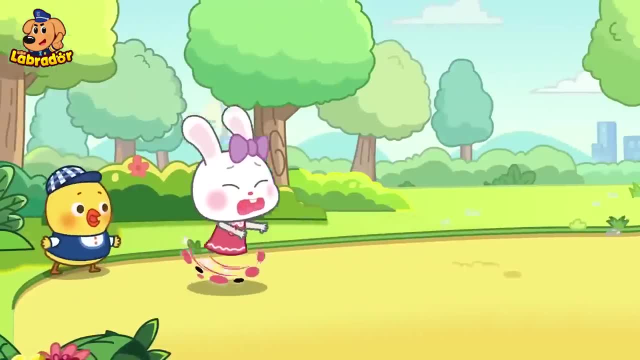 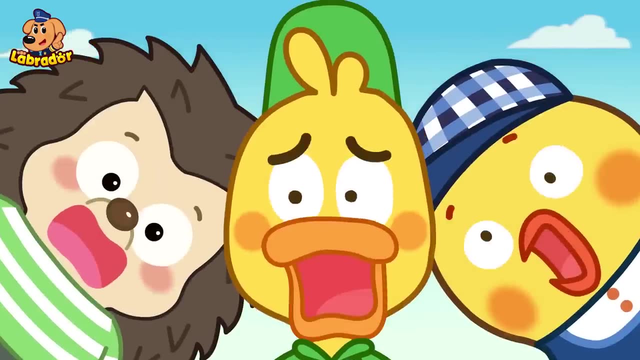 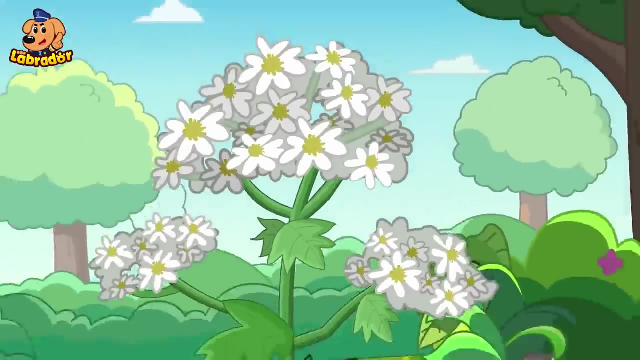 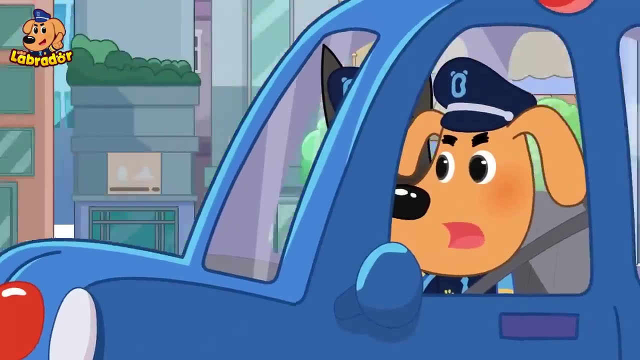 Ah, So itchy, I'm so itchy. Ah, My hand hurts. You don't think I have time for that. Huh, Huh, I think I got bit. Oh, It's a monster Run. Something's going on. 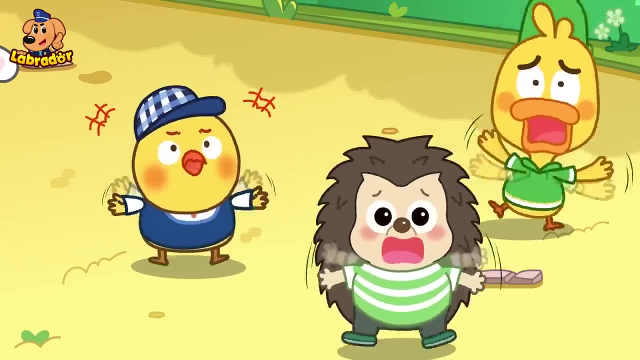 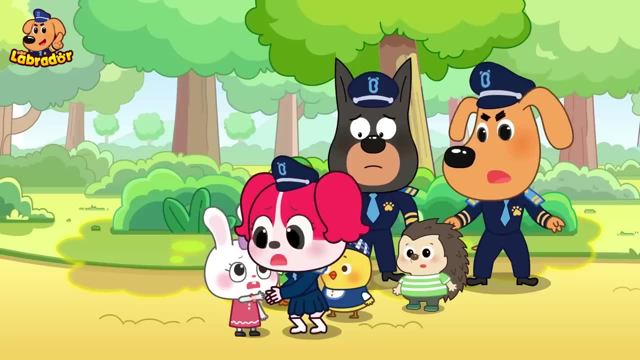 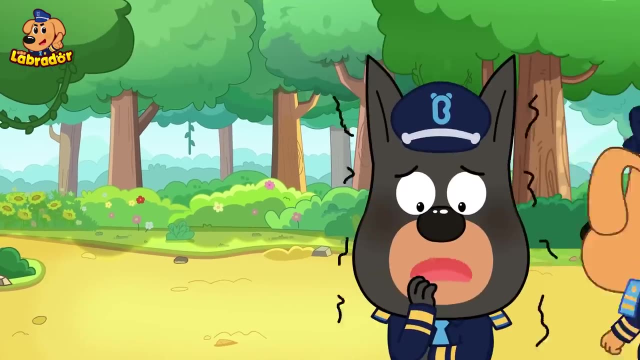 What's wrong, kids? Sheriff Labrador, there's a biting plant over there And it bit Little Rabbit. Let me have a look. He looks serious. I'll take her to the hospital. So biting plants are real. Toby, let's go have a look. 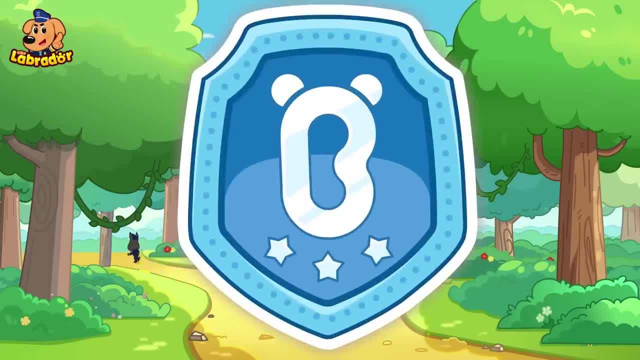 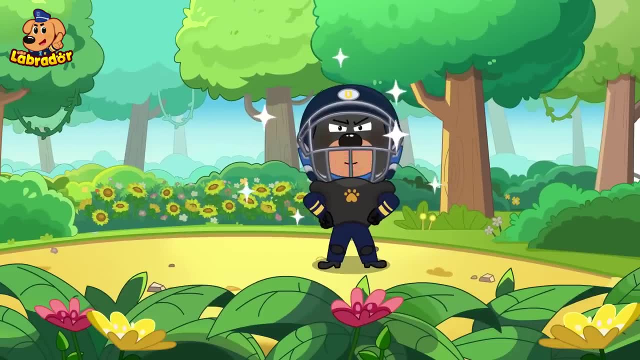 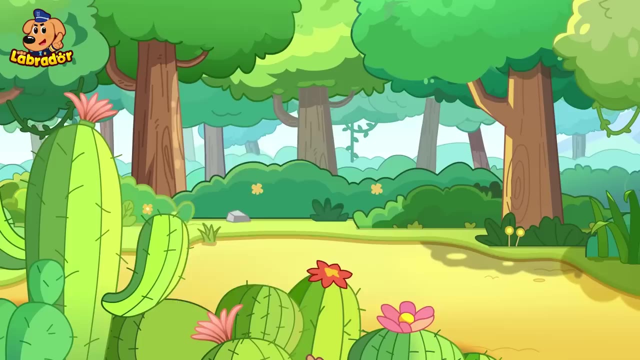 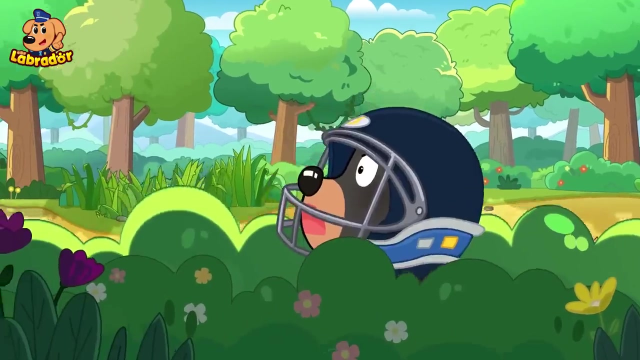 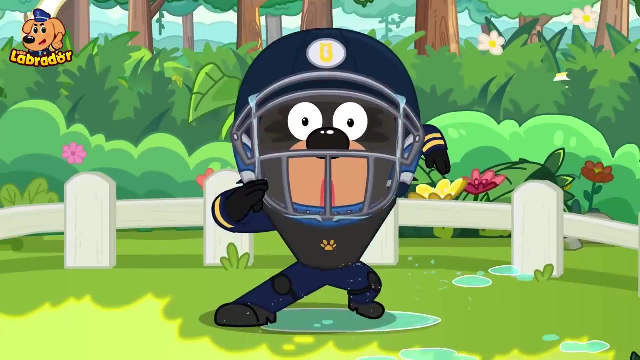 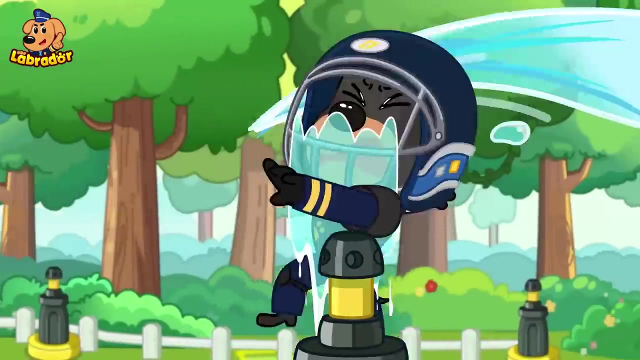 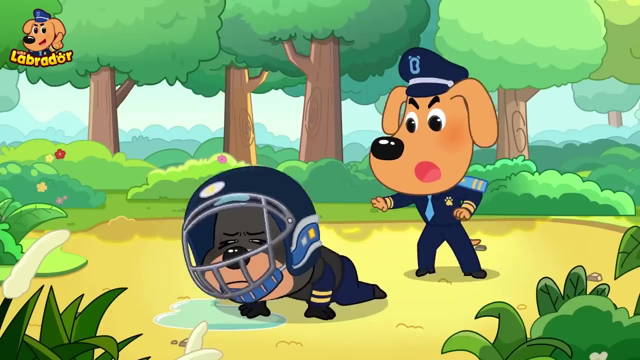 Wait for me. Now. nothing can bite me. Let's go look over there. Okay, Where is it? Huh, Found it. Hey-ya, They are just sprinklers, Toby, What's going on? There's no biting plant. 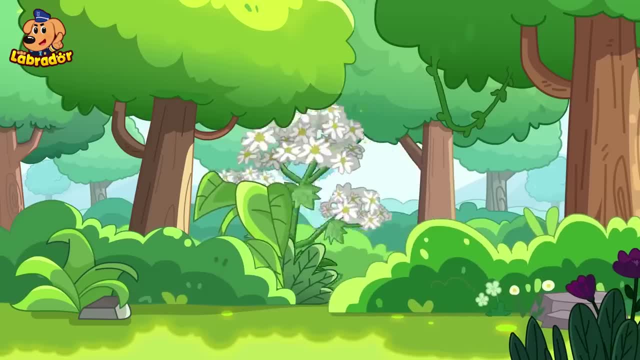 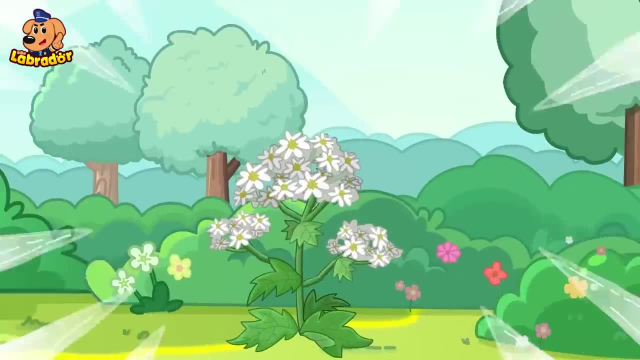 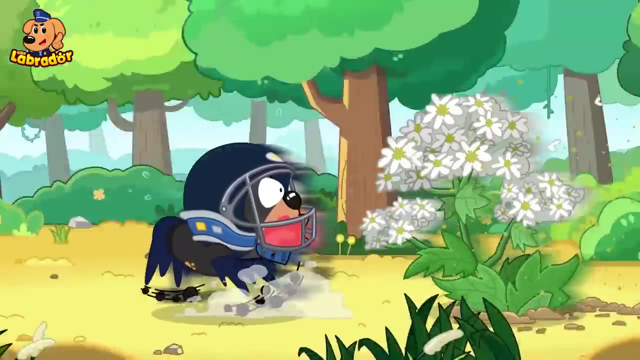 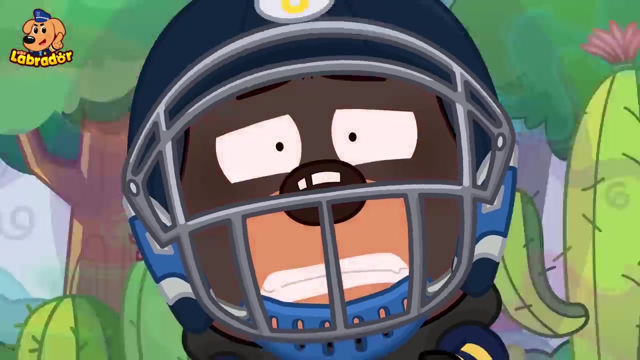 Huh, The biting plant. See my gear, I'm not afraid of you. Hey, It's giant hogweed. Don't touch it, It's toxic. What Toxic That hurts? Ouch, Huh, Ouch. 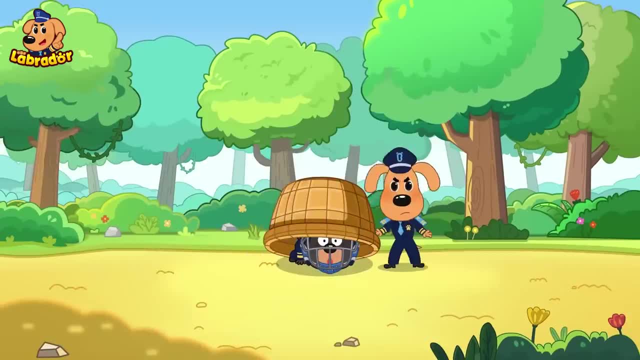 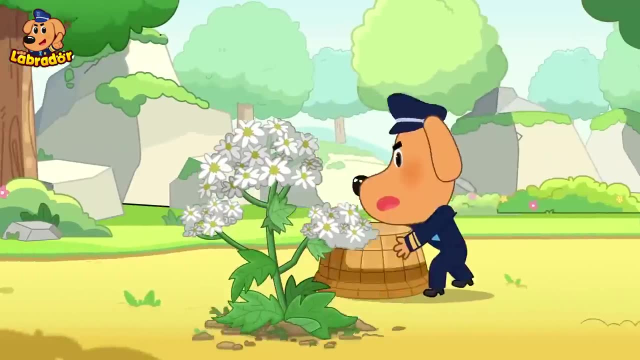 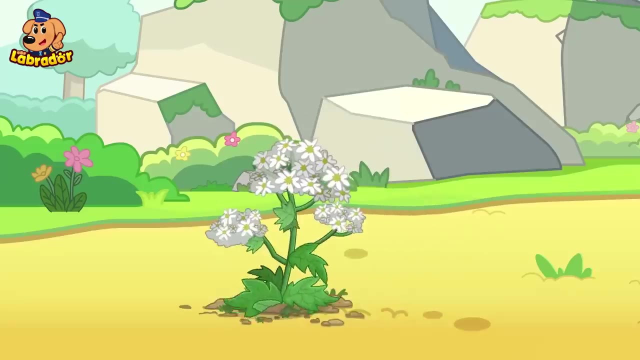 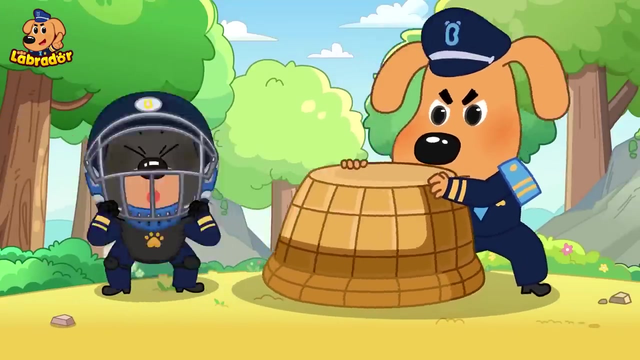 Ouch, Uh, Huh, Uh, Use a basket. Uh, Uh, Hey, Got you Got you. Oh, ouch, Got you Got you. Hey, Hey, Hey, Ey, Hey, Hey, Hey Hey. 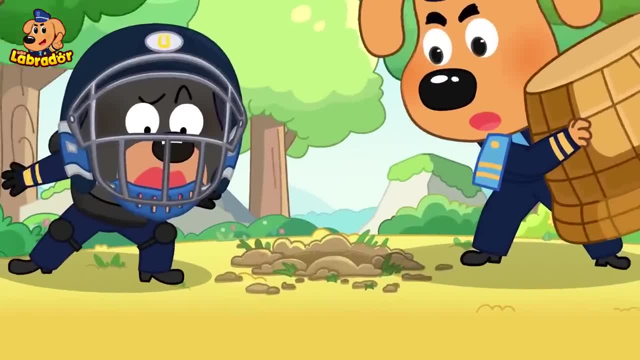 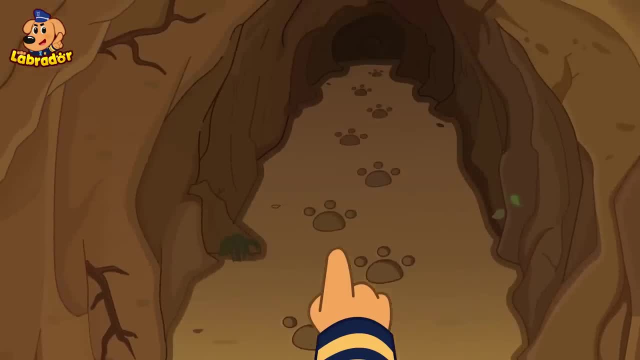 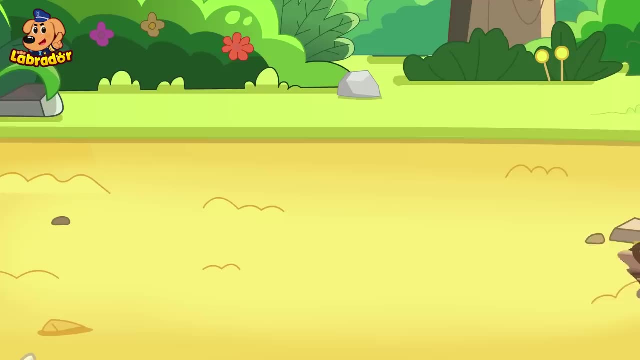 Oh, Finally got it. Huh, How did it dig a tunnel and run away? Look, These are Mr Marmot's footprints. What's going on? I'll go up and take a look. Found it Over there. 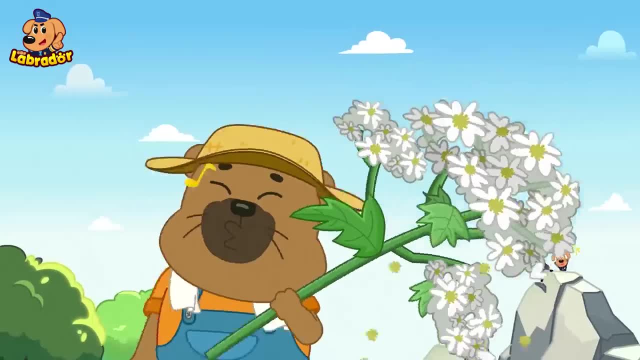 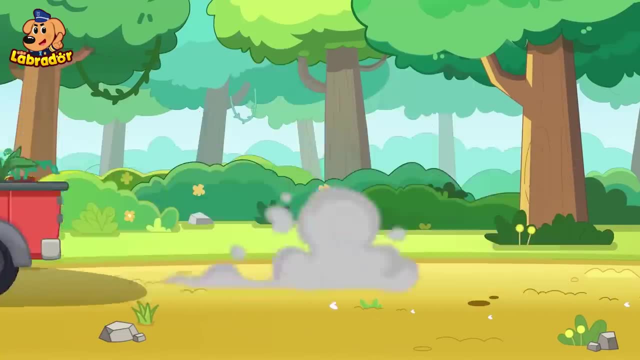 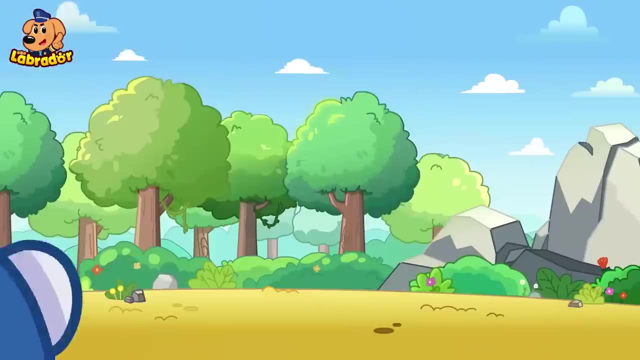 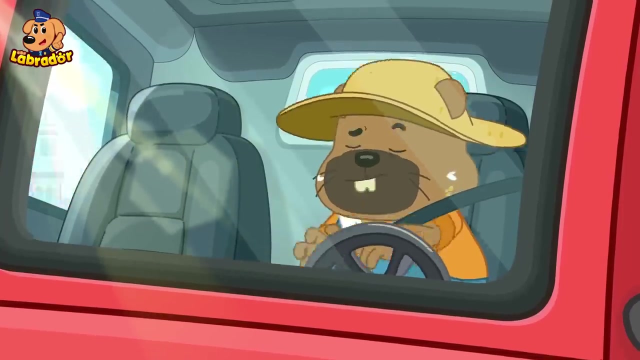 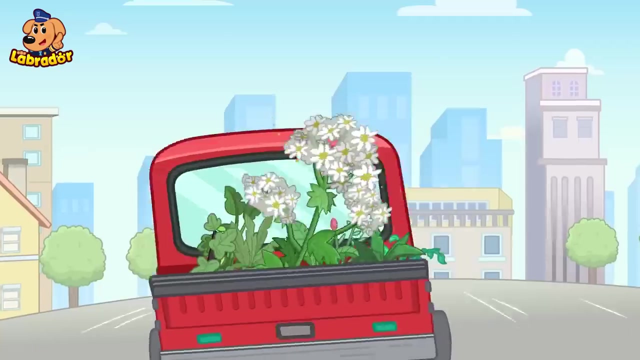 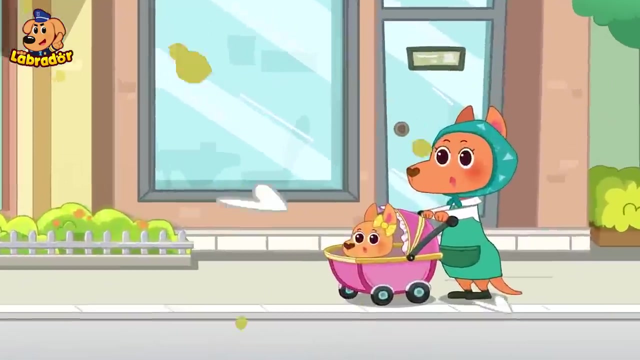 Ah, Mr Marmot, Don't touch that plant. I'm gonna take this beautiful plant home. Uh, We need to stop him. Uh, I'm so itchy. What's going on? Uh, Oh, no, Watch out. 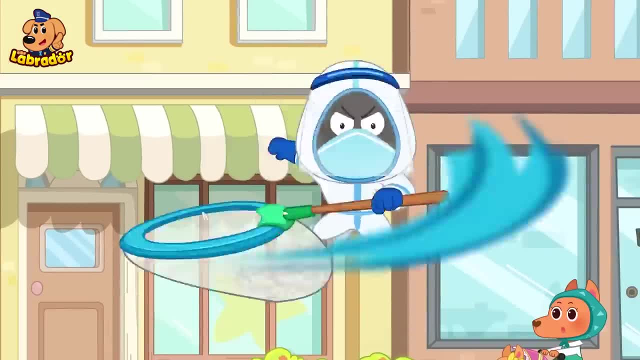 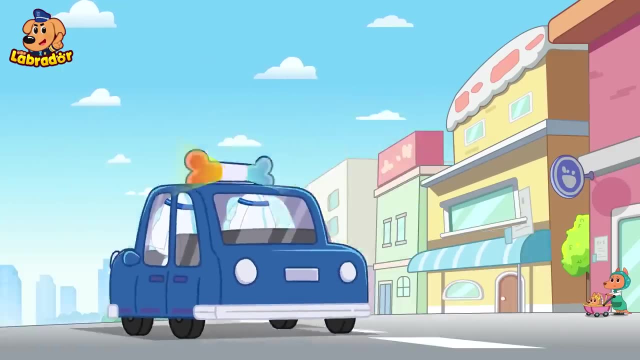 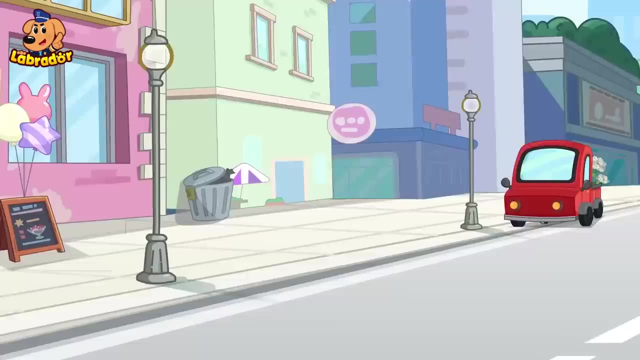 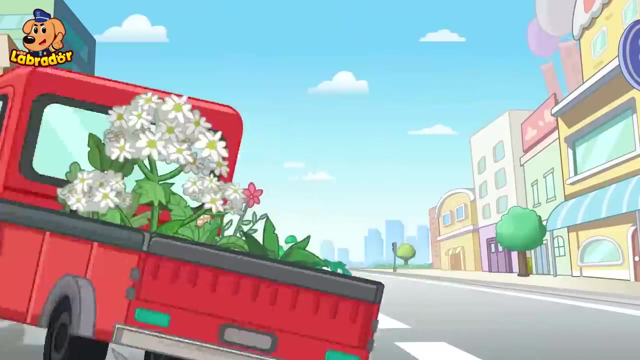 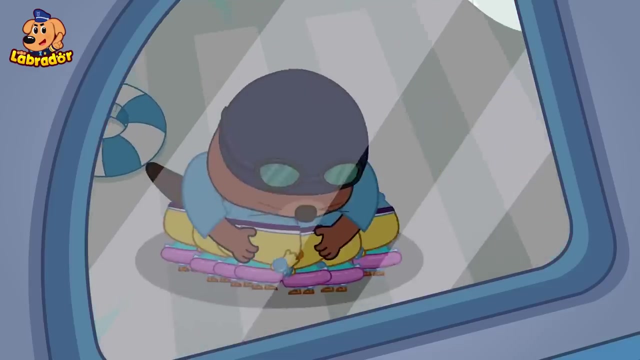 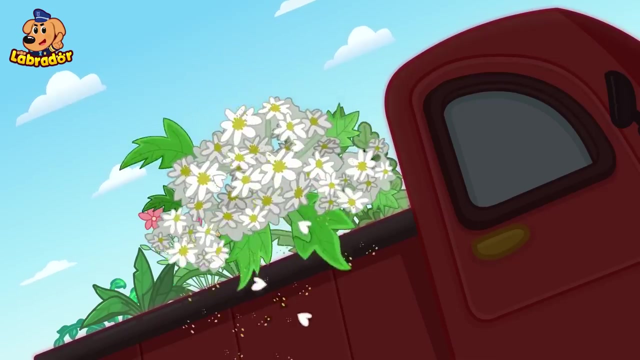 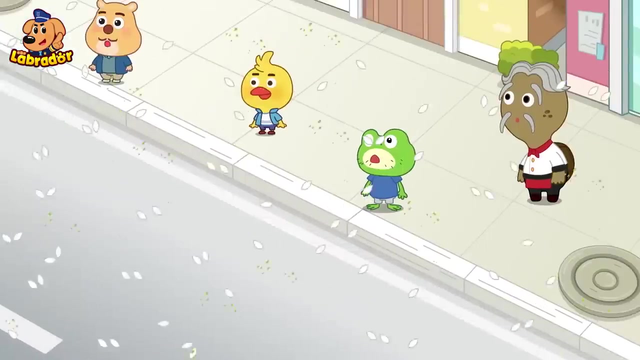 Hey, Ow, I can't stand it. Ah, Pedestrians ahead. One, two, one, Huh Ah, Flying Claws launch. Oh, Huh, Huh, Watch out. Hey, Ah, Oh no. 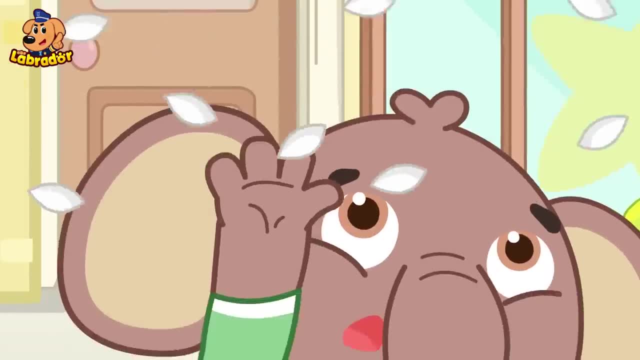 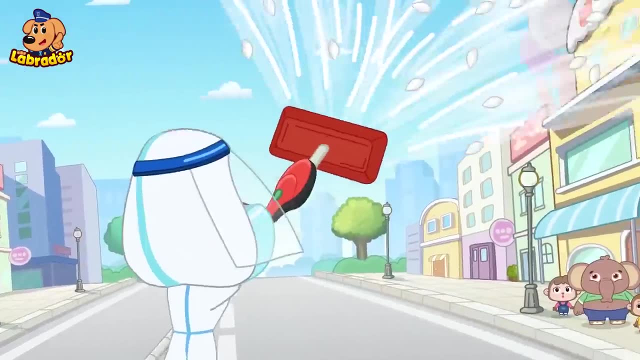 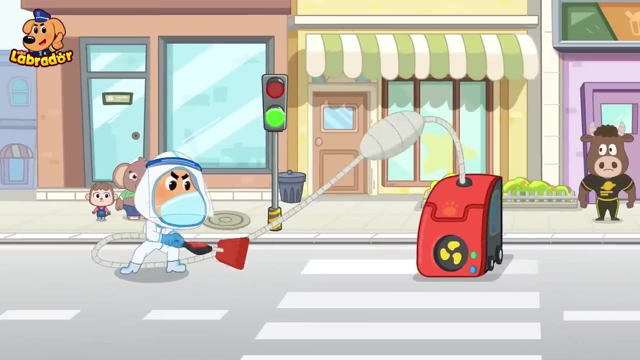 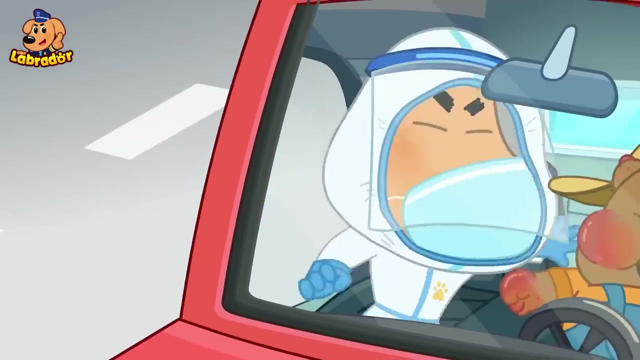 Hey, Watch out, Don't touch it. Oh, Oh, Uh, Huh, Ah, Huh, Huh, Ah, Ah, Ah, Ah, Ah, Ah, Ah. Phew, Mr Marmot, Err, hurry, Take him to the hospital. 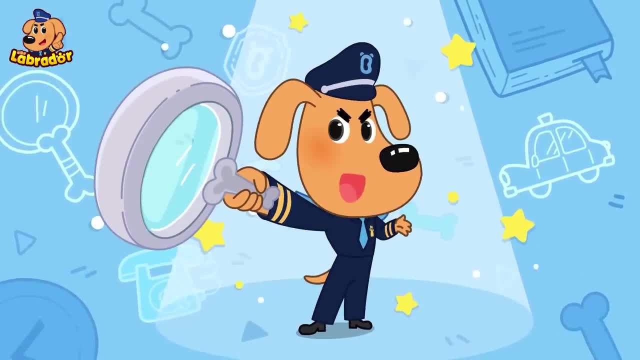 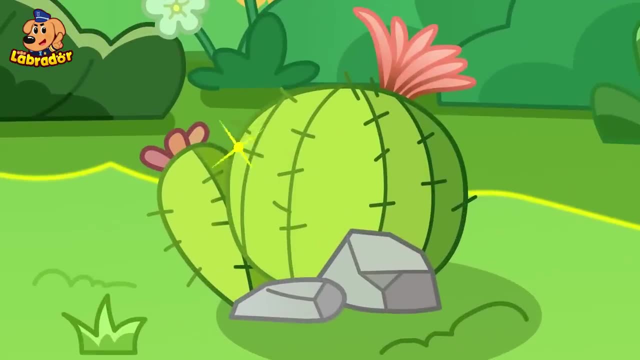 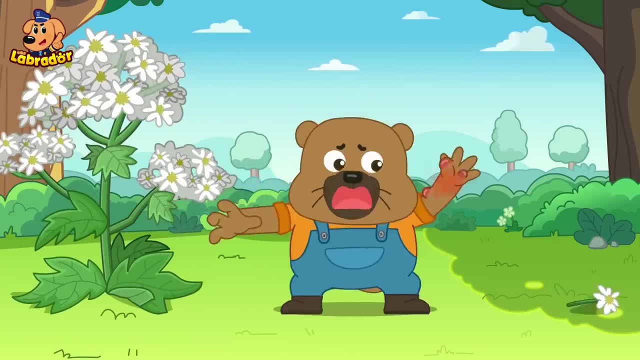 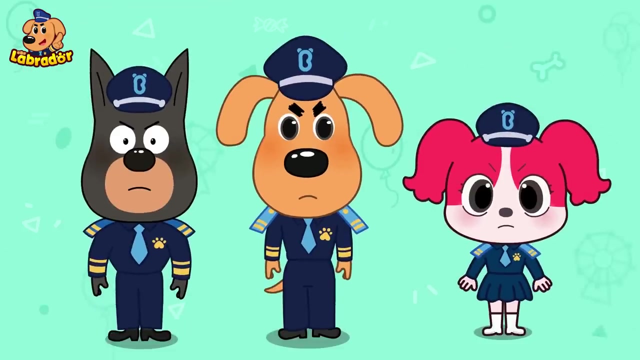 Sheriff Labrador's Safety Talk Kids. there are many different wild plants outside. Some plants have thorns And some plants can be toxic. It's best not to touch them. If you touch them, you might get hurt Or even endanger your lives. Please remember that Life ring for sea safety. 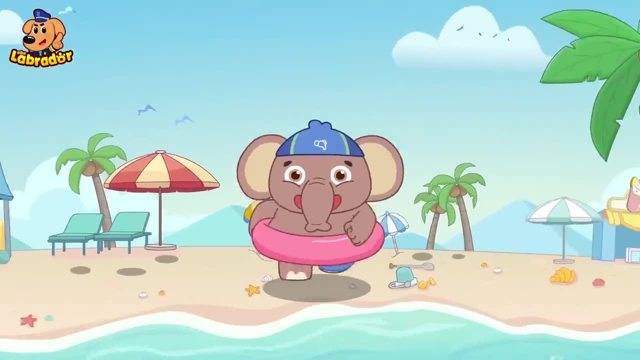 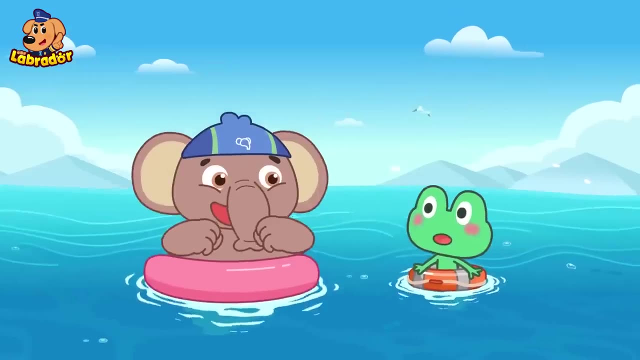 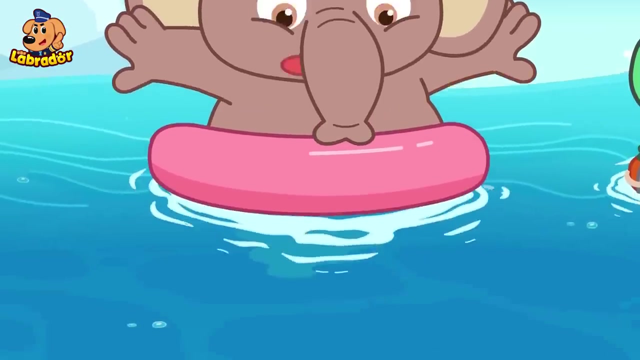 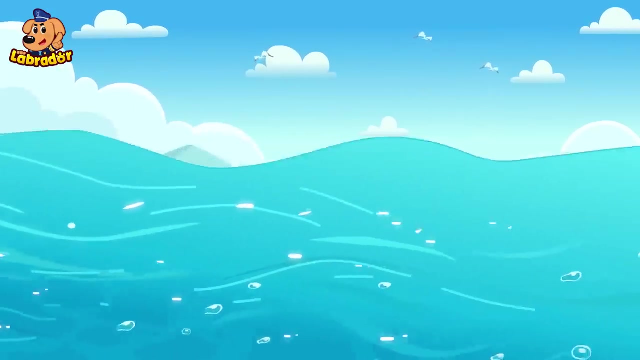 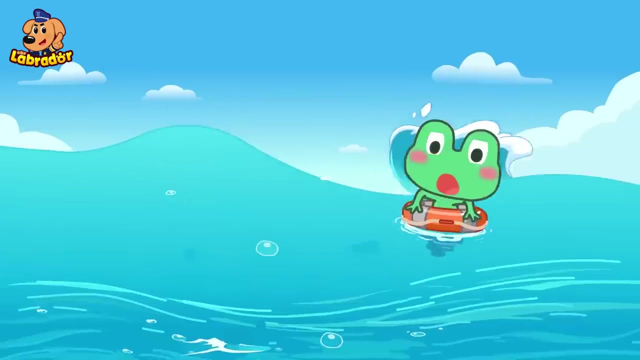 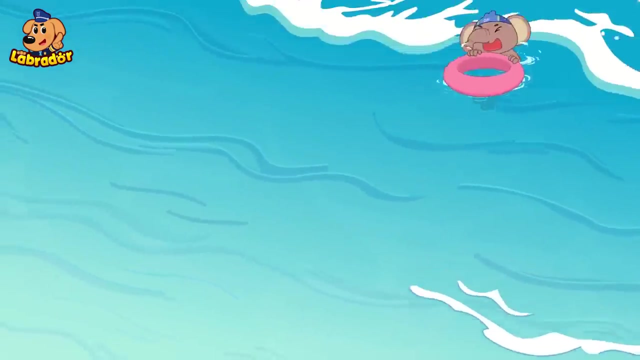 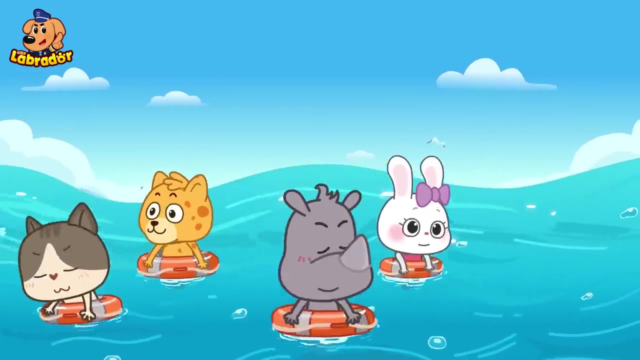 Yay, I'm here, Little elephant, why are you wearing a swim tube? You should wear a life ring in the sea. Huh, They look alike And mine looks better. A fake wave. It's gone. Huh, Where's little elephant? 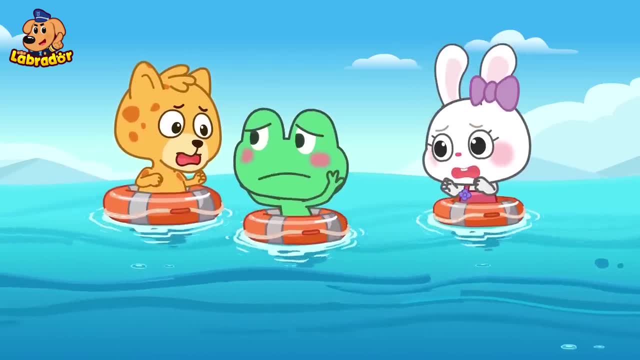 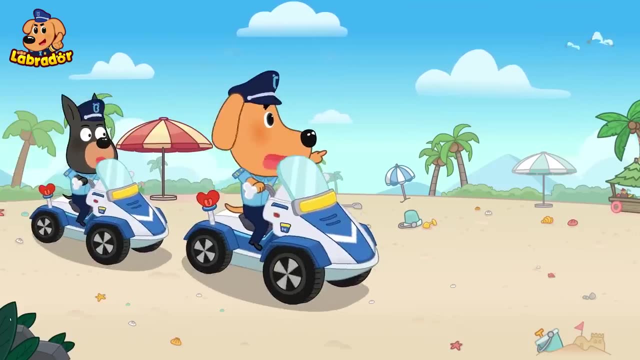 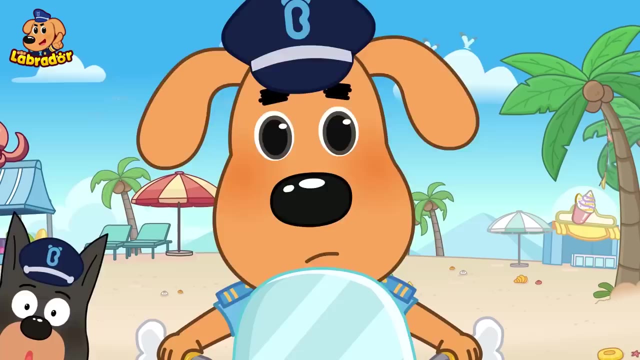 Little elephant- Oh no, Little elephant was swept away by the wave. What My child? Something's wrong over there. Let's go, Sheriff Labrador. My child was swept away by the wave. What Wasn't he playing? in a safe swimming area? 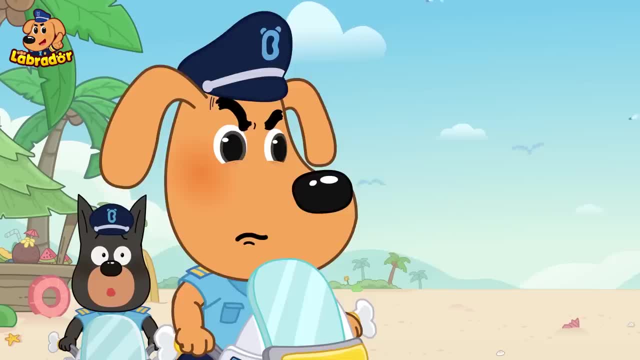 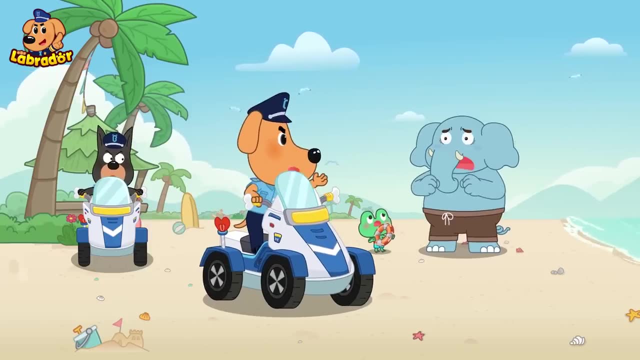 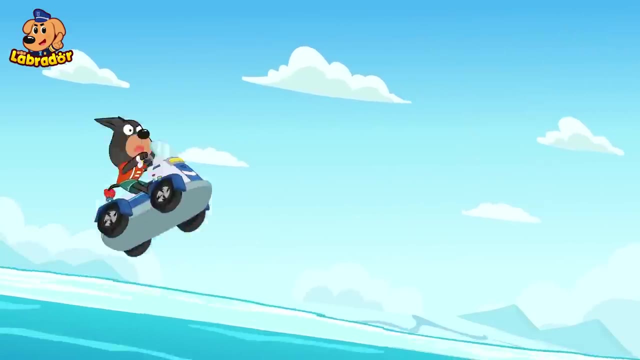 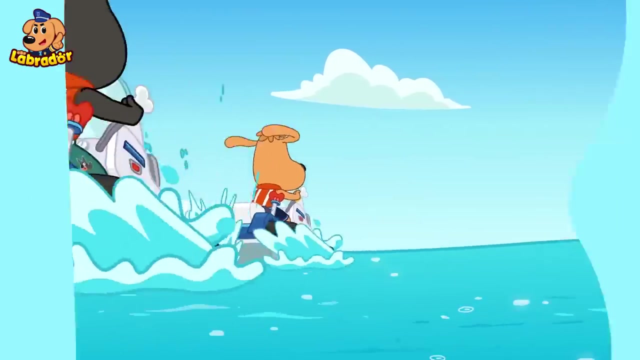 That's right, But he was wearing a swim tube. Swim tubes can easily get swept away because they're so light. Mr Elephant, children should wear life rings when playing in the sea. We'll go find your kid. Oh, My child, Little elephant. 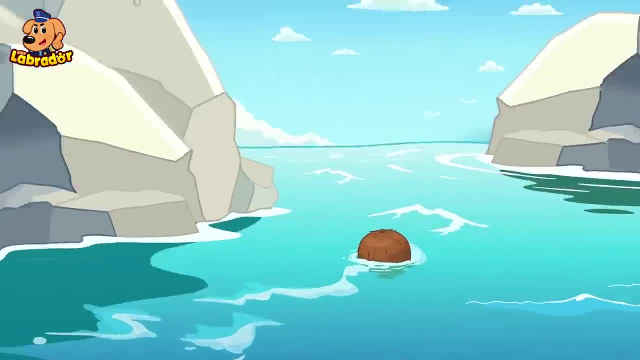 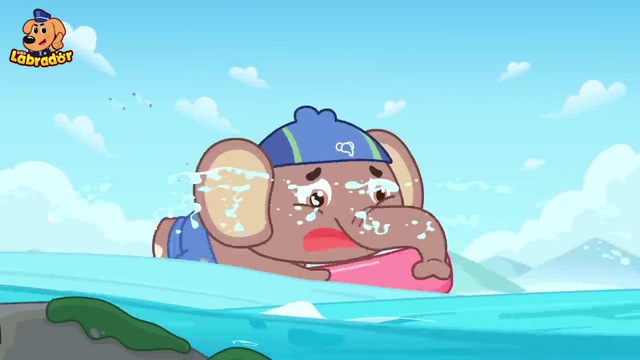 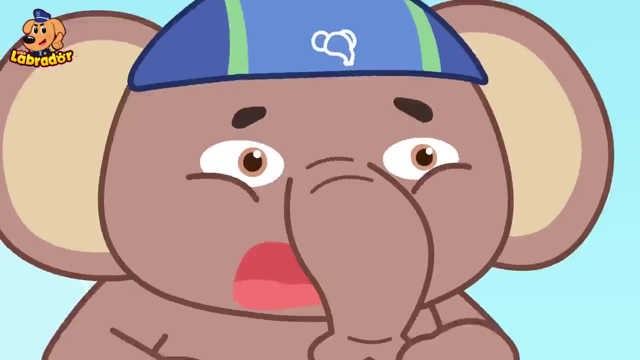 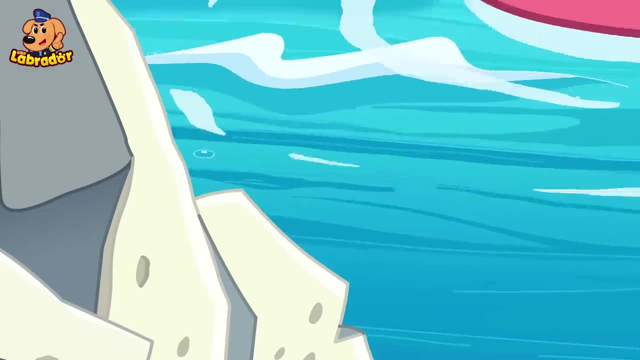 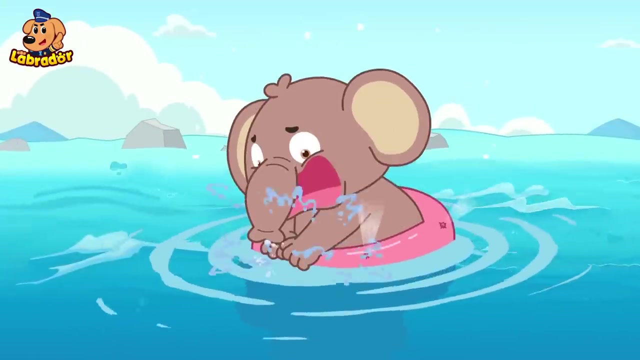 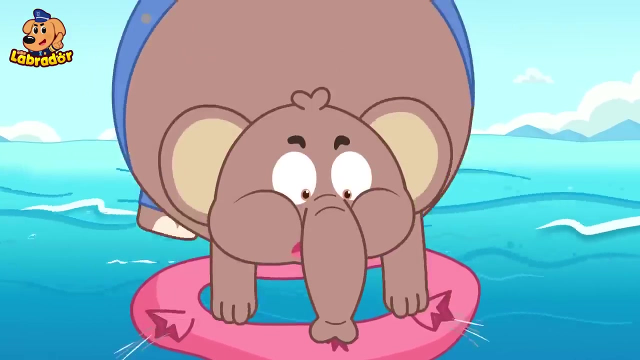 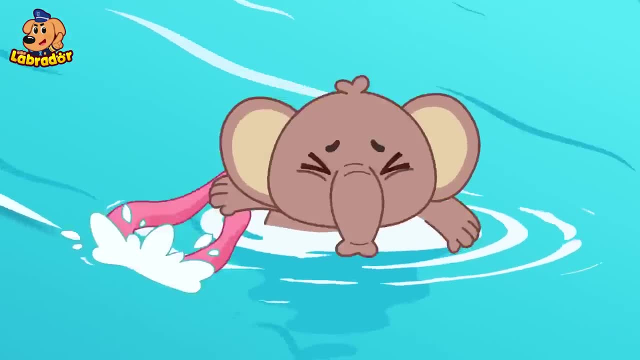 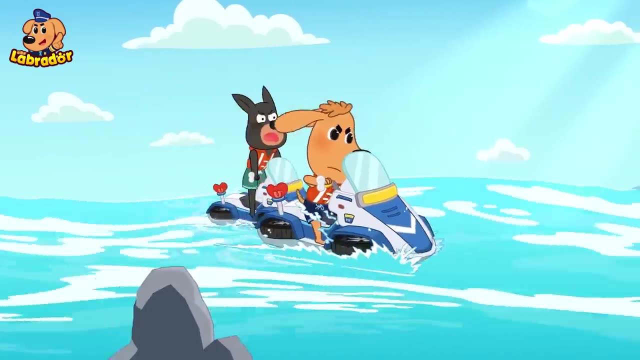 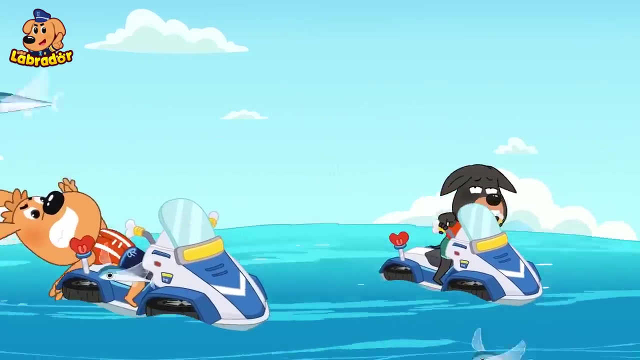 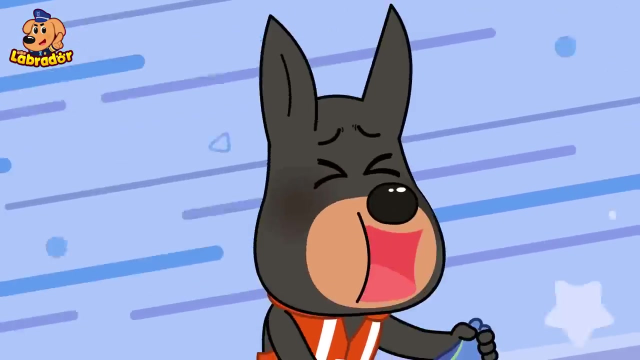 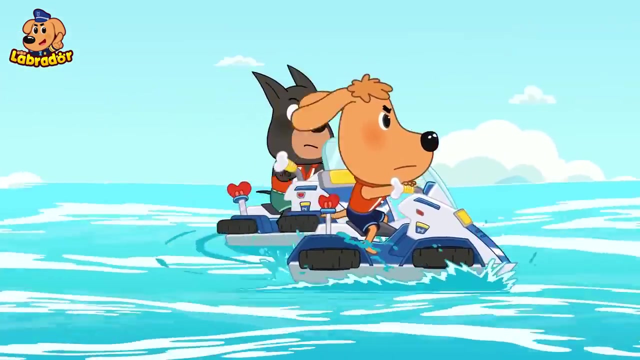 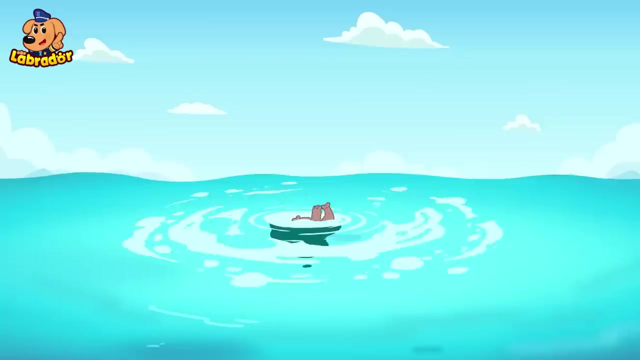 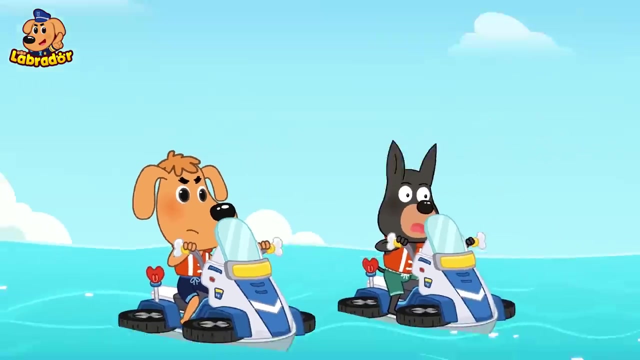 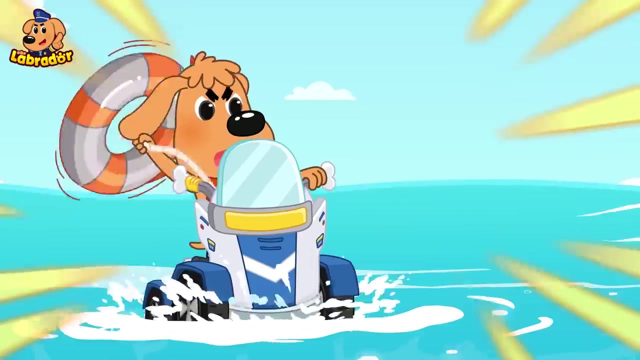 Aaaaah, Aaaaah, Help, Little elephant, where are you? What's this? Look, Huh, Little elephant's swimming cap. Let's go that way. What's that? It's little elephant. Grab the life ring. 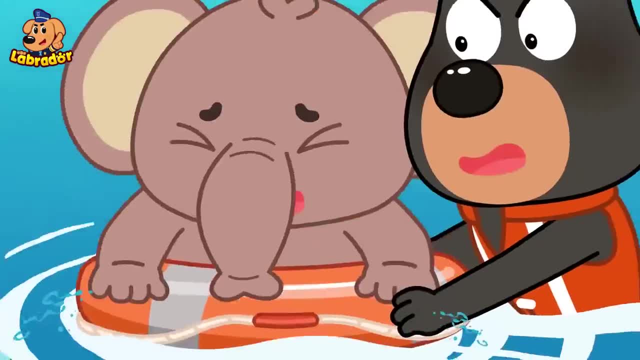 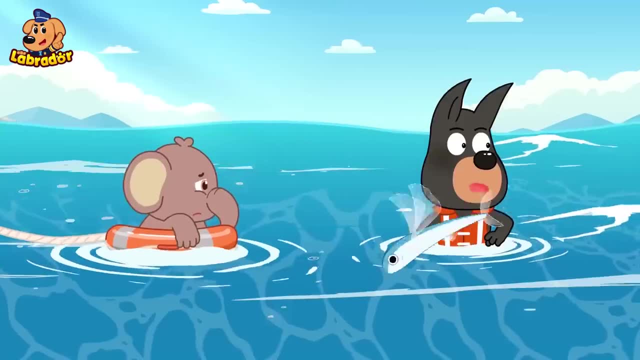 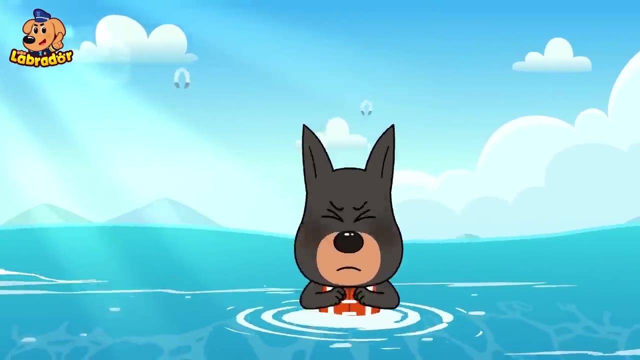 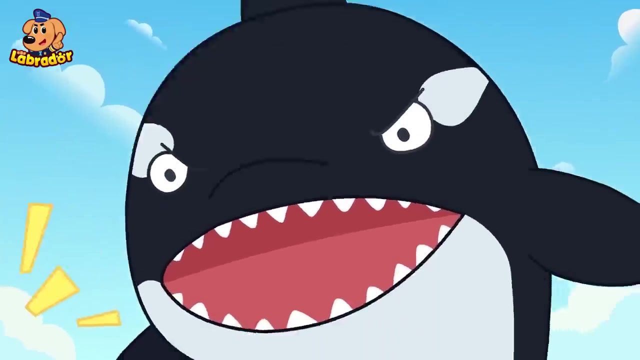 Little elephant. you should wear a life ring when playing in the sea, not a swim tube. I got it Flying fish again. Don't be afraid, I'll keep you safe. Watch out, It's a killer whale, Aaaaah. 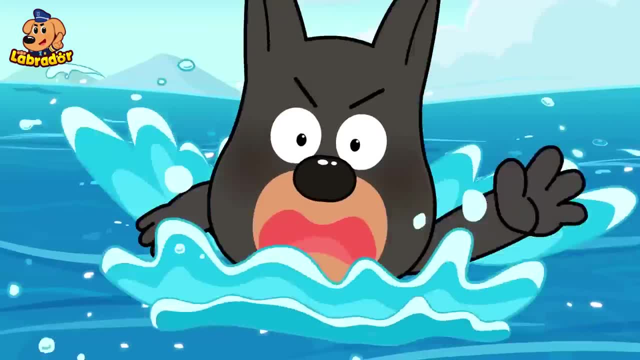 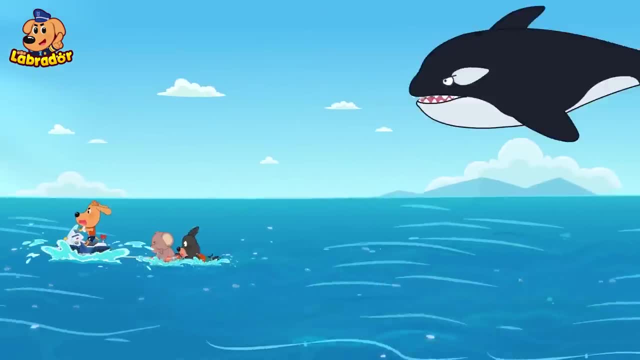 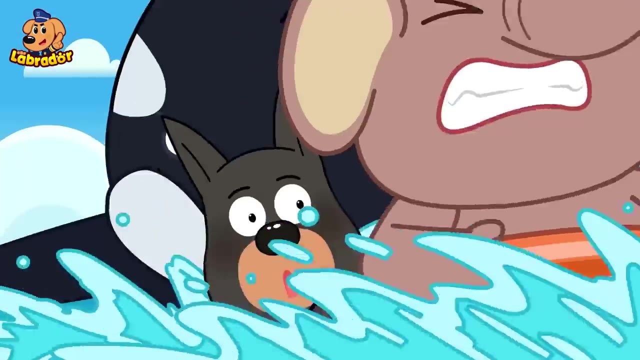 Aaaaah, Aaaaah, Oh, wow, It didn't pop. Let's get out of here. Hold on, Aaaaah, Aaaaah, Aaaaah, Aaaaah, Huh, Hmm, Oh, Aaaaah. 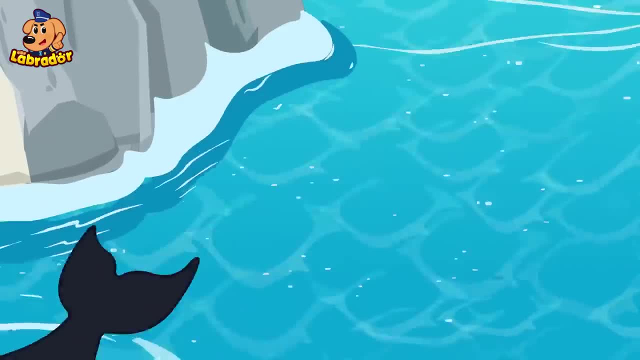 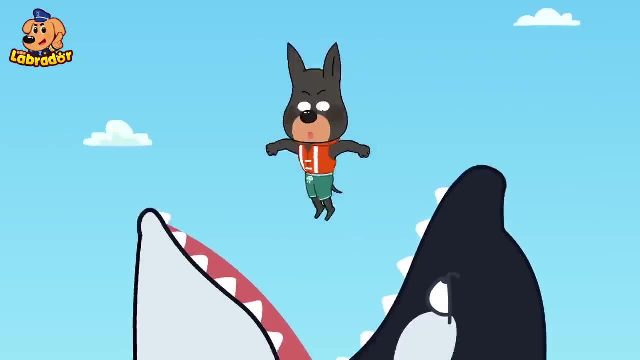 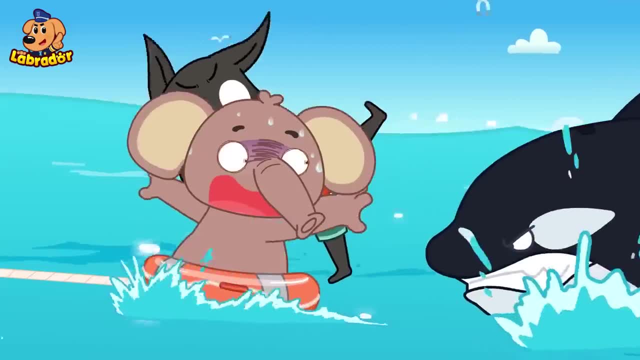 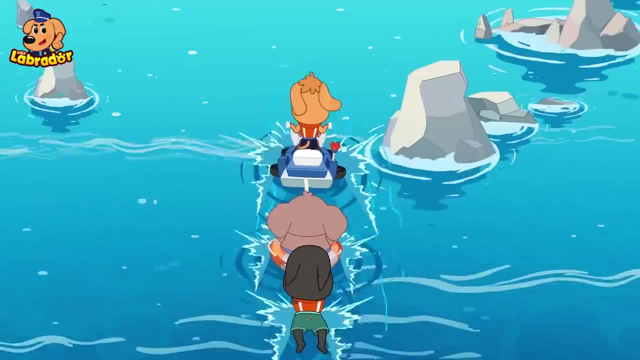 Aaaaah, Aaaaah, Aaaaah, Aaaaah, Aaaaah. What is that? What is that? What did her hide there? Wait a second. Let's use our sharp eyes and alert. She already 몆ed the fan. 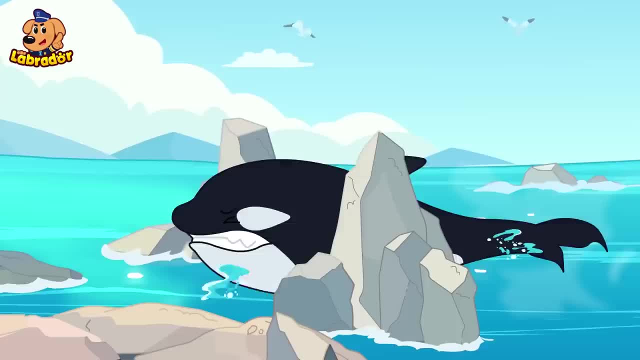 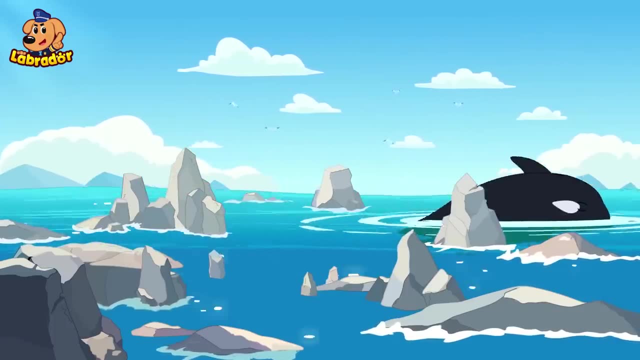 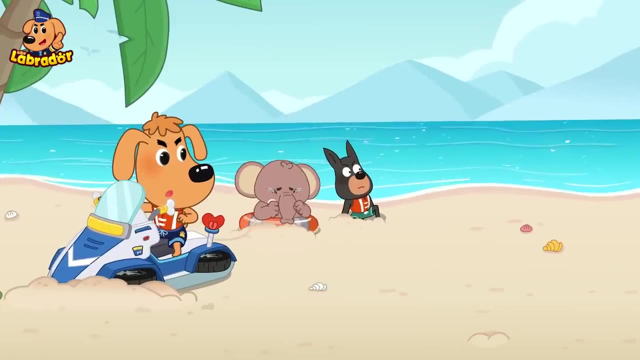 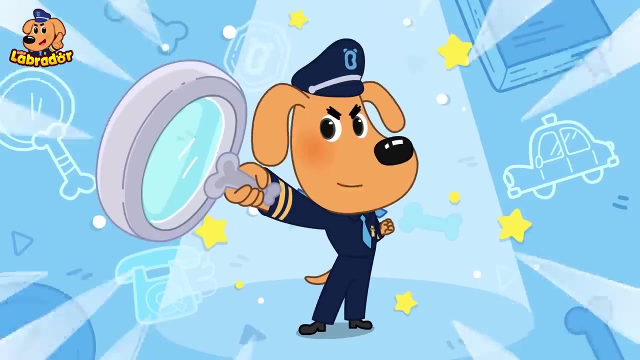 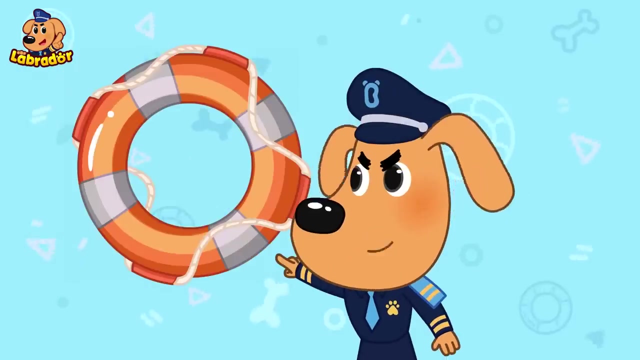 Aaaaah, Someone is there. Aaaaah, Huh, Aaaaah, Aaaaah, Phew, We're safe now. That was so scary, Sheriff Labrador's Safety Talk. Kids, when you play in the water at the beach, you should wear a life ring, not a swim tube. 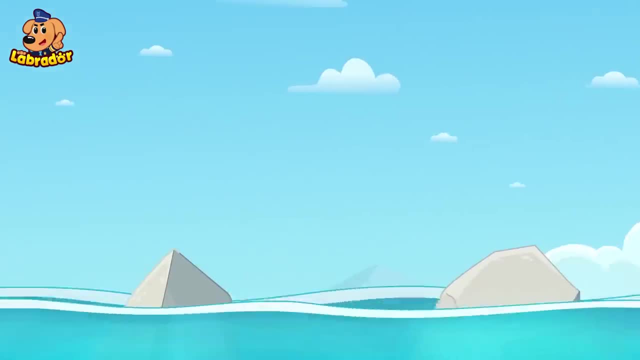 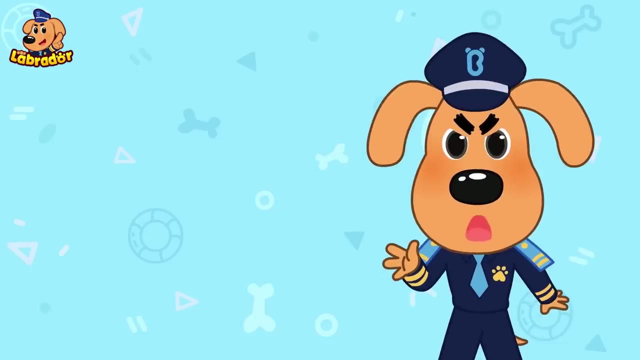 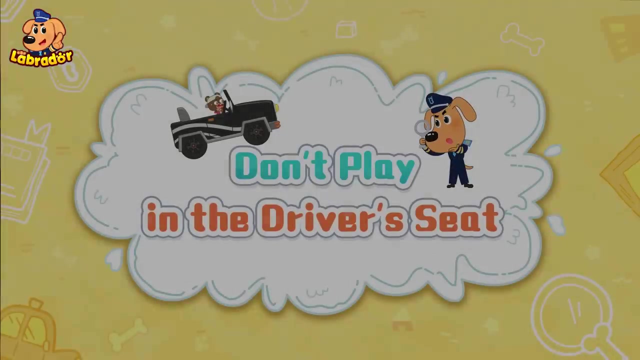 Swim tubes are toys for water play and they're very thin. They can leak easily or pop, and can even be washed away by waves, which is very dangerous for you. So please remember to wear a life ring in the sea. Don't play in the driver's seat. 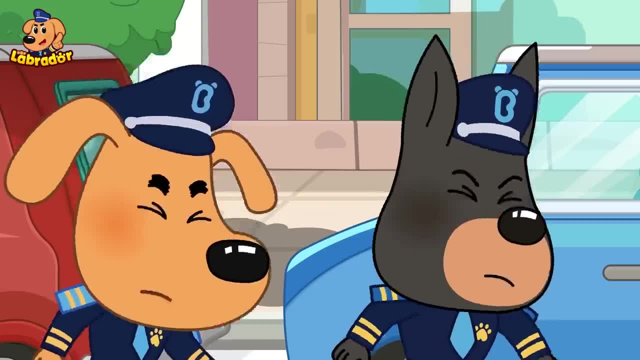 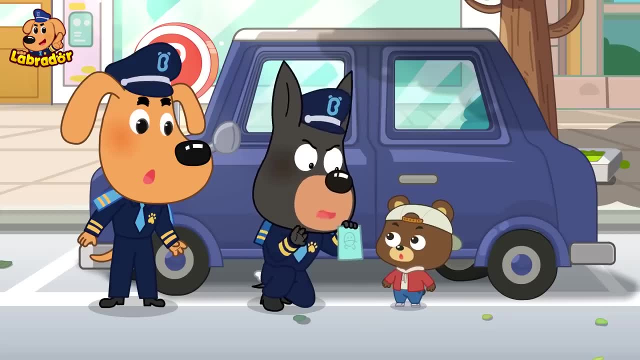 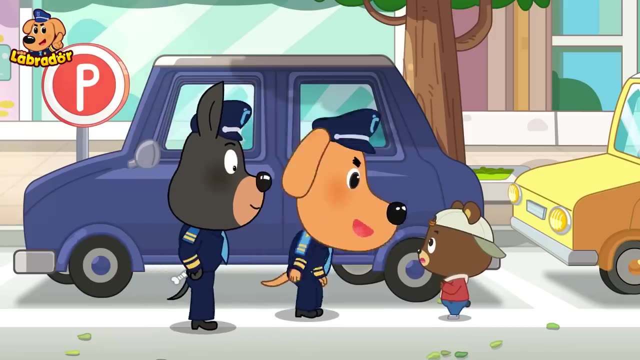 Hey, parking here, You'll get a ticket. Haze, Stop, Little bear. you shouldn't stick things like this on cars. I'm sorry, It's dangerous to be outside by yourself. Come on, we'll take you home. 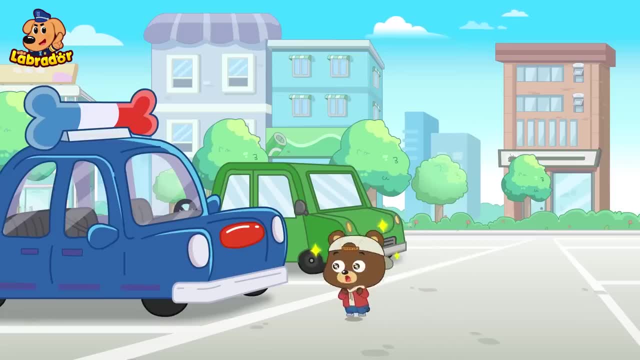 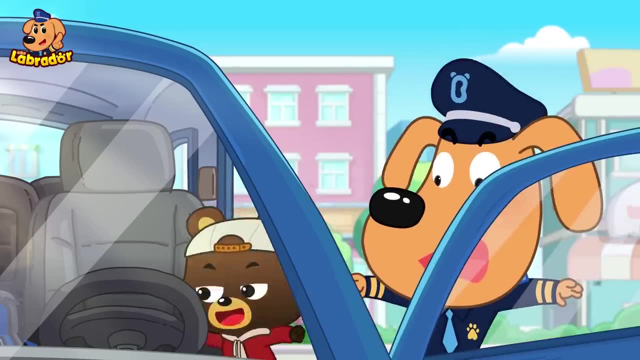 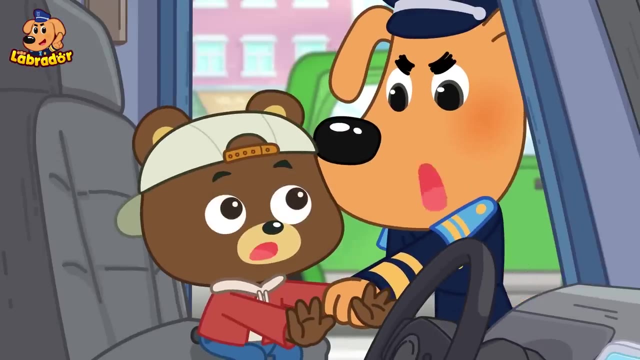 Whoa Awesome, I get to ride in a police car. Yay, Hey, Whoa Go police car. Stop, You shouldn't sit in the driver's seat. It's very dangerous. Okay, Then I'll sit here. 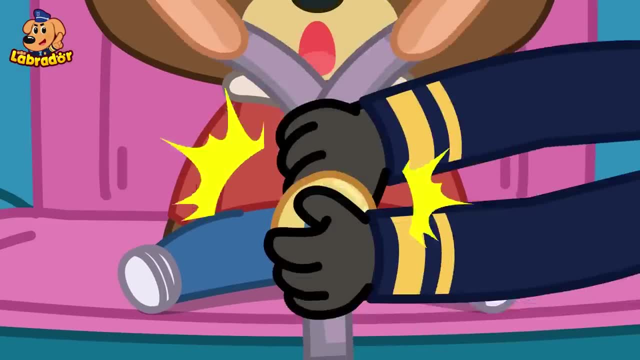 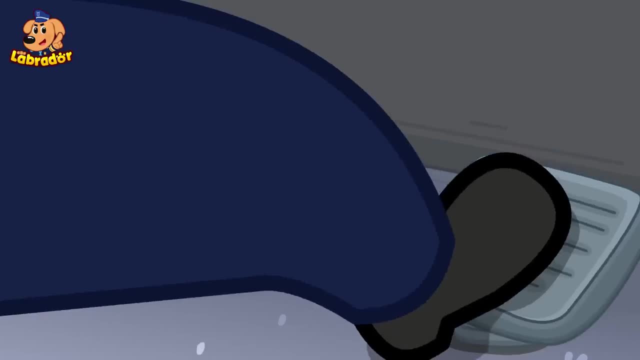 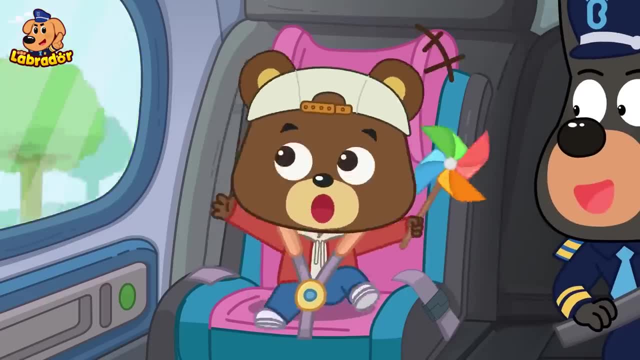 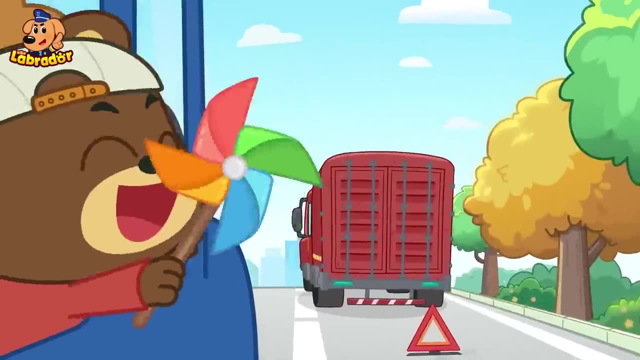 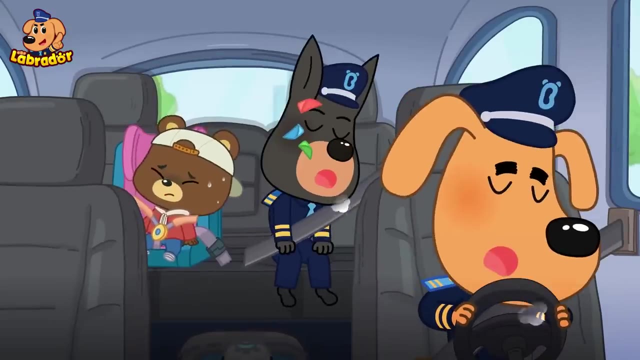 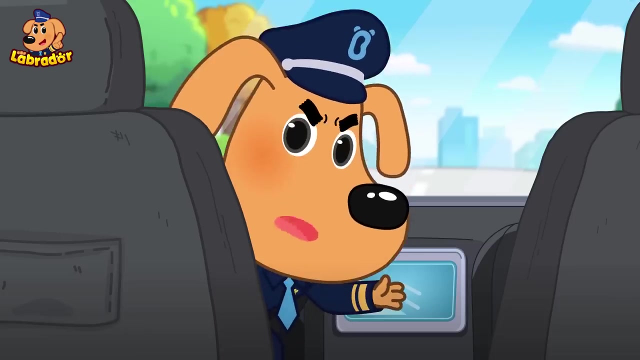 Too much of a Lost. the king, I was scared-. I was scared- Little bear, I was scared- Little bear, You should never stick your head or arms out of the window. That was really close. That was really close, Good. 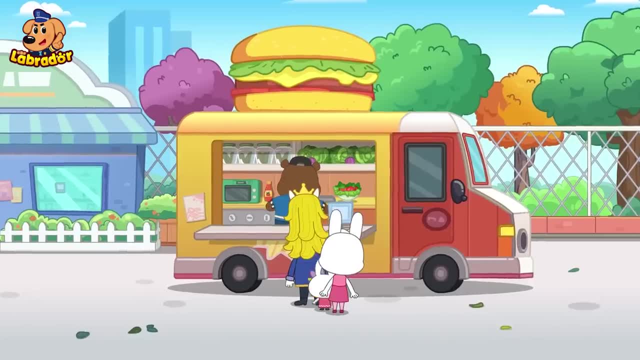 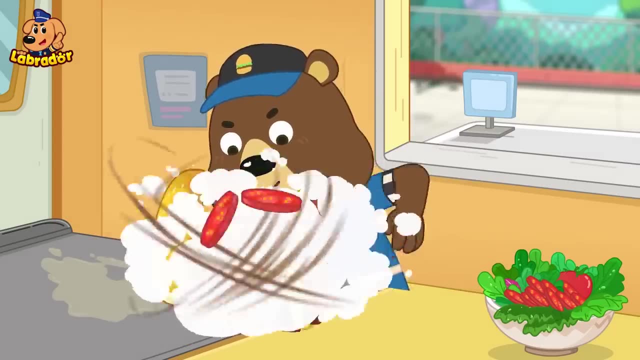 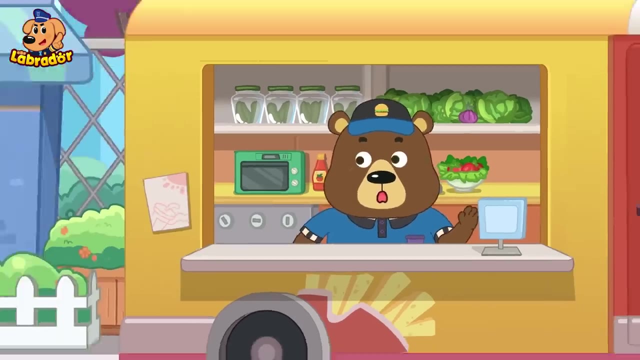 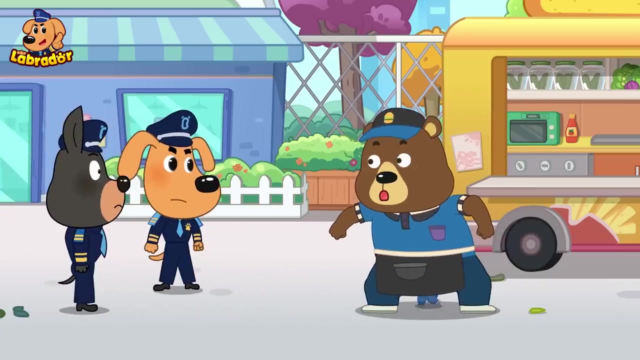 That was really close. I got you, I-I got it Here. Two burgers, please. Alright, Here you go. Wow, Thanks Bye, Daddy. Daddy, Sheriff Labrador, why is my son with you? Mr Bear, it's dangerous for Little Bear to play outside alone. 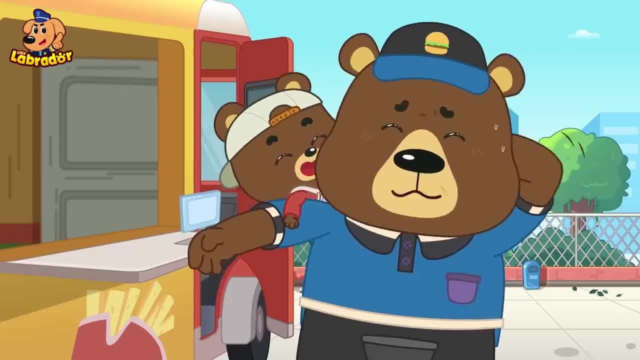 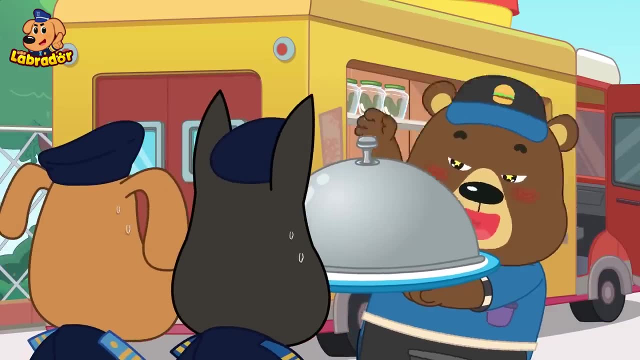 Please be careful. Sorry, I was so busy today I didn't keep an eye on him. Oh, Thank you for bringing him back. Please try these, my special burgers. They're really good. Wow, Such big burgers. No, we're alright. 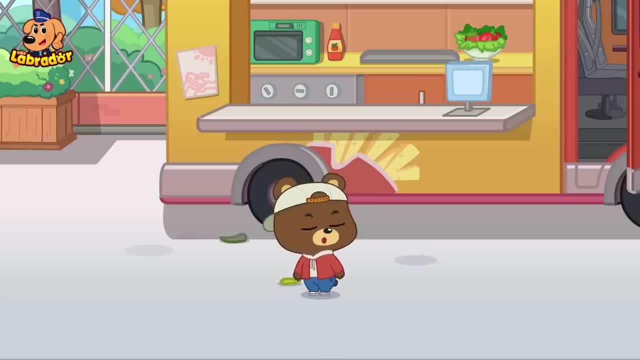 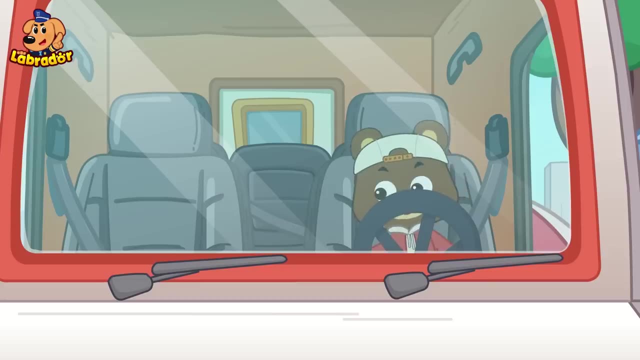 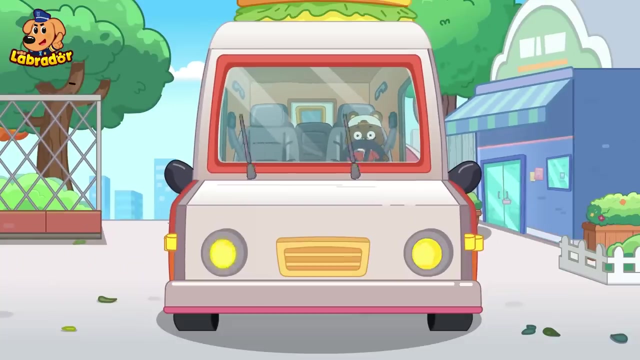 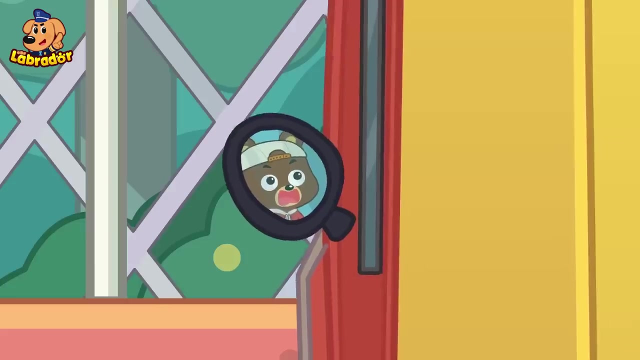 Come on, Please have some. Whoa, Hey, Whoa, Vroom, vroom, Let's go. Hey, Uh-oh, What's going on, Huh, Ah, Oh, no, Stop right now. Vroom, vroom. 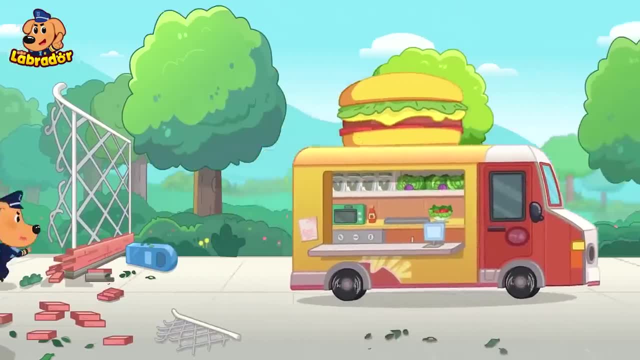 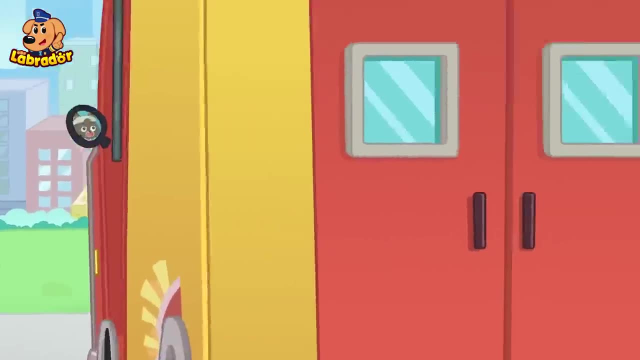 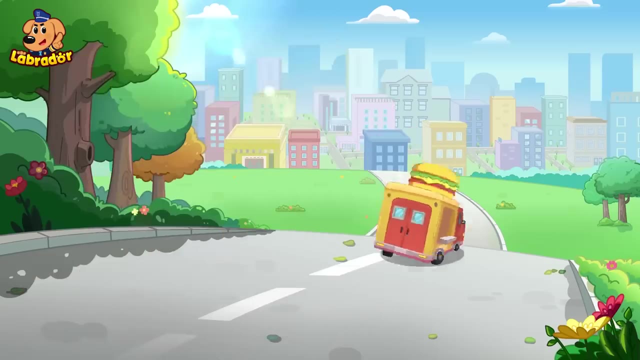 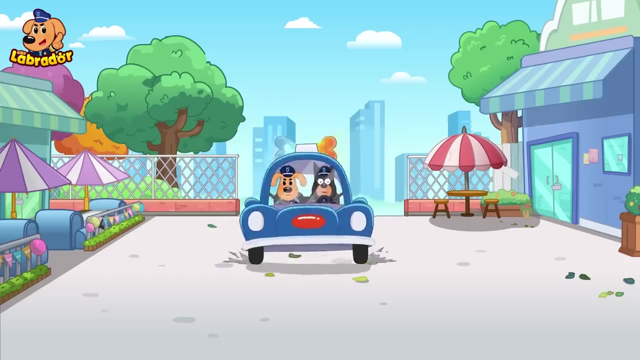 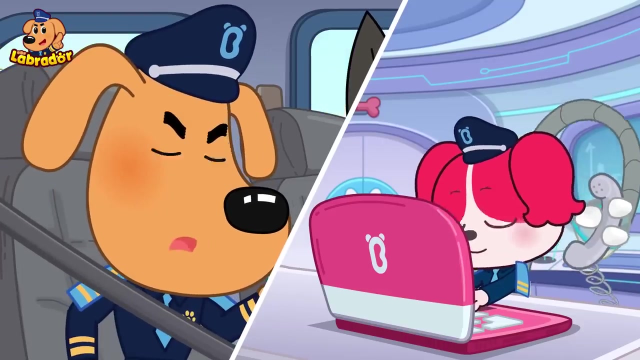 How do I stop this Little Bear Watch me. Ugh, Oh no, It's heading downtown. Get in the car. Papillon Sheriff, Labrador, A burger truck is out of control and Little Bear's in it. We need your help. 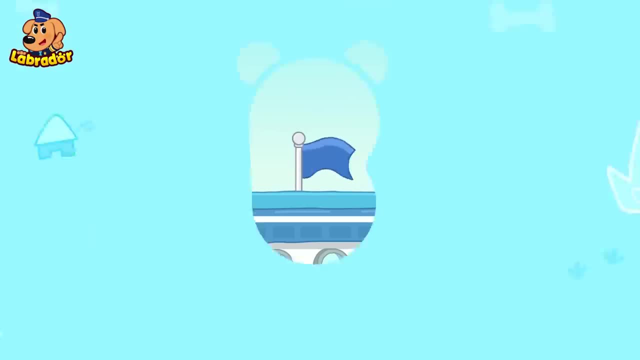 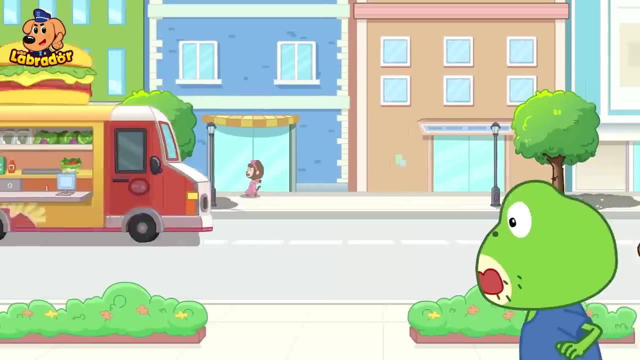 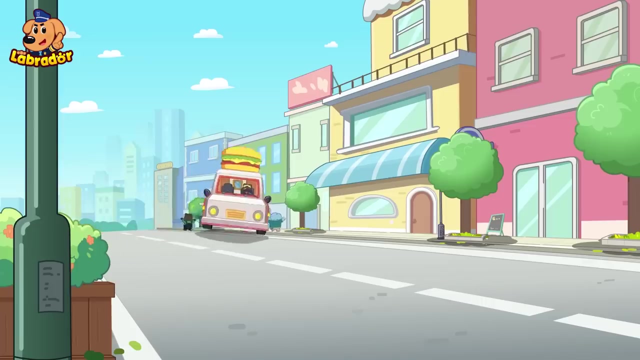 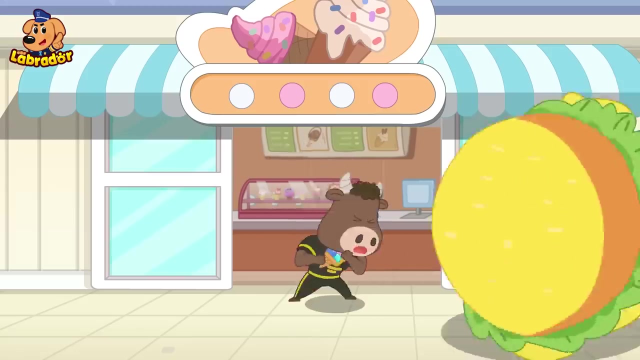 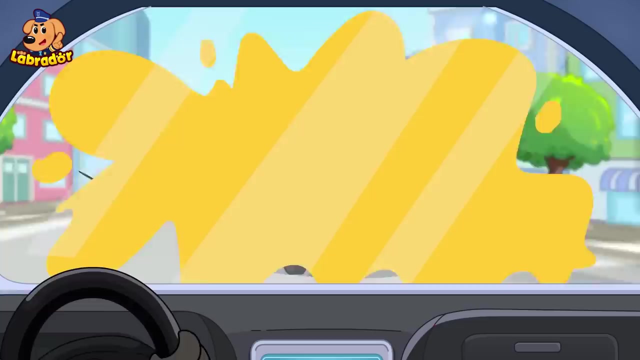 Got it. Oh Ah, Ah, Help, Oh, Ooh, Oh, Oh, Ah, Ah, Ah, Ah, Ah, Ah, Oh. no, Huh, I can't see anything Papillon's here. Papillon follow the truck. 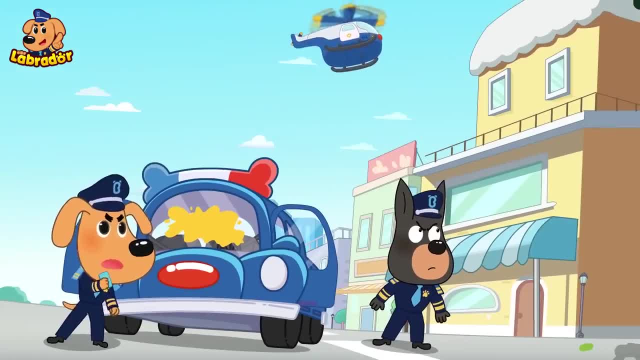 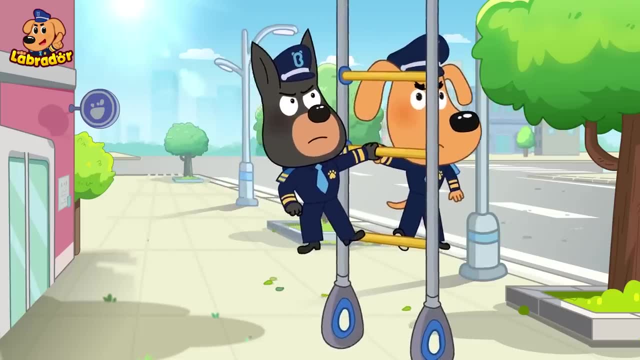 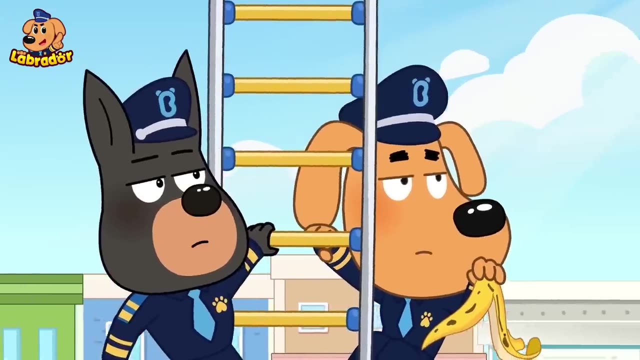 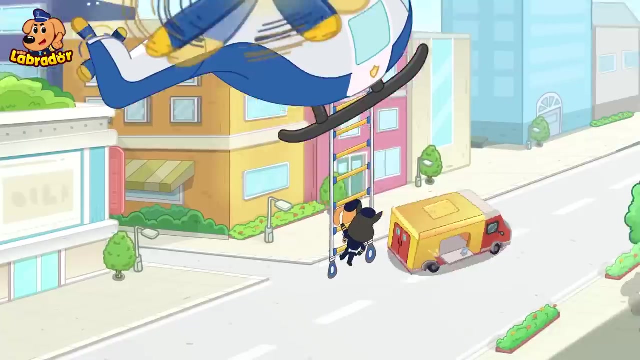 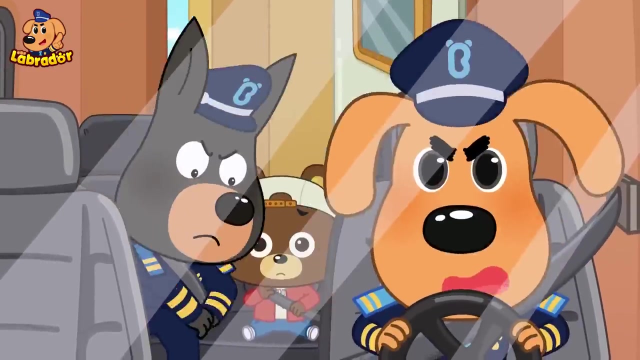 Got it. Hey, Hey, Hey, Ah, Hey, Hold on tight, Get us on top of the truck. No problem, Leave it to me. Papio, Sorry my mistake. Yeah, Sheriff Labrador, Fasten your seatbelts. Hold tight, I'm gonna break. 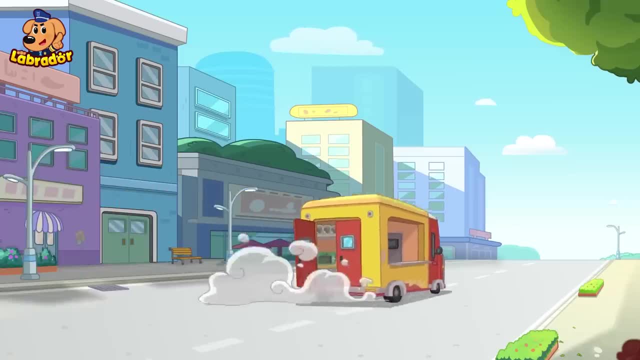 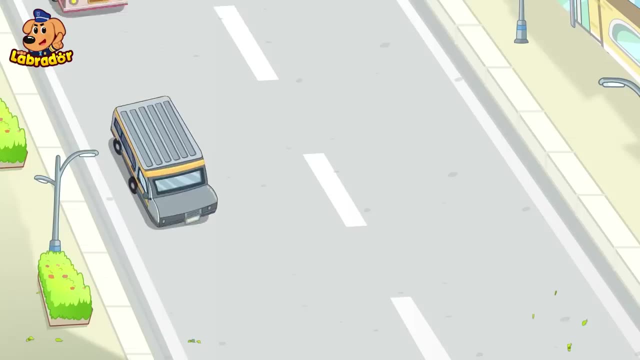 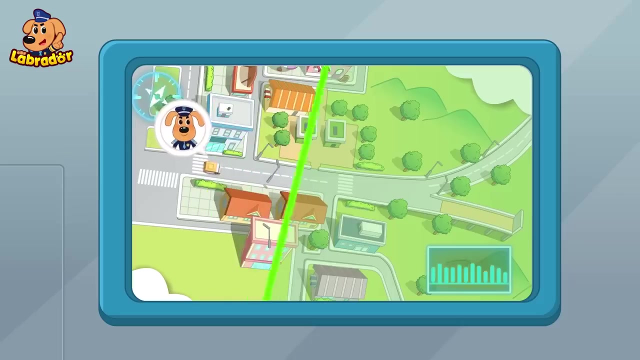 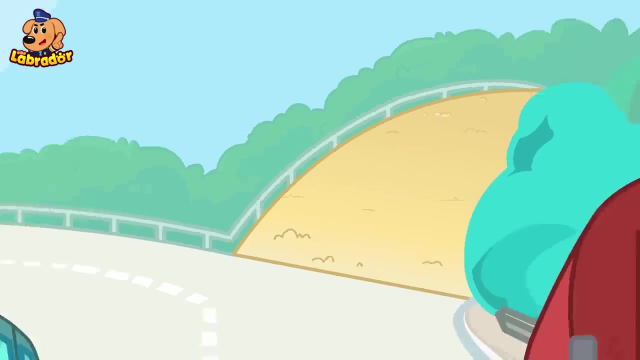 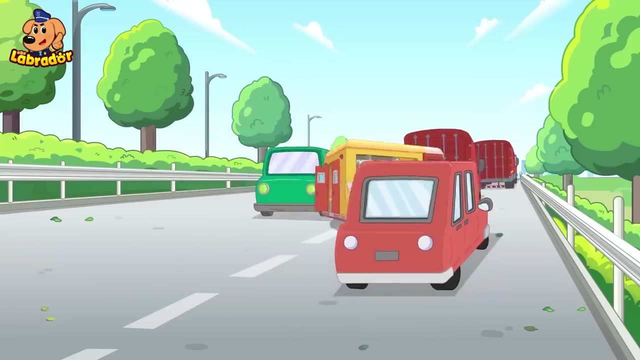 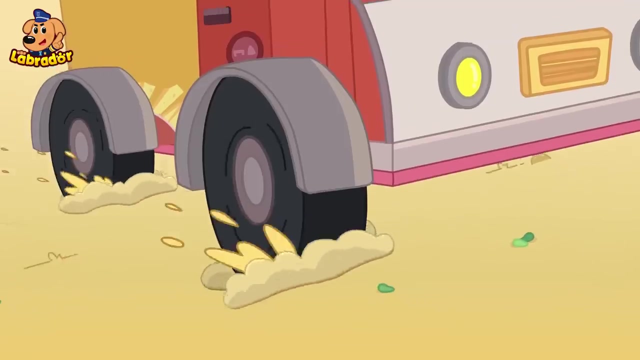 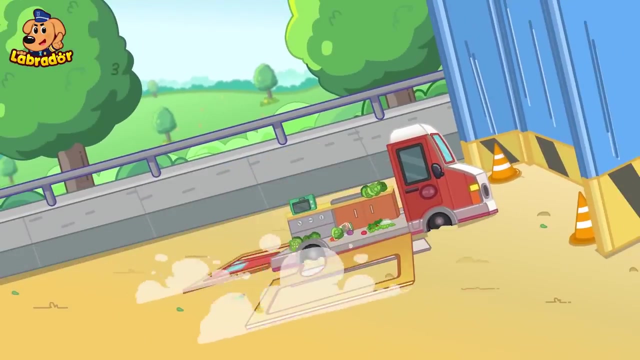 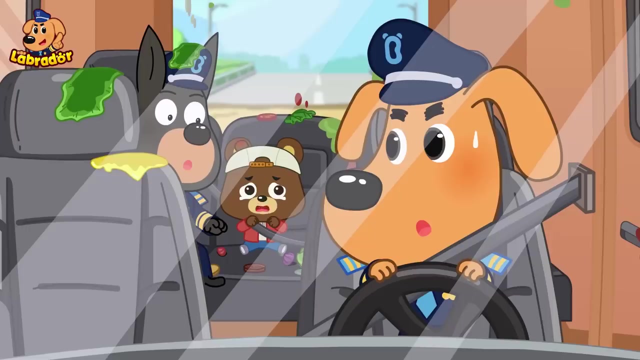 Oh no, The brake's broken. Papio, Where can I make an emergency stop? There's an emergency lane ahead. Got it Too many cars ahead? Leave it to me Sit up straight. Hold on tight. Phew, That was so scary. I'll never play in the driver's seat again. 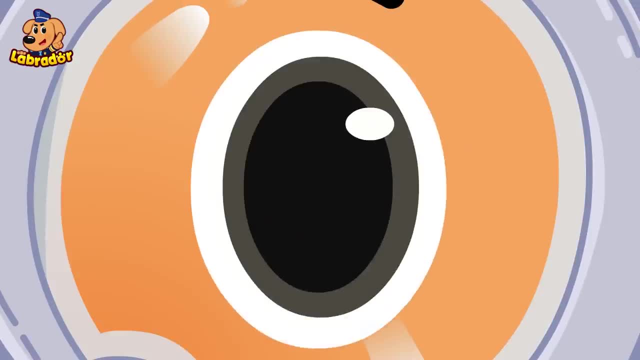 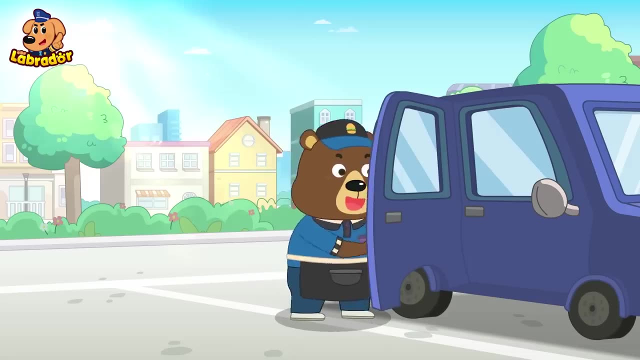 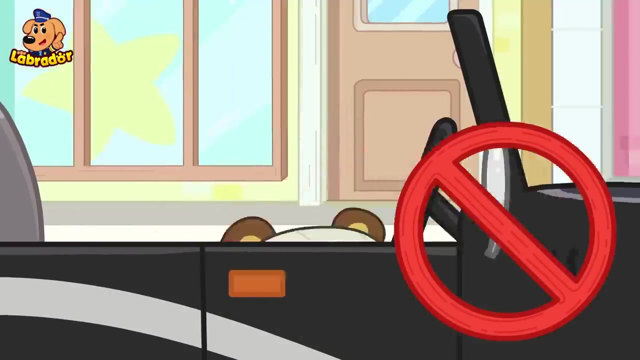 Ha ha ha, Sheriff Labrador, Sheriff Labrador, Safety talk Kids. when you ride in a car, always sit in the back and fasten your seatbelts. Never stick your heads or arms out of the window or play in the driver's seat. 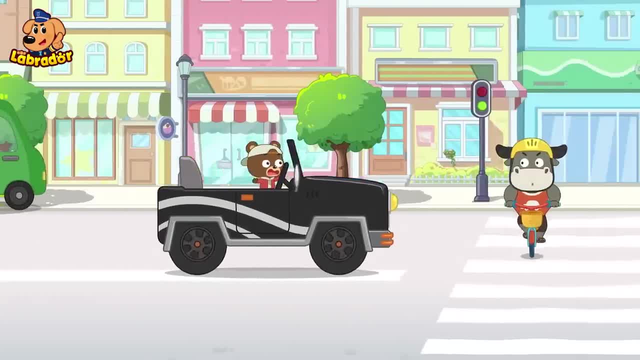 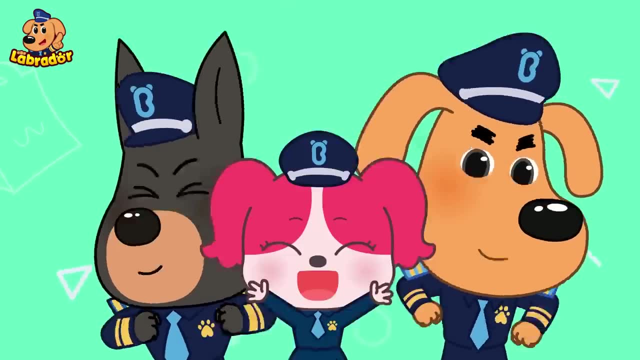 If you start the car by mistake, you can cause a serious traffic accident, hurting yourself and others. Let's stay safe when we're outside and when we ride in a car. Woof, A big tornado. Here's your balloon, Woof. 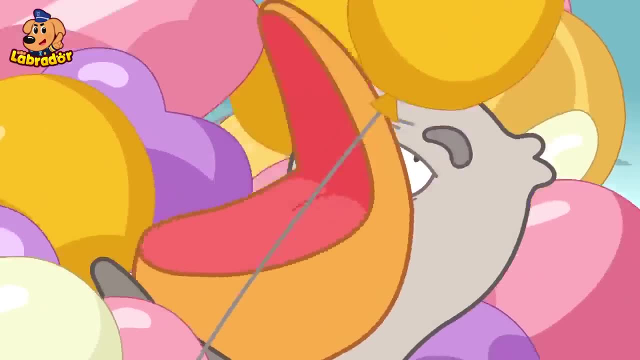 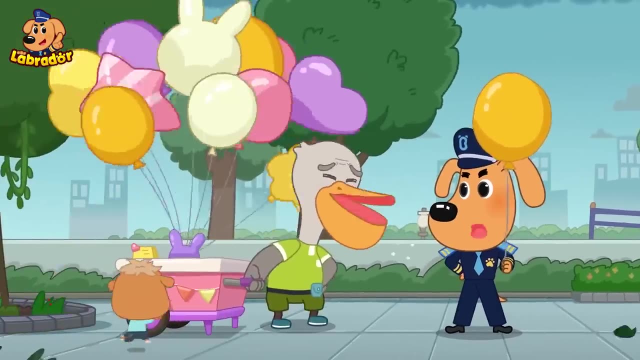 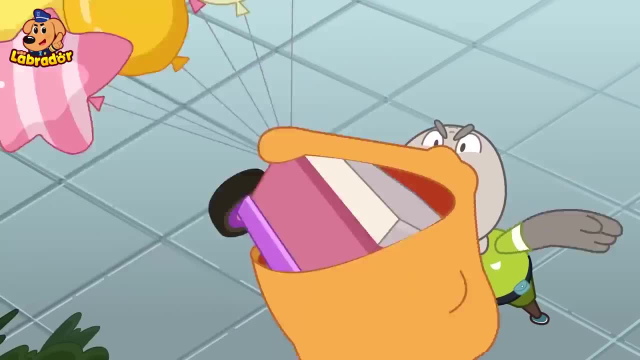 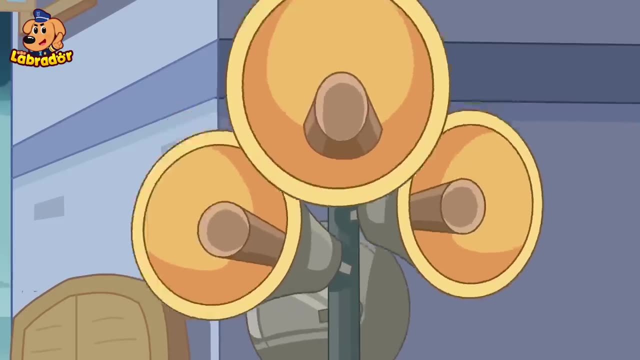 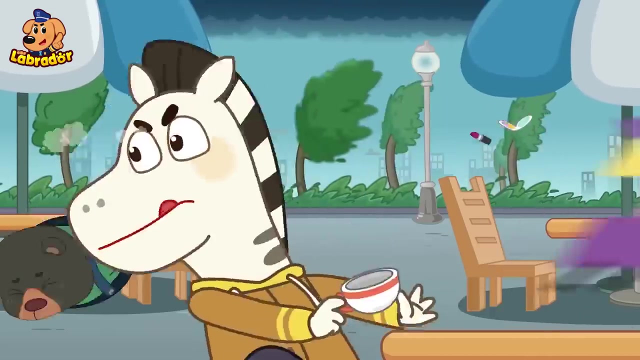 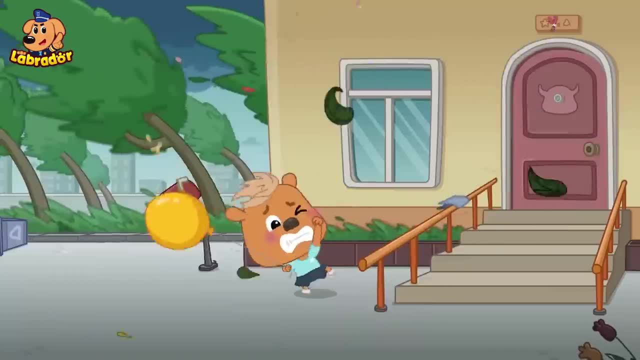 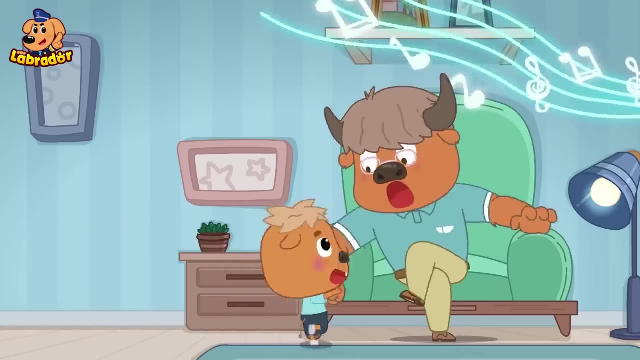 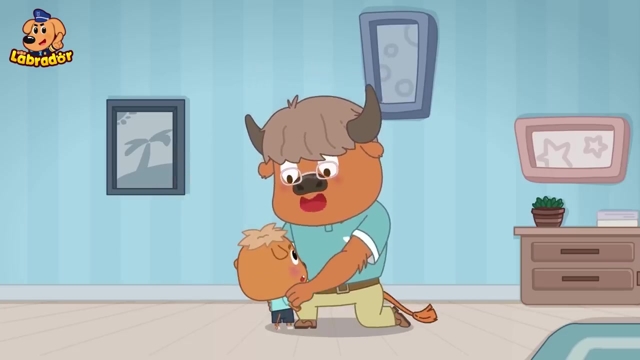 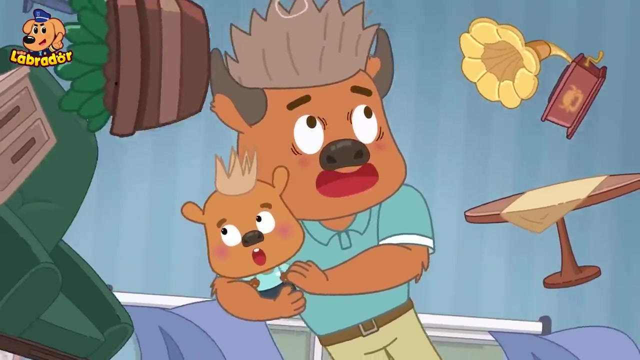 and prepare for the tornado. Aaaaah, Ouch Daddy, we need to go to the basement. A tornado is coming, It's okay. it's okay, Our house is very strong, But Don't worry, Relax Aaaaah. 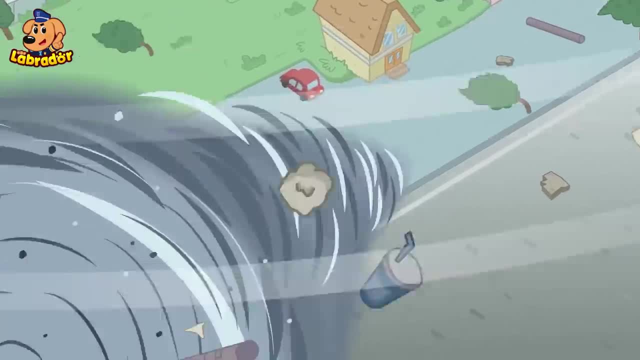 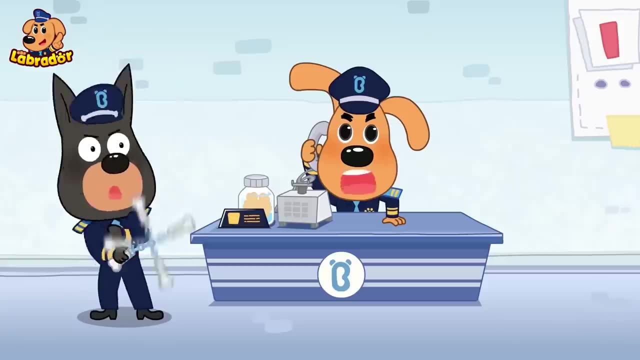 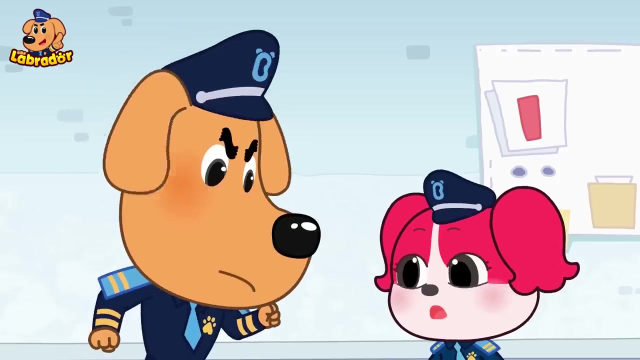 Ouch, Aaaaah, Aaaaah, Help, Woof, Hi, I'm Sheriff Labrador, Help, Hello. Hello Papillon, find out who called just now. Leave it to me. Found it. The call was from Mr Yak's house. 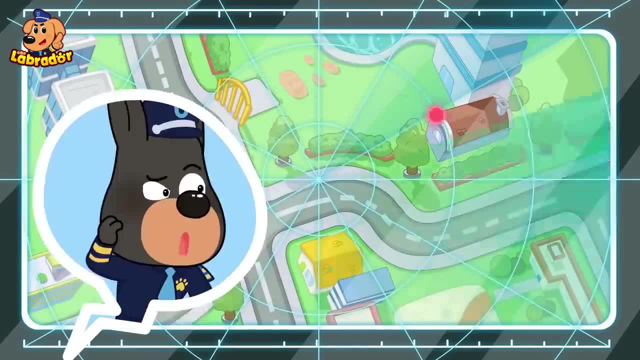 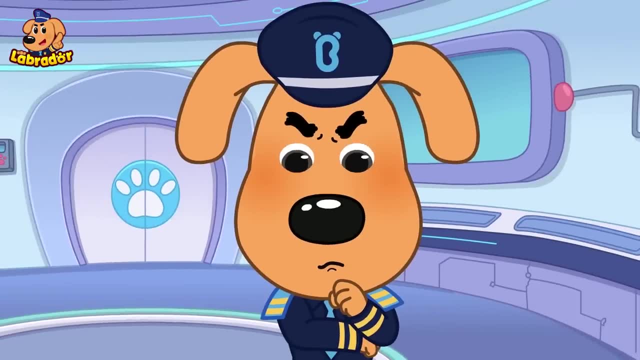 This is the location. This is strange. Why does it keep moving? It's moving so fast and in circles. It can't be. They're caught up in the tornado. Huh, Let's go. Uh-huh, Let's go. 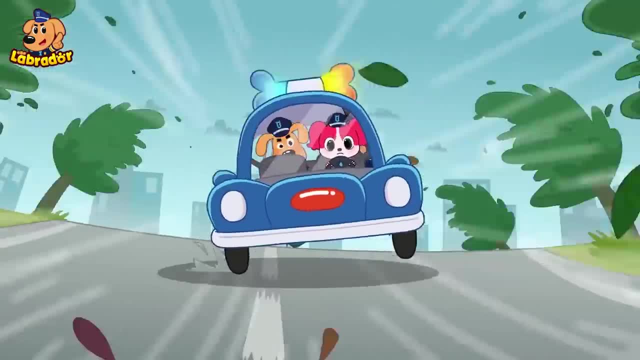 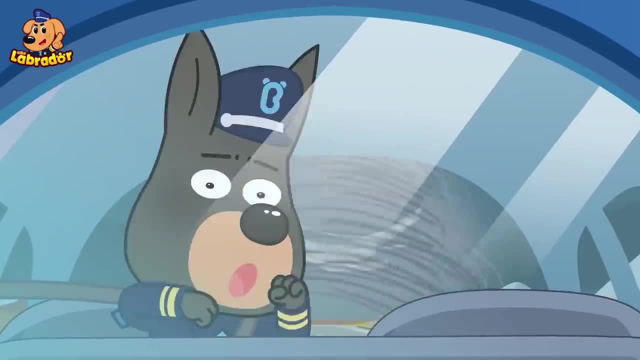 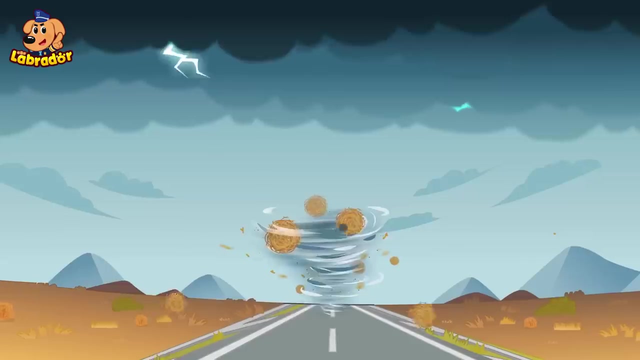 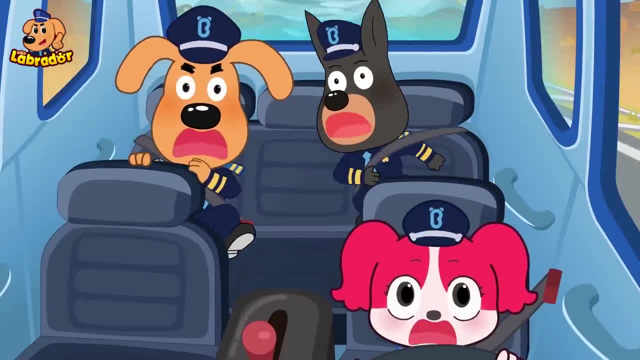 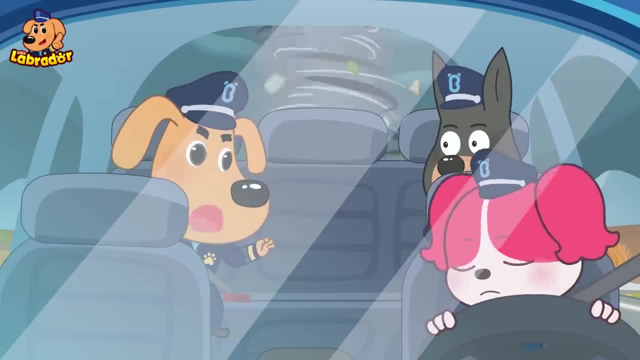 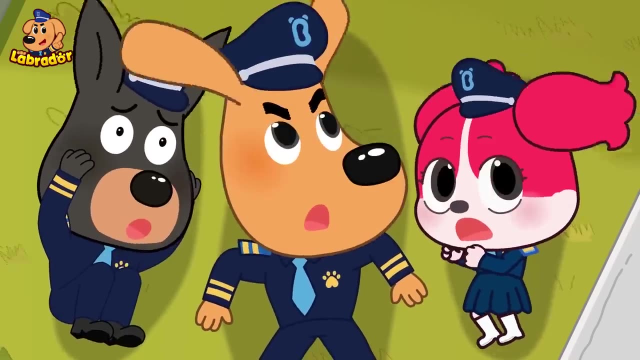 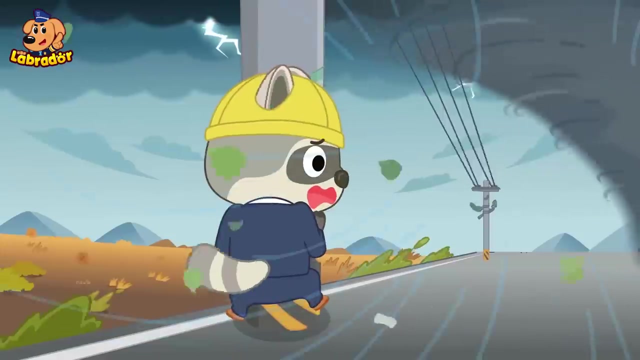 Ah, Ah, Huh, Oh no. Ah, It's a giant tornado. Ah, Everyone, get out of the car and go to low-lying places. It's coming. Watch out, Mr Raccoon, Don't stand next to the telephone pole. 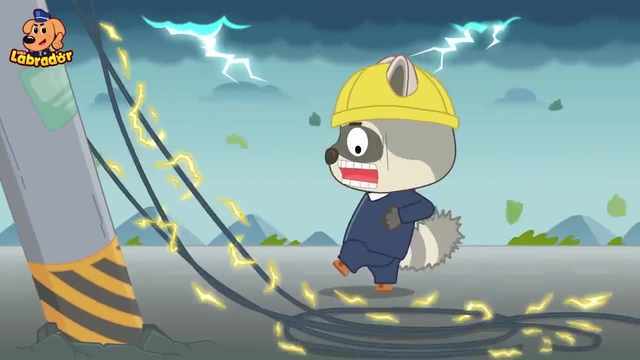 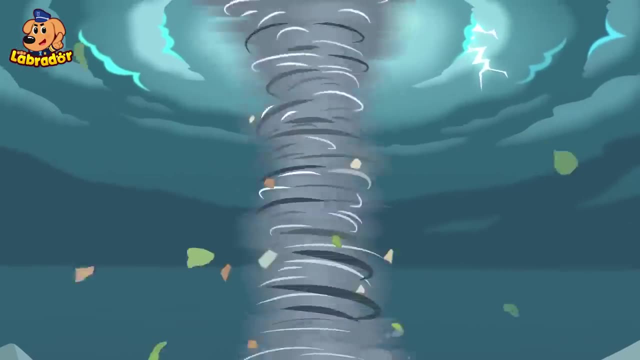 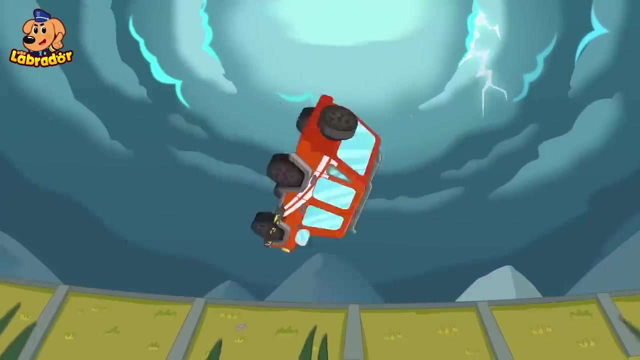 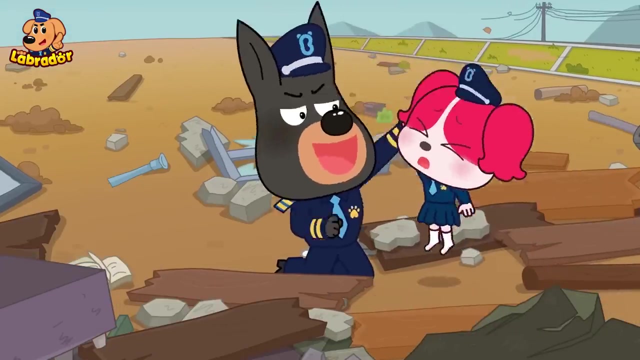 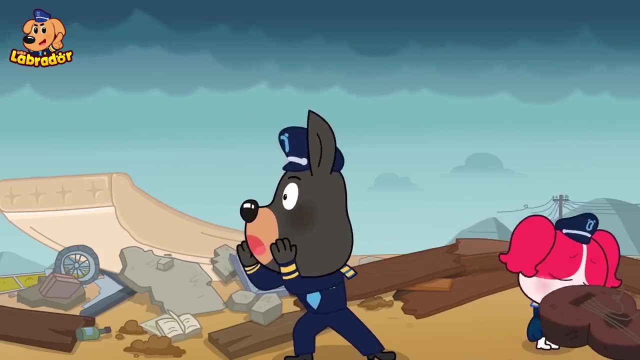 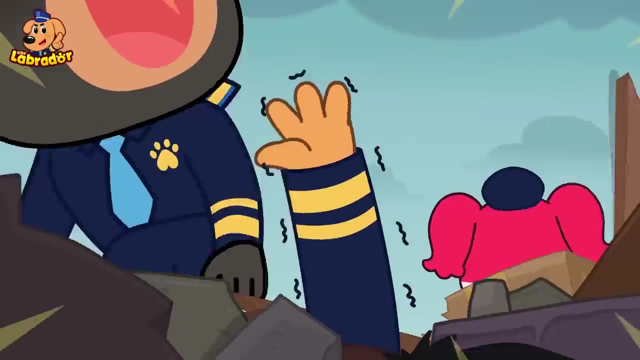 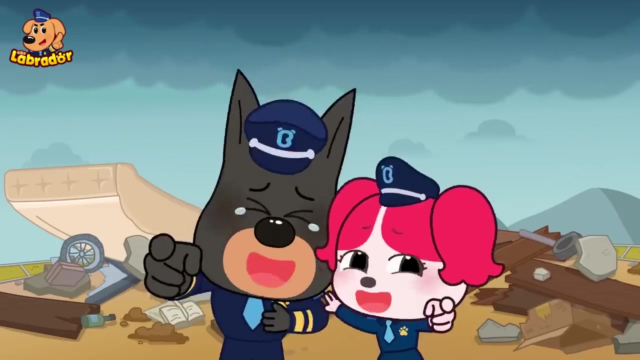 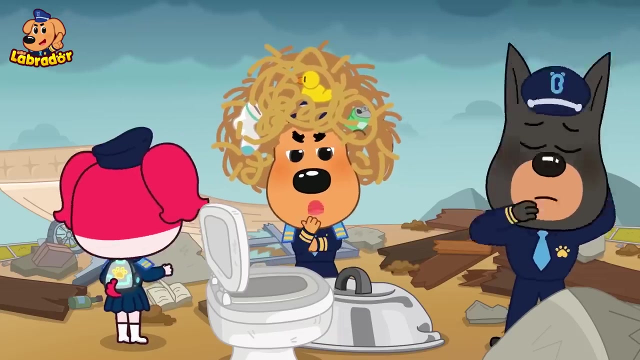 What, What was that? Watch out, Get down. Where's Sheriff Labrador? Sheriff Labrador, Sheriff Labrador, Where is he, Adobe under your feet? Ouch, Ouch, A pot lid and a toilet. These are things in a house. 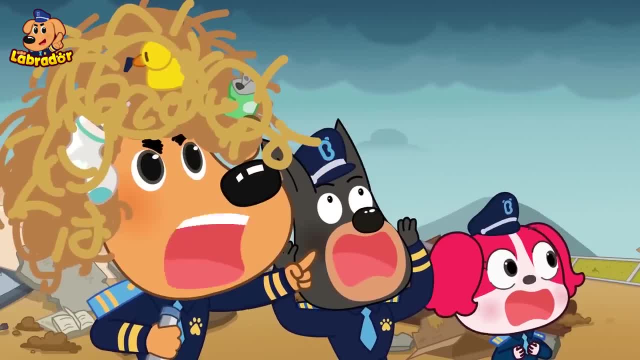 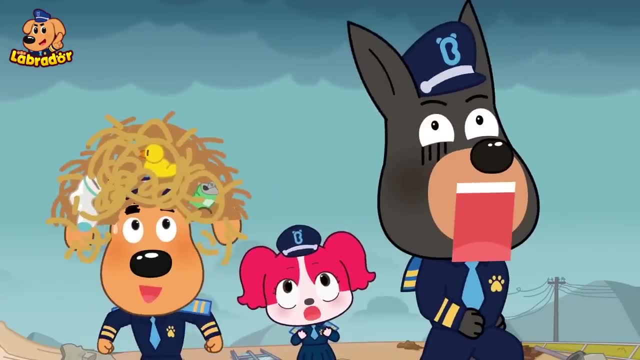 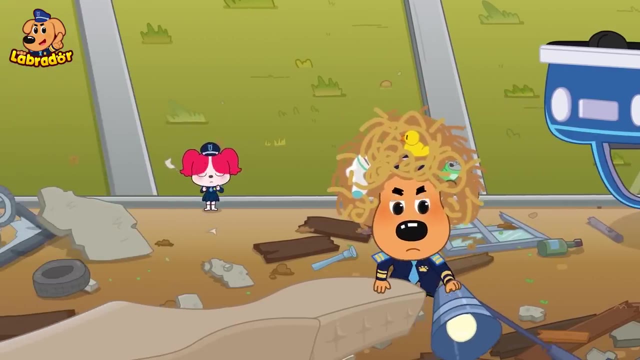 Oh no, The yaks are in the tornado. They may get thrown out at any time. Yobi Papillon, Let's go save them. Okay, Oh no, The car can't be used now. What do we do? I have an idea.